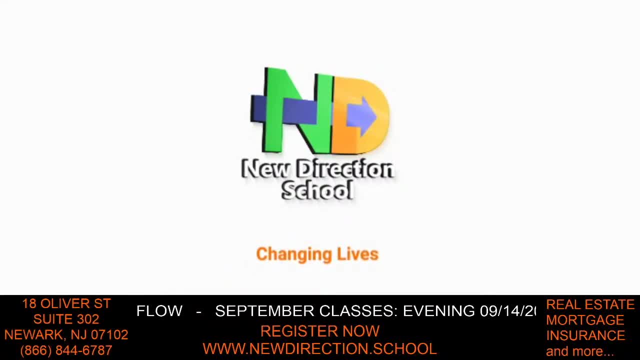 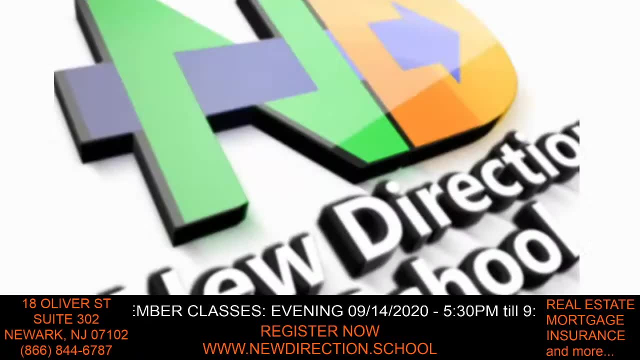 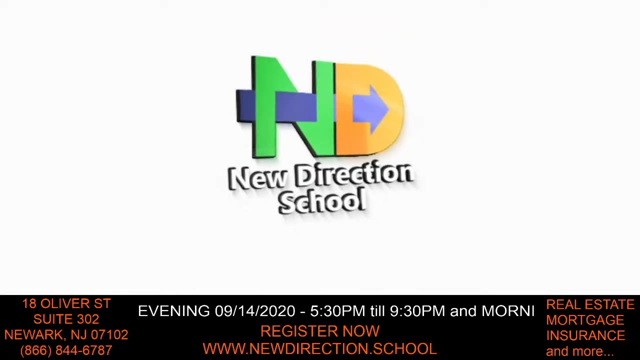 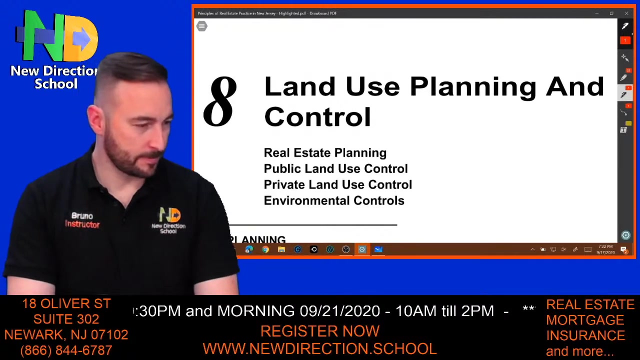 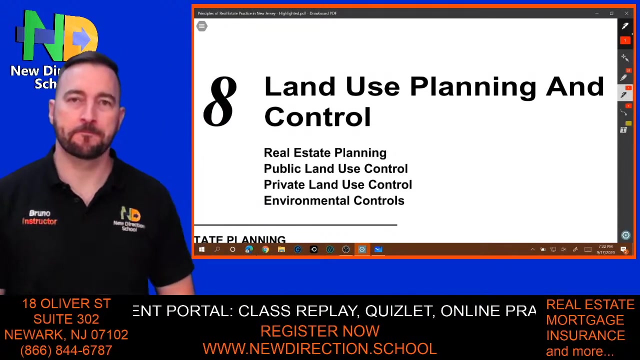 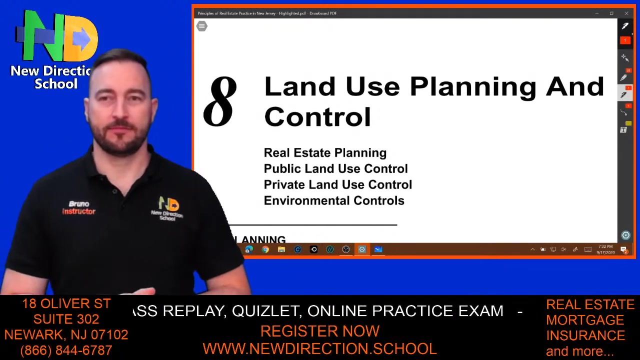 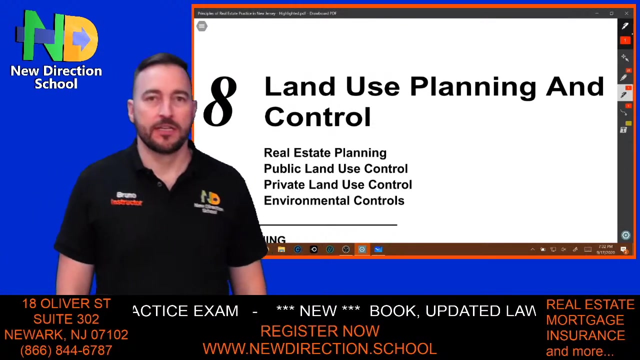 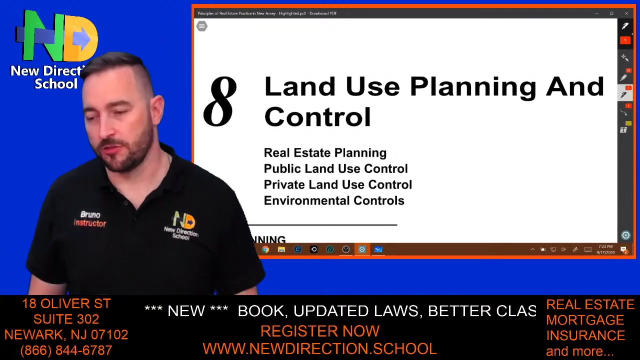 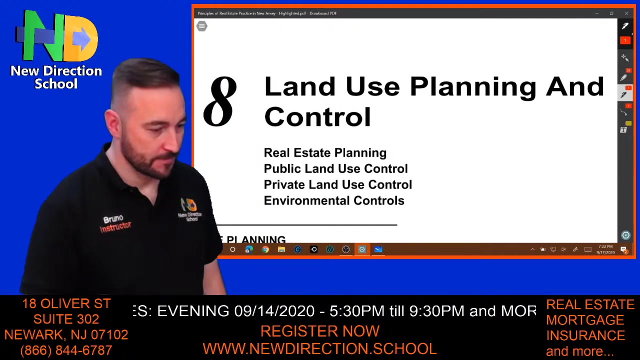 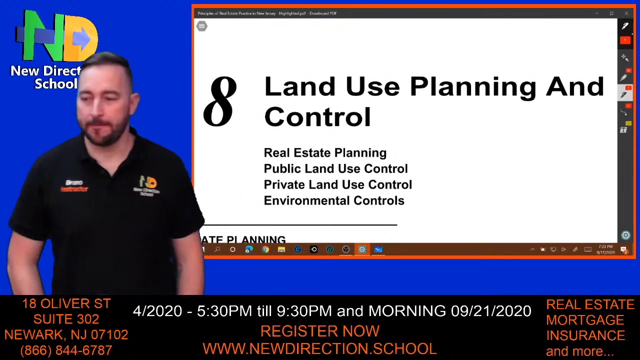 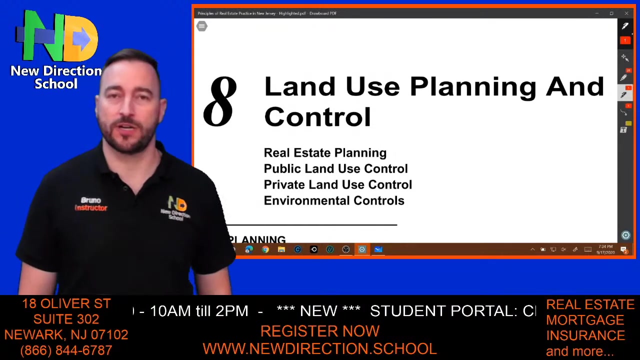 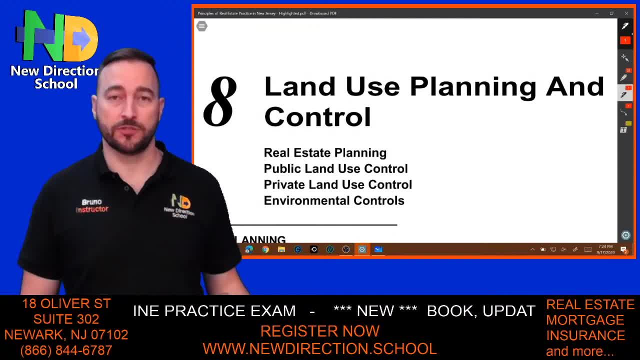 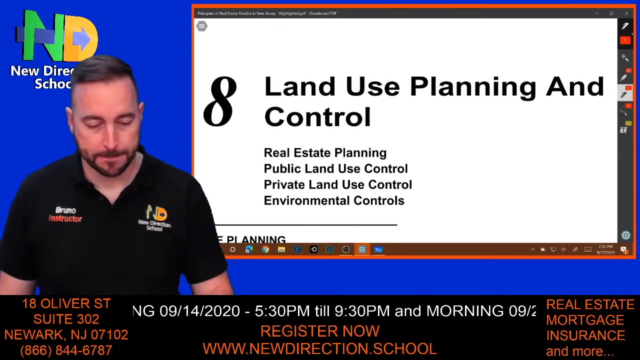 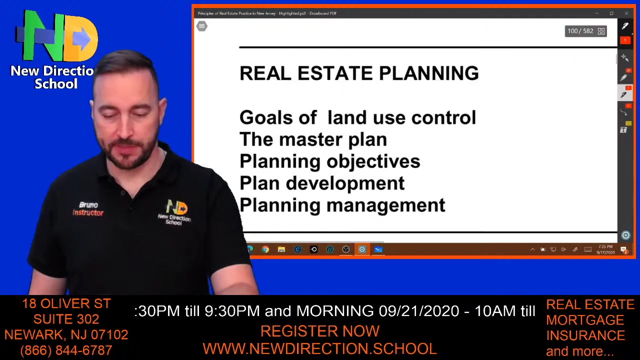 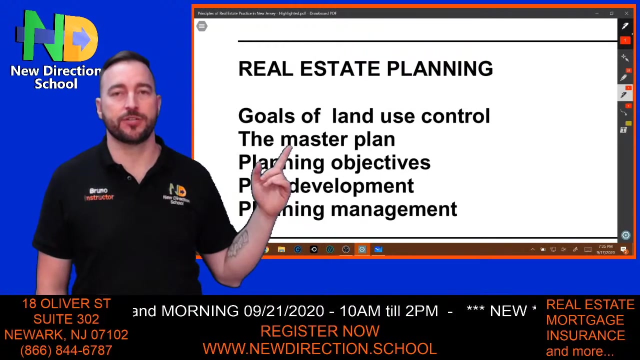 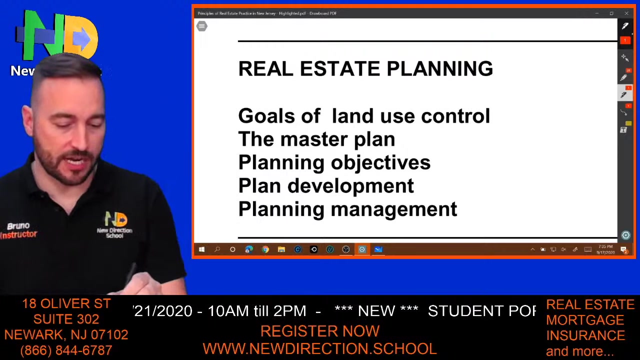 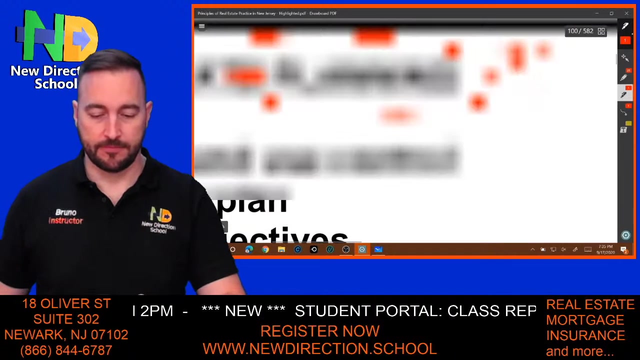 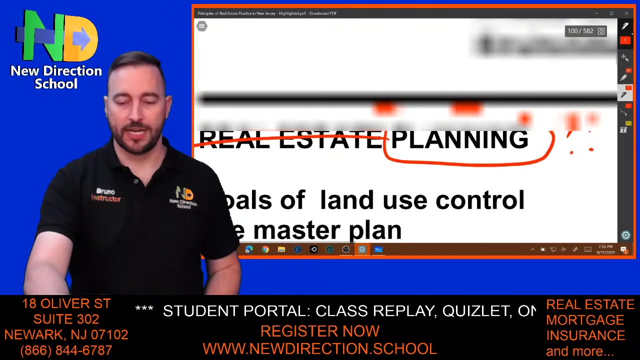 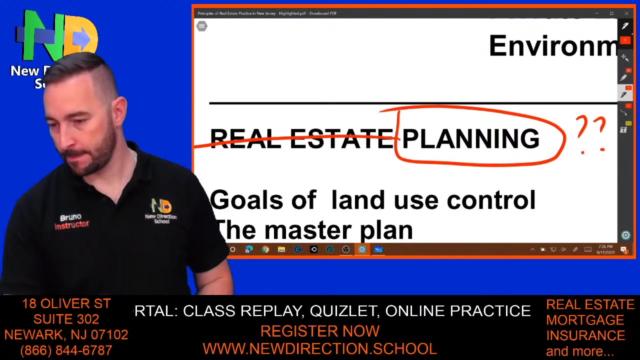 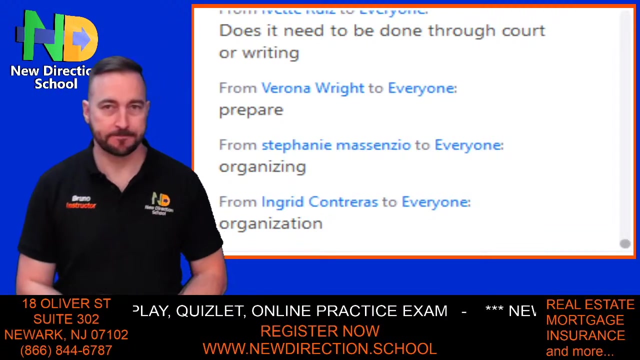 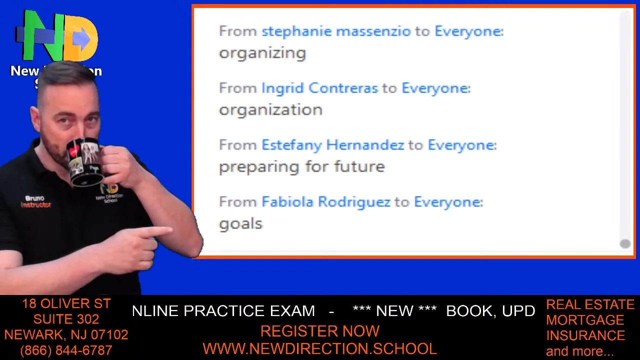 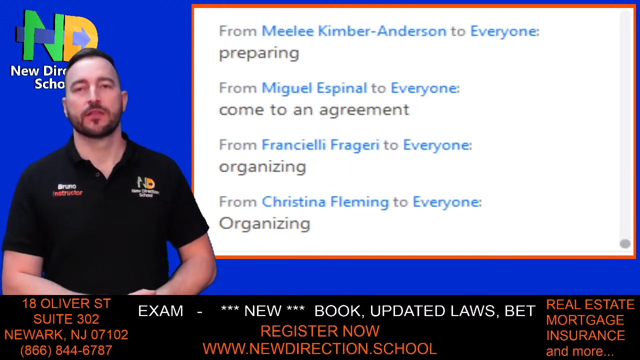 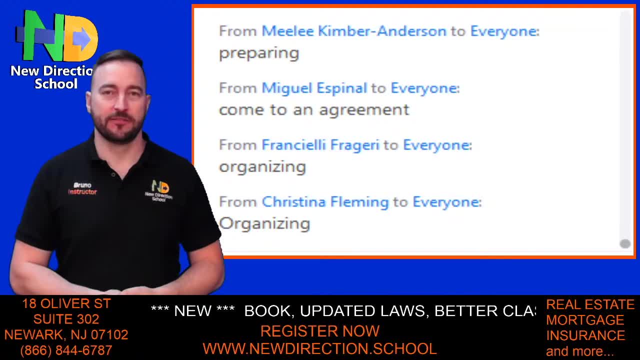 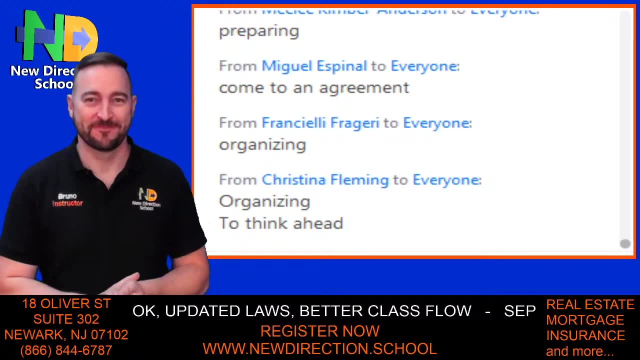 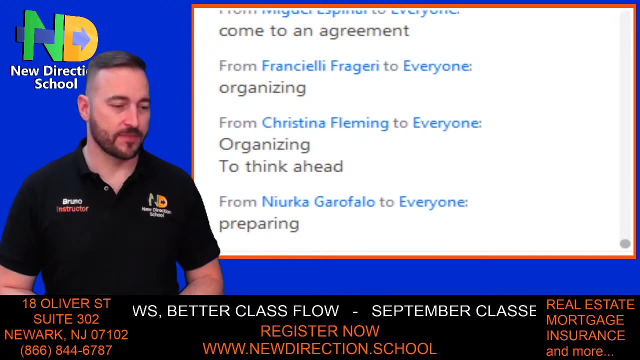 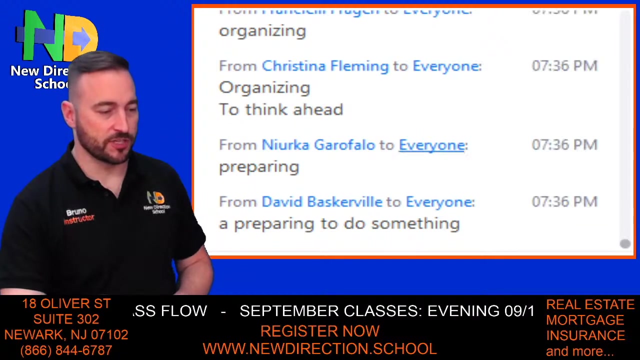 Okay, Organizing, Organizing. Okay, You guys are just repeating. It's easy to say: This is what you do. You write whatever Stephanie said. That's what you have to write there. Okay, But make it easy, Think ahead. Absolutely Preparing. All right guys. So why? Oh, now we're getting somewhere. David Preparing to do something And Fabiola wrote goals. 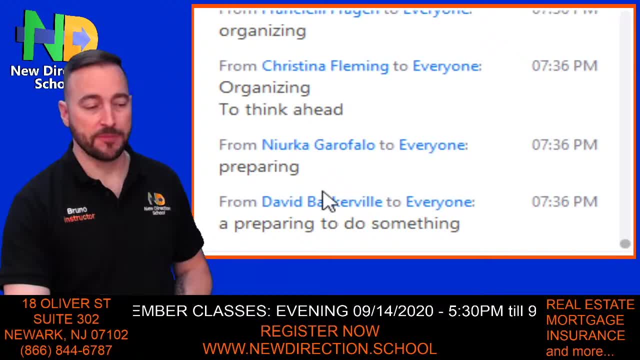 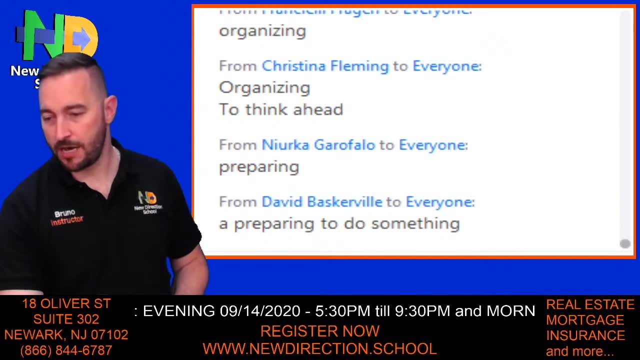 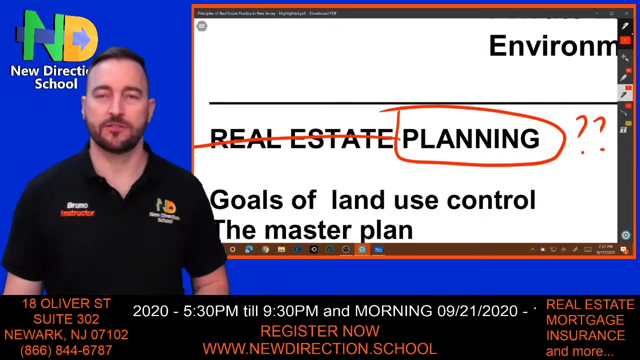 Goals. The reason why we plan, and what planning means, is we're preparing to do something. We have an objective, We have a goal, Right. So I'm pretty sure that nobody here started coming to this class without planning. And I'm not talking about planning of the hours you need to take. I'm not talking about planning of the amount of weeks that you're going to be here. I'm talking about you thought. 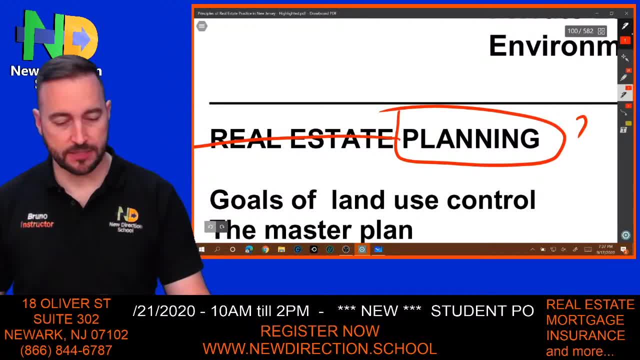 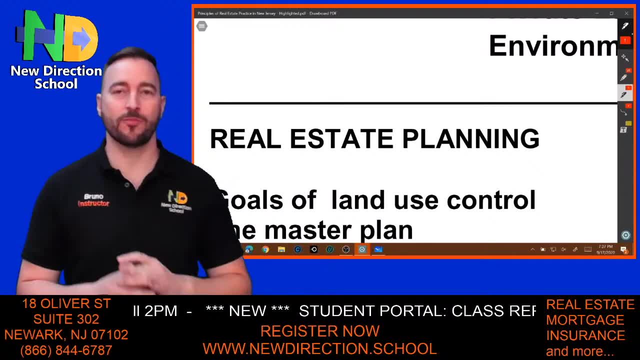 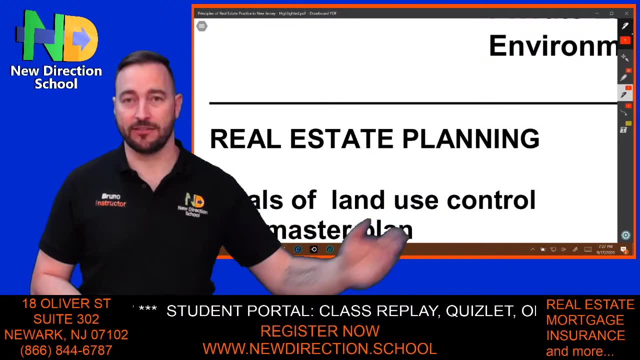 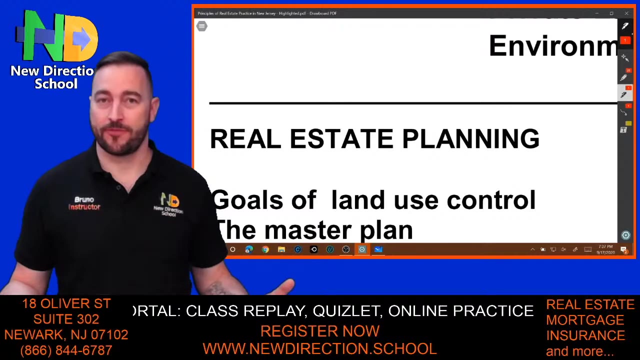 Real estate might be a good opportunity to question mark Right. Real estate is a good opportunity to question mark. Everybody has their own Right, So you have what's called a goal, an objective. for you to reach that goal, You need to plan. Some people are blessed with: Hey, let's see where it takes me, Right, So no planning whatsoever. But the majority of the people, unfortunately, need planning. 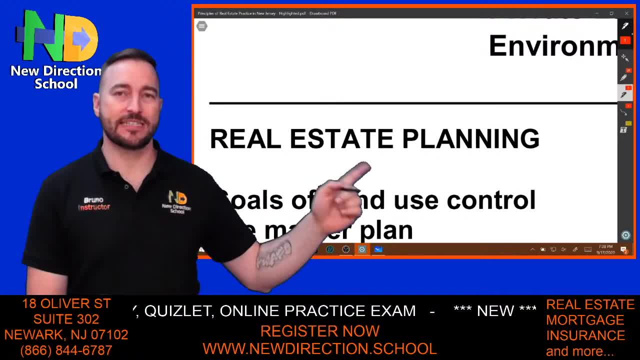 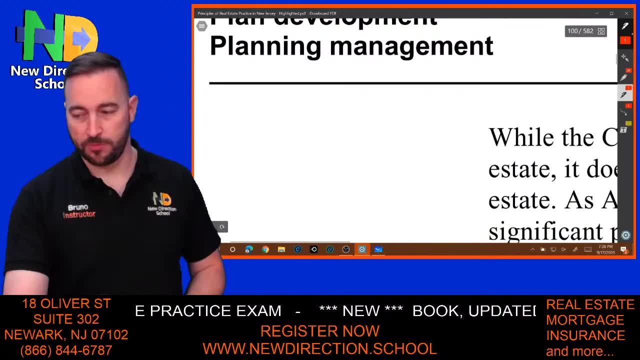 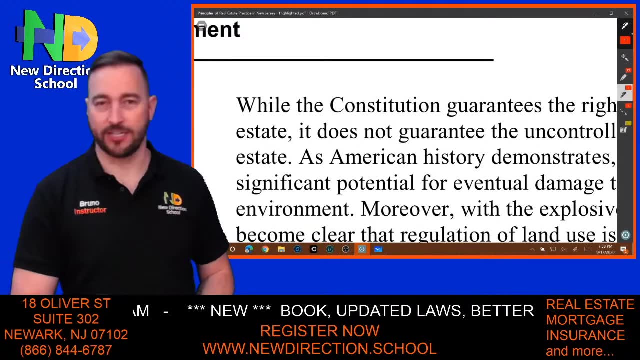 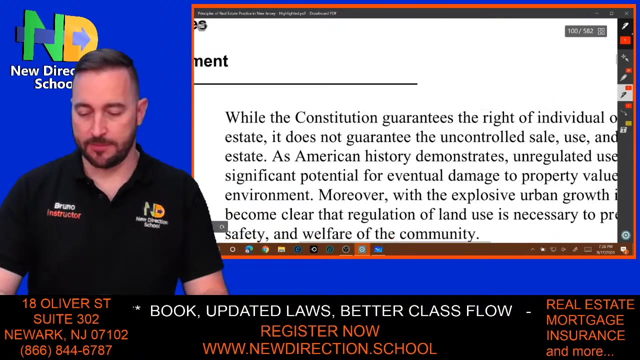 To reach the goal. So, ultimately, real estate planning is reaching goals and planning to reach those goals, Okay. So why is that so important? Oh, you got Laura in the house. Hey, Laura, Planning to build for the future? I just saw your message now, Sorry. Planning to build for the future, for instance? Yeah, it could be for building. It could be any type of goal in the future. 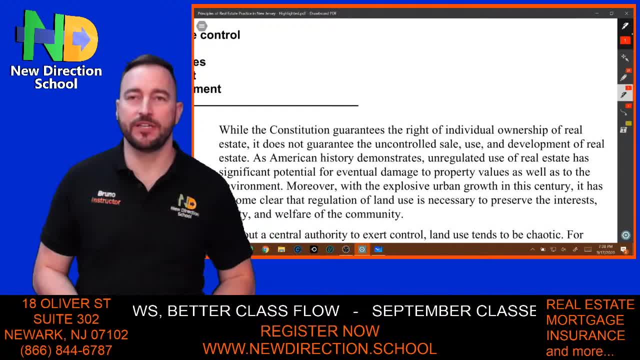 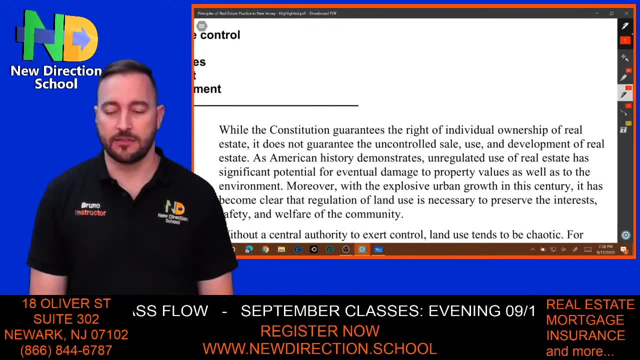 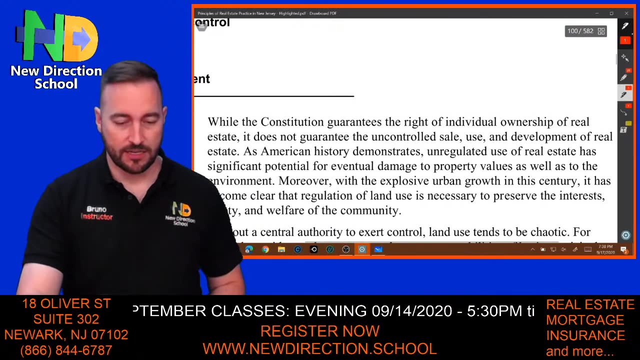 So, while the Constitution guarantees the right of individual ownership of real estate, it does not guarantee the uncontrolled sale, use and development of real estate. As American history demonstrates, unregulated use of real estate has a significant potential for eventual damage to property values, as well as to the environment. 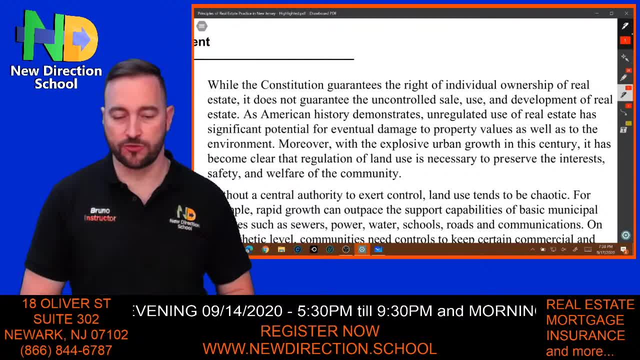 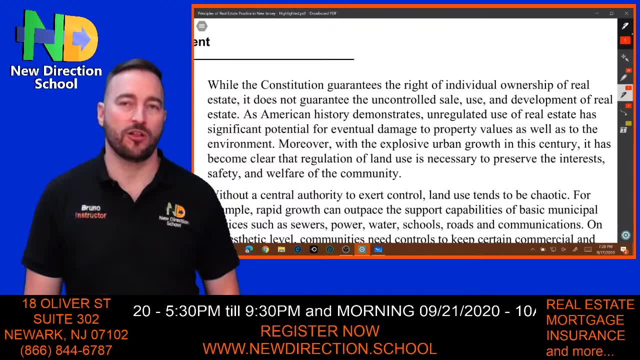 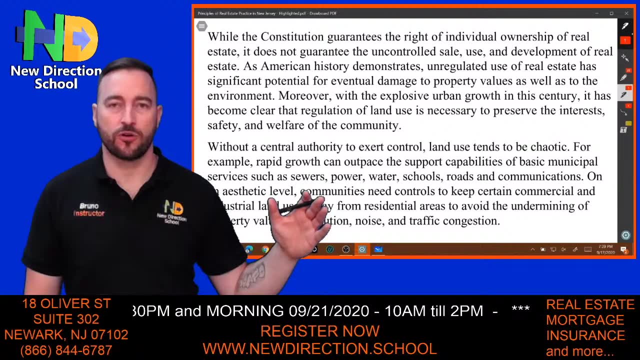 Moreover, with the explosive urban growth in this century, it has become clear that regulation of land use is necessary to preserve the interests, safety and welfare of the community. So without a central authority to exert control, land use tends to be chaotic. 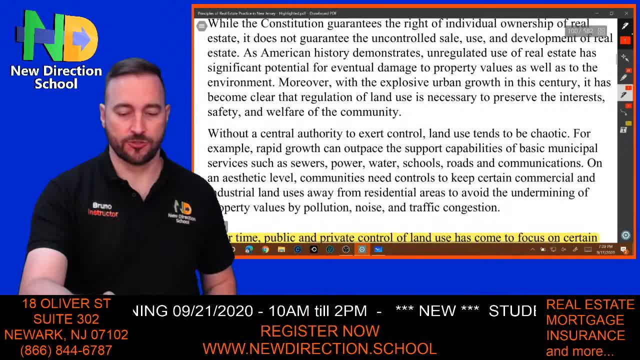 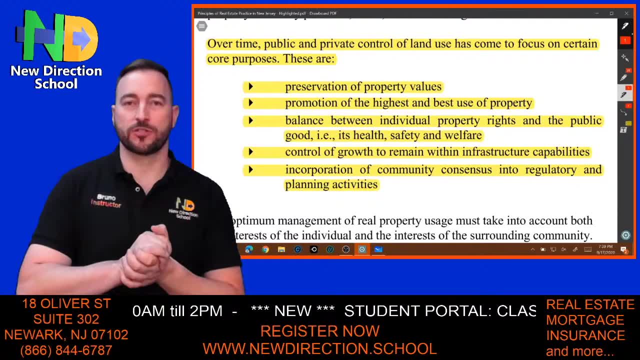 And we're going to stop right here for a second. We're going to actually jump this For a second. Here's my question: Who remembers? Raise your hand, Who remembers the story of the three little pigs? Raise your hand, Three little pigs. 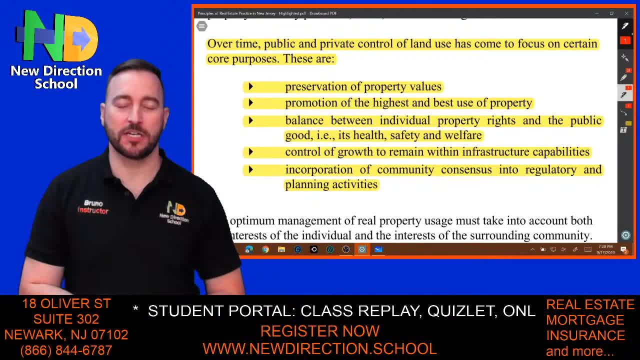 Okay, cool. So who wants to tell me the story? I'll give you the mic. Who's going to be? One person, Tell me the story. Don't be shy, Chris. you want to tell me the story, Even Liz. 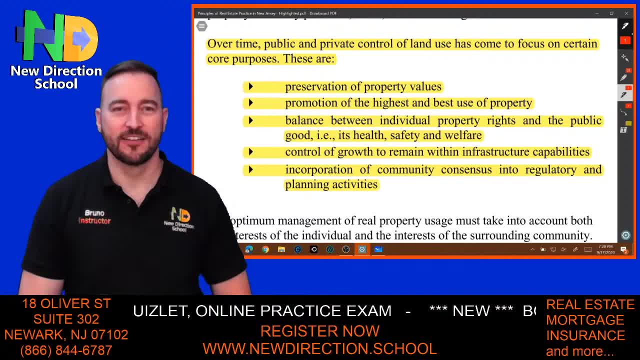 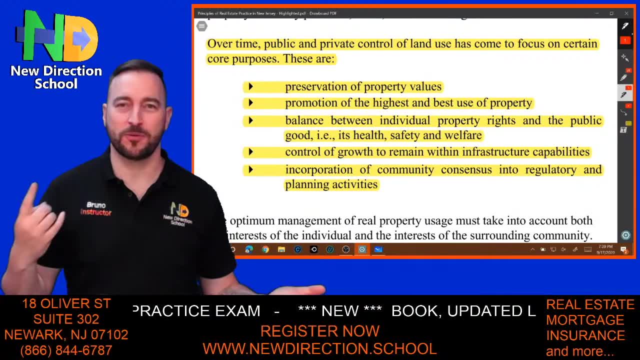 All right, Francielli, Mirka, Vanessa, Stephanie. Who's going to tell me the story? Robin, Come on, Don't be shy. Just one person, Verona. you want it Okay, So hold on. 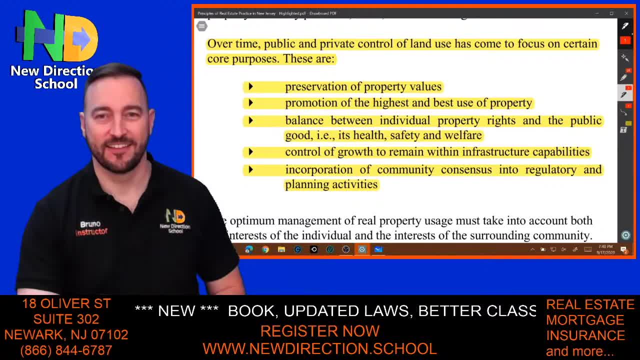 You're going to speak. Good, Yesterday was milk, Today is three little pigs. All right, What's wrong with this guy? Okay, Go ahead. Verona, You can speak. If you have a mic, you should be able to speak. 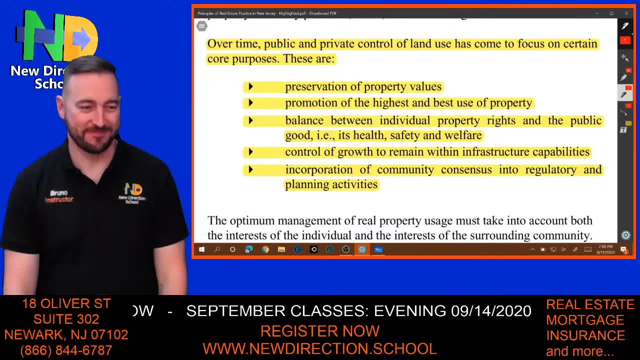 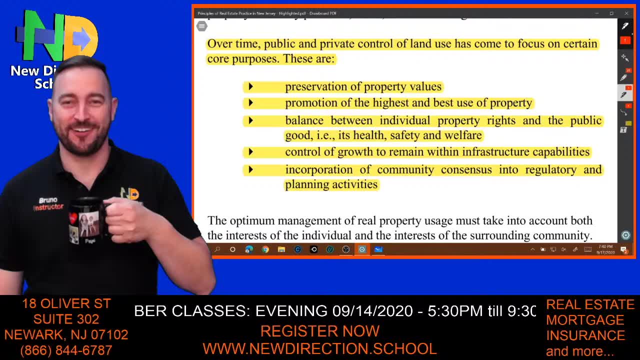 Let me in, Let me in. There you go. If you don't listen to me, I will huff and I'll puff and I'll blow your house down. Ah, we come with effects. All right, cool. So that's what the wolf was doing, right? 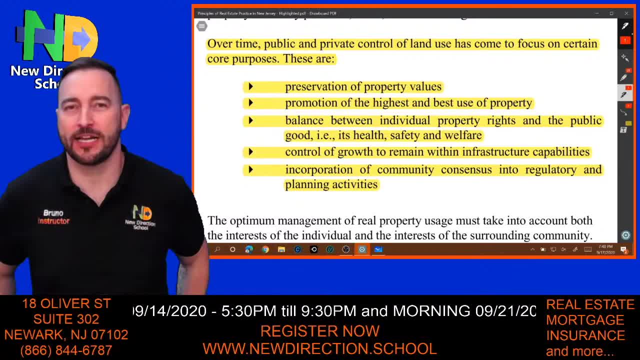 Now, what did the pigs do? They had what? What kind of houses? Straw, Straw One was. the last one was brick Very solid, Yep, very solid. So you had straw wood and brick, Very good. 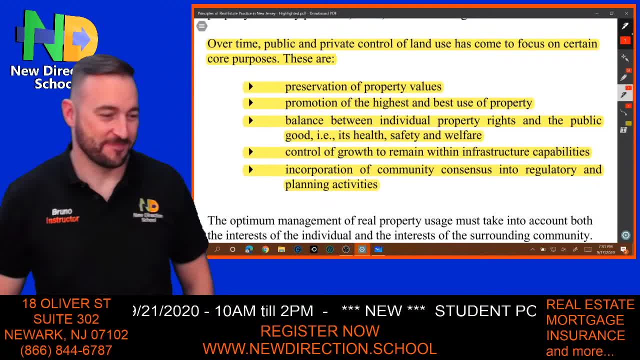 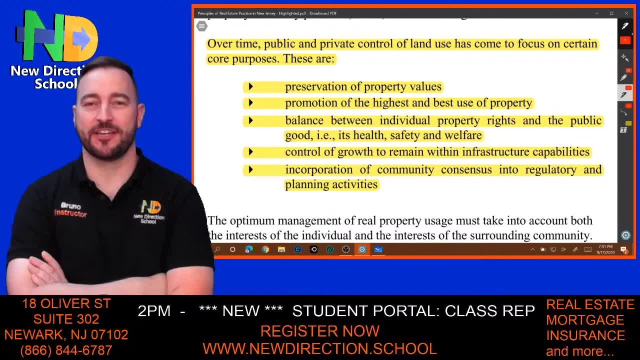 Okay, Cool One was like the. So they all, like, ran to each other's house until they got there. Okay, Why did they have to run to each other's house? That's the question. It wasn't the security, It wasn't you know, it wasn't the park. 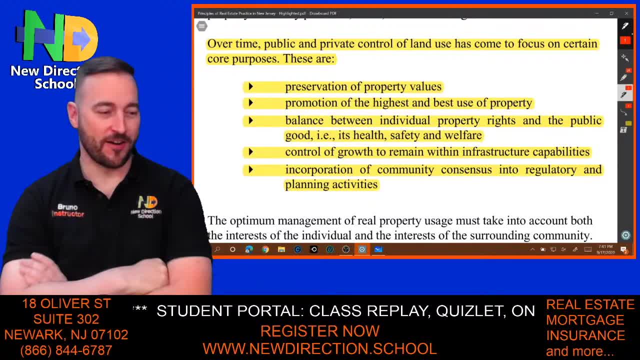 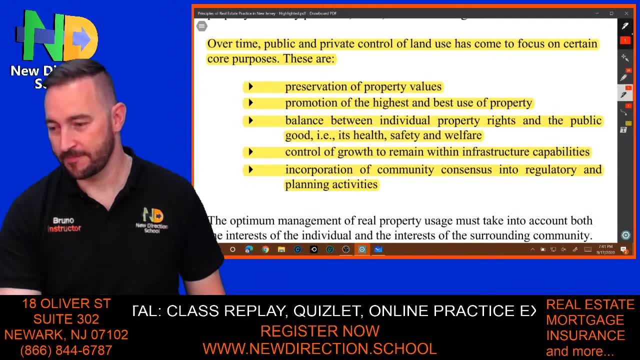 It was the foundation. Ah, there you go. All right, cool, I'm going to mute you for a second, okay, So why the three little pigs? Such an innocent story, right? But it's told to the kids about preparing, about foundation in your life, right? 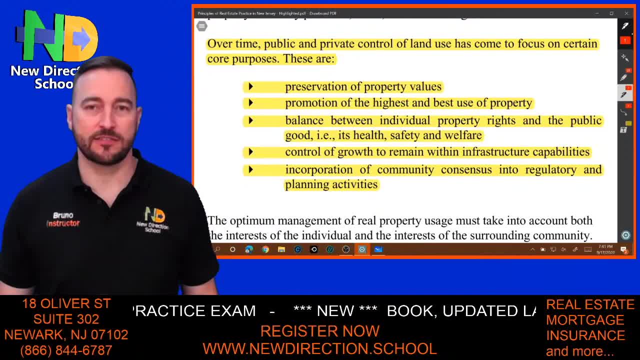 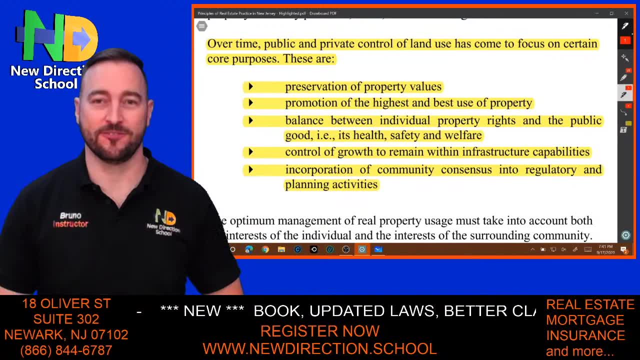 In buildings, in business, it's about foundation. So there's three little pigs and they all have their own attitudes, because that's about attitude and we all have our own attitudes, right, And one says: I'm going to build my house of straw or sticks, as somebody wrote, Robin, okay. 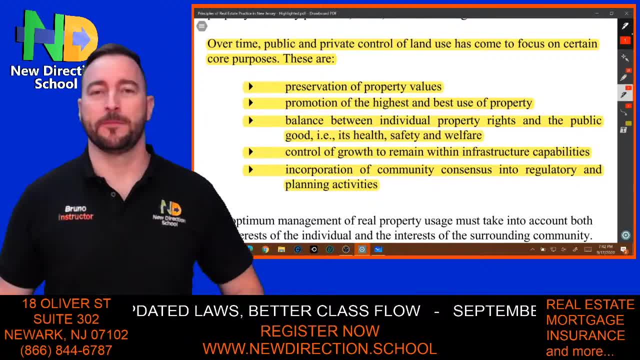 Right. And then the other one says: I'm going to build my house of wood, It's better. And then the other one says, Nope, My house is going to be a brick house. And then they made a song about it. 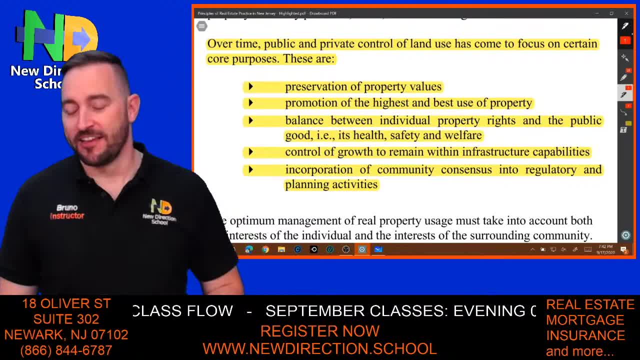 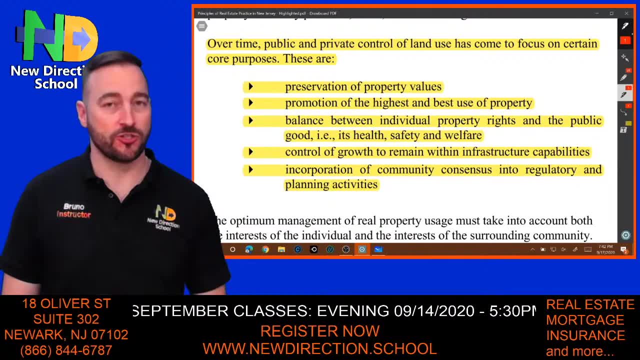 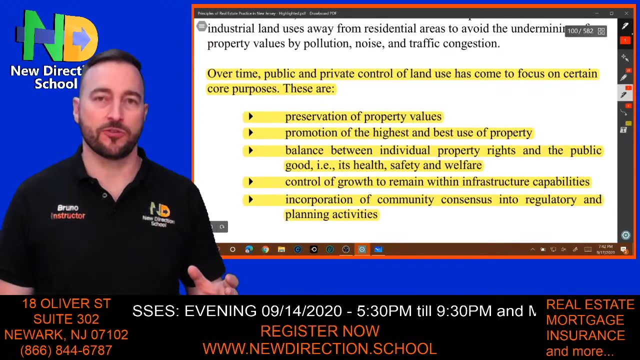 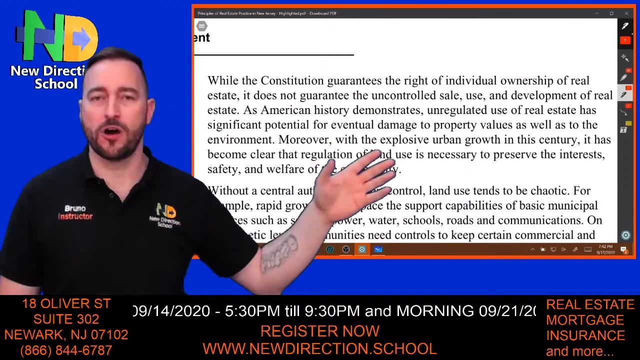 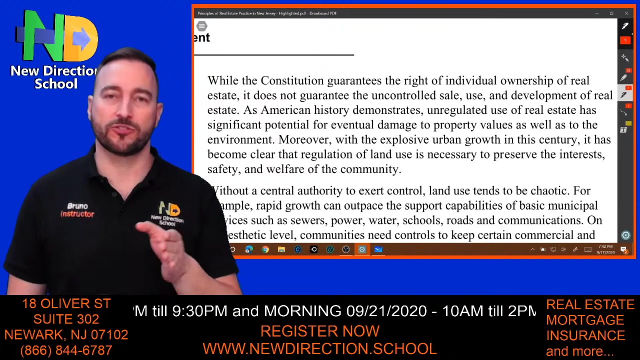 So my house is going to be brick. It's even better. What happened after was showing the world that if you don't have a proper foundation, everything could collapse, But not only yours, it could also endanger everybody else. So these rules and regulations that we're talking about that were created to. even though you have constitutional rights to your property, it's yours. you can do whatever you want. if it's going to affect the community, right then the government wants to make sure that you follow certain guidelines. you can still do whatever you want. you can build a house, as long as it's according to these guidelines. why? 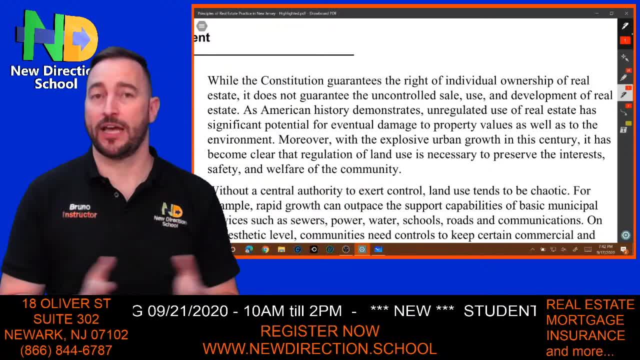 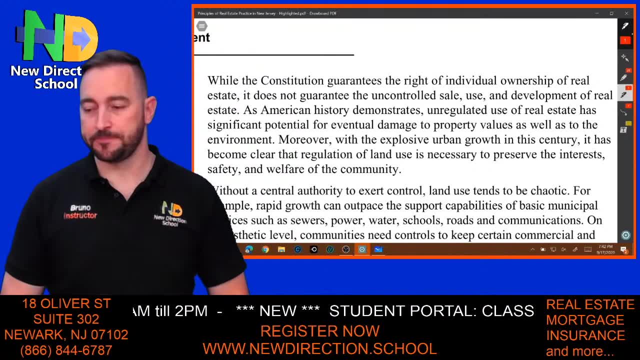 Because, as we know, we have houses that are attached one to the other, as an example, right, And if one starts a fire, all of them go right, If there's. you know, in certain areas of our country you still deal with this, but if there's a tornado, hurricane, whatever, your house goes because of the structure, other houses stay because of the structure. 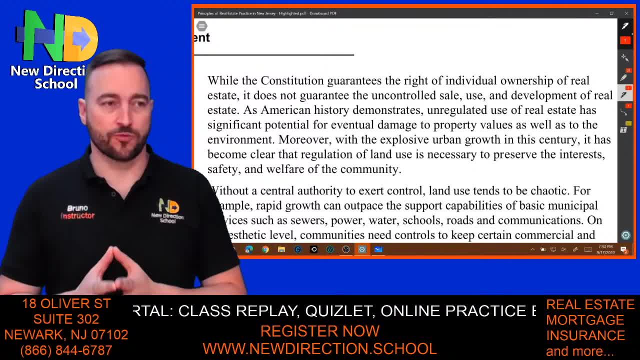 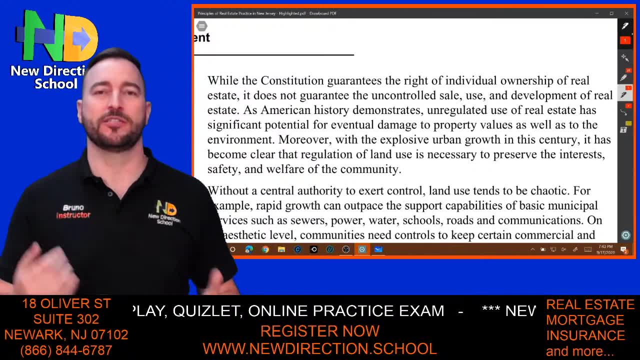 So the idea behind this is there are certain rules to protect the welfare of the community. It's not about, as some people tell me, oh Bruno, they just want to tax, they just want money. I want to build whatever I want in my house, but they just want money. 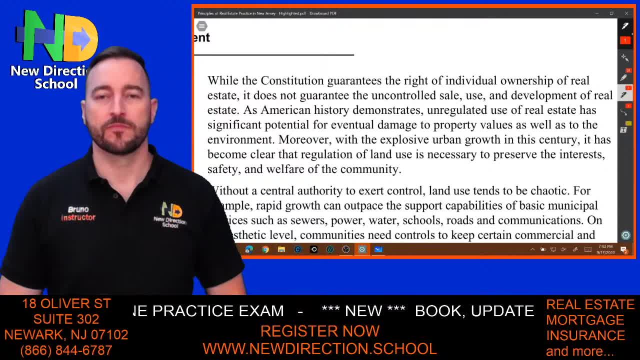 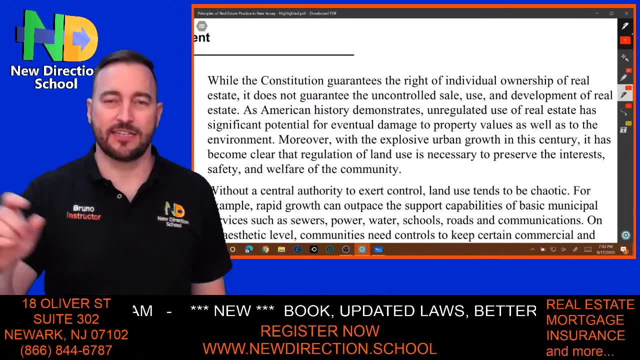 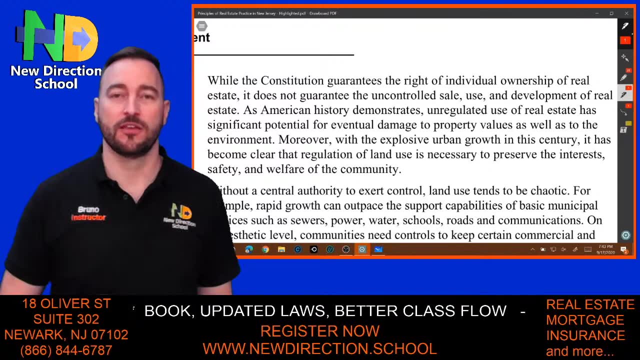 They want permits, they want this, they want that. No, Obviously money is involved, obviously, right, Every government wants money, we know that. and there's a little set aside for corruption, right, But most of it is towards infrastructure and making sure, planning, making sure everything is done right. 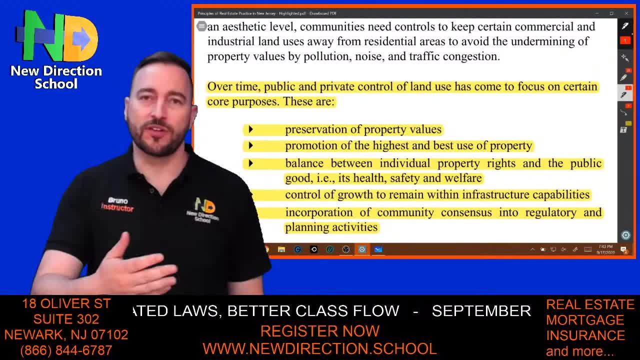 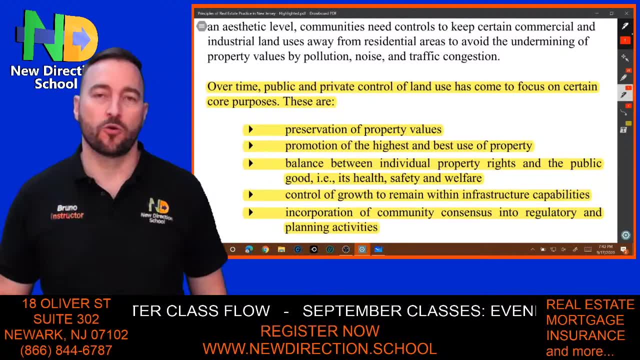 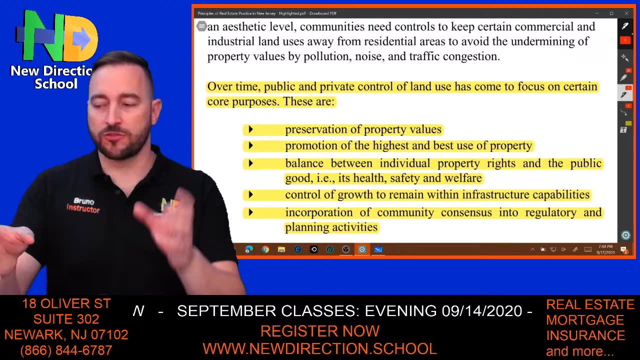 So we have to understand this. Over time, public and private control of land use has become has come to focus on certain core purposes: preservation of property values. What do you think the values are going to be on the straw house, the wood house and then the brick house? 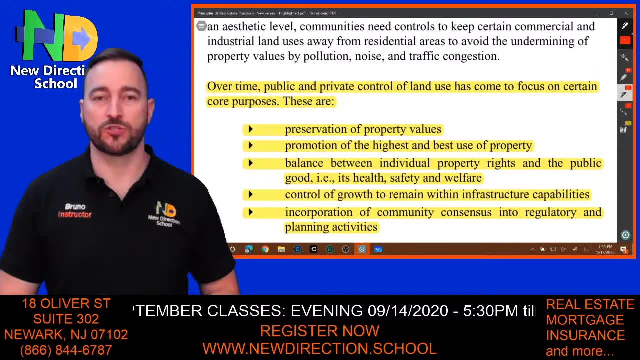 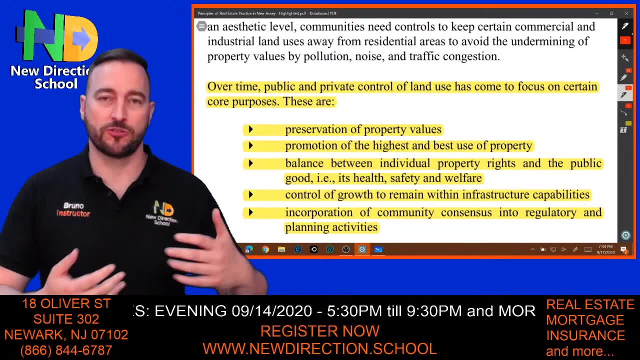 Which one is going to be the most expensive? Which one is going to be the least expensive? So we just talked about foundation. the one with the sturdiest foundation most likely is going to last longer and most likely is going to be worth more right. 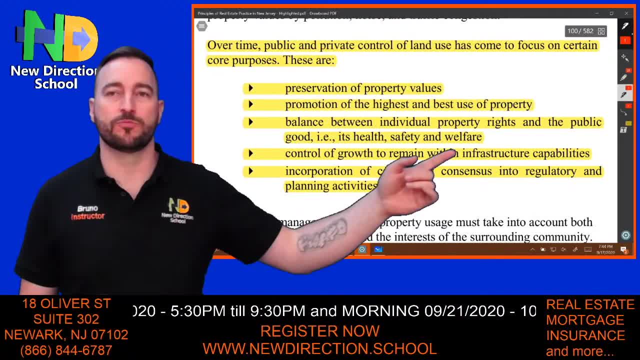 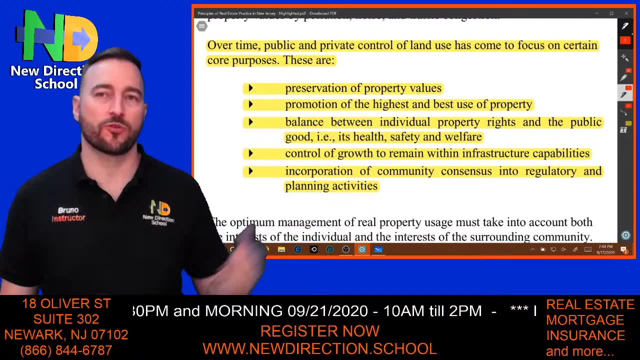 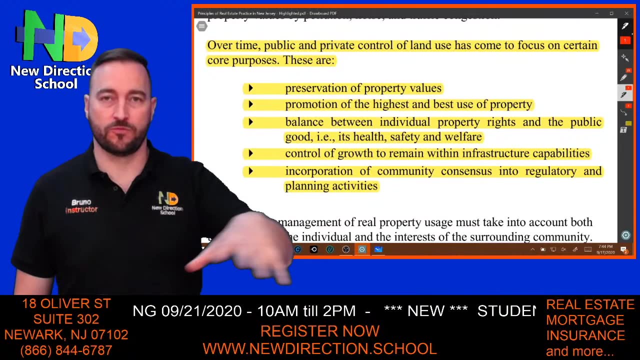 Promotion of the highest and best use of land, Balance between individual property rights And, again, public good, Health, safety or welfare, Control of growth to remain within infrastructure capabilities, which is what the town believes that's best for the growth of the community. 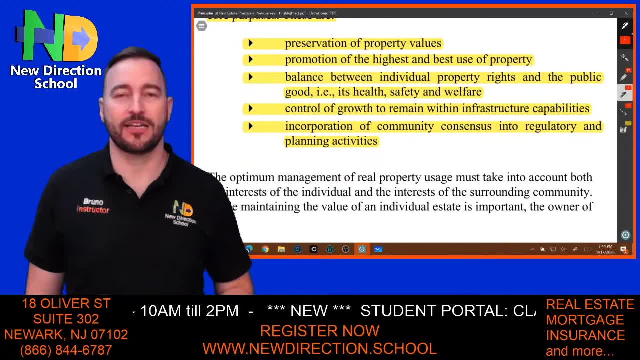 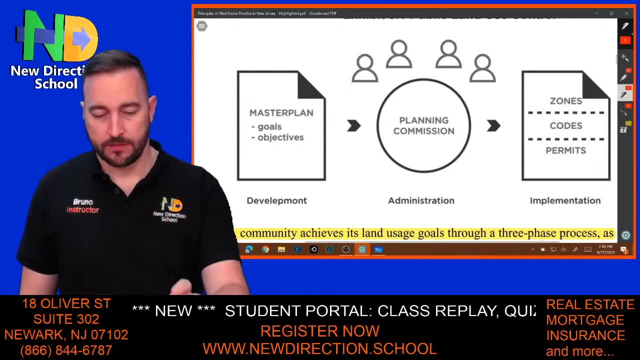 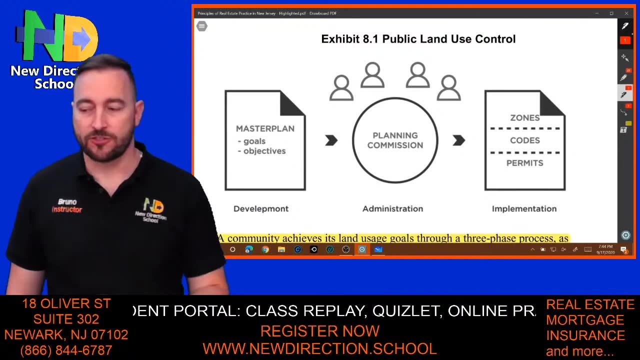 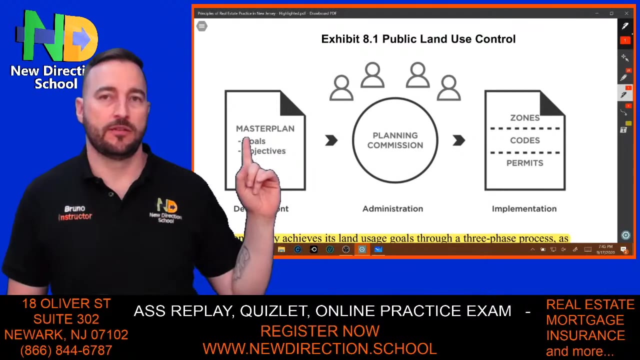 And incorporation of that growth into the community consensus, into regulatory and planning activities. okay, So There is something. There is something that everybody should get And that's called a master plan. Why is it so important For you realtors? for you realtors and even if you're an investor, this is the main thing. 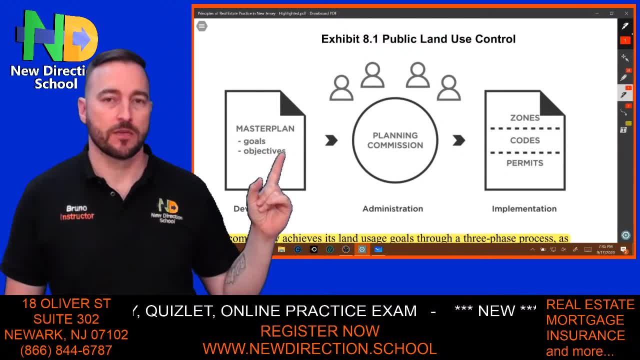 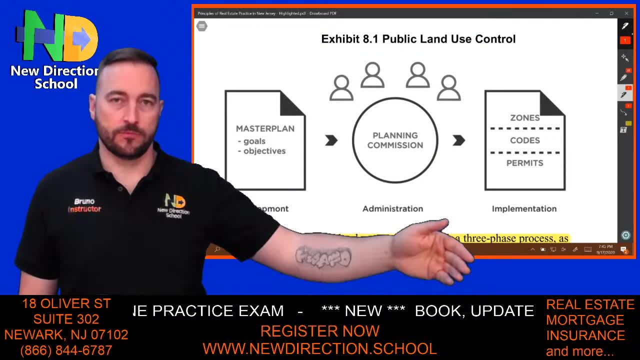 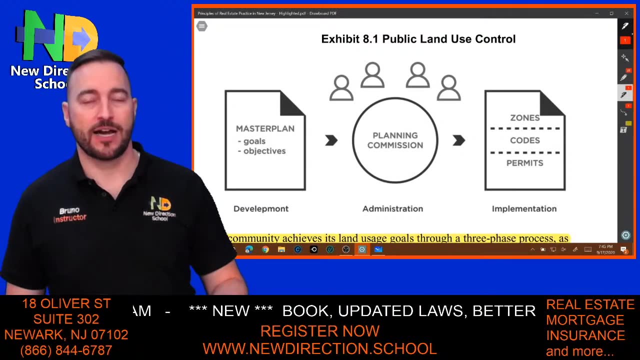 This is like predicting the future Because, just like I said a few minutes ago, we plan to reach a goal right, And I don't know if everybody uses it or not, But every day I go home right, Every day I come to work. 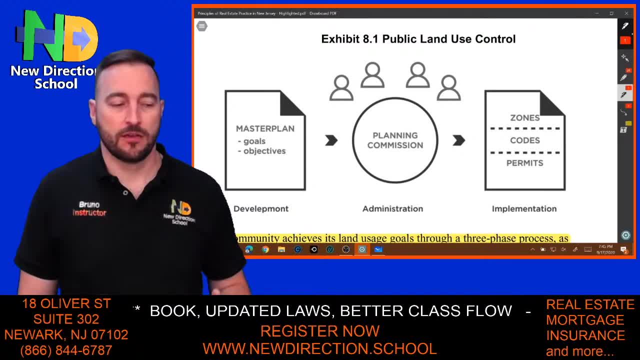 And I use a little something called GPS, But I use it every day. The route is still the same. I mean the destination is still the same, It's home or work or wherever I need to go right, But the most common ones is home and work. 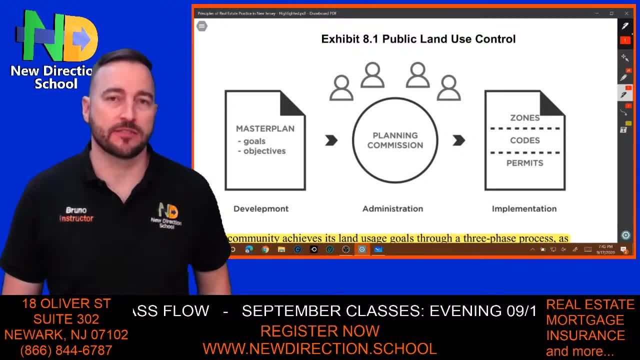 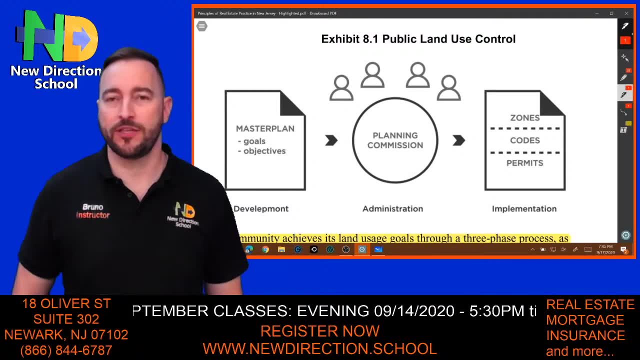 Destination is the same, Why do I still need the GPS? Why do I use it every day? A lot of you are probably thinking that's crazy. It's again same destination. Why do I use it? Let me know. 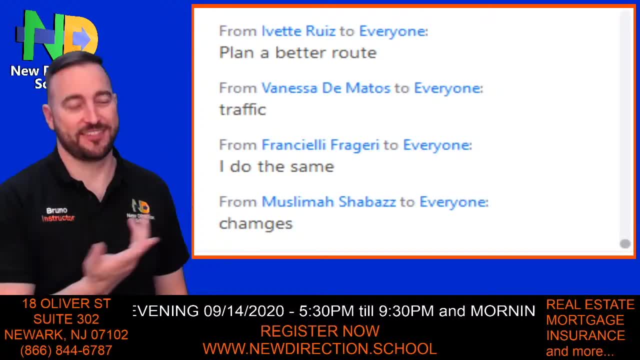 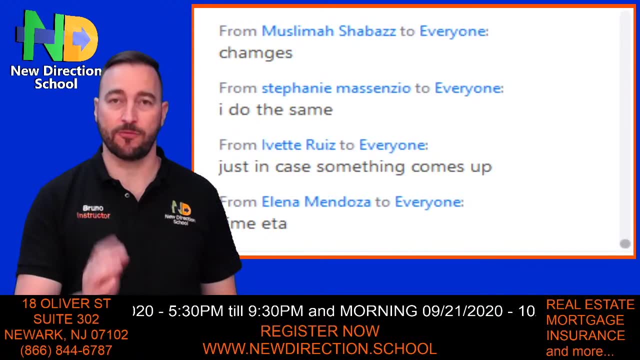 To plan for a better route for traffic. right, You do the same. Great Changes? Yeah, because, guys, even though we have the same goal every day, which is to reach home, as an example, right, Stephanie does the same. 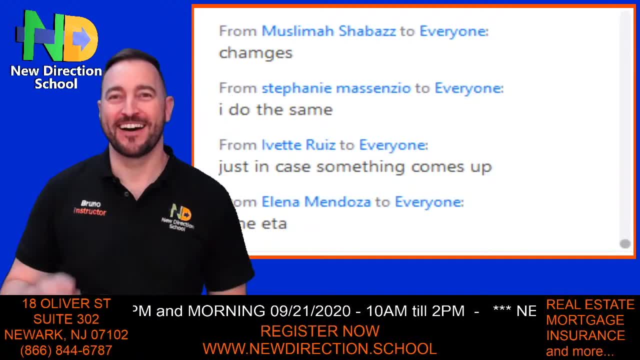 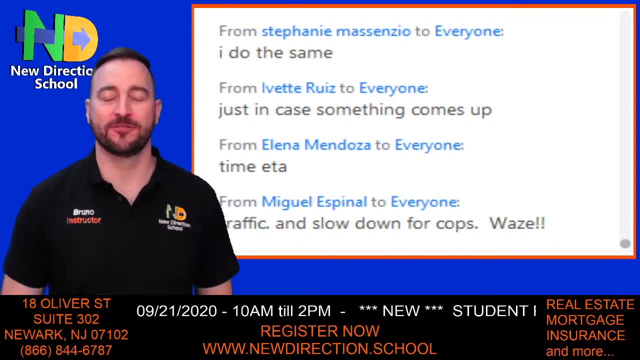 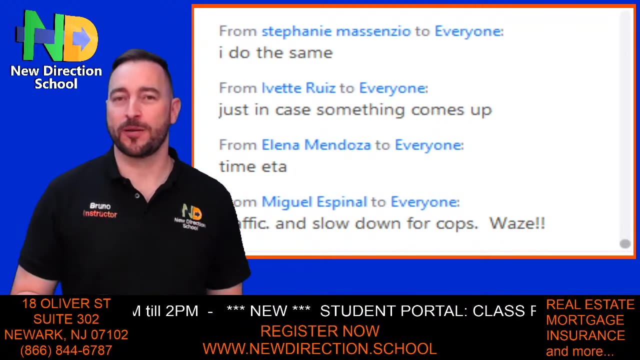 Cool, I thought you were going to say whatever friend said, Because she says I do the same. But yeah, just in case something comes up. Time, ETA Traffic Slow down for cops, Yep Ways. Anyway, Laura, just said planning your trip, right? 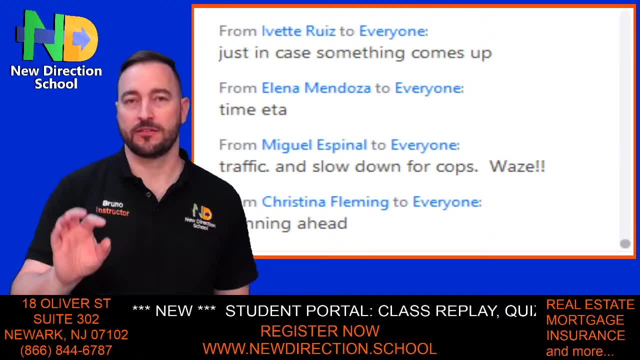 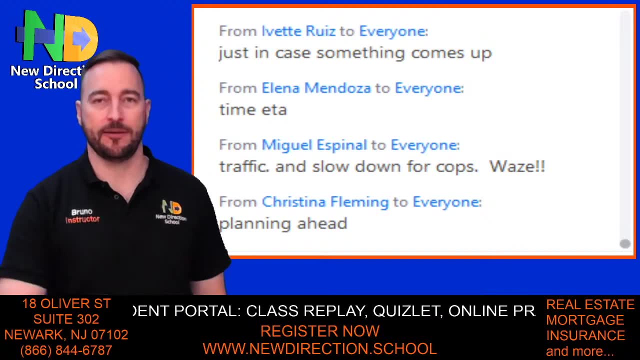 Exactly. Do you think that buildings show up from one day to the other, Meaning the guy that decided: oh, I'm going to put here a stadium? Let's talk about Barclays Stadium. Let's talk about Red Bull's stadium close by, or even the Prudential Arena. 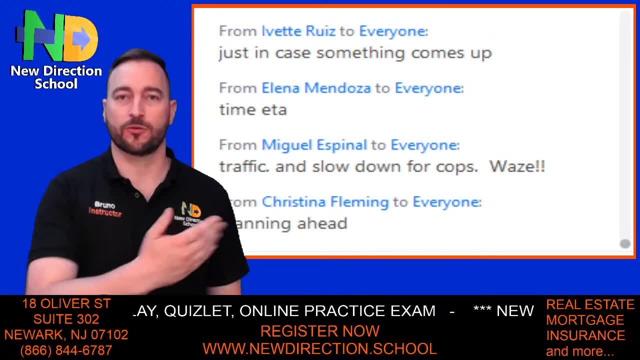 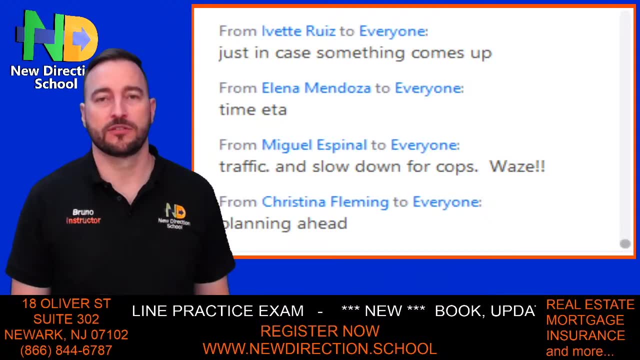 Do you think those were planned from one day to the other? I think this is a great place to put this here. No, A lot of these were planned with years and years, like 20 years sometimes. This is the ideal place for me to build this right. 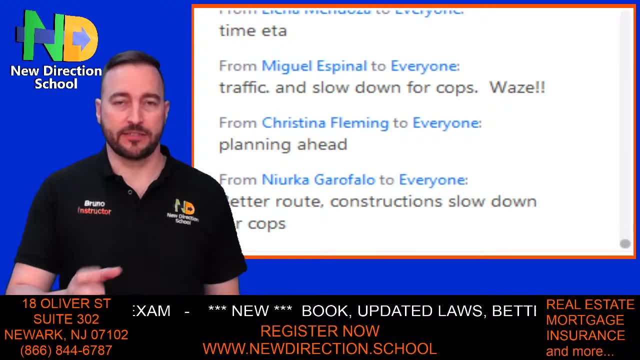 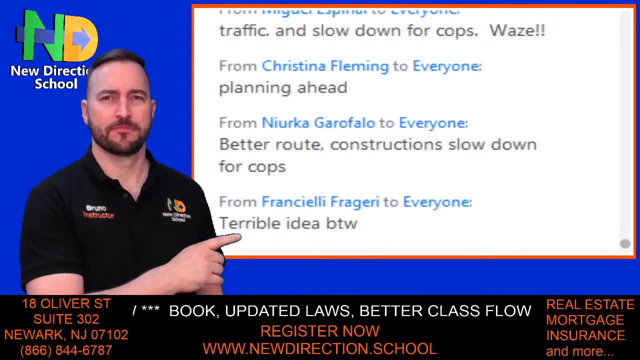 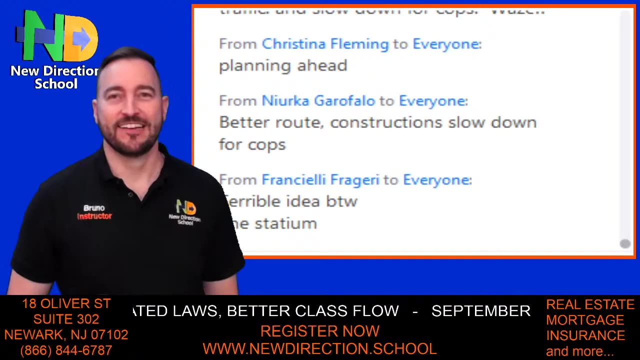 So I'm going to use the GPS to reach the destination. That GPS in the sense of the terrible ideas, because of the cops or the stadiums, The stadiums, Okay, Kind of, because it also brings jobs, So kind of. It brings revenue and reduces your taxes, if there's something else compensating. 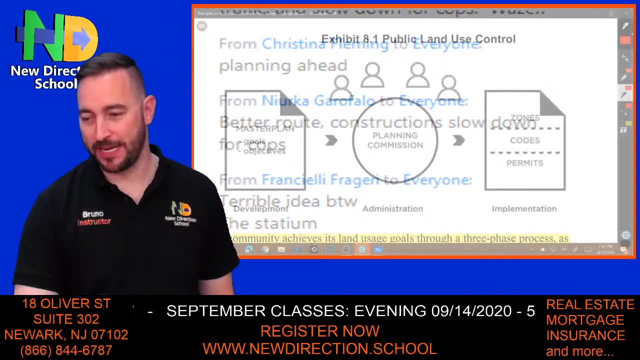 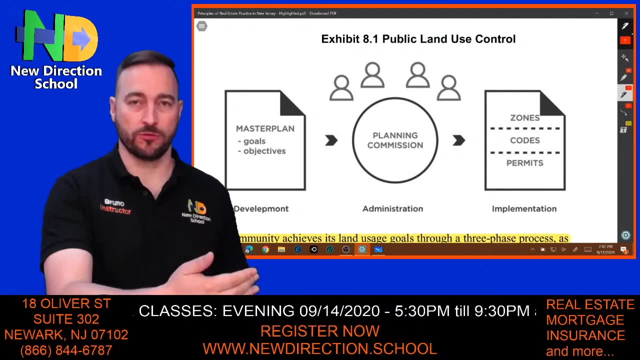 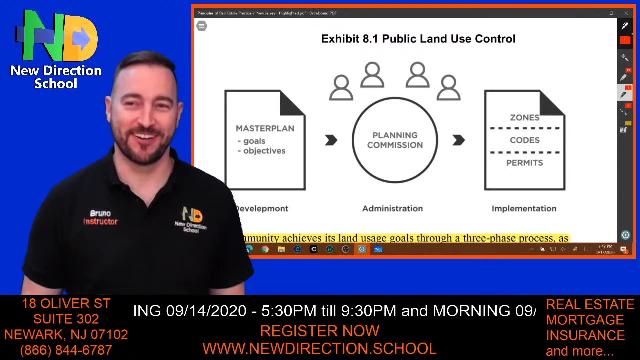 But anyway, let's go back here. So the master plan is like your GPS for knowing what is the town's goals, What does the town plan for the future And is it possible, Let's go. Red Bull says: Robin, Let's go. 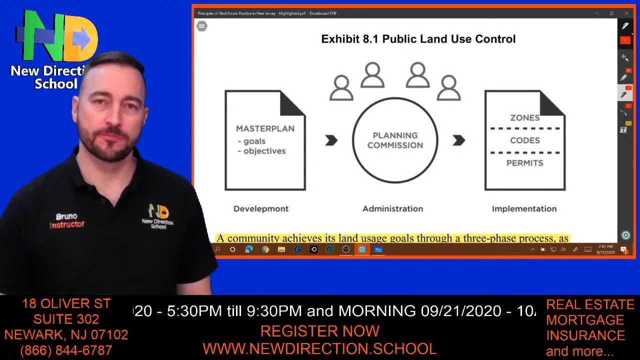 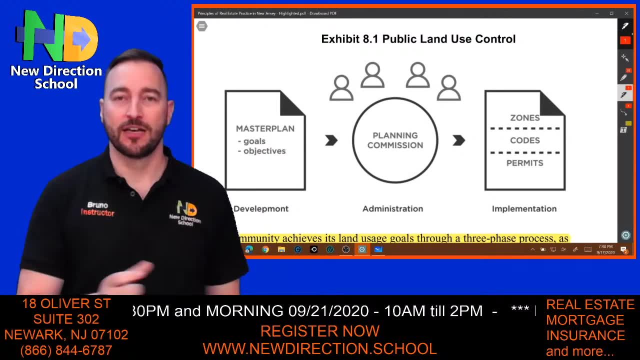 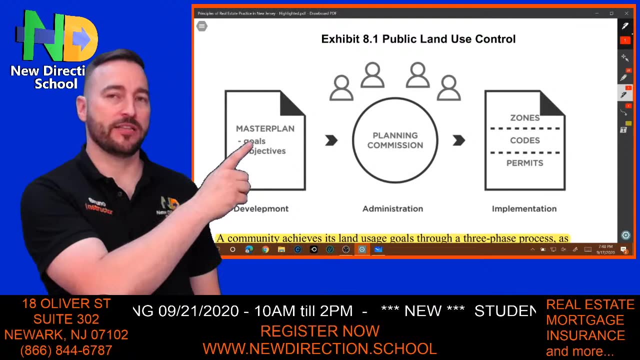 Is it possible that the plans change? Yeah, That's why you're going to alter the master plan accordingly. Just like your GPS adjusts because of traffic, adjusts because of accidents, adjusts because of whatever right, The master plan is also adjusted according to new buildings that are put there. 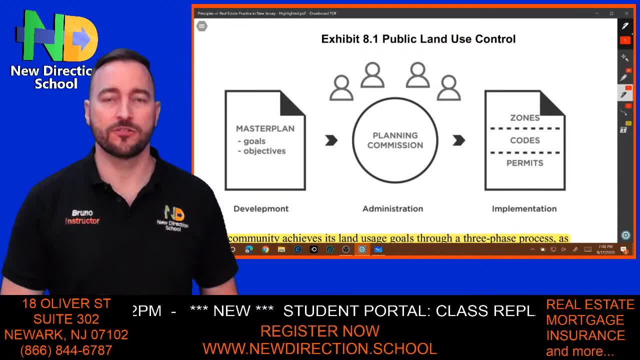 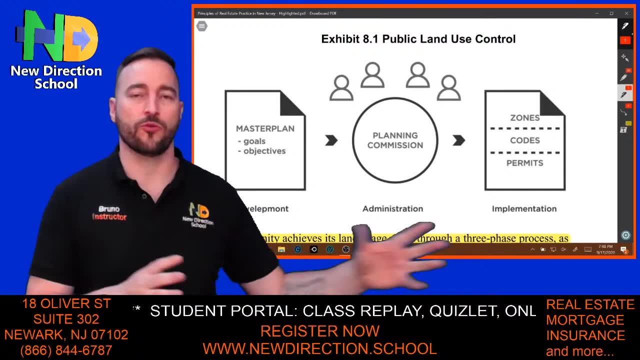 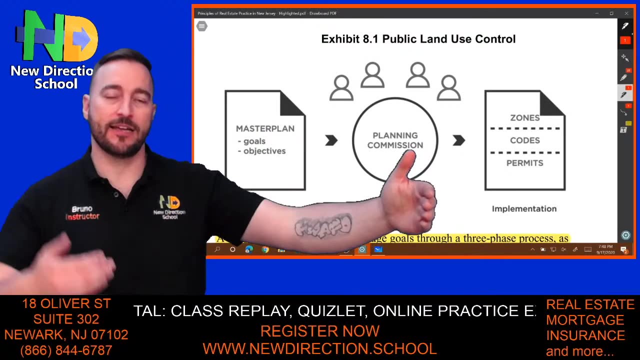 according to new roads that are placed there, according to new desires of the economy, According to the economic and aesthetic concerns that the town has. What is the town's growth? Where are we heading Right? So the master plan has that goal and then it allows you to plan for that goal. 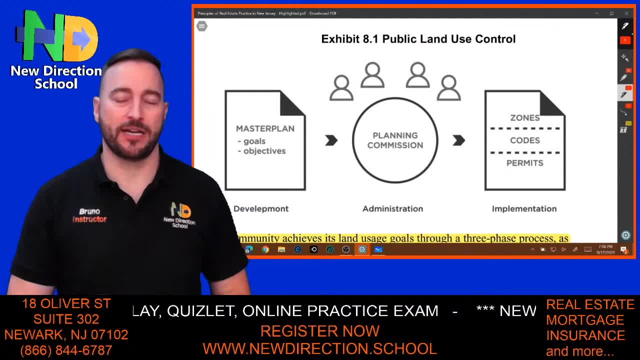 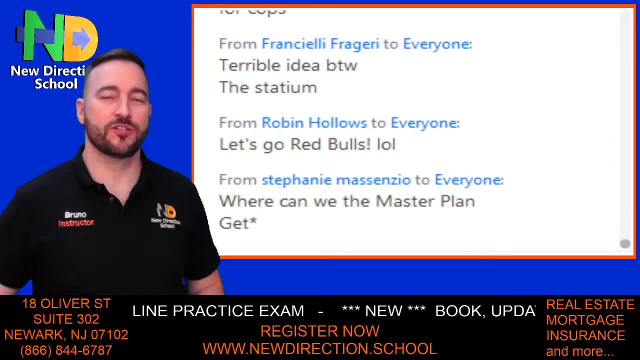 Okay, So that goes through the planning commission and then implemented by zone codes and permits. Great question: Where do you get the crystal ball that will tell you the future and make you a whole lot of money? That's your question, right? Very simple. 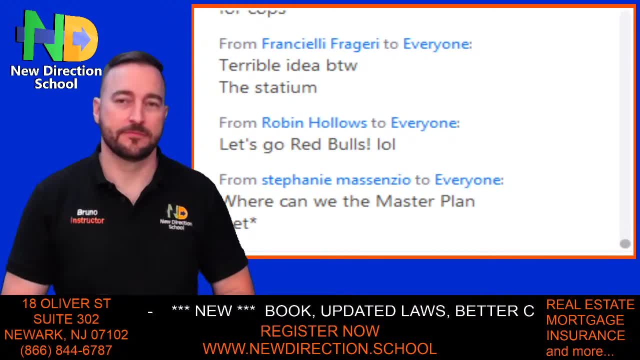 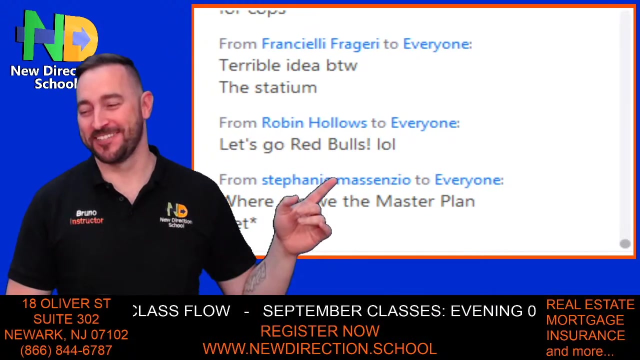 Ready? Write this down. WWW Ready. Let me make sure everybody's ready. wwwgooglecom. Don't give me this tank face. I'm sorry. I always mess with everybody. Here's what you're going to do. Here's what you're going to do. 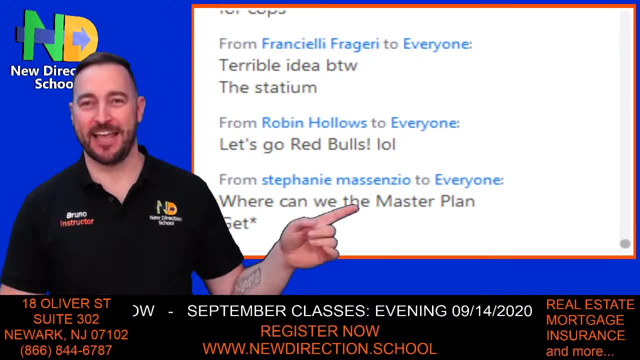 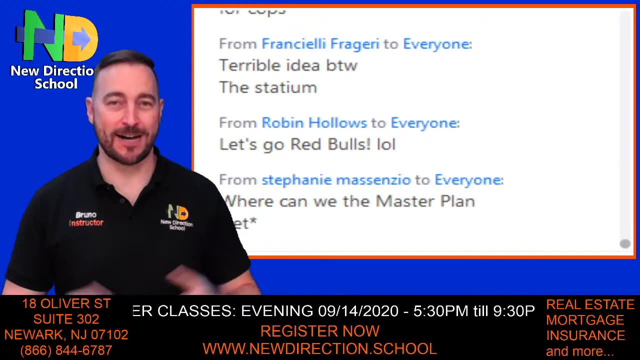 You're going to put your towns Name, whatever it is, So let's say Newark- and then master plan in Google, Right, You're going to put Linden master plan or comprehensive master plan or general plan. But what I do recommend is that you go to City Hall and request it there directly. 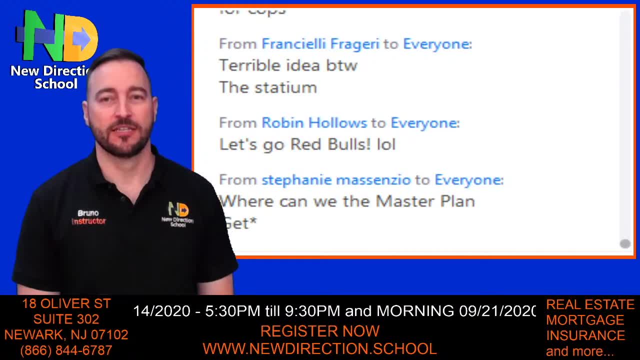 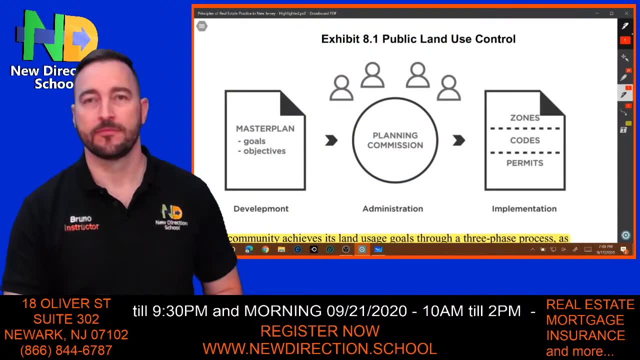 Most likely, they're going to tell you to get it online, But you should start getting familiar because, the same way- this is important- Online they don't talk to you. They don't talk to you. Look at this, This is going to be a paper online. 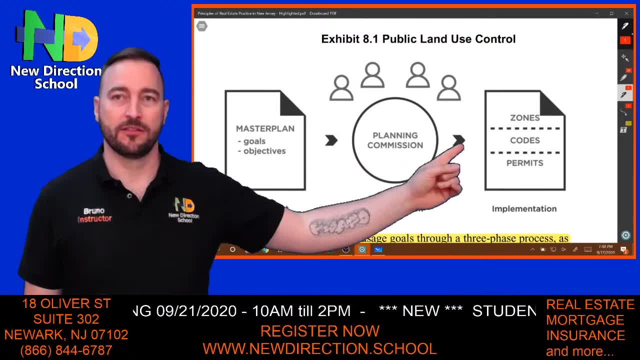 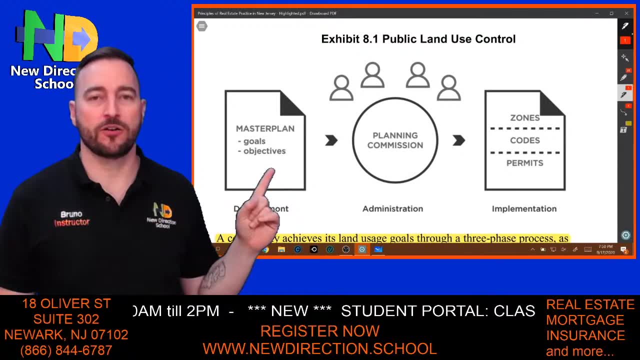 These are people online until you meet them. These are rules online until you get to know them. So what I recommend? even if you get it online, try to go to City Hall. Try to get to meet the players, not just the planning commission, but everybody else there. 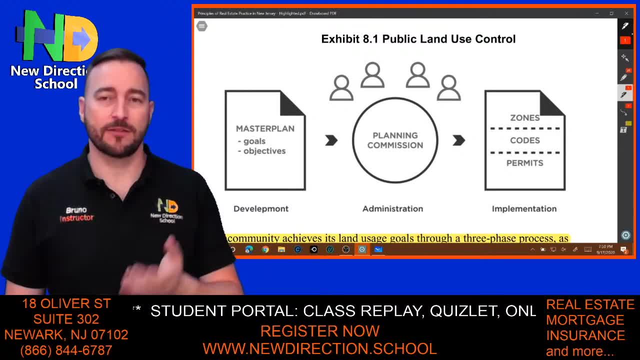 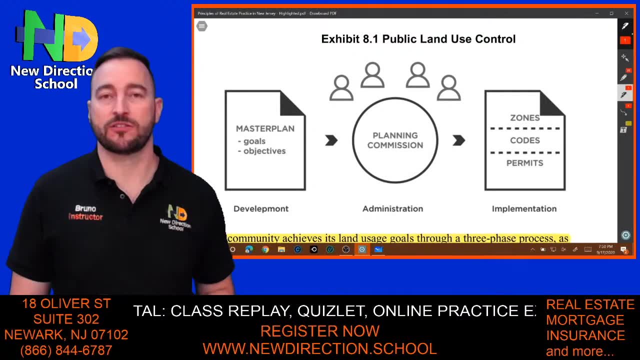 Because, especially as a realtor, sometimes we go there on behalf of our clients to apply for CEOs Right To find out what the taxes are, the real taxes are for a property, To find out what can be done with a property, what permits are needed. 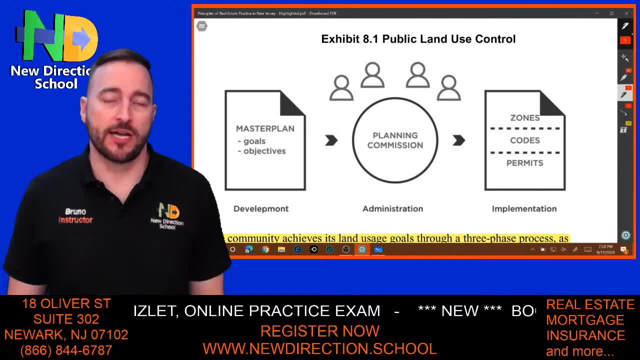 Sometimes we handle that for our clients or investors right, Or if you're an investor yourself. So get to know the players Very, very important. Build a relationship with the players Very, very important. Treat them very nicely, because you need them. 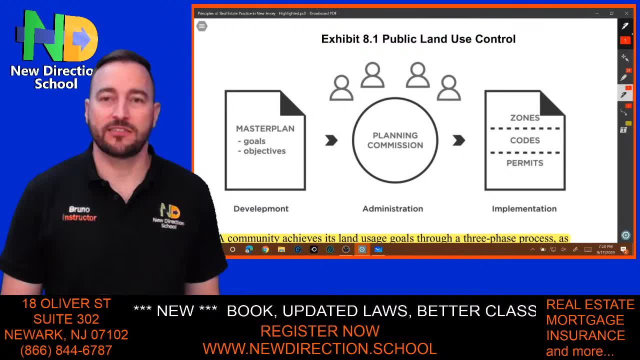 I see some people when I go there. I see some people giving attitude Like I need this, I need this And you should be doing your job. No, it's not going to help. It's not going to help to have that attitude. 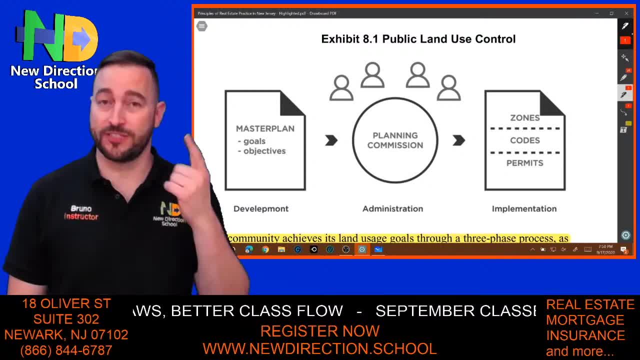 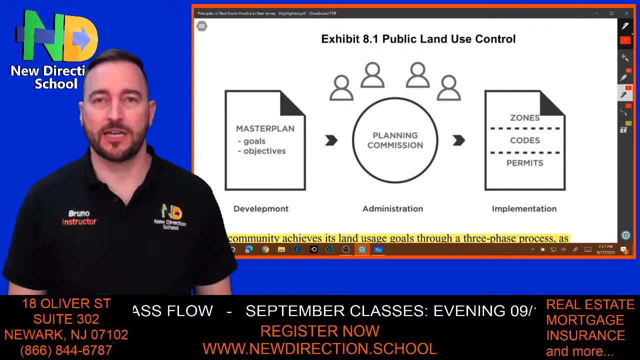 We know they need to do their job, But if the person before you was giving that attitude, how do you think it's going to happen to you? For you, I mean Right. So go there, Be nice, Hey, listen. 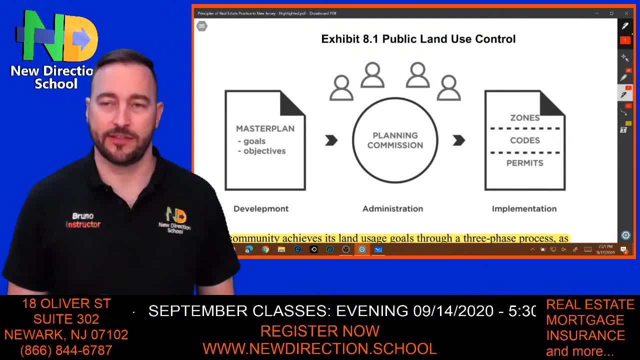 I'm going to be a brand new realtor in the area. This is the script I try to tell everybody. I'm about to be a brand new realtor in the area, or I am, And I'd like to know what's the process for getting this. 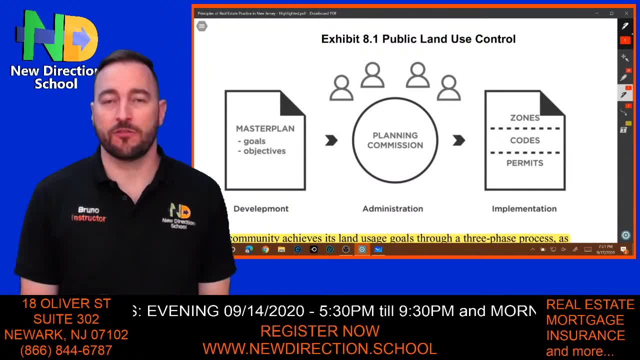 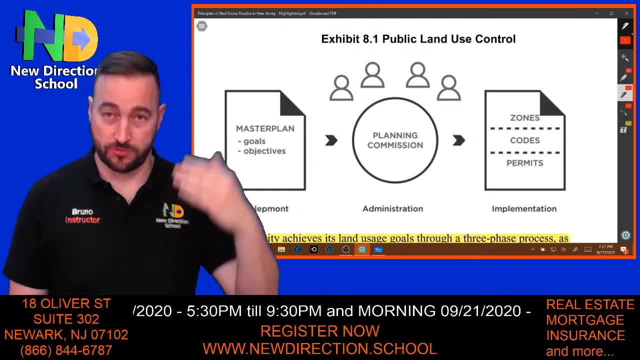 And that, And make sure that next time that I come here I am prepared So I make your life easier. The moment you guys say I'm trying to get info to make your life easier for them, How do you think they're going to treat you? 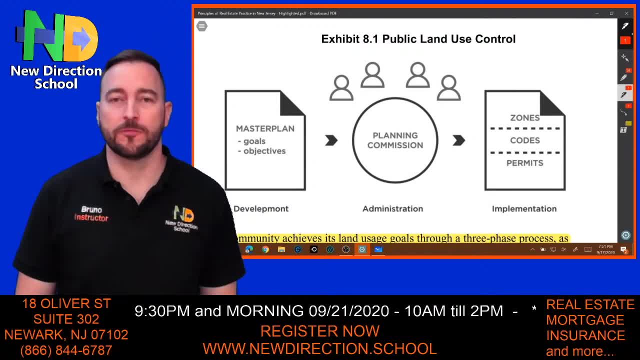 I just did that at the water department not too long ago. One of my agents was having trouble getting information. I went there Myself, Okay, One of my agents, actually Mario. He asked me: Bruno, do you know anybody there? 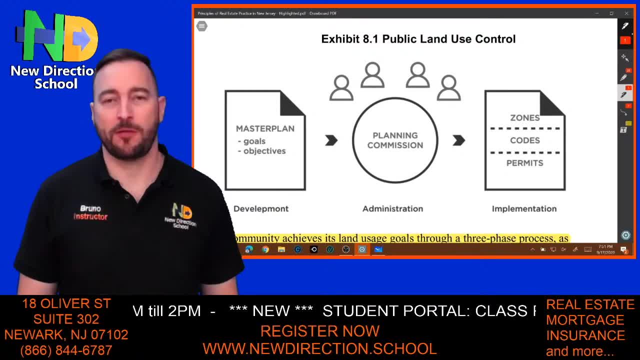 I'm like at the water department. I don't, But I'll pass by because it's two blocks away. So I went there And the information that he could not get: I got there in less than two minutes. I had the information and much more. 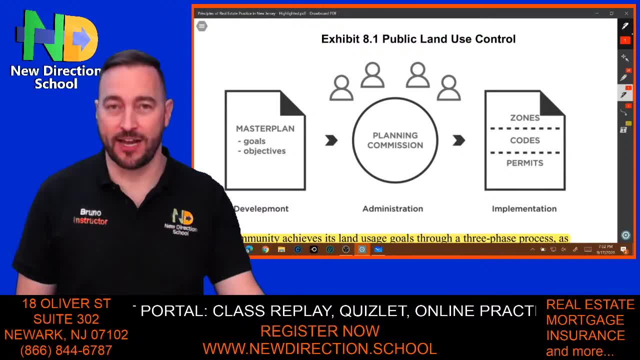 Like this person, gave me way more information than what I asked for about the property, Which was cool. Why? Because some people in that department recognized me, including that person, Even though I never dealt with her directly. Recognized me. I tried not to give trouble. 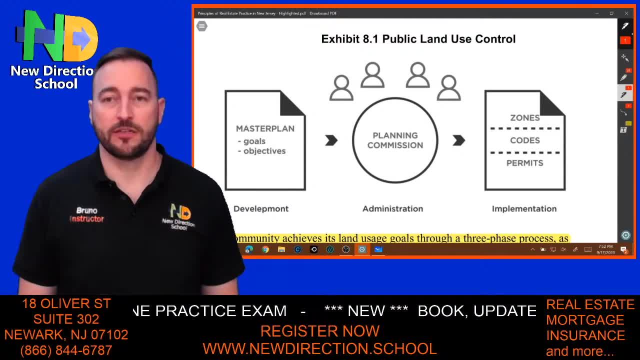 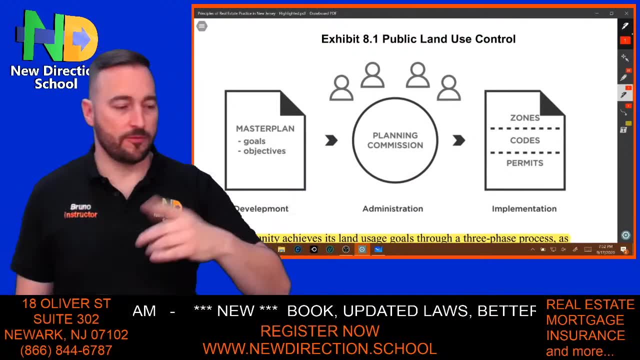 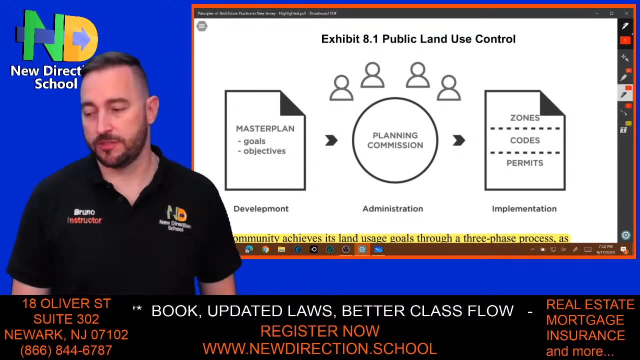 I'm very respectful of everybody and their job Right, And understand. You need them, You need them, Okay. Okay, So Milly is here. She helped me out with a property a few years back, Right, She's now one of our students. 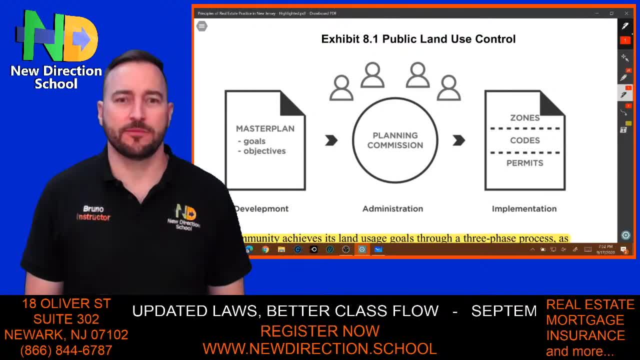 And Milly, did I ever treat you badly when you came to the property? No Right, You better say no because you need the certificate to pass, Just saying All right. So never treated her badly. I think I was very respectful and I got her number the same day and she was very nice to me. 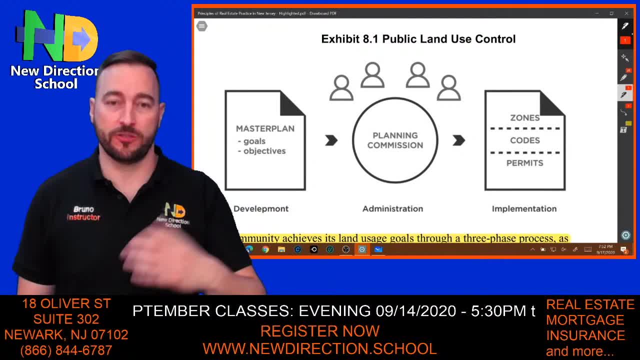 And I took care of what I needed to take care of when she told me she was inspecting my property And she told me: hey, Bruno, you need this, you need that, whatever, Once you have it, let me know and I'll come back. 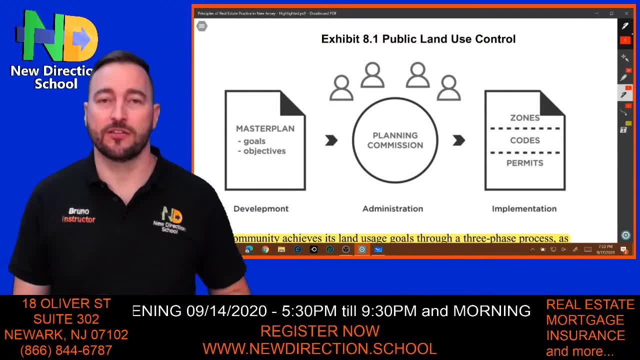 Right. And the same day I resolved the problem, I sent her a message. Guess what, Instead of waiting another week or two, a couple days later she was there. All right. She looked at it, said: okay, you're good. 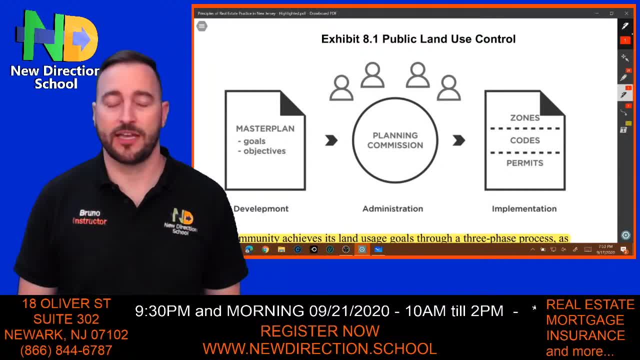 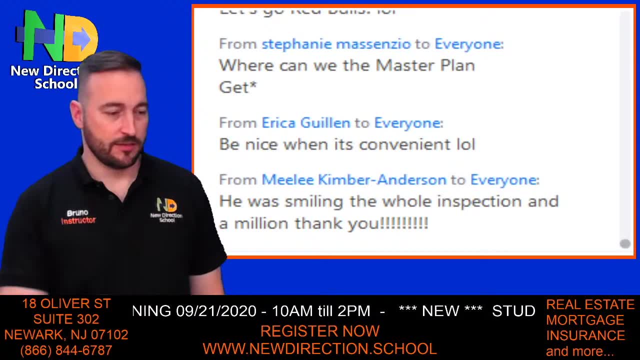 And I asked her: when can I get the report Next day? it was done, All right, So it's a matter of: yeah, right here. Be nice when it's convenient. No, Be nice all the time. Be nice all the time. 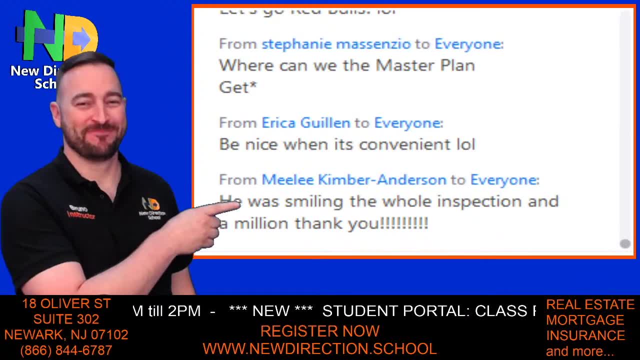 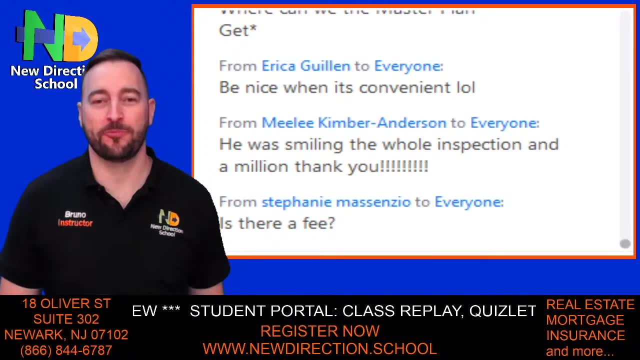 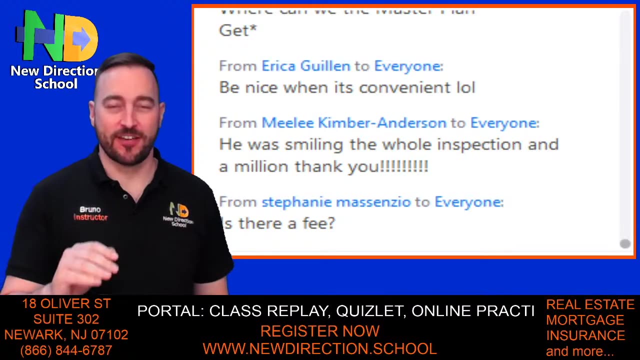 Okay, Yep, This was me. I mean, this is still me, And a million thank yous, Absolutely, Because I appreciate everybody in it. Is there a fee? What To the inspector? Never give a blank envelope, Never. 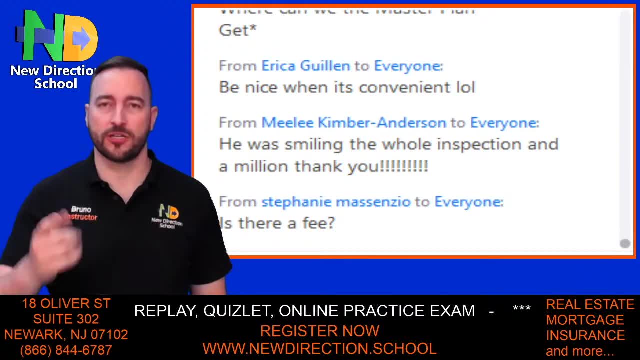 Yeah, There's a fee for inspections, But that's for the master plan. If you get it online, it's free. If you go there, some municipalities offer for free, Some charge you like I don't know, like five bucks, ten bucks. 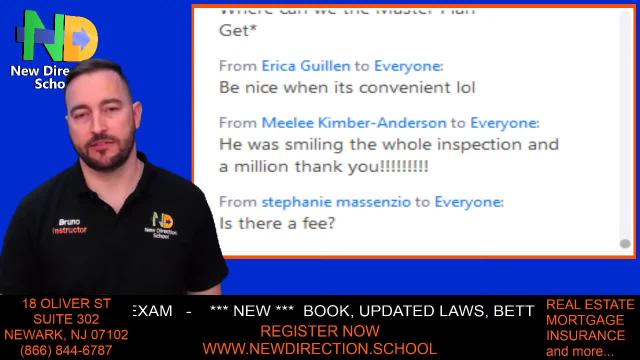 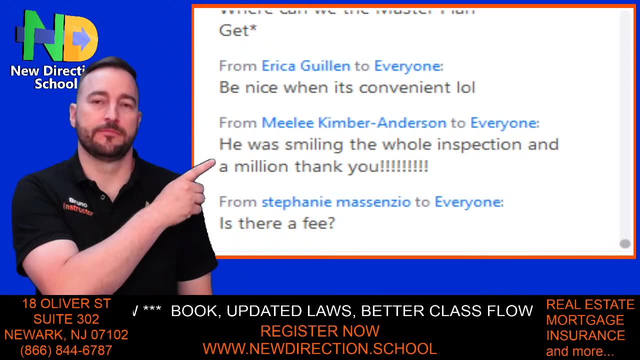 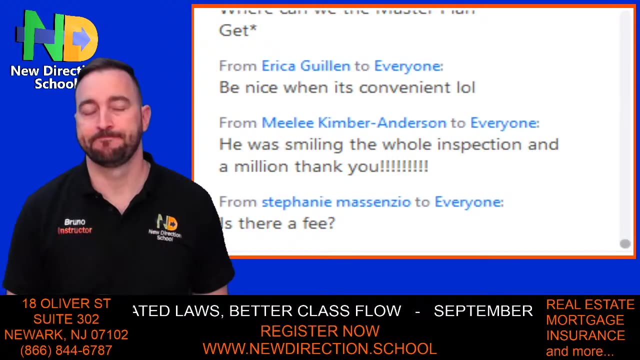 It's really not much, But definitely get it. You can get it online. like I said, I still recommend build a relationship. Okay, Still recommend build a relationship. This is the most important thing, because these are the people you're going to work with. 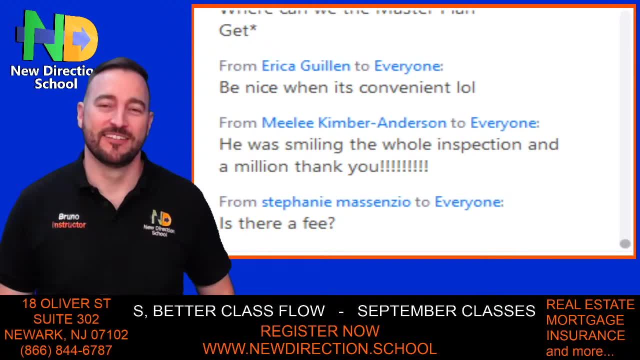 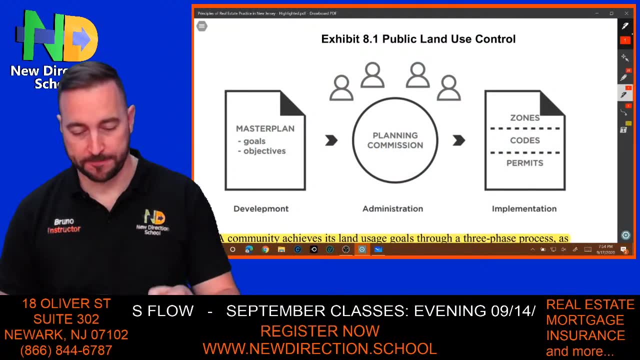 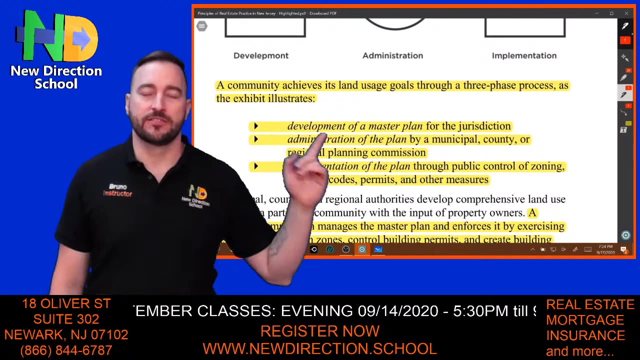 And eventually look they come back to do some type of business with you, All right. So master plan Very important And this is a three-phase process to get into the master plan Right. It's the development of master plan, administration of the plan and then implementation. 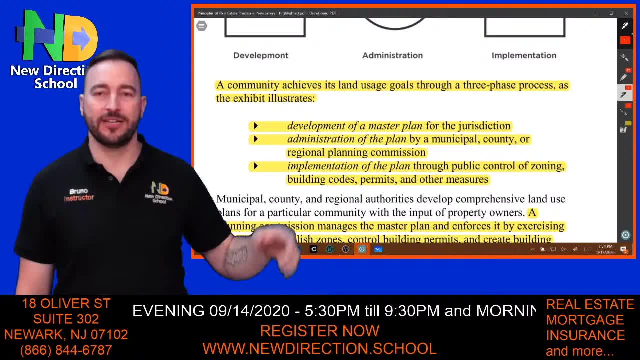 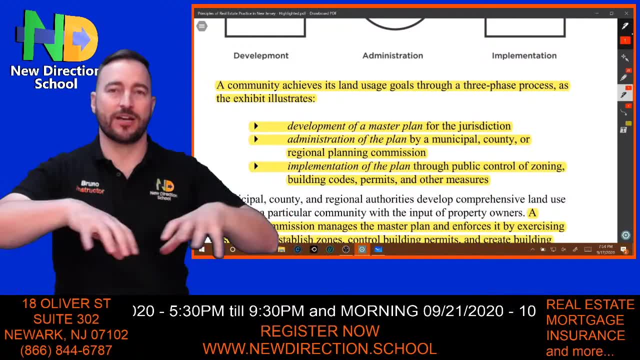 What is implementation? It's determining zoning. Zoning is okay, this is residential, This is commercial. Let's not mix Okay. So we try to keep it separate. This right here is industrial. Definitely don't put it next to residential. 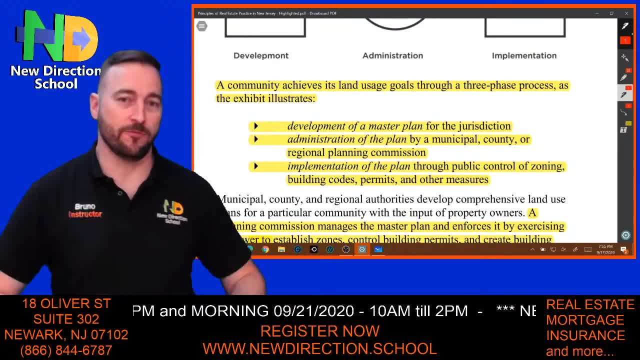 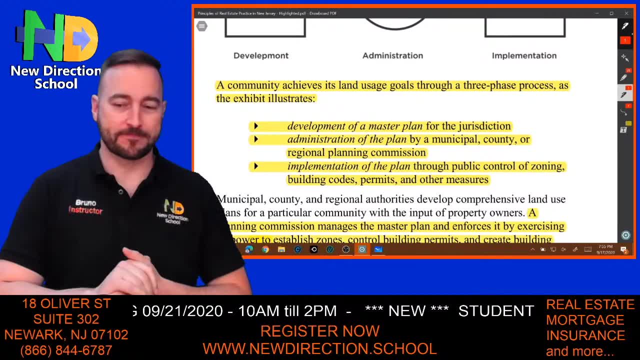 Unless you're in Newark. If you're in Newark, we mix everything. We have a factory, And then we have a single family or two family right next to it. Right, That's Newark. Newark is special. And then you have- we have recreational and institutional. 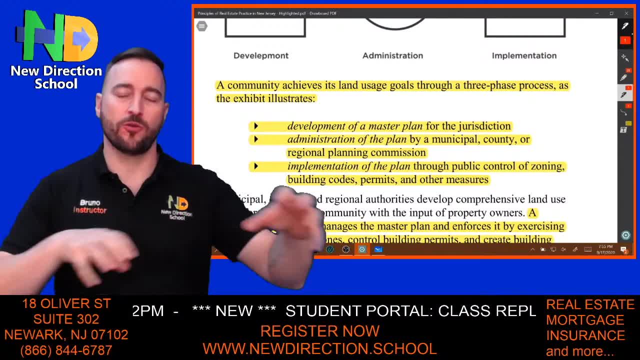 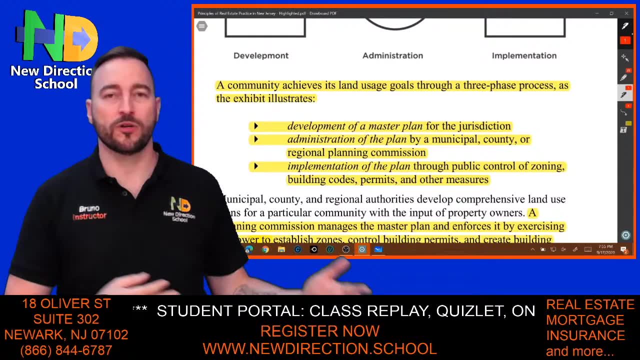 Schools, parks and so on. These are different zonings And the town grows. When I said Newark is special, it's because until not too long ago Newark was industrial, Mainly industrial- Right. So there's a lot of industrial zoning that's being converted to residential. Or commercial. So that's why you still find factories near or right next to residential homes. All right, So that plan was changing according to the town's growth. Very important, Okay, Again right here. Public land use planning incorporates long term. 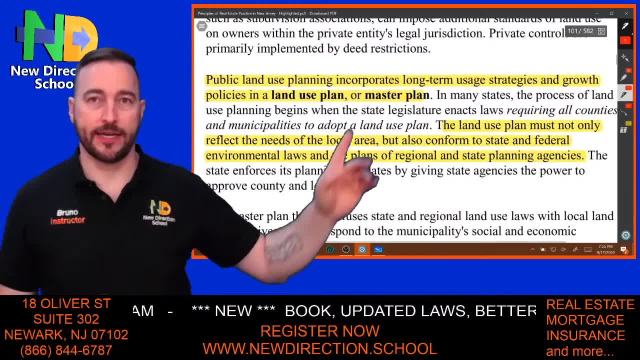 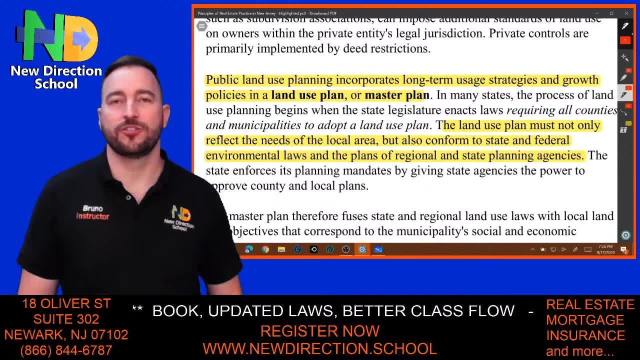 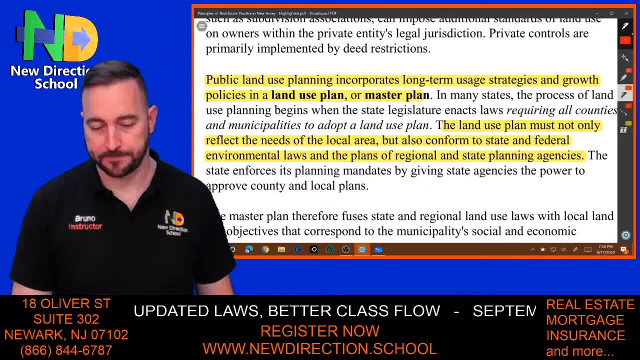 And then we have residential, And then we have residential, And then we have residential. So it CombatEL right. And then you look at the budget united within the community, And then you look at the budget united within the community. Okay, 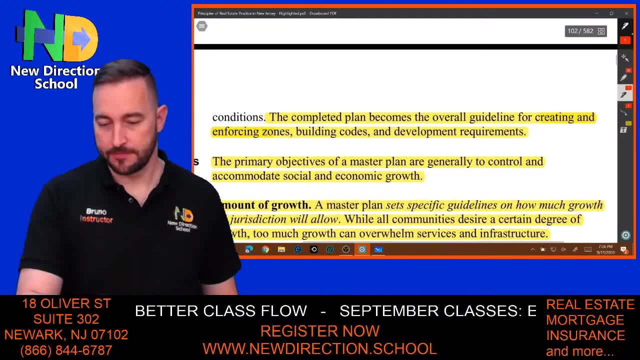 So there's lots of grants that are gonna get higher. It's aware of our need And it's conscious of our need. It's qualified toagle. It's qualified toagle And the deferred Battlig mess shows us that we have time to build those. 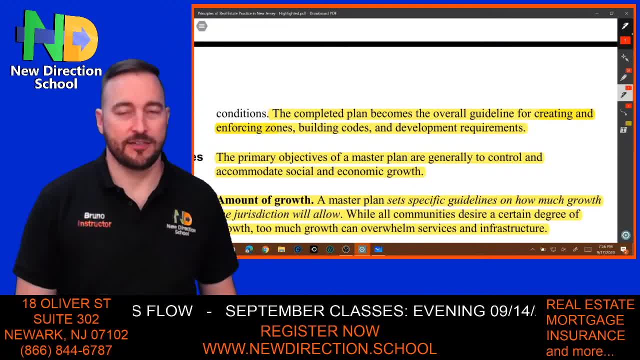 What I just showed you is data, as well as an input that can be be parties to the, or rather rather its four and logics. All right, So again, this is a problem. What I wanted to focus on одна using different business concepts. 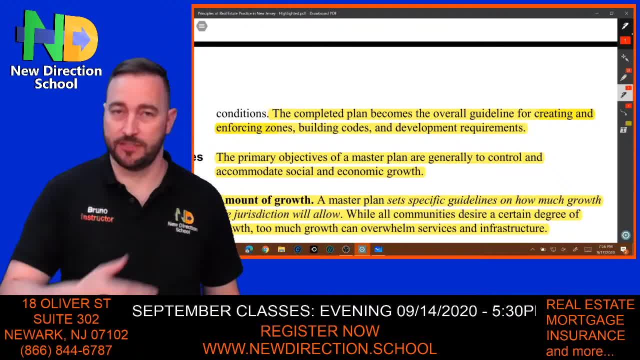 I have other people from City Hall in different various departments of City Hall that took my course or are taking my course. One of them is the senior aides to the mayor here in Newark right, So he's taking the course as well, or registered it's going to take the course as well. 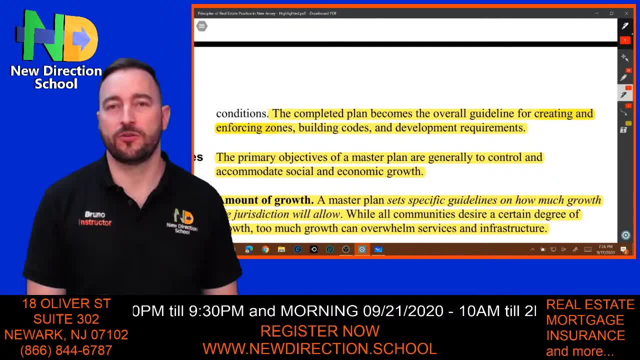 You know what I'm saying. So build that relationship. You never know when you're going to need them. It's very important. And Erica says: Stephanie, Stephanie M love your doggy. Yep, I thought Erica was smiling at me like, oh, Bruno is so cute. 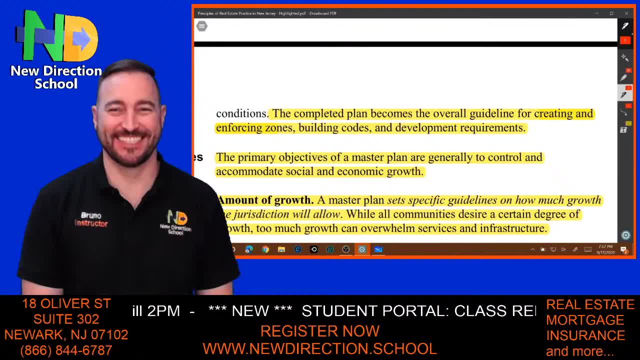 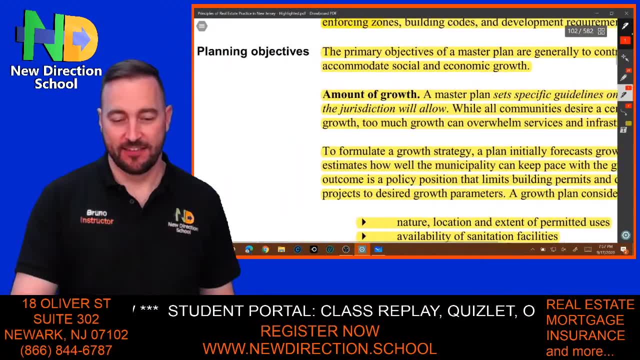 No, it's the dog. that's cute. All right, next, Planning objectives. Guys, I already addressed most of this When we were talking about planning objectives. I already addressed most of this When we were talking about planning objectives. I already addressed most of this. 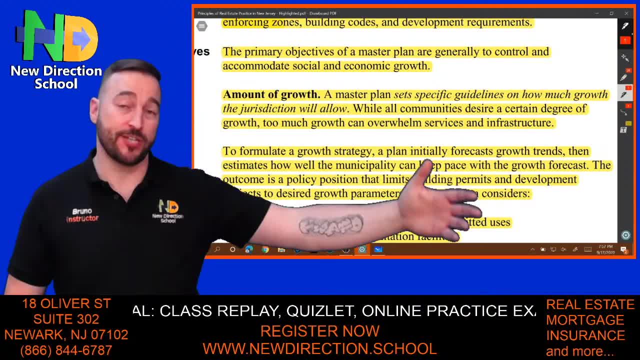 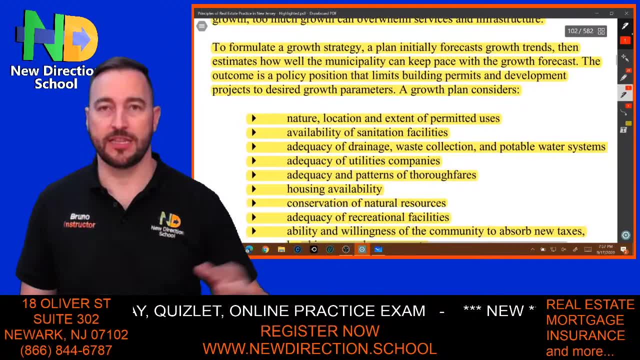 What we plan is because we have a plan to go, a goal and objective right, And these objectives will have to be implemented into the plan. So a growth plan considers the nature and location, the extent of permitted uses, availability of sanitation facilities, adequacy of drainage, waste collection, potable water systems, utility companies, like a bunch of stuff that I think you guys understand. 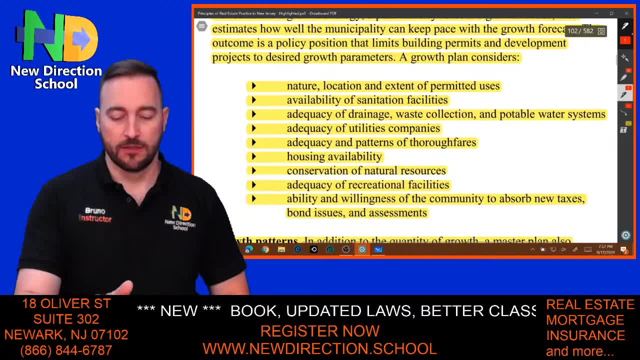 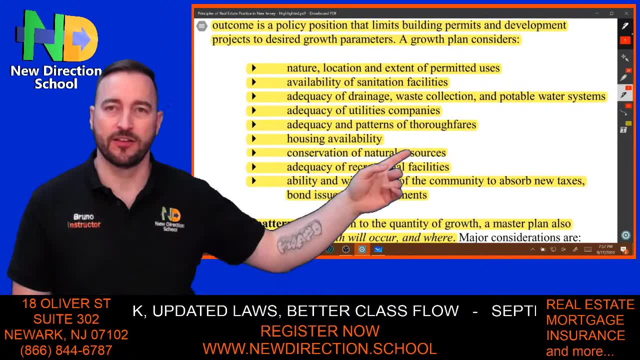 It's common sense. I highlighted just to be here, But you probably, I'm probably thinking also: why do I need to know this? That's, the town has nothing to do with me whether they have sewer mains or they have water mains or all this housing availability. 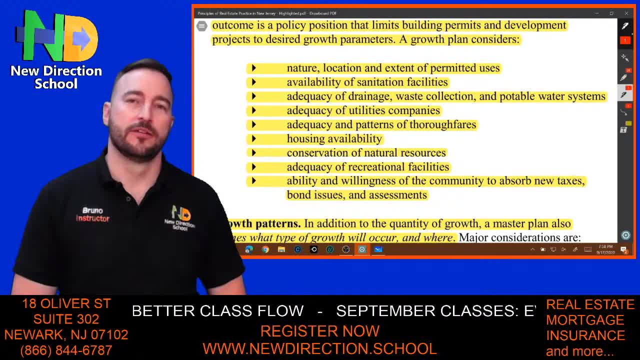 What do I care about that right? Very important. Knowing your markets and the changes to the market is very important. Like I said, Newark was industrial Jersey City. Look at Jersey City, Jersey City properties 10 years ago were worth like $200,000. 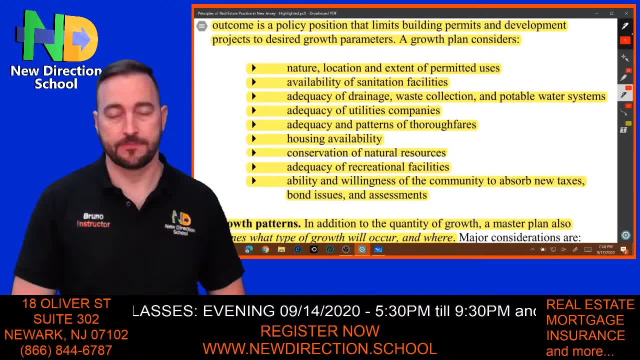 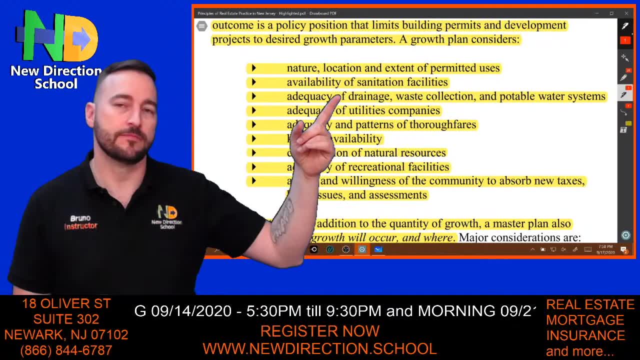 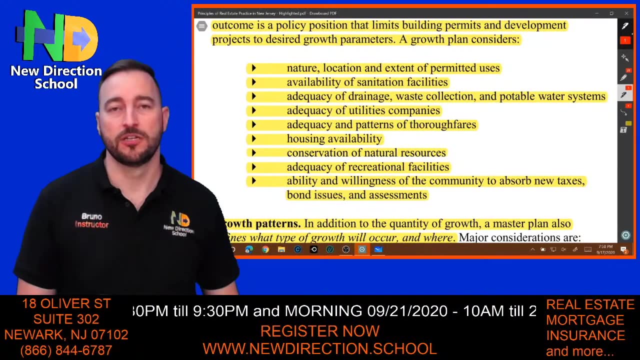 They're worth a million dollars in 10, 15 years. Knowing the master plan, knowing the changes, what could happen in certain areas, will give you an edge compared to everybody else, Will give you the advantage to make money. Very, very important that you know this. 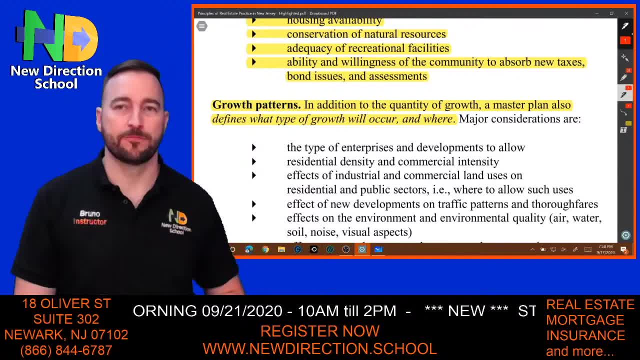 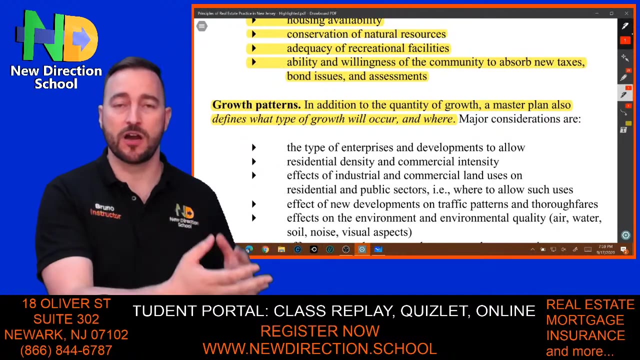 Growth patterns, The types of enterprise and developments that will be allowed in certain areas. Residential density: If you guys notice in certain towns or certain areas Within the town, right, there's a more dense population than in other areas. You need to know these things because the more properties we have, right, the least expensive the property is. but the higher crime, the more difficult to put some certain types of projects into that particular neighborhood. 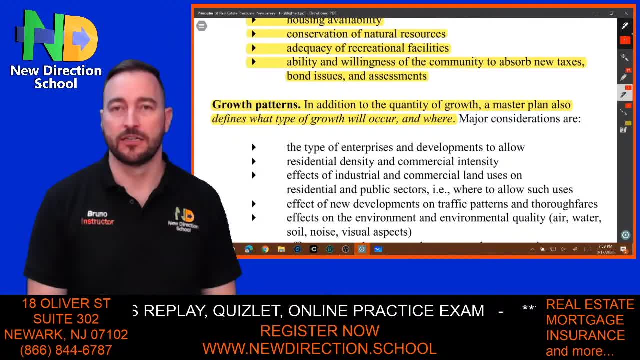 You go to other areas, you might be able to do different types of planning right. So I have a client that's looking for land only As an example, Land only to build- probably the first here in the area, the first mechanic shop for electrical vehicles. okay, 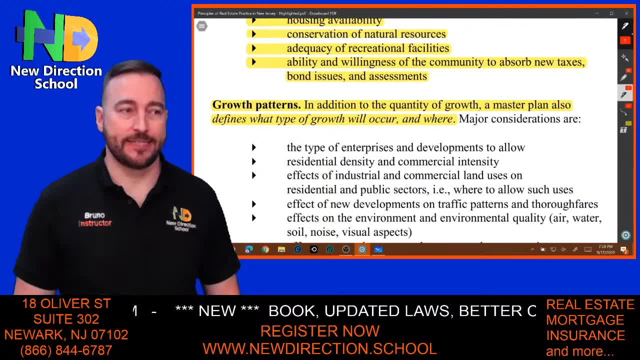 So that's what he's looking for. Can I just get land anywhere? No, it has to be in the third type of area that will allow, So most likely commercial. So I cannot put it in residential right But depending on the commercial intensity right it might not be the right place for him as well. 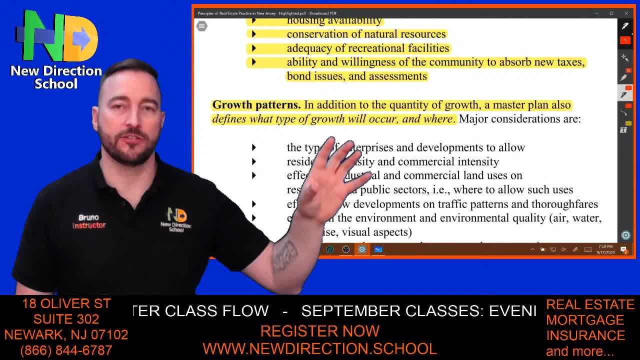 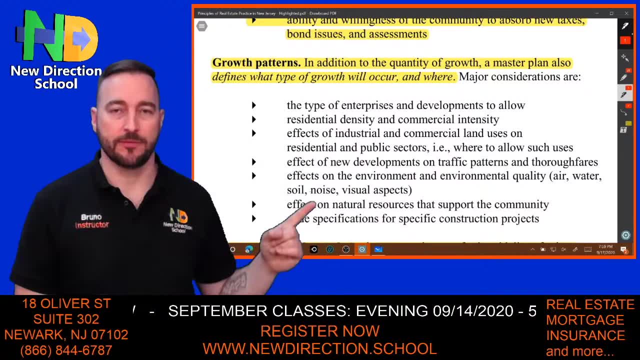 So we need to study these things, Understand the local market that you're in. I don't need to know the whole New Jersey, but I need to be the pro in my area. That's where I'm looking for properties for him in my area, because that's what he asked for. 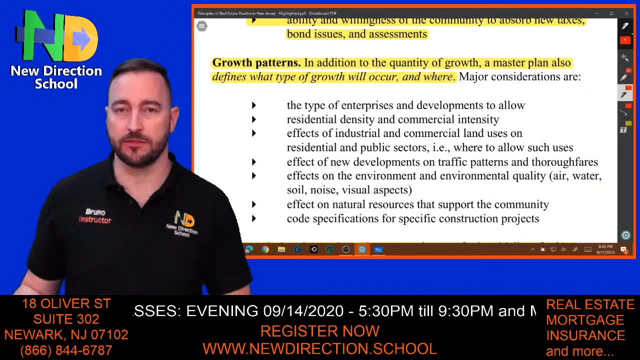 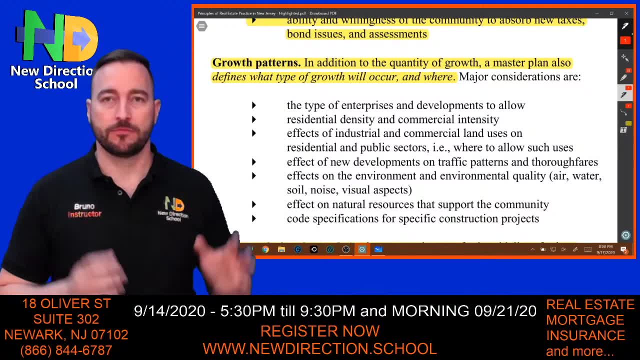 Now I know where I could place him and where I could not place him, Sometimes within the neighborhood, zoning changes within the neighborhood. You guys got it, So make sure you guys understand these things. It's very this chapter very, very important. 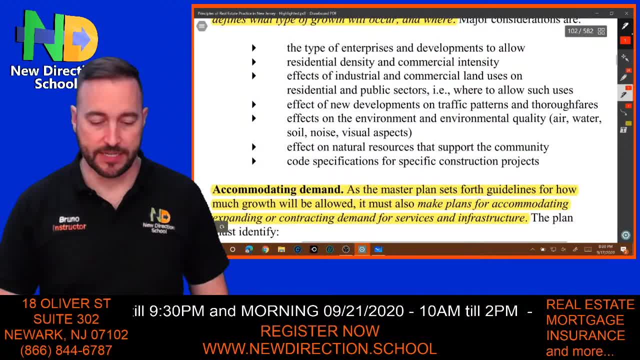 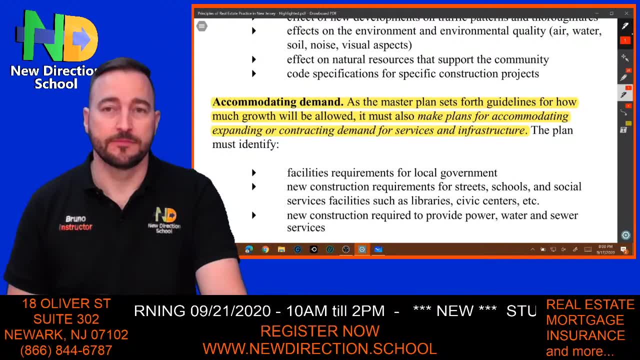 Very, very important for you, All of them, but this one in particular, very important for your success. Okay, Accommodating demands. This is obvious. Right now, there's no demand for industrial. Again, we go back to the example here in Newark. There's no demand for industrial manufacturing. Should I have a manufacturing company move to Newark? Probably not What Newark needs because of the residential demand. what Newark needs is more. We need more apartment buildings, new structures instead of the two families, three families, four right now. we need to be another Jersey City or New York City buildings. 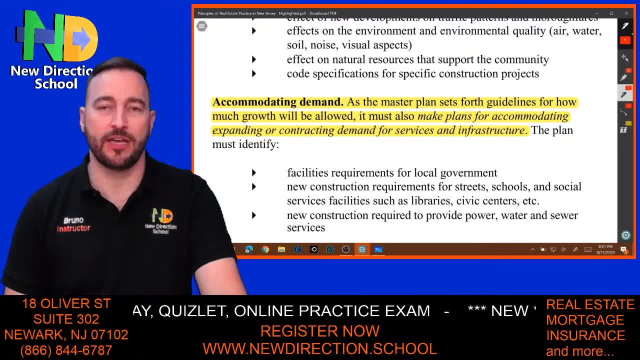 That's what's happening now, And recently Newark approved the MX three, which is mixed use three, which means they can go up to 12 floors. right, That's what's happening in the Ironbound section or the eastward of Newark. 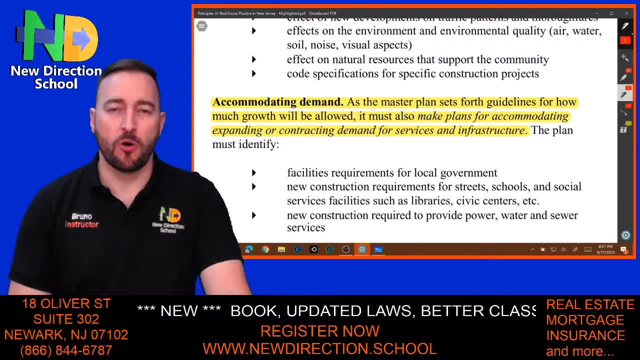 You guys understand what I'm saying. Most people don't even know about this. It was all over the newspaper, all over the news. but people don't know, they don't care. And then, once things happen, they're like: oh my God, I can't believe they're doing this, they're doing that. 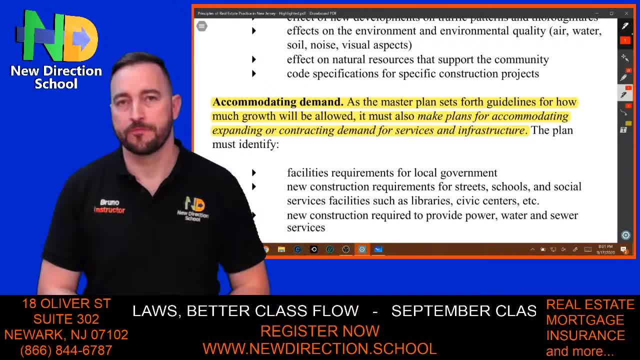 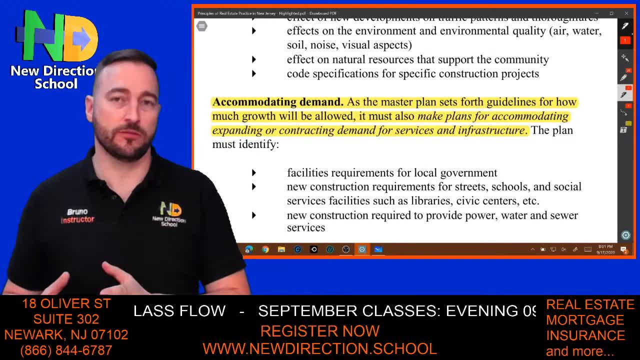 No, Okay. So make sure you guys understand what's happening and accommodate for that demand as a realtor right based on what the town is accommodating for. that demand right for that infrastructure. It also allows you to be a realtor. 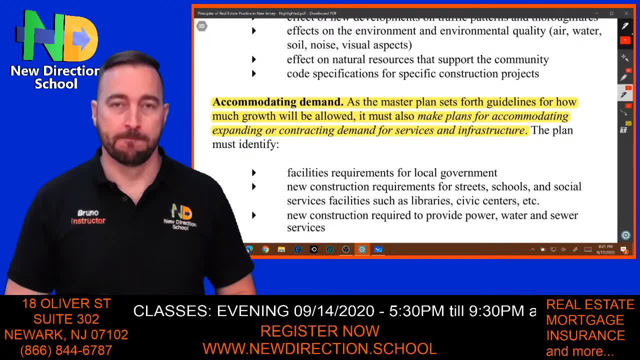 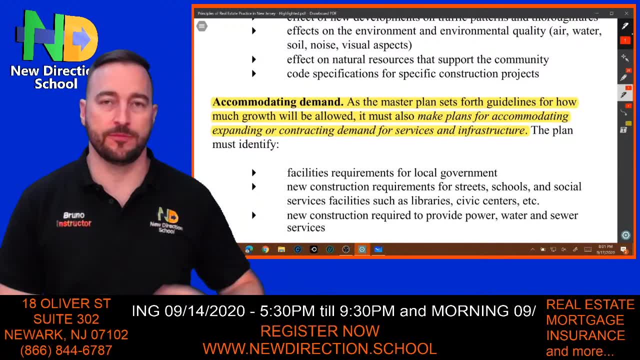 This is what's killing to be in Kearney, yeah, But all these things. if you look at it as an investor, as a professional right, it allows you to understand the market that you need to be in- Simple, The reason why we decided for this location where we are right now. we saw a few here: 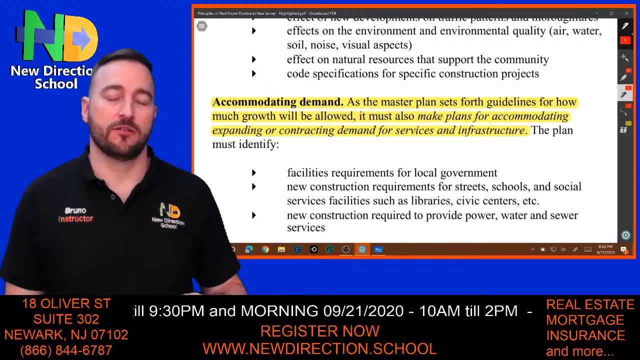 Just to give you an idea, The reason why we decided here one is all the development that's happening around, So we're very centralized. We're actually in central ward of Newark, But also we're right on Route 21.. There's an average of 25,000 cars that pass by here every day. And during wintertime, which is coming, so during the holiday season. right, it's an average of 34,000 to 37,000 cars per day. Talk about exposure. You see what I'm trying to say. You need to know what your client needs and program for that. 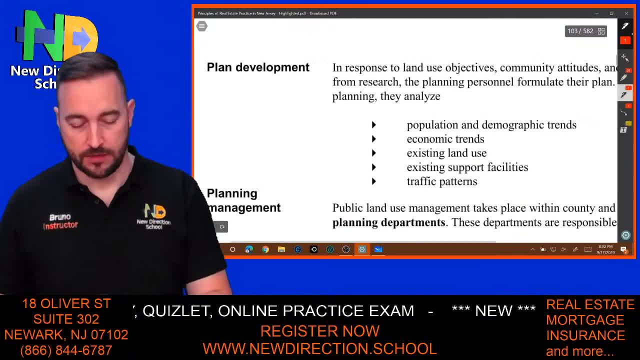 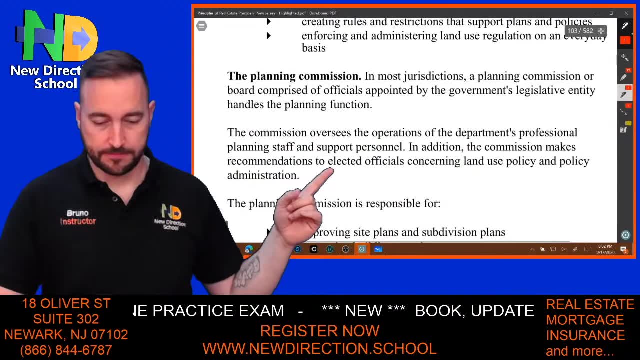 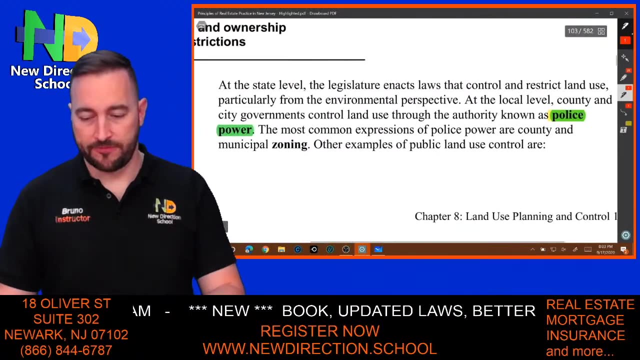 Okay, We just talked about that: Demographics, trends, economic trends, Existing and use, Go on, Got it, got it, got it. Public land use control. One of the forms of public land use control- guys- we already talked about it- is the building regulations, the zoning and all that stuff. 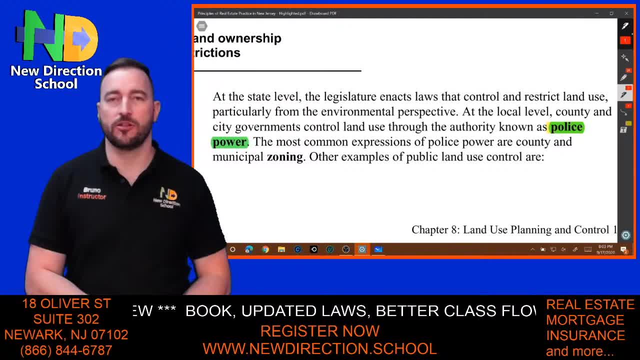 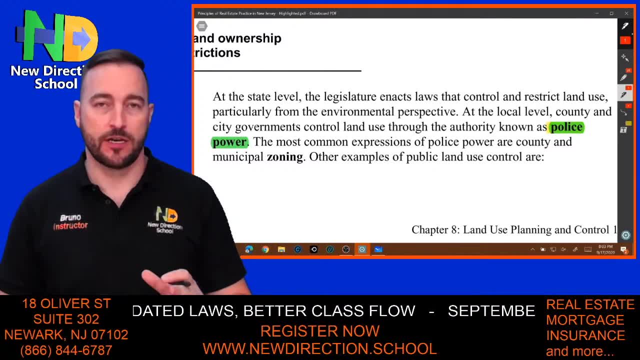 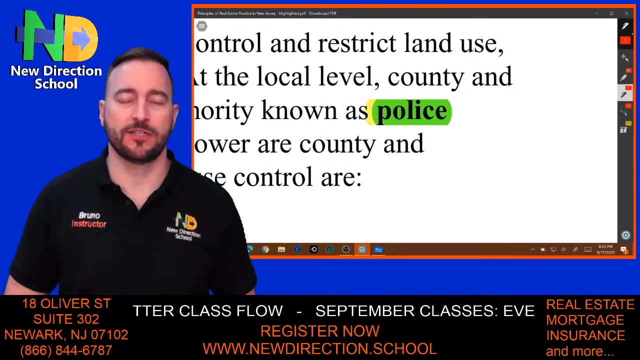 And that is called police power. I just want to talk about it real quick because you might get confused when you see in the exam. You might get confused when you see in the exam: Okay, When you see this word Police power, What does that have to do with real estate? 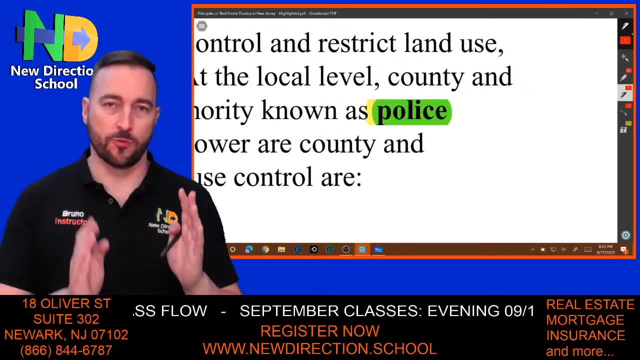 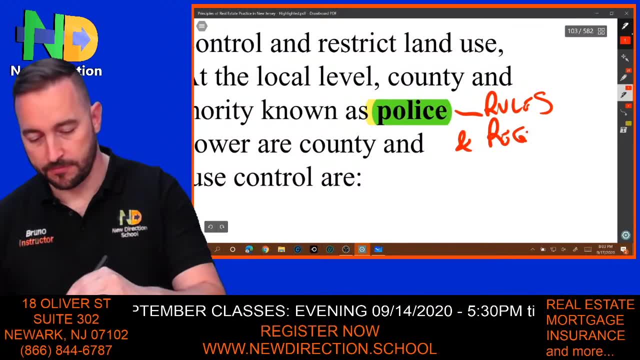 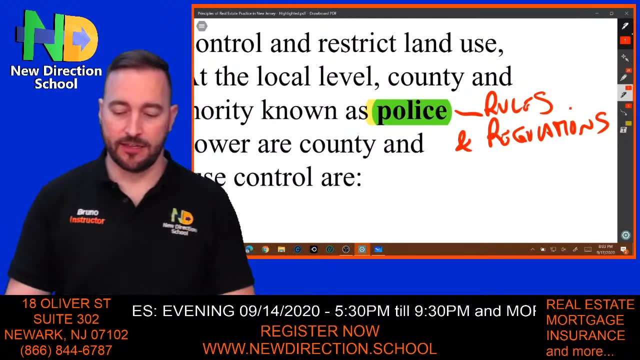 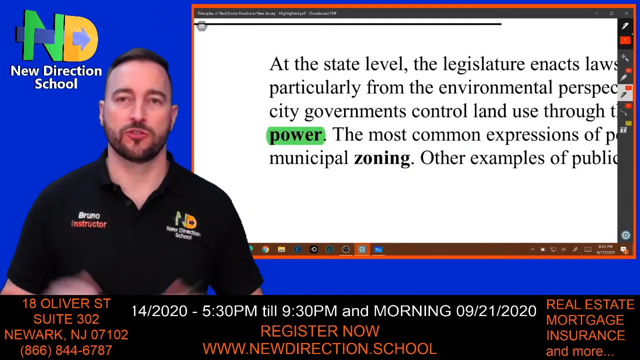 Police? What does that have to do with real estate Police? The word police means rules and regulations, So the government sets rules and regulations and then attributes that power or authority to the city. So it trickles down. But these are rules and regulations. 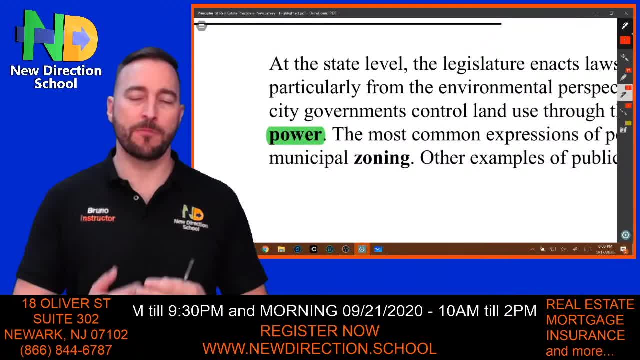 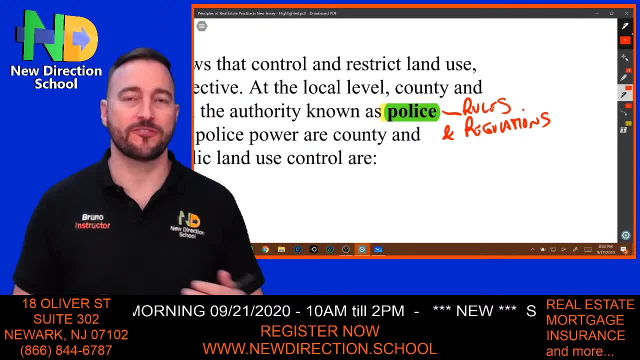 And then when you have a police officer, it's somebody that's enforcing what- The rules and regulations. The officer is not the police. The officer is enforcing police. And again, the reason why I'm saying it this way is because a lot of people don't understand. 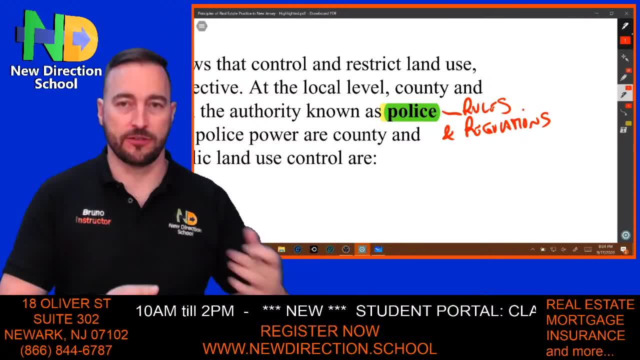 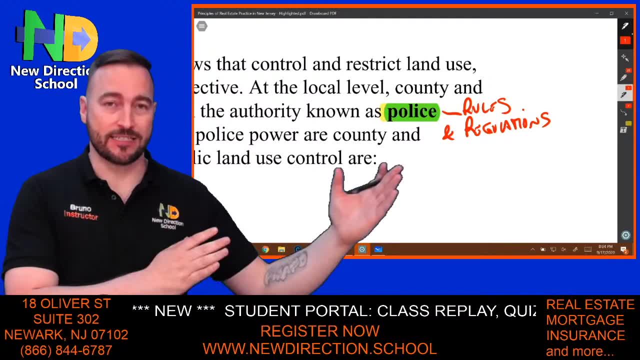 They think he's the police. No, He's a police officer, Somebody enforcing Just like Millie as an inspector. right, She's not the police, She's not the police inspector or fire or whatever inspector. It's not like that. 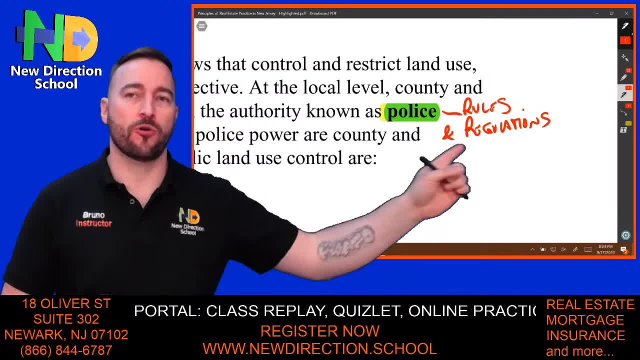 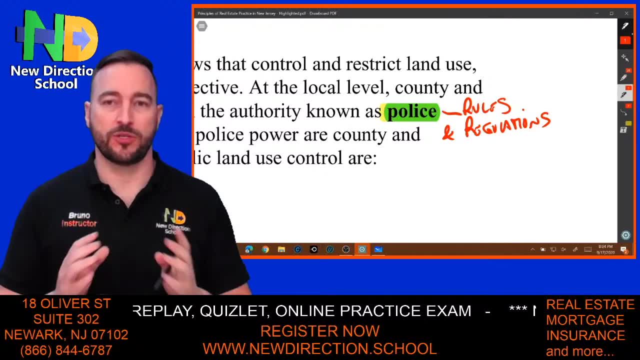 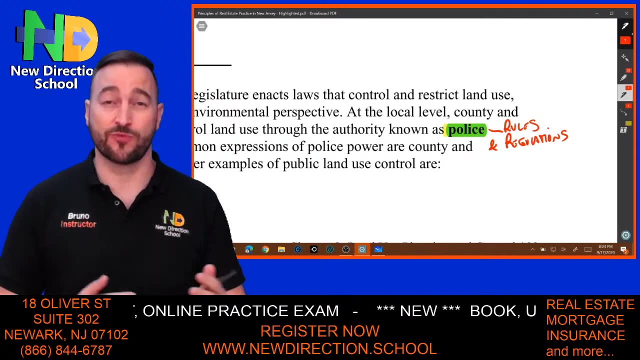 Being an inspector gives her the power to enforce these police powers or these regulations, rules and regulations. Does that make sense? So police just means rules When you go see in the exam, if they talk about which power allows the municipality to regulate or enforce certain rules, regulations, whatever you look for. 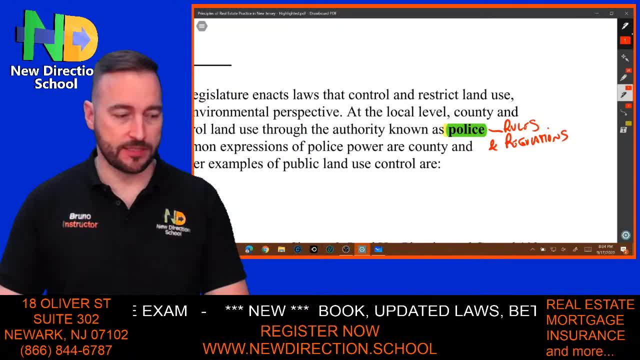 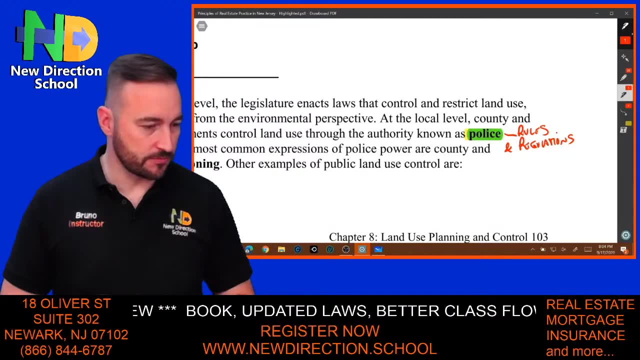 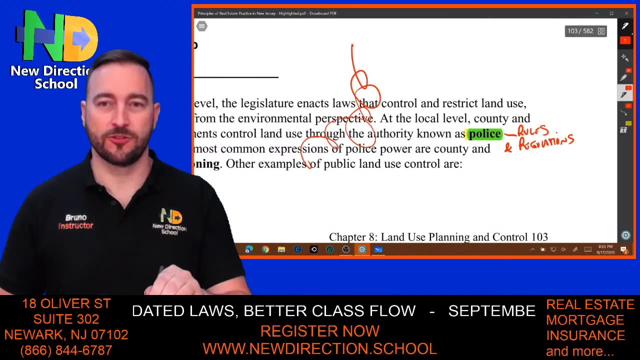 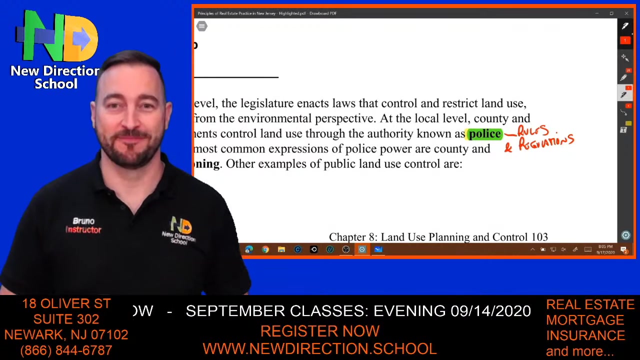 Police? Okay, Police power. What is the name of the app you're using? What To do this? Okay, It's called Drawboard PDF. It might not exist for Mac. Okay, You're using a Mac Or iOS. 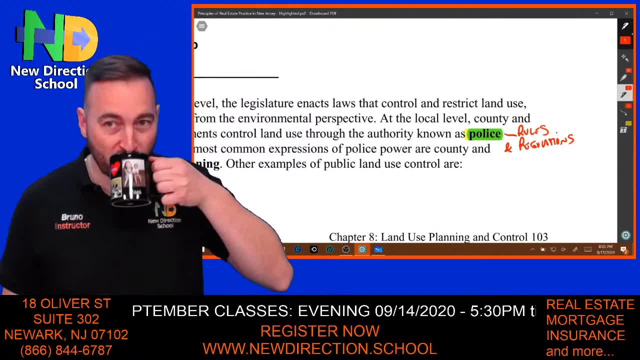 Just letting you know. Yep, Laura, I'm getting to that in a second, So Laura is ahead of the game on YouTube. She just told me the acronym I'm going to use for you guys in a little bit, So yep. 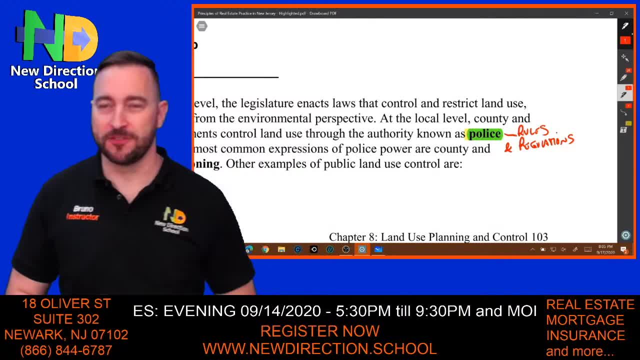 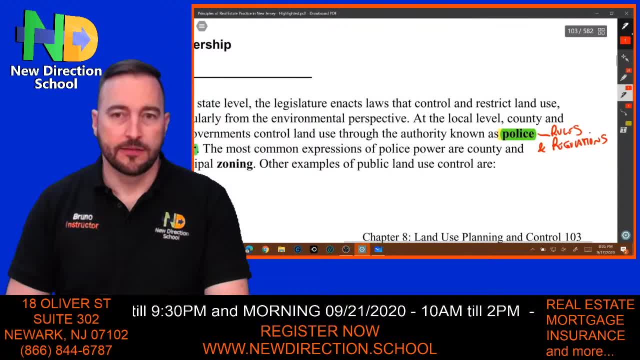 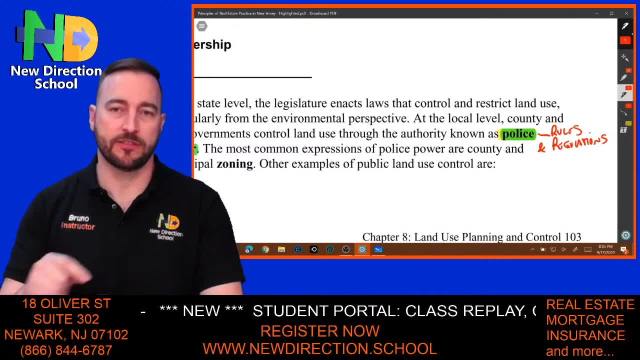 Okay, He mentioned during Zoom and instead of putting in the WhatsApp group, he put in the Zoom chat And once I'm done with the Zoom chat, with the Zoom session, it closes the chat- that I don't have access to it unless I go over the whole review of the chat. 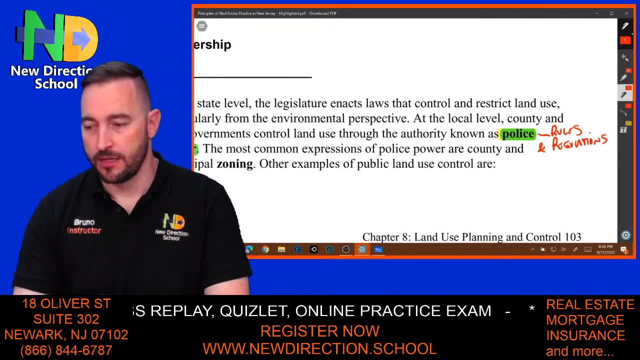 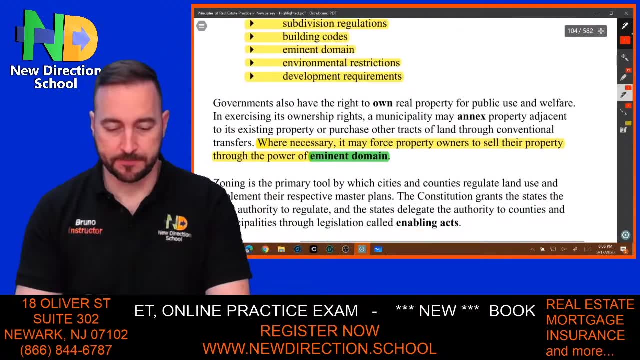 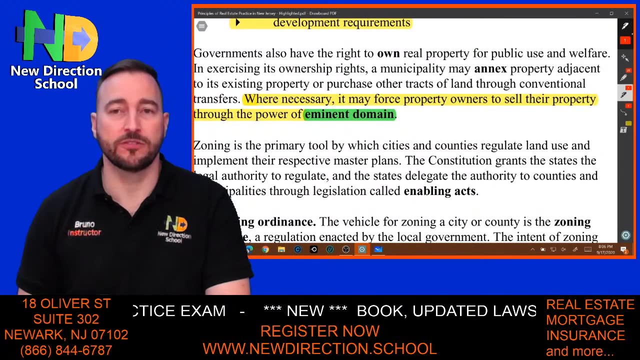 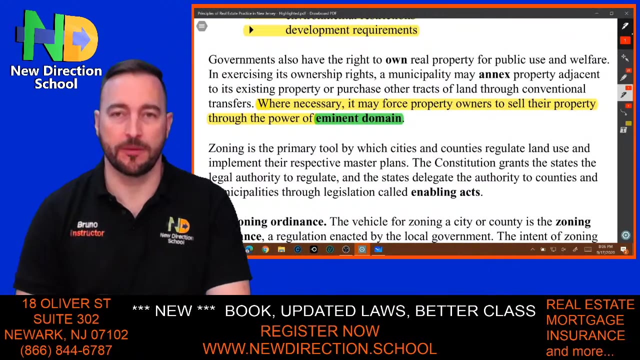 okay, but i'll let you know, all right. so police power: we talked about zoning. we already covered that- building codes and so on. the next one is eminent domain. we talked about eminent domain. you guys already know that through eminent domain, the government can take your property so force you to sell your property to them. 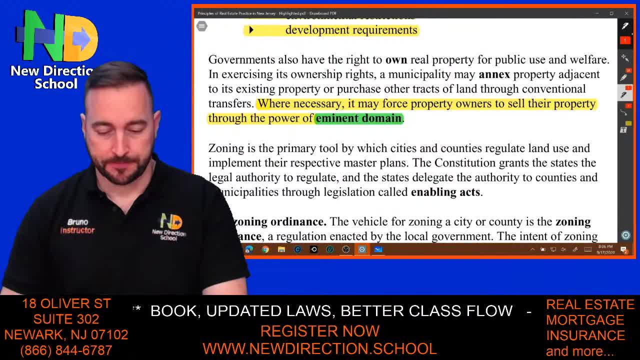 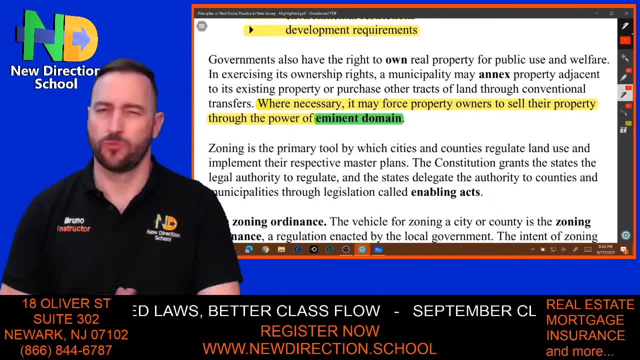 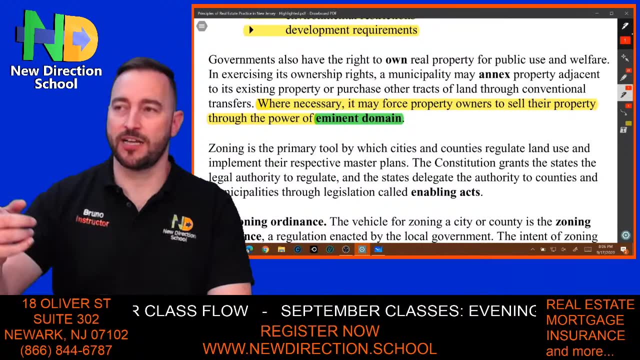 through eminent domain right. but it's very important to understand that the the even though you're selling the property. in this case- we talked about this also yesterday- you're selling the property but you're receiving compensation. they're not forcing you to sell and be out on the street. 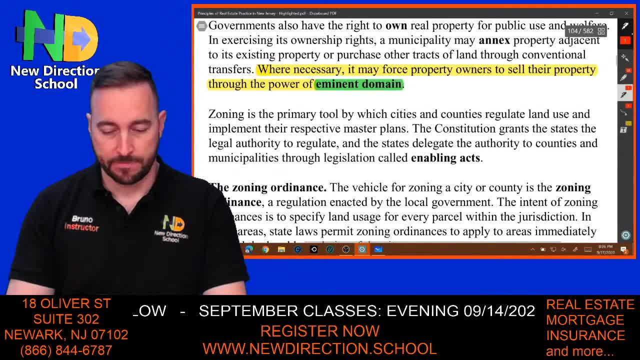 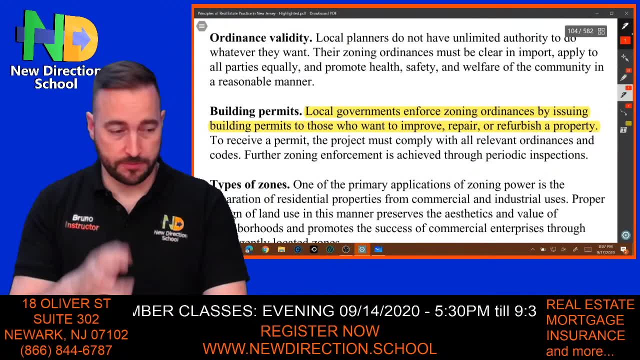 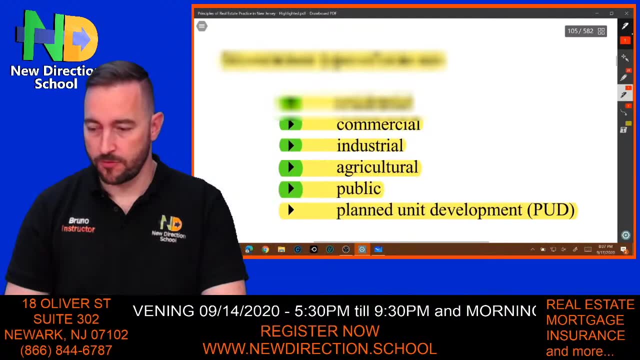 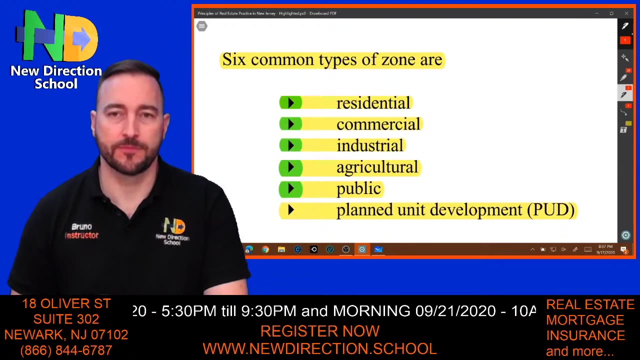 now they're giving you money for it, all right. this is also uh within the police power and so on. we are ready to go. talked about it right here. six common types of zone. notice that i only highlighted, uh, a few of them, not all of them, right? so there's? there's five main ones. okay, there's five main ones, and that's uh residential. 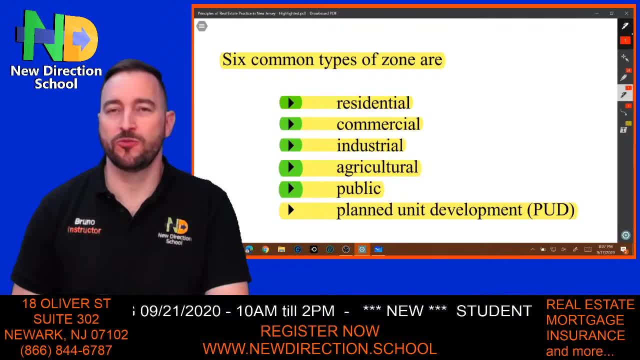 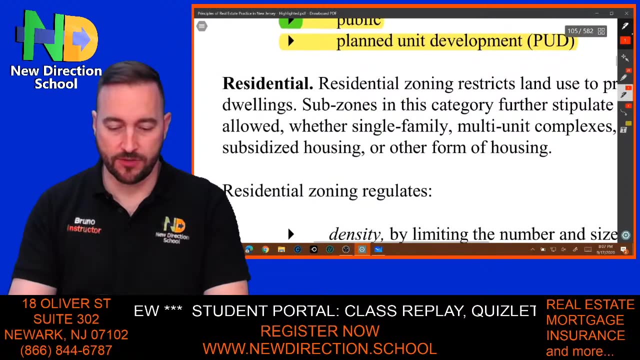 commercial, and then here there's, there's two, we'll get to them, but it's, it's a residential, commercial, institutional, recreational and, um, industrial. so we're gonna get to these, uh, in detail right now. residential, you guys know it's for homes, single family, multi-family and so on. everybody knows residential. 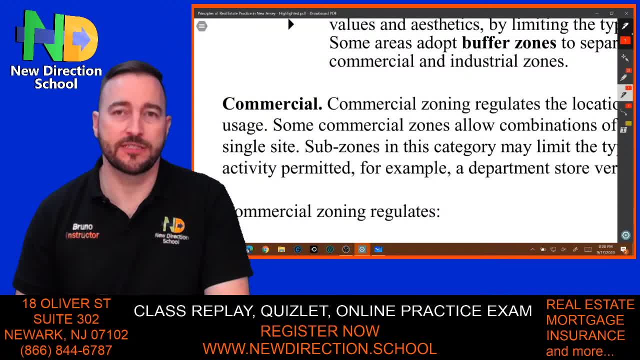 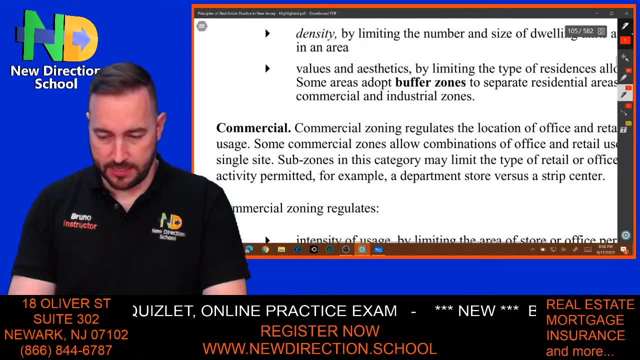 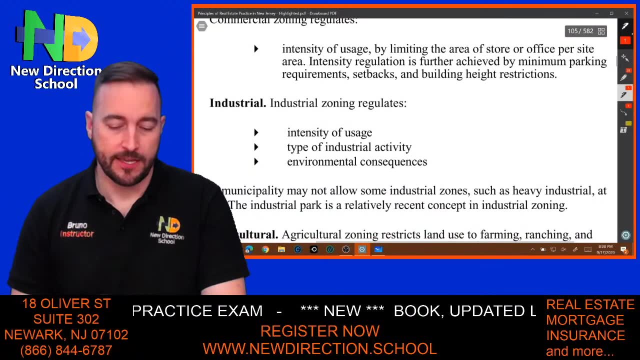 commercial. we're talking about business, right? so that's uh some things, that some things that you need to write down. permission. commercial is uh, business here is being 17.5萬 and, as you can see, right in the upper left corner here to the left, it says: 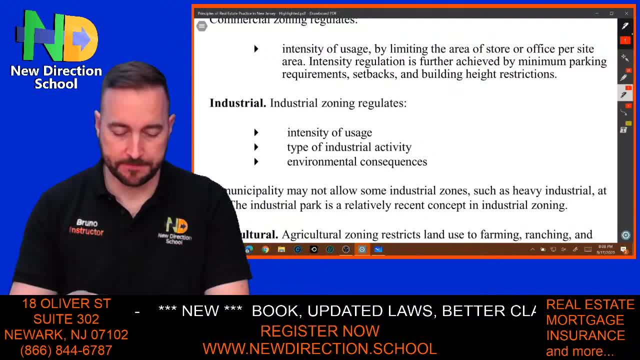 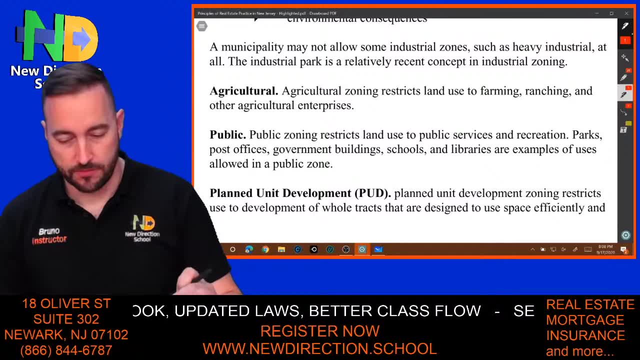 et cetera. you got some things that you need to write down. some things you need to write down. and here's me. i have to go look for the phony martial law. i can't get all these numbers because it only has oneonyfi, which is a- um, you know, black blues man. you need to write those. you. 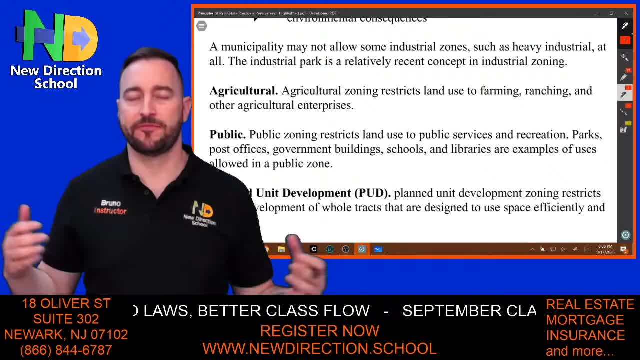 need to write down, or you need to fill in these first three daresskills, or, if you don't know, they go in your Excel ID and then they come up and they tell you your- emphasize, your Crystal score. okay, i'm just going to say i did. 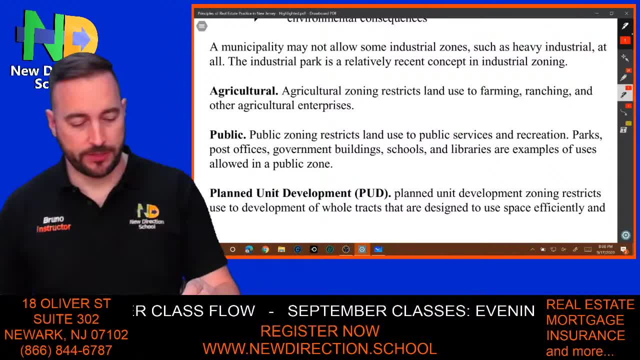 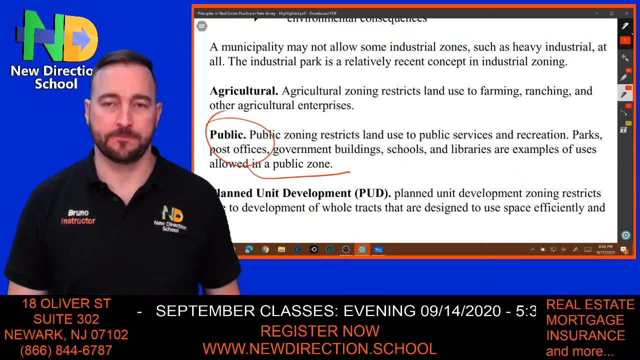 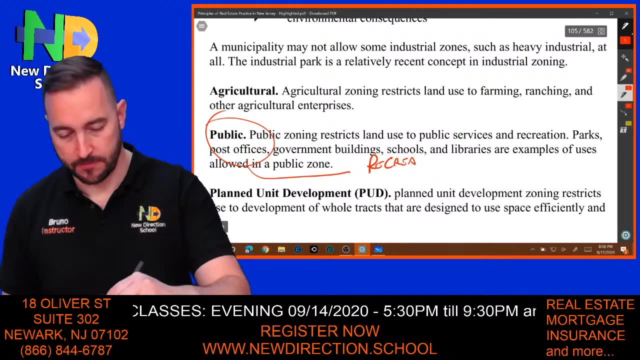 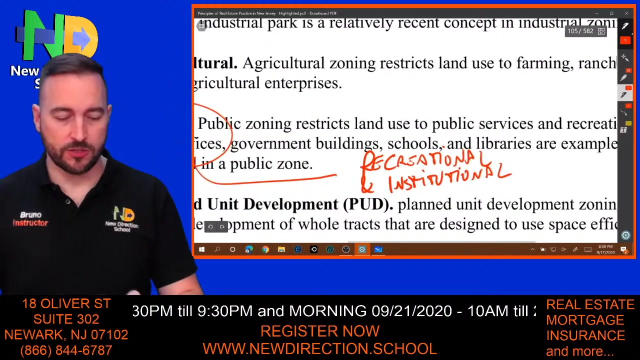 They are separate, as you can see, Under public- that's what I want you guys to remember- Under public there's two different types of zoning that are very important: Ready, Recreational And institutional. So under public, we have recreational and institutional. 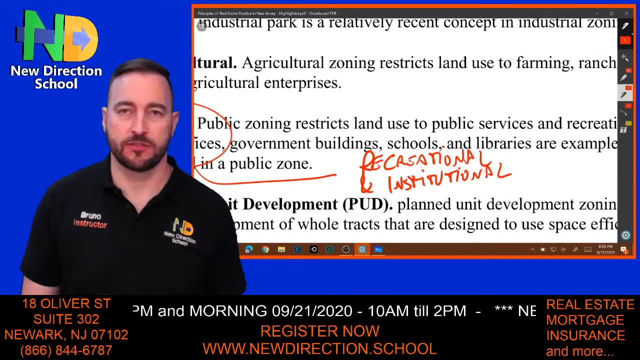 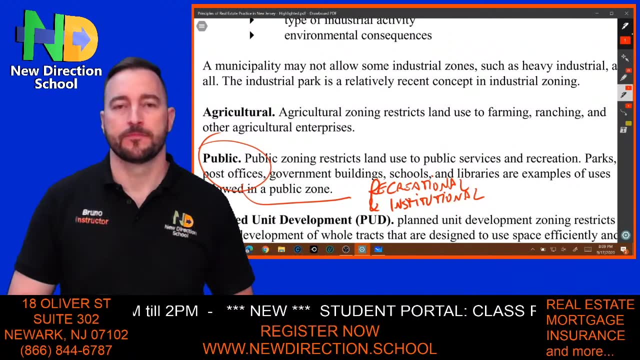 Why? Recreational Parks, for instance, Institutional? you're talking about government buildings, schools, libraries and so on. Right? So institutions, hospitals, institutionals. So what are the five main types I know? here it talks about six. 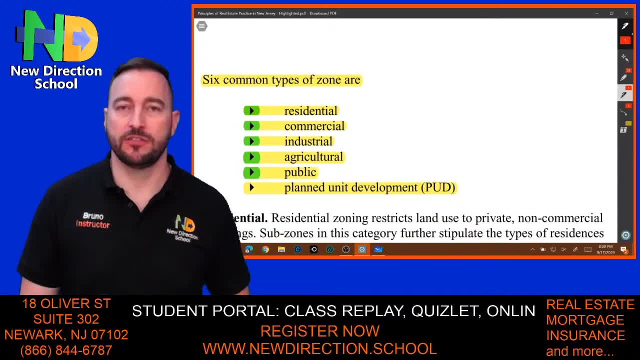 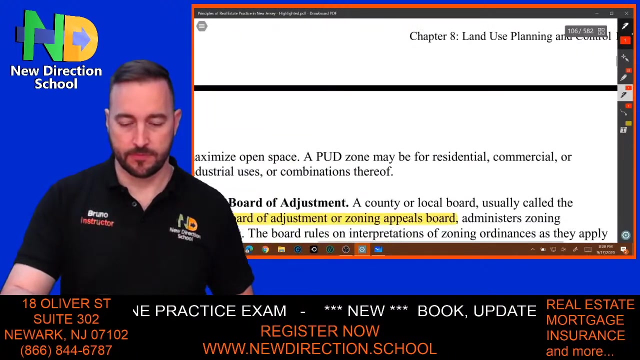 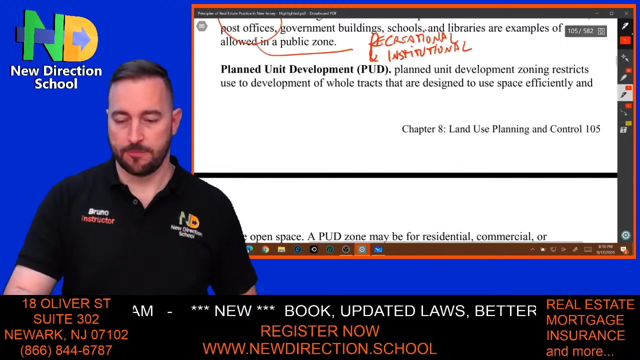 and they're a little bit different, But the five main types you need to remember is residential, commercial, industrial and then under public. we're gonna split this into two: recreational and institutional. okay, Plan unit developments: if you ever hear about plan unit developments or PUDs, it's like 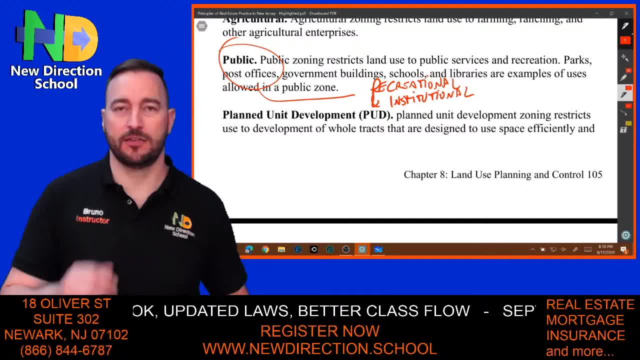 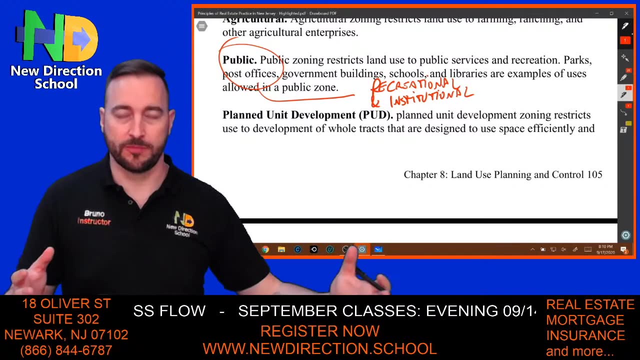 having a town within a town. It's a totally separate segment within the municipality. so they have a whole tract of open spaces- it says here, and then they transform that into a mini complex, let's put it like that, And within that complex you have almost all the benefits. 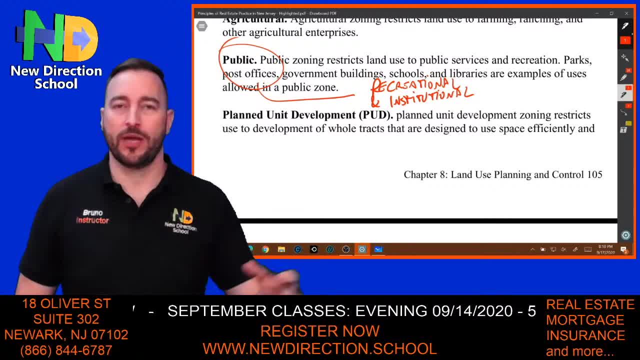 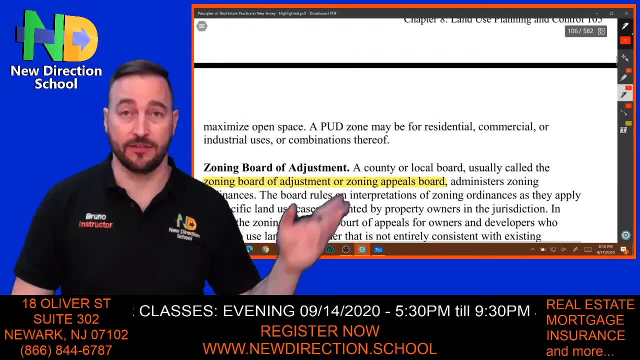 You can have businesses, you can have recreational, you have a bunch of stuff there, but it was planned to be commercial. it could be a combination, as it says here, So they're maximizing the space within a small part of the town. 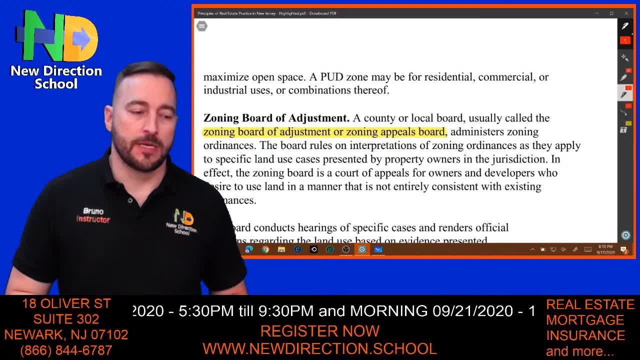 Zoning board of adjustments. So if you guys are not happy with the way, because things change, zoning changes- I told you let's go back to Newark. I told you that Newark was industrial and now it's changing a lot of stuff to commercial. 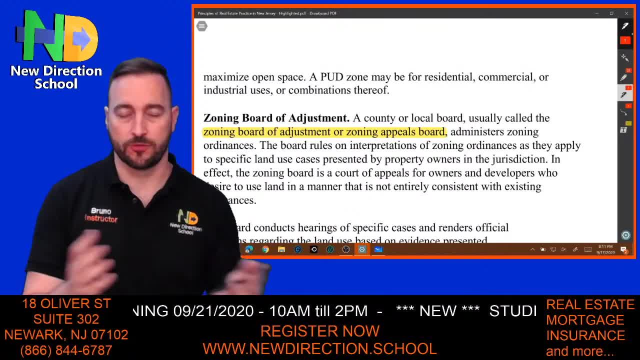 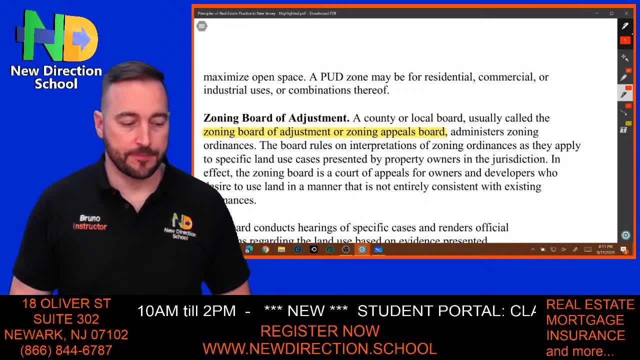 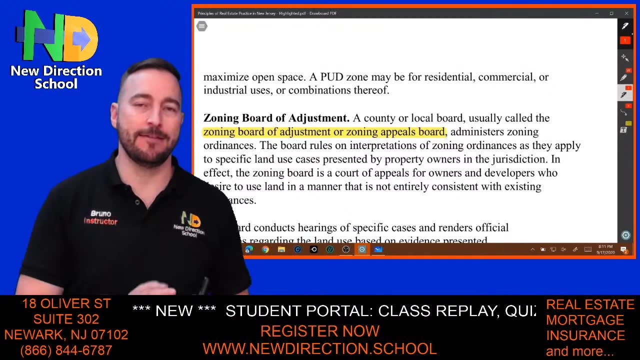 or residential Manufacturing is out of here. We have a section that still has a lot of manufacturing, but the majority of Newark is gone, Jersey City as well, and so on. If there's a change in zoning and that change in zoning impacts, 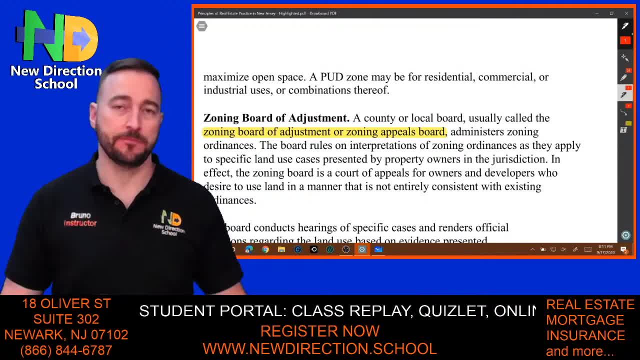 your lifestyle or your business, whatever it is that you have here. if you're not happy with something, with any change. guys, what can we do? If we're not happy with something, we can cry about it, right? It's a very old saying in Portugal. I'm pretty sure in several countries you have this. 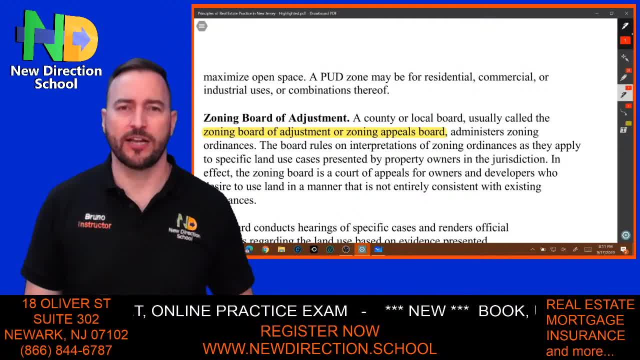 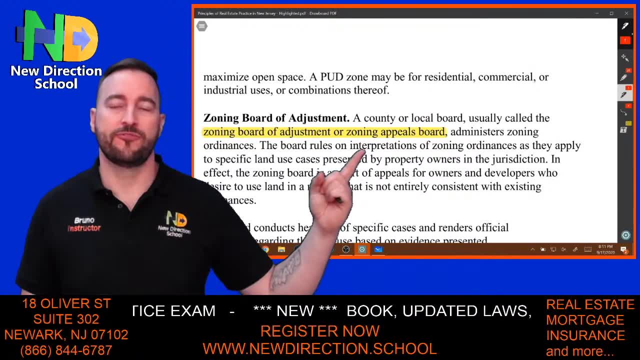 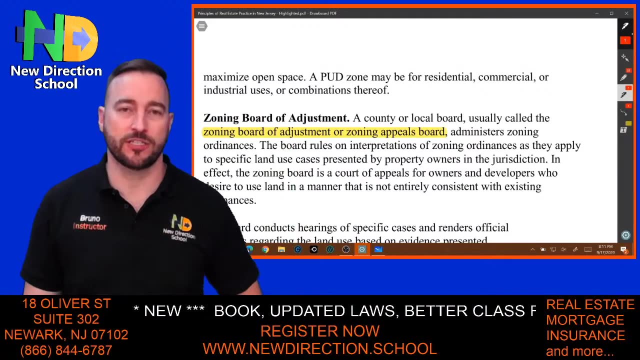 If you don't cry, you don't get to eat. So rough translation: when babies cry, they're usually asking for something right? They're uncomfortable, They need something. So if you're not comfortable with the change, You can always appeal to the Zoning Appeals Board or the Board of Adjustment, because 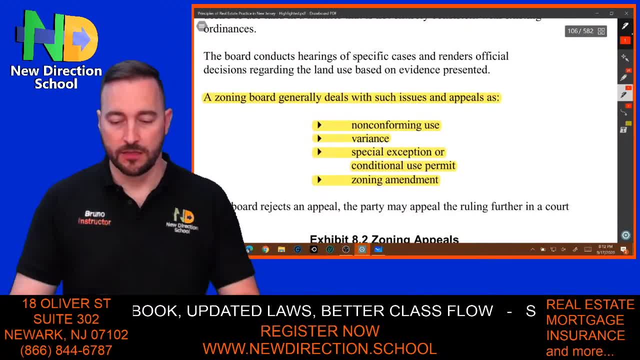 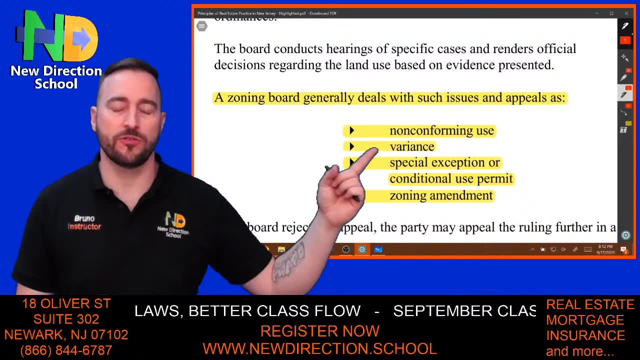 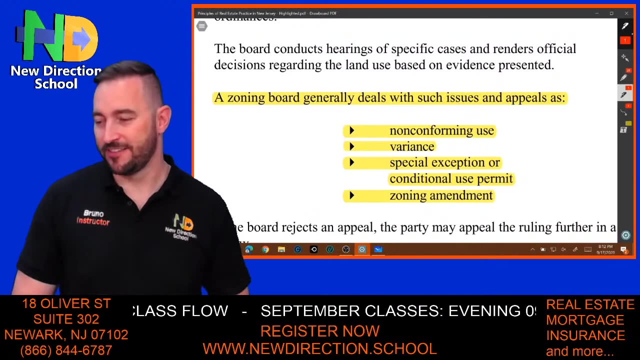 that's where they make decisions, So the Zoning Board generally deals with such issues and appeals as non-conforming use, variance, special exception or conditional use permits and zoning amendments. Laura is on point. I didn't even get here, She was already talking about variance. 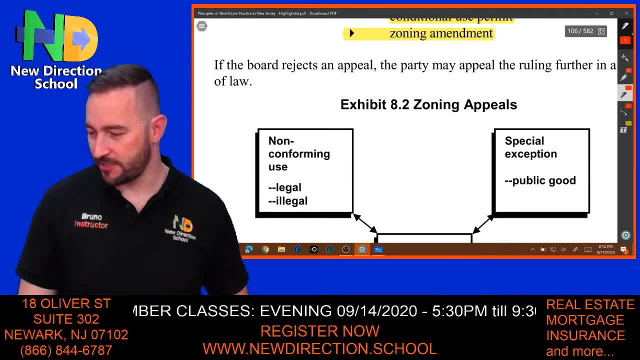 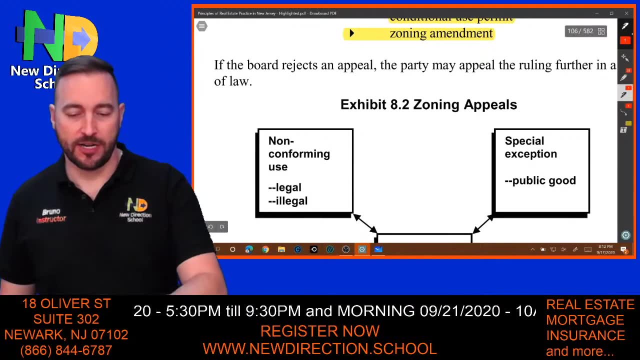 Cool, There you go, Laura. your test is on the 19th, If I remember correctly. that's what you told me Coming up doing. great, All right. So if the board rejects an appeal, that the party may appeal the further ruling. I mean. 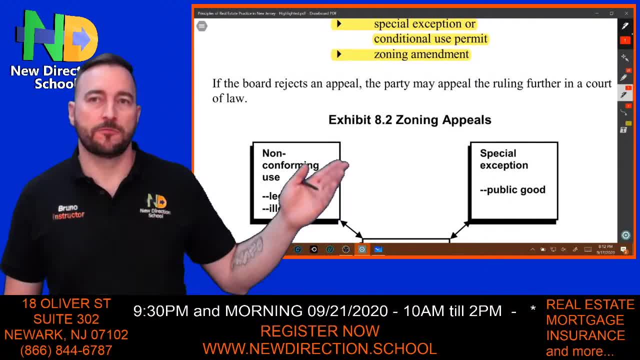 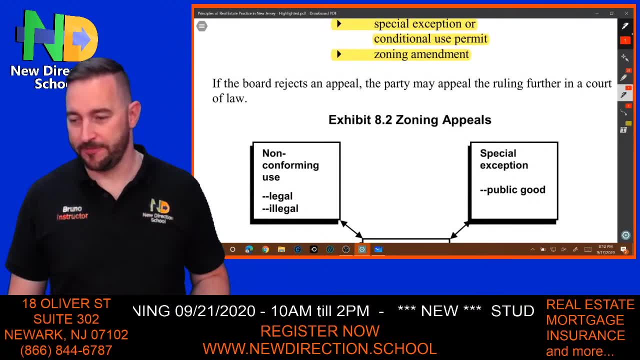 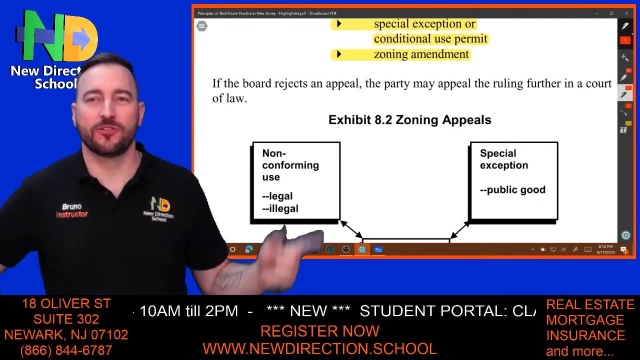 the ruling further in the court of law. So zoning appeals: You change it to the 20th, You change it to the 23rd. Why Just get it done? Don't change anything. So zoning appeals: Non-conforming use could be legal or illegal. 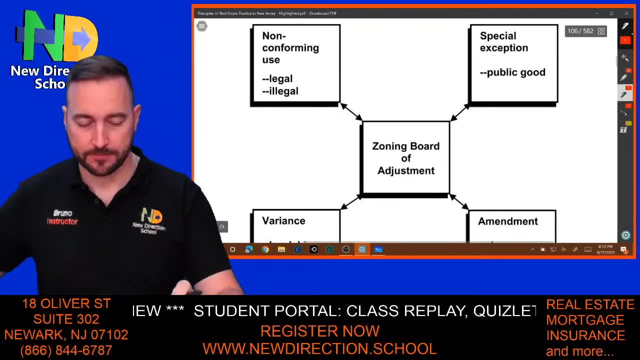 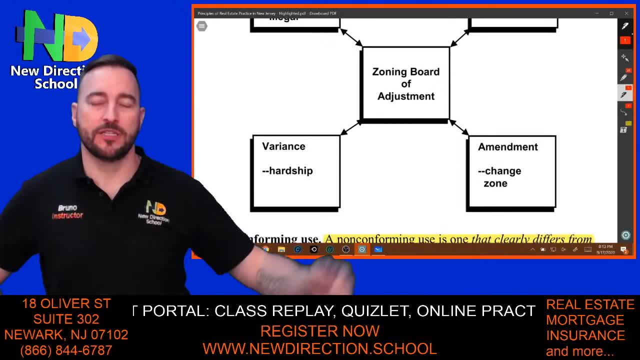 Special exceptions, which is for public good, and I'll talk about it in a second. Variances because of hardships and amendments because of changing zoning- All right, So let's start with non-conforming use. What is non-conforming use? 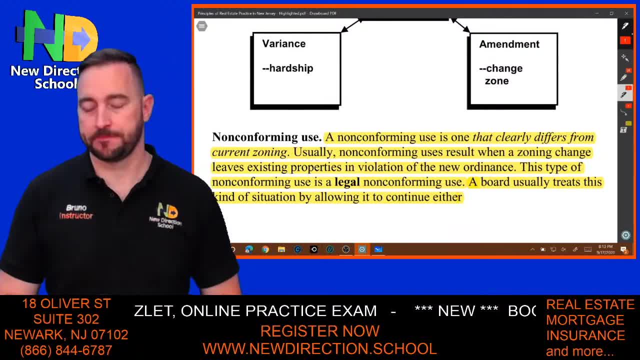 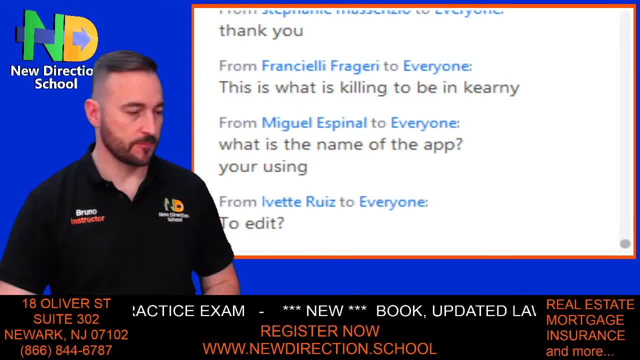 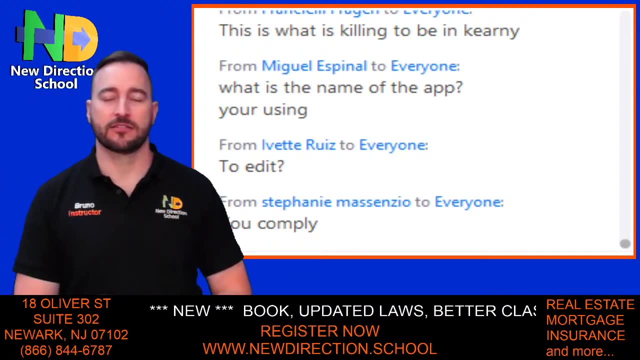 Quick question: What is something that's conforming, Conforming, The word conforming. Does anybody know what it means Conforming In compliance? Yes, All right, I don't comply with anything, but okay, In compliance, Very good. 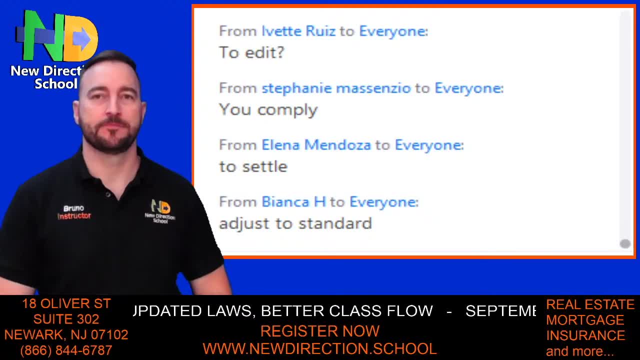 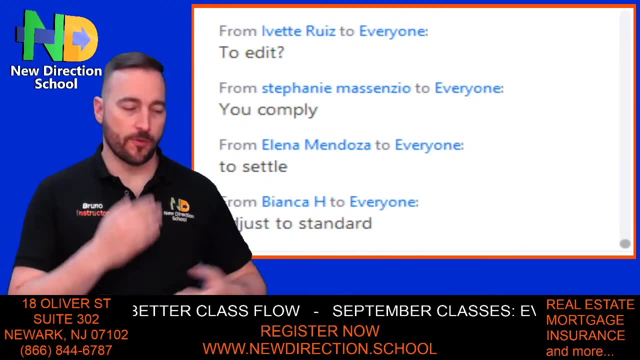 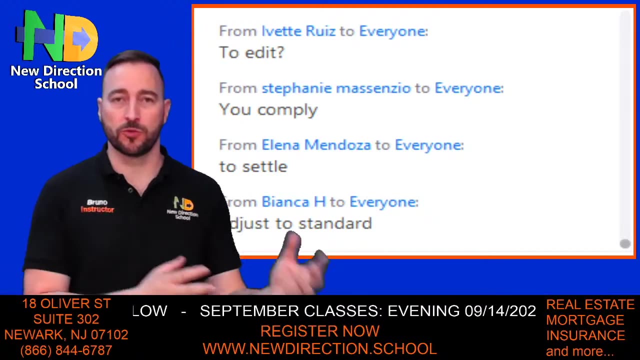 To settle. Okay, I can use that Adjust to standards. Yes, So if you guys understand what was written here, these are all correct their own way. But conforming is following certain standards. to comply with current rules. to settle for certain rules. 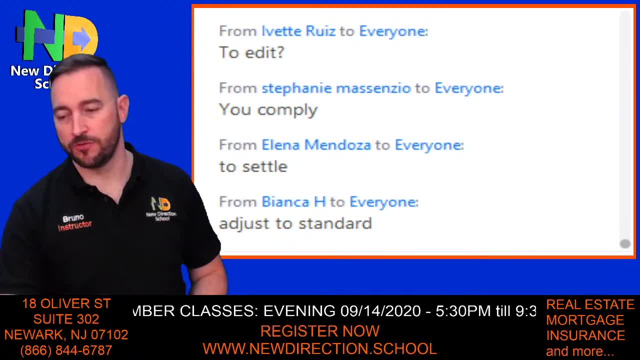 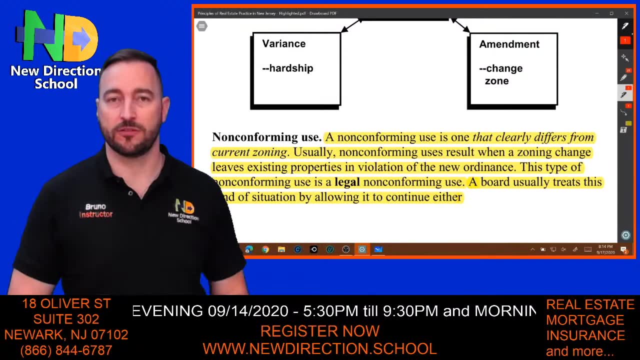 Okay. So when we're talking about non-conforming use, it's something that goes against the grain, something that goes against the standard, something that doesn't comply with whatever was implemented. Now, non-conforming use is allowed for properties. They're already there before the change of zoning. 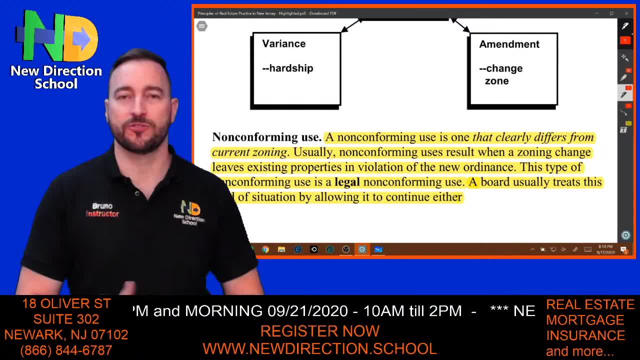 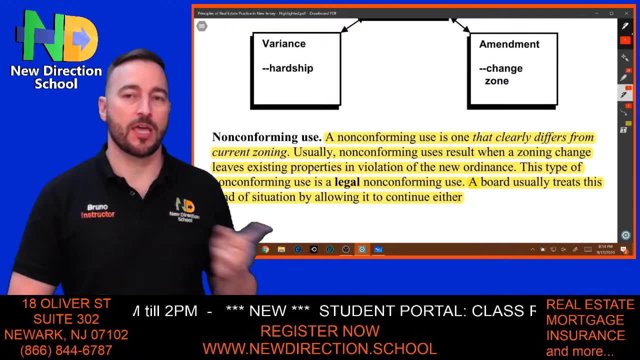 So I'll give you an example Again. let's bring Newark and the industrial sites. industrial sites converted Now, most of them converted to commercial or residential. but because it converted to residential, we have to tear down that factory and make everything converted, everything to. 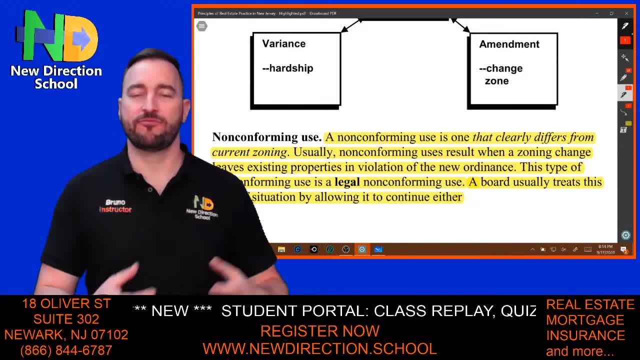 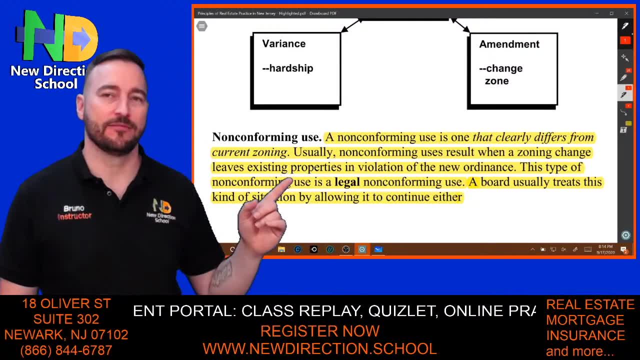 residential. We don't. it's grandfathered in, So they allow right. They allow the legal non-conforming use. It was existing but it's not in violation of the new ordinance. because it was existing already, I don't have to tear it down. 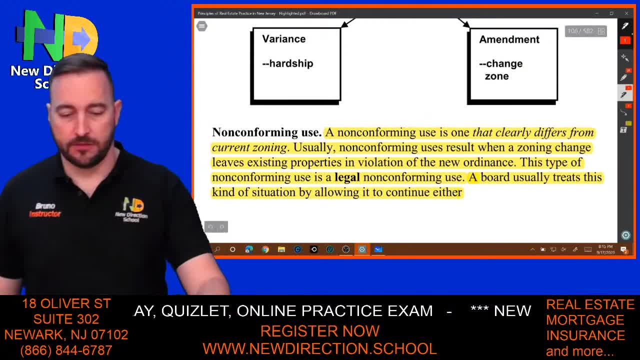 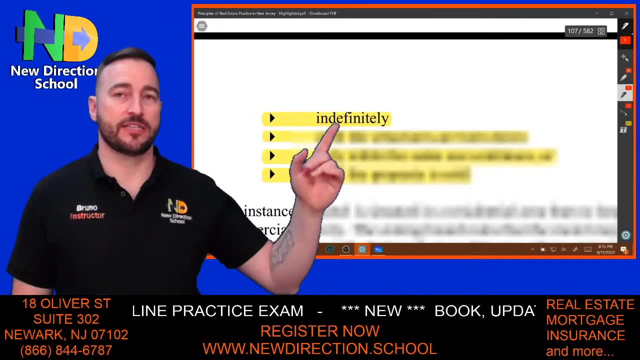 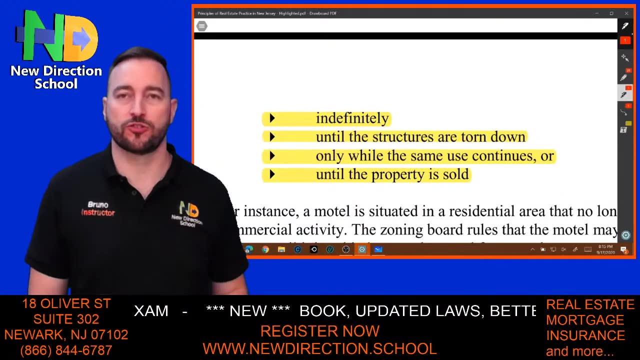 Okay, So the the non-conforming use could be altered, though right here it could stay indefinitely If nothing changes, But if the structure is torn down. so if something happens to the structure, right, then the new structure must comply right. 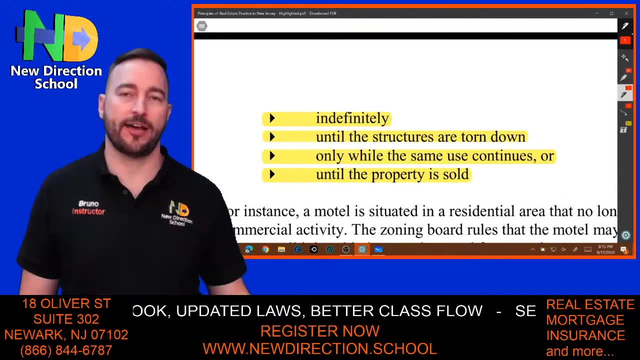 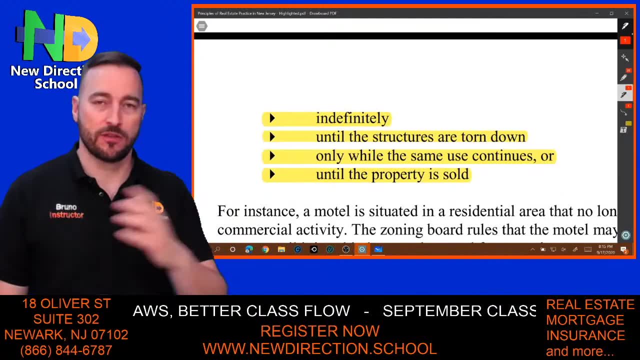 If the same use continues, then you don't have to change, right. But if the use is abandoned, the current use is abandoned- Then the new structure cannot be used the way it was before. I mean, the old structure cannot be used in the same way. 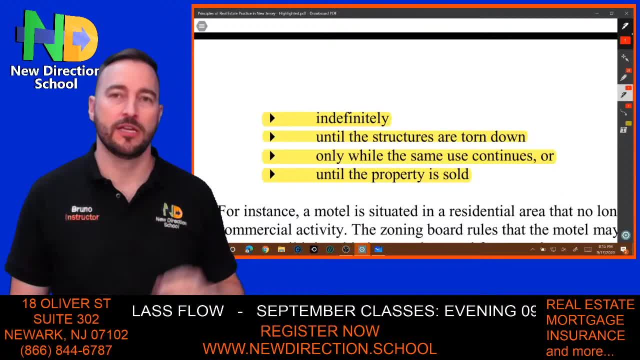 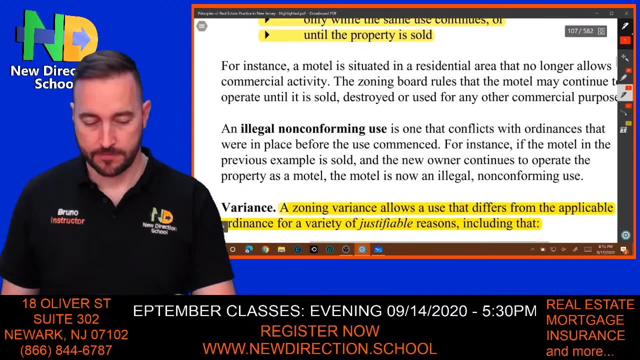 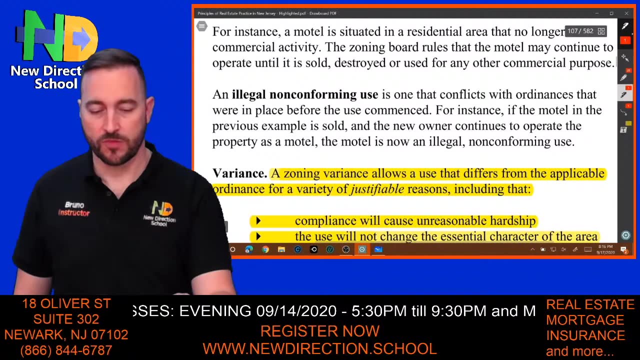 It needs to comply, just like a property being sold, It needs to comply with The new zoning ordinances, with the new laws. Okay, Right here. This is a great example of illegal, non-conforming, for instance. in this case we're talking. 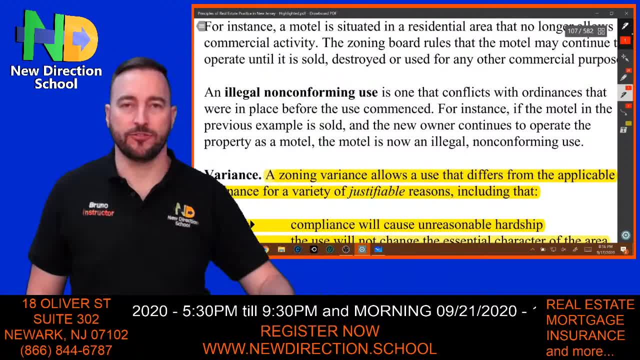 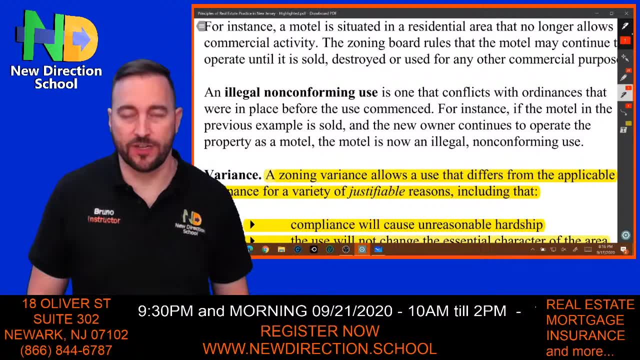 about a motel: zoning changed right And the it's saying it changed to residential. So if it's residential, Okay, A motel is not residential, You're sleeping there, but it's not residential, It's not your residence, right? 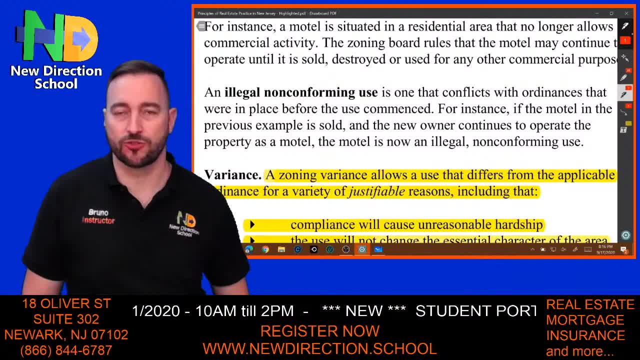 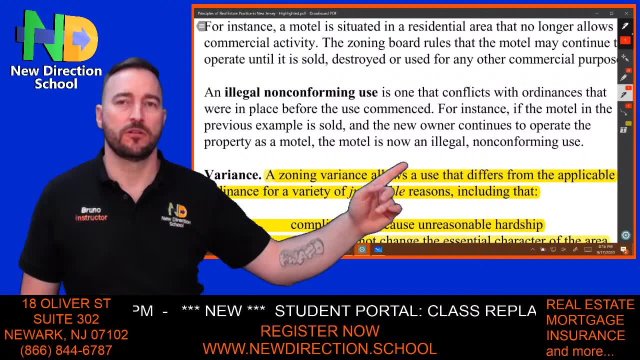 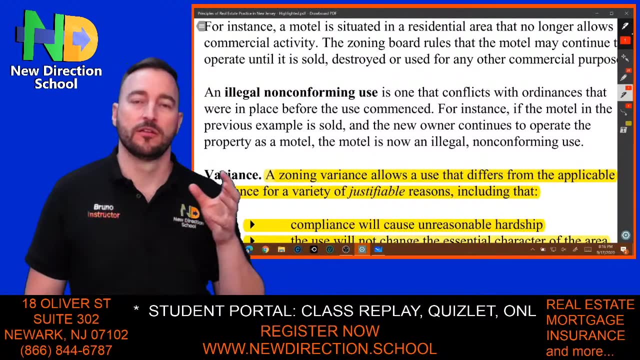 It's a business. So if you change it to residential once the motel is sold, the new owner cannot continue to operate as a motel. So now it has an illegal non-conforming use. Okay, So there's legal non-conforming where you're still within the guidelines. 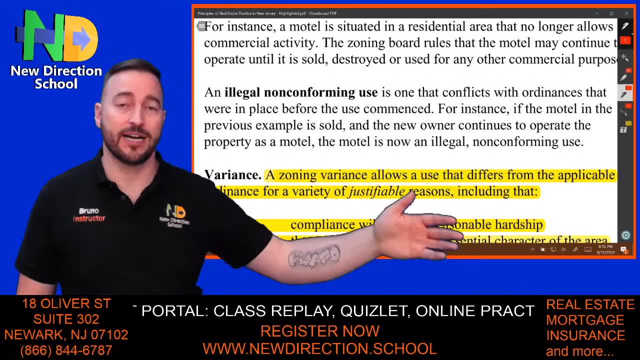 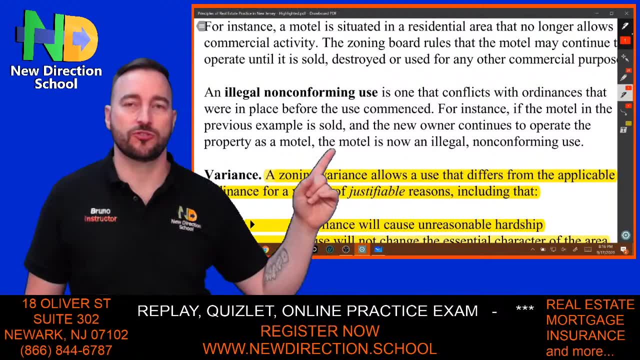 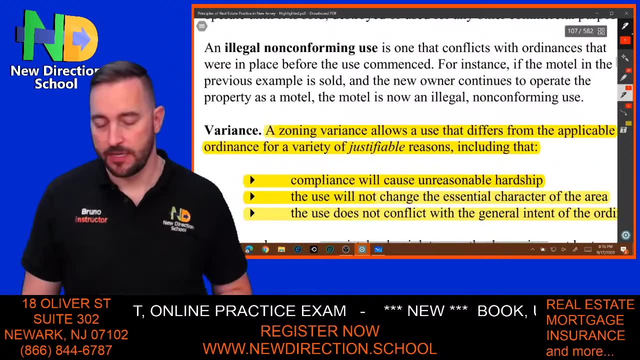 It wasn't sold, It wasn't torn down whatever, Still within the guidelines that was before. If it's sold or torn down or abandoned, then it has to change to the new standards or it becomes an illegal, non-conforming use. A variance. 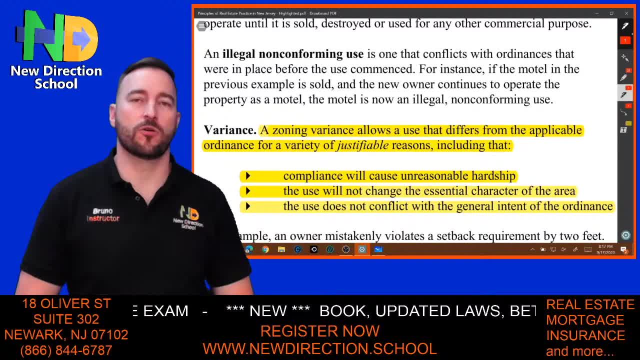 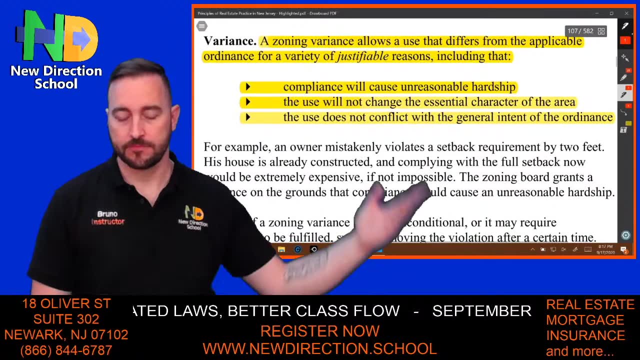 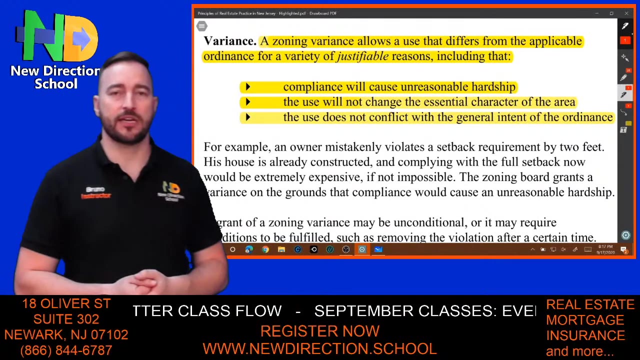 A variance zoning, variance or variation zoning, variation, variance or variation is where we're stepping away from the current zoning. So let's assume, let's assume for a second, that right here, a setback, the new zoning, the new zoning says: um, you have to be six feet away. 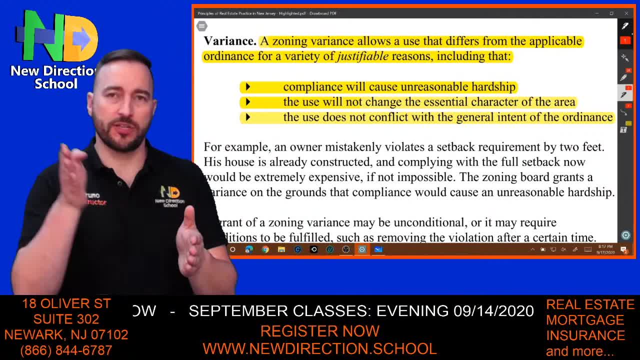 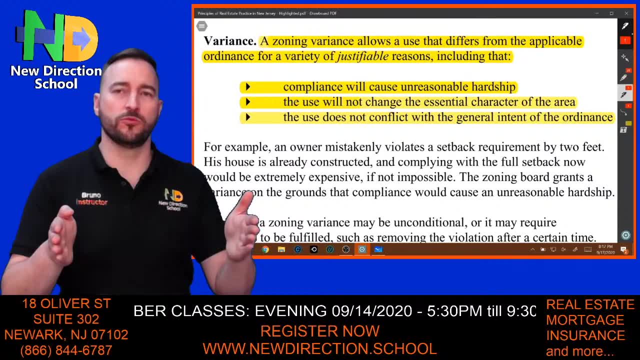 Most, most places now have something like this: Your, your building structure must be six feet away from the road. Okay, Six feet away. In this example, it says that the owner has a setback from the road of two feet. Okay, 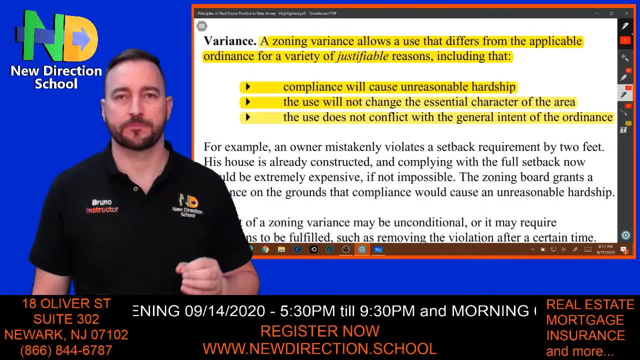 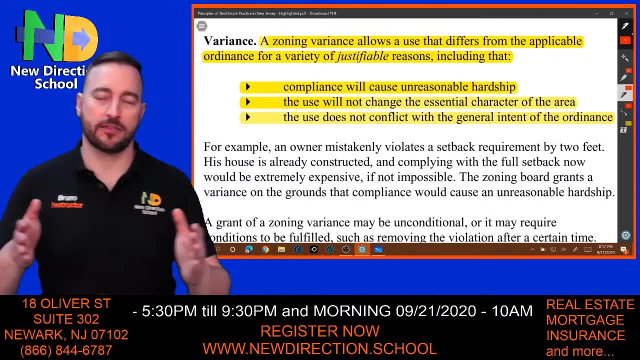 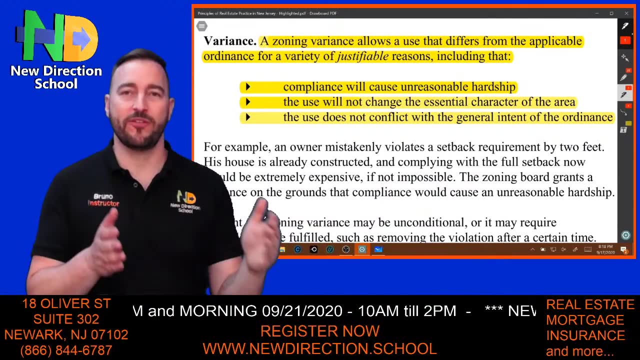 The house is already constructed, So if he had to comply with it, you would have to tear down the house and move it back, Right? So somebody allowed them to do this. Nobody regulated it at the time that he built it, but it would be very expensive to tear. 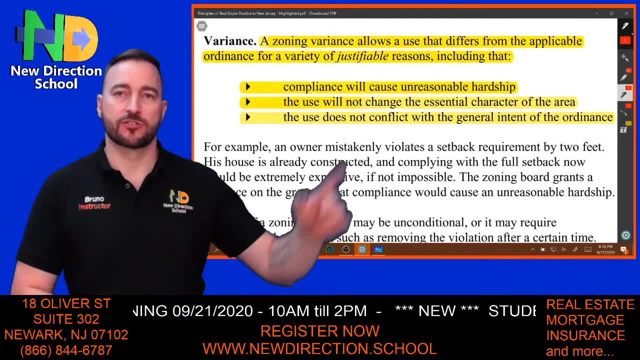 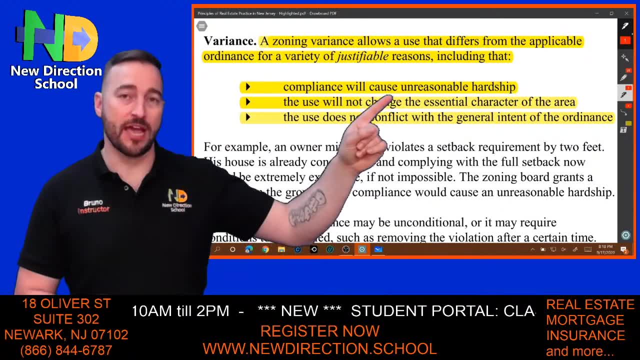 anything down just to move another two feet. So they might allow, when you appeal for a variance, they might allow, Okay, The property to stay with that two feet. only if it would cause an unreasonable hardship. it wouldn't make sense to force you to tear it down. 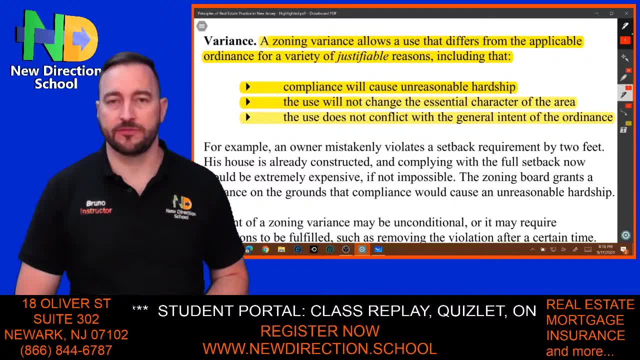 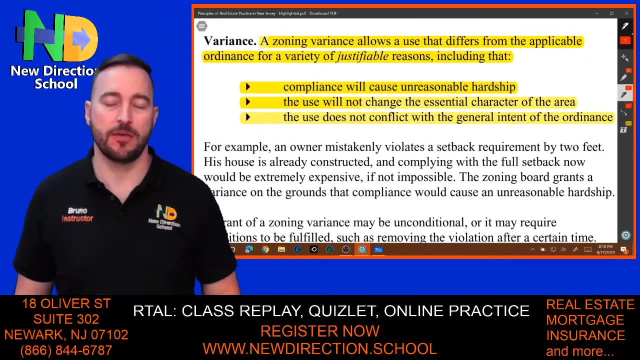 Okay. If the use does not change the essential character of the area, sometimes it might be allowed. If it does not conflict with the general intent of the ordinance, sometimes it may be allowed. Okay, So that's variance. Okay, So that's variance. 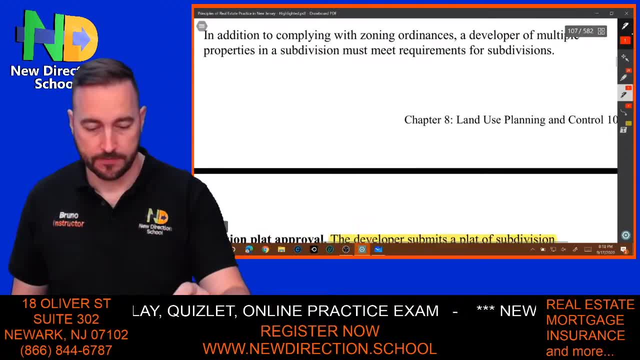 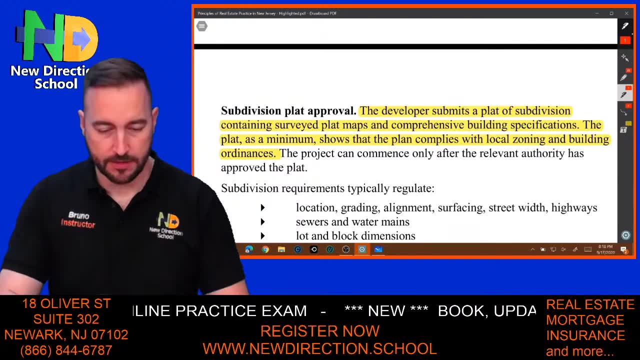 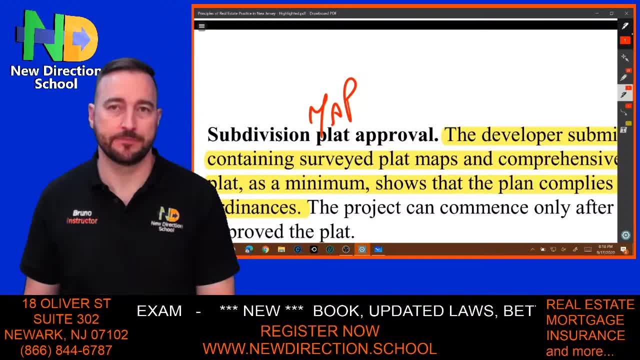 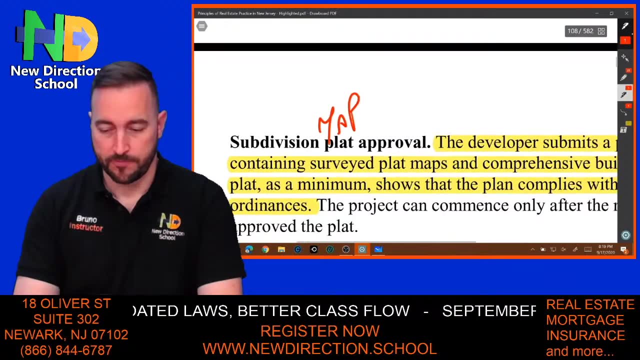 Every time you see the word Platt it means map. Okay, So a subdivision plot is simply a map of the subdivision. It shows the whole subdivision, versus a map or survey of that individual property. Okay, So it shows the whole subdivision. The developer submits a plot of subdivision. 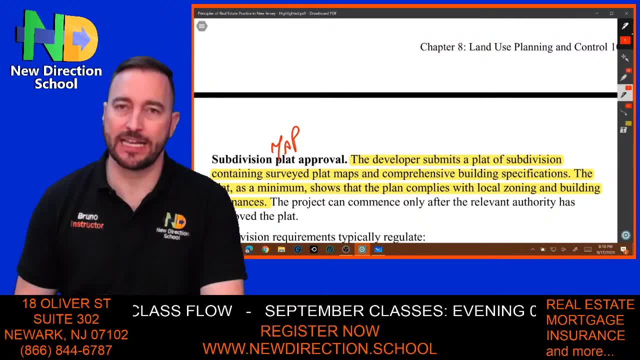 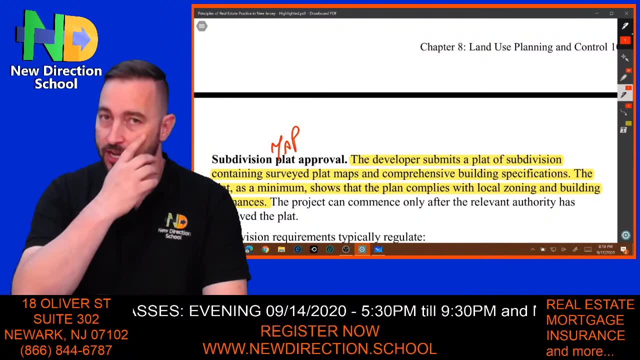 Once this is approved, then it shows all the buildings, just like a survey. it shows all the buildings that go with it and the intention of the developer, just like a survey. right, This is submitted to the city, The building department or zoning department, whoever it is in. every town has different rules for this. 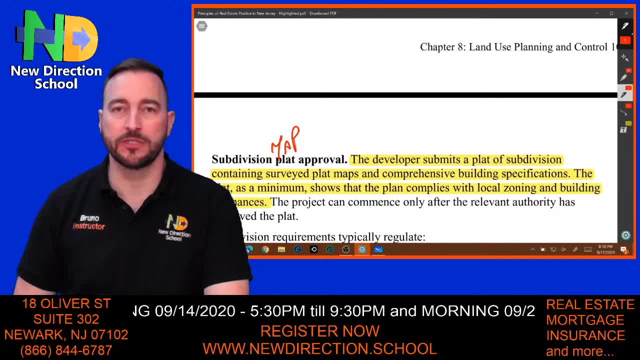 Some places have an independent zoning department, Some places have independent building departments, Some have it all combined. Some are so small that the town next to it is the one that controls the zoning in that one right as an example. So they submit this to be part of the master plan. 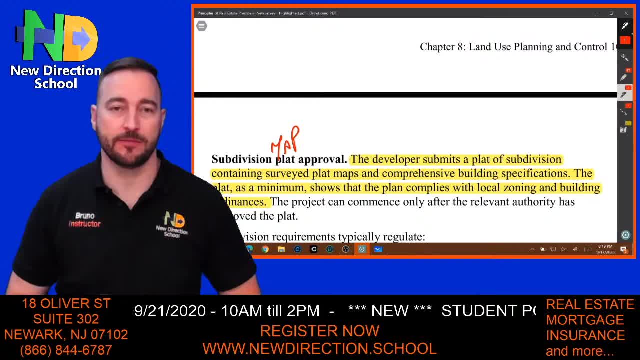 Once it's approved, it's going to be implemented into that master plan. So when I was telling you guys about the stadium, right, the stadium did not pop overnight. Somebody decided to build, presented it to the city of Newark or the city of Harrison or in Brooklyn as an example. 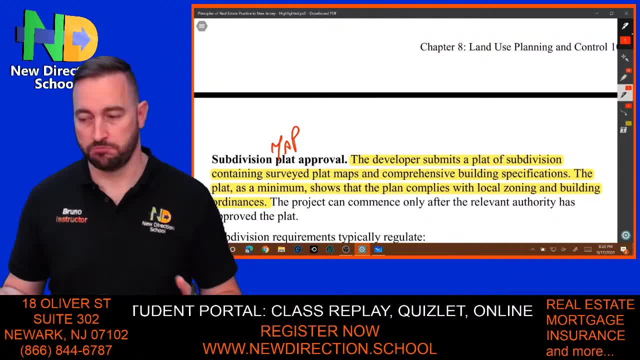 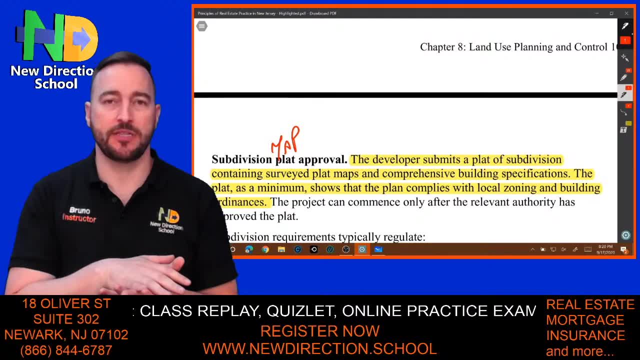 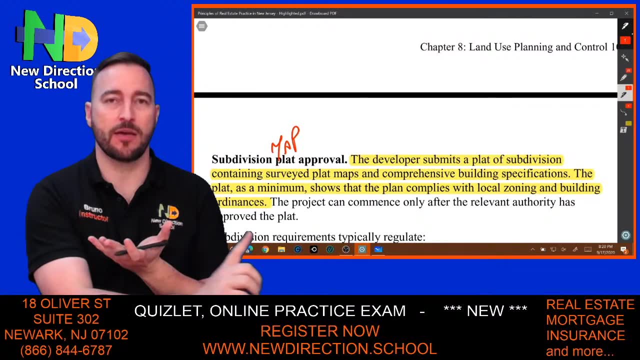 And the city said, okay, it's approved, It's now officially part of the master plan. And guess what happened next Once it became part of master plan, it was approved, all these tall buildings came around right, All these new developments happening. 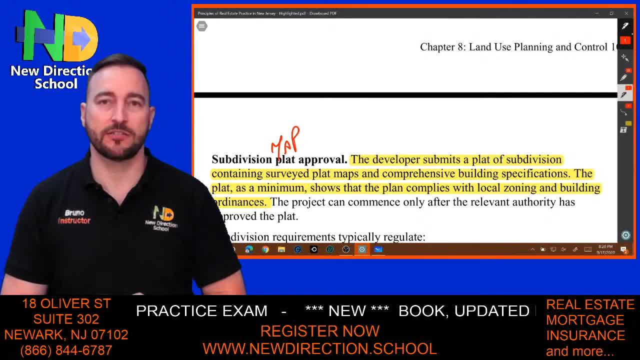 People started buying left and right. You guys understand how this works Once something is approved. that's why you got to keep up to date with these, With the master plan, Once things are approved, you know the new direction of this town. 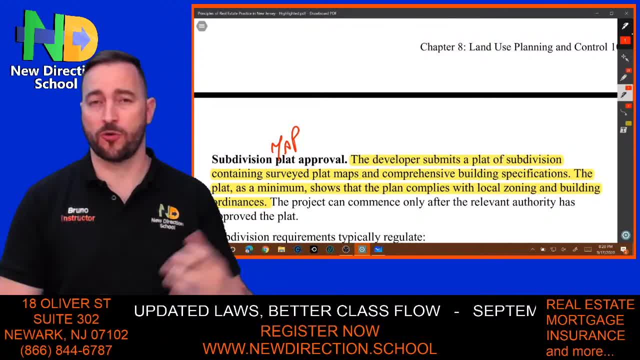 You know that something is going to change- For better, for worse, I don't know- But something else is going to change, right, Harrison, right now, unrecognizable, Like it's a totally different world now, Totally different world. 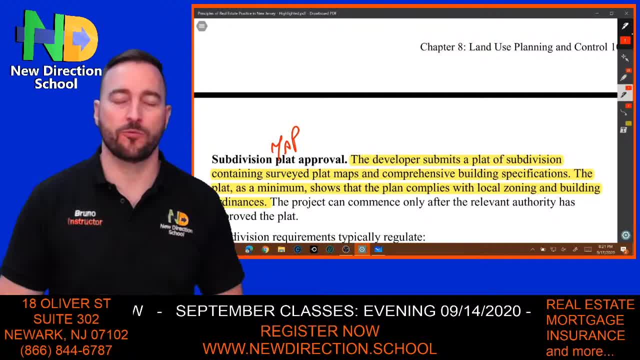 So you get there. There are streets- My partner and I were talking about this the other day- Where you just drive through it And like, wow, they put in more units here. There's like 300 units in one block. 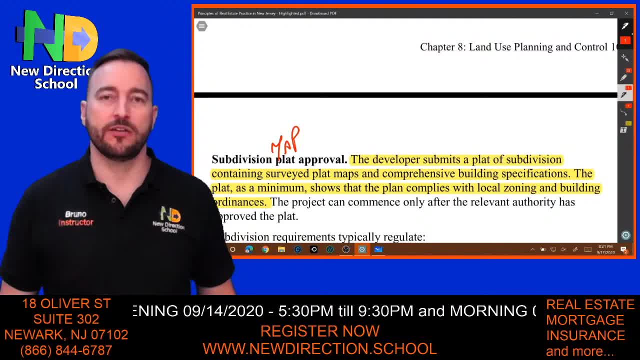 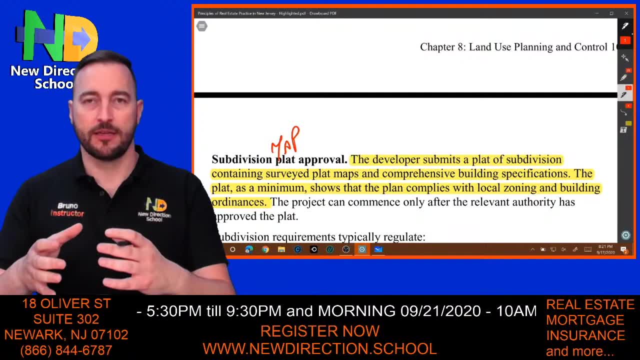 And then there's another 400 units somewhere else In roads that you're thinking you could never be done. Do you guys understand what I'm trying to say? So once something changes in the town, Once one thing is approved, that will change the town. 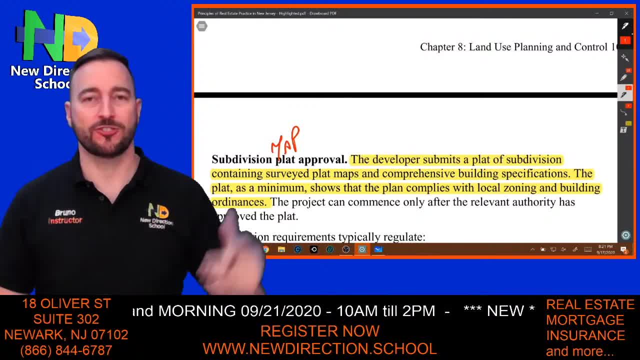 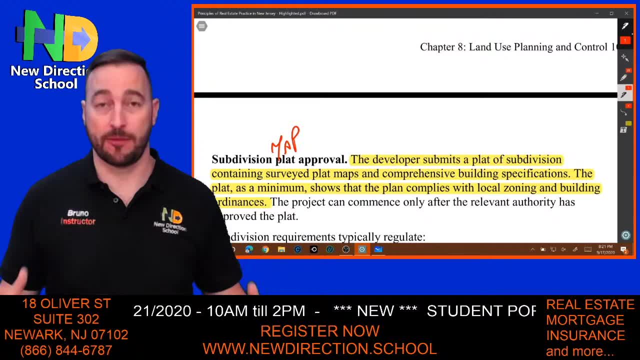 Everything else around will also change. All right, They just tore down the Bear Stadium. There's good stuff that's going to come right next to Route 280. That's why there's a lot of developments happening around Route 280 as well. 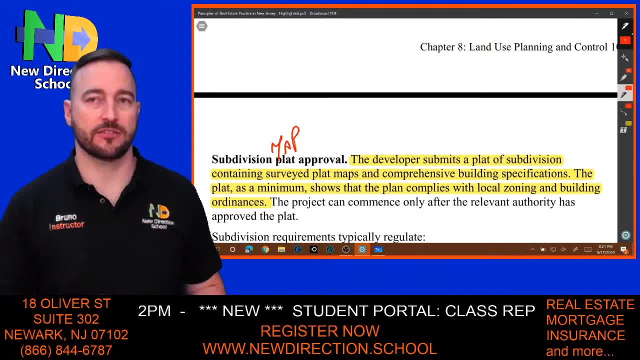 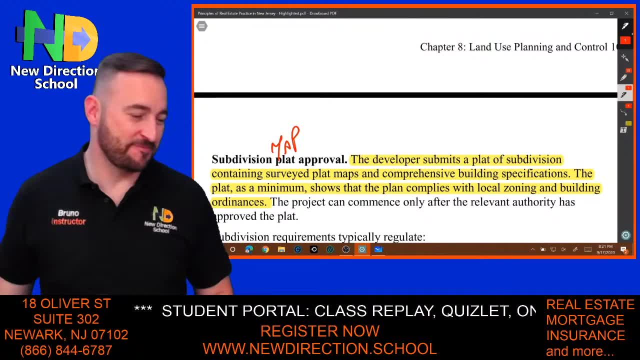 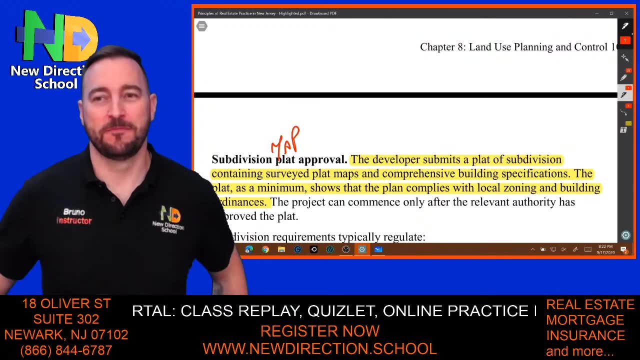 So think about these things. Very important to have access to all this stuff again. So Newark will soon be having a skyline. Let's put it this way: The whole Hudson River is going through a major, major change. So get the master plan. 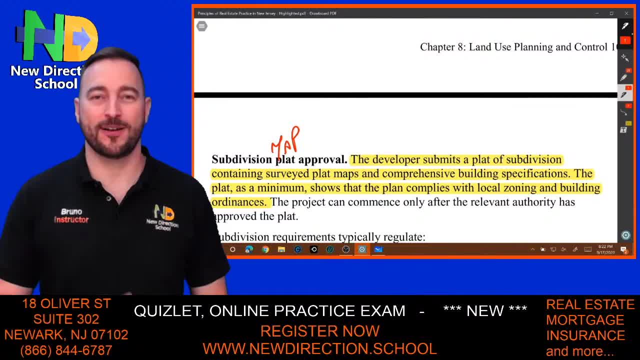 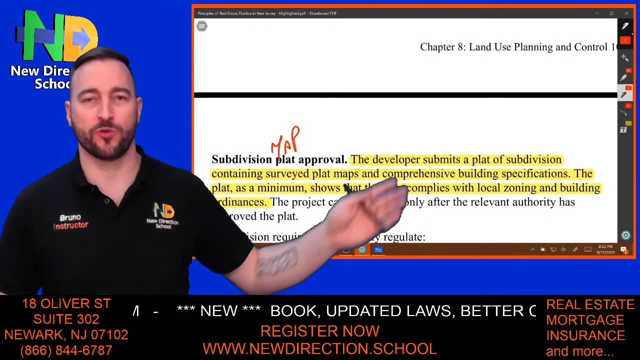 If you have friends with money that want to invest, Newark is always a good investment right now, Harrison, All around Around the Hudson River or around the train stations Along the train stations, All the way to Woodbridge. Train stations are very valuable right now because, just like Stephanie M said yesterday, 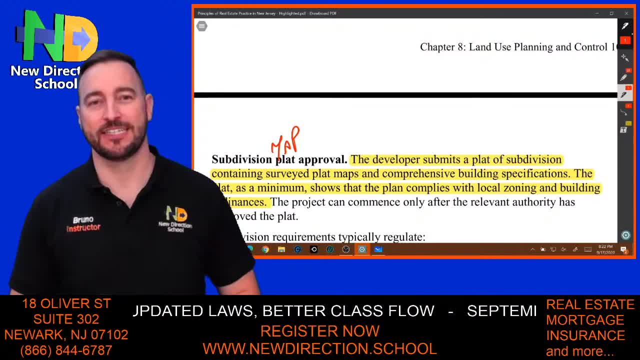 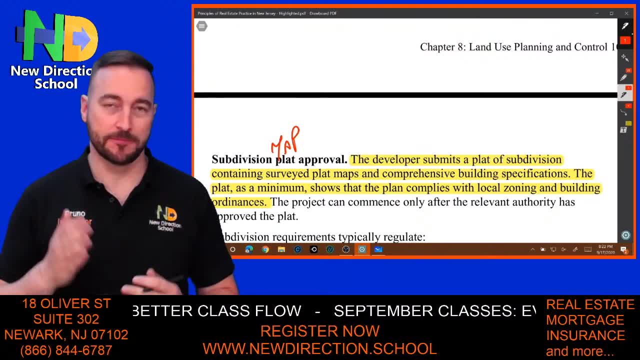 these people from Manhattan are just flowing into New Jersey, So You're going to have a lot of new. So You're going to have a lot of stuff happening: train stations, along the trains, and Hudson Millie says I inspect there. 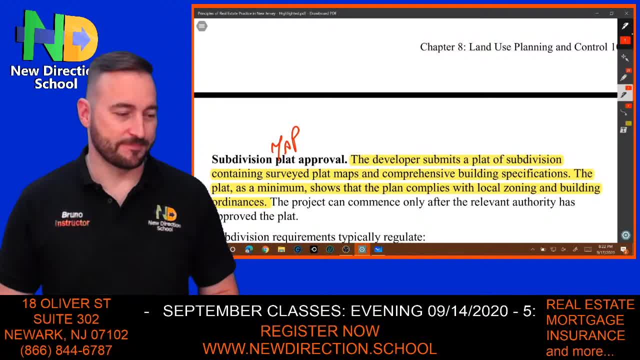 You are right, Hudson, there you go. Erica says Elizabeth- straight train into the city and the ferry. Finally, after 20 years of listening to the whole ferry story since I came to the United States, there's going to be a ferry in Elizabeth to take you straight to New York. 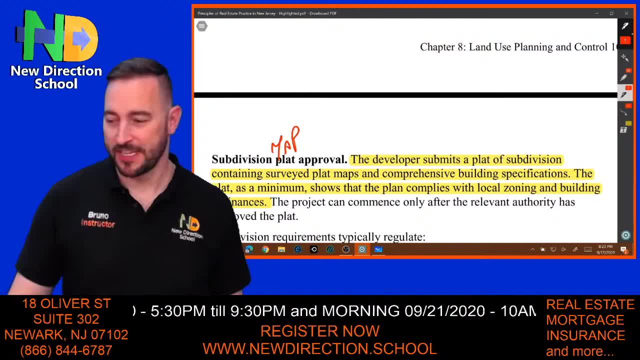 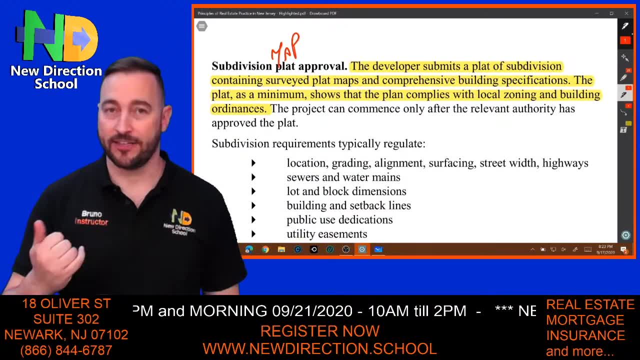 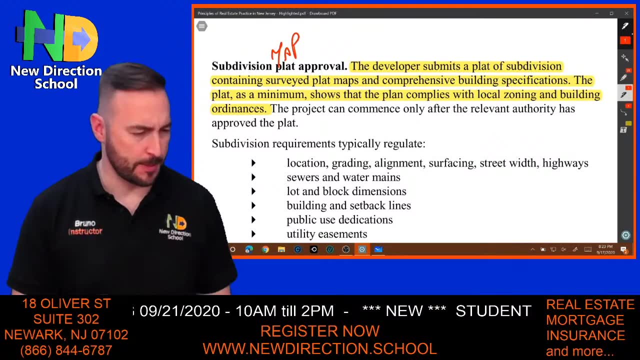 Finally it gets there, Okay. So understanding these things will change your life as an individual, as a professional and to your investors or partners. All right, Mazlima says. all those buildings being built in Linden and railway along the train. 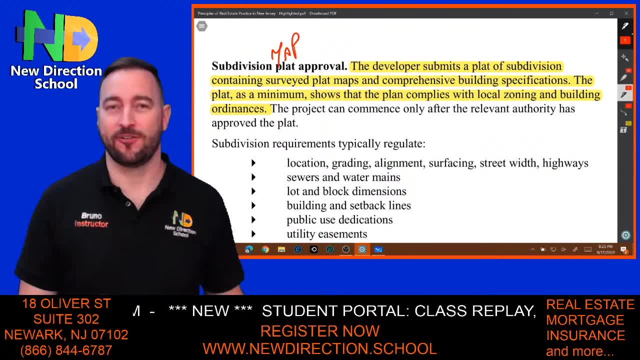 See, I'm not lying. I don't travel that far. I don't go to those areas, I'm Newark, But yeah, I know that this is happening. You got to follow the trends. That's what will make you money. 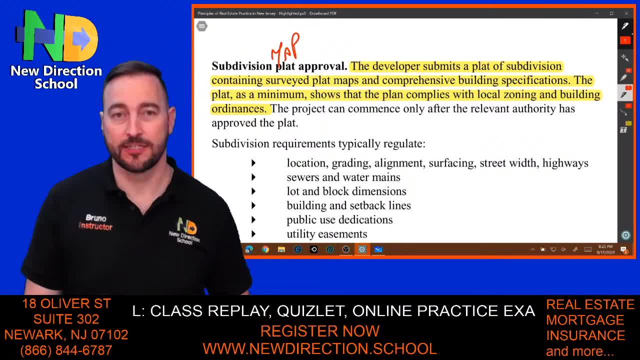 And the people that have money to buy lands near these areas: just land. You don't have to do much. Then the developers come and pay you for that land. Okay, Then comes a Walgreens that says, hey, I'll pay you $20,000 a month for me to build a Walgreens. And you're like: okay, I bought that. I bought the land for like $30,000. But sure, Give it to me. You see what I'm trying to say. All right, So FHA requirements- Real quick. 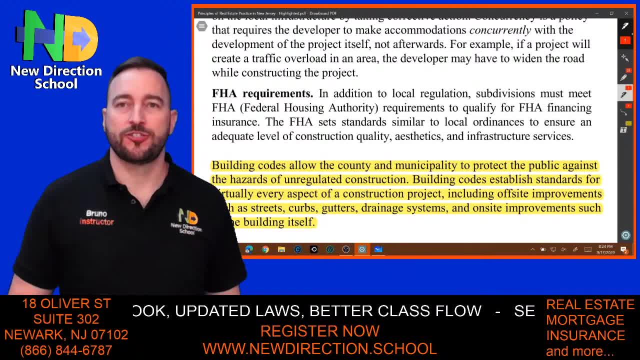 FHA requirements. If you guys know FHA, there's something called FHA loans. We didn't get into mortgages yet, But there's something called FHA loans And FHA loan is a government-sponsored loan. Now the loan comes from Bank of America. 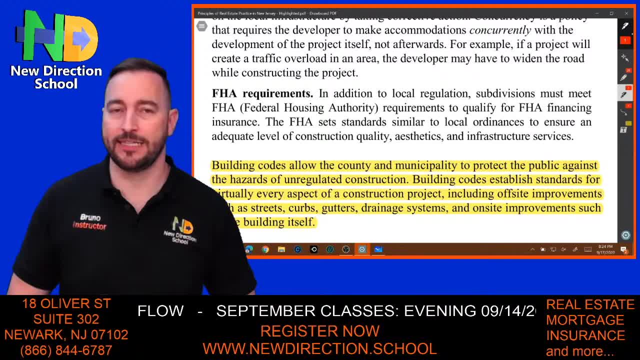 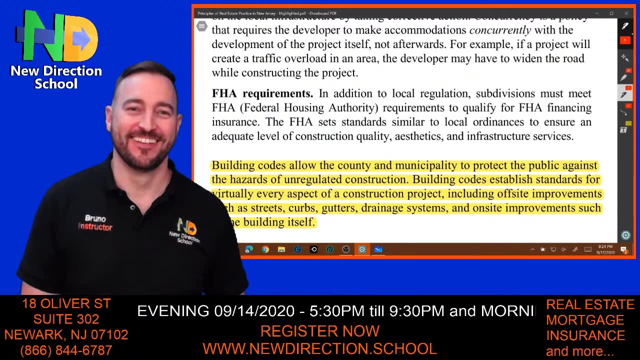 It comes from Chase, It comes from Wells Fargo, It comes from your local lending institution with a sponsorship or insurance by the Federal Housing Authority. Okay, So, Verona, just have him sit down. It's fine, I'll give you a free pass today. 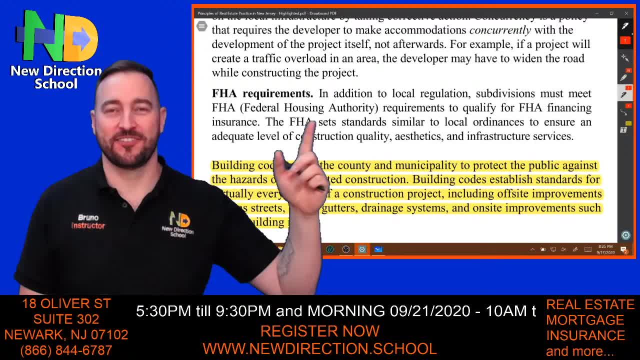 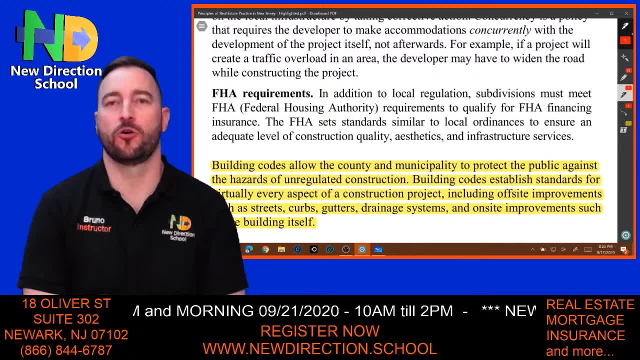 So, like I said, so FHA- Now FHA is not available everywhere. The government will insure the loan, but FHA is not available everywhere, only in certain areas, And for FHA to approve insurance and allow a lender to lend an FHA-approved loan right. 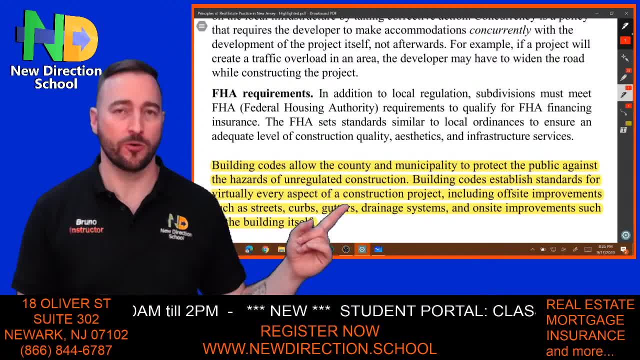 that means that those areas have to follow certain building codes. So FHA is not going to insure the loan if it's not within certain guidelines. Okay, So you have the building codes from the municipality And then you have the building codes from FHA. 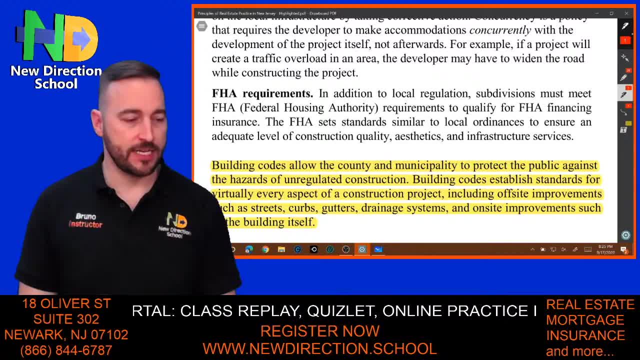 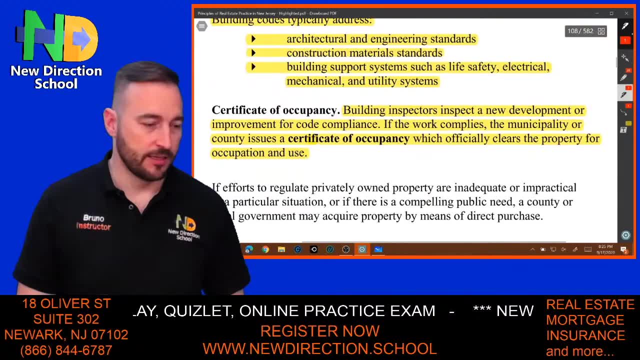 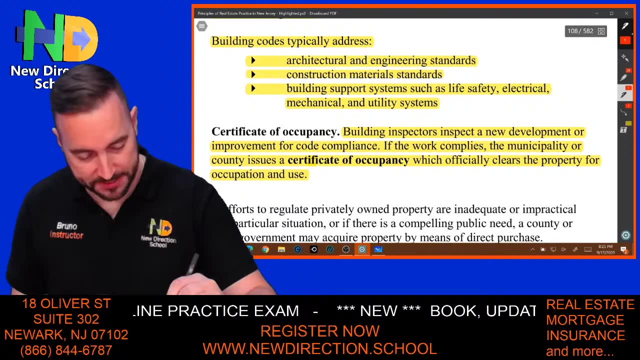 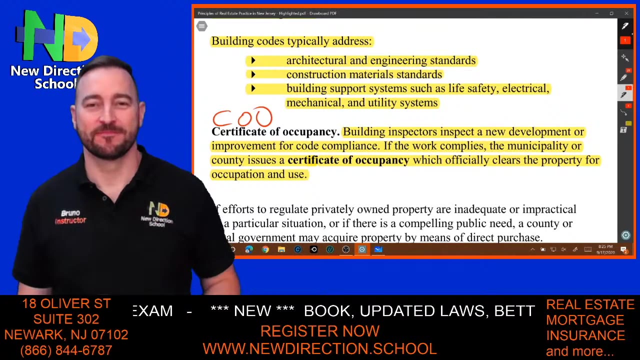 Hopefully they will match and you get the loans approved. That's how we get FHA loans in certain areas. Certificate of occupancy: I think everybody knows what this is, Or, as Stephanie M says, two Right Certificate of occupancy. 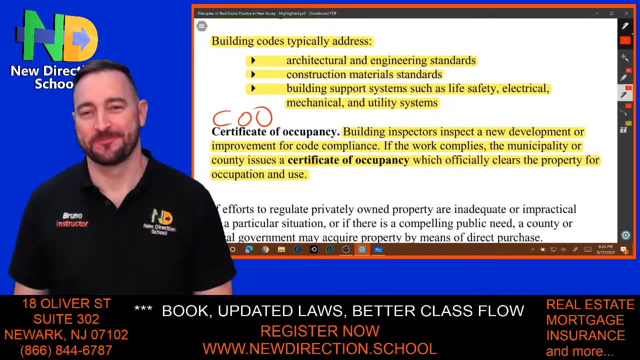 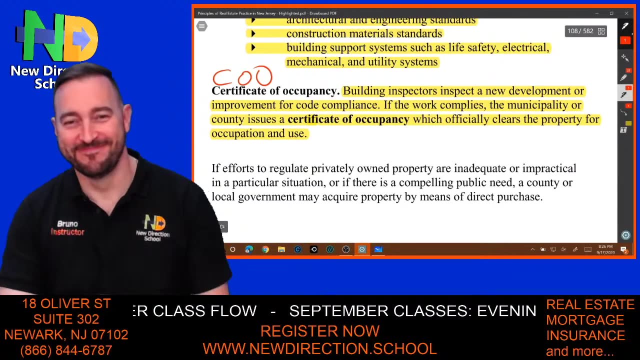 Two, One, Vanessa C in this case, what are you doing? Are you okay, Lol? Yeah, that's what you were saying. Okay, All right. So Vanessa saying lol. So CO or C of O. certificate of occupancy. 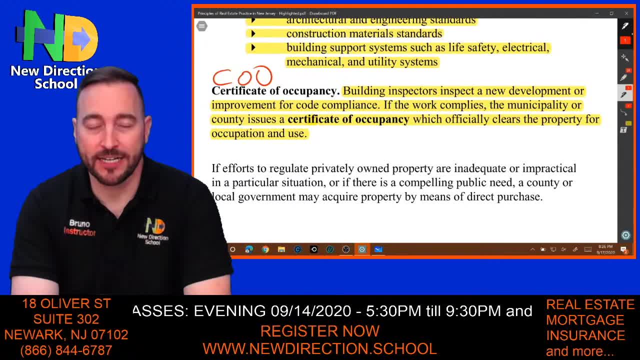 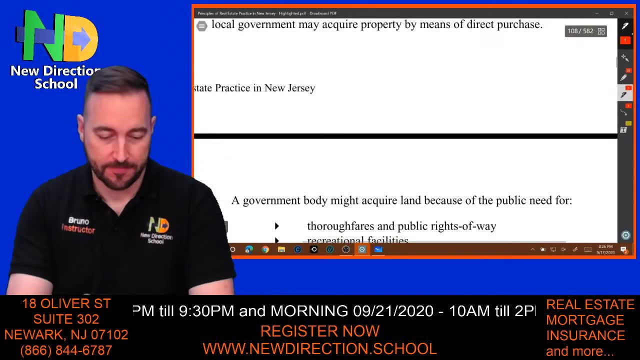 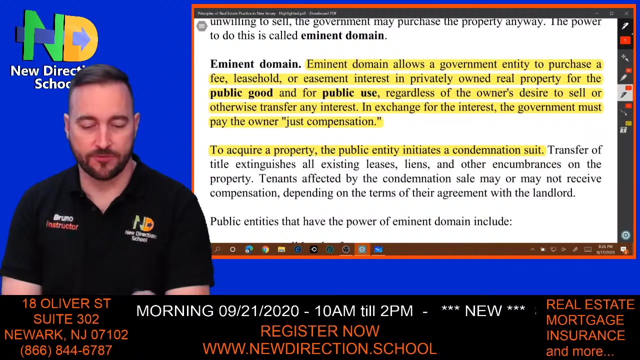 is where the city inspects your property and says it's according to guidelines. right, so we approve you. it's okay for people to now occupy your property. that's what a certificate of occupancy is: simple, straightforward, eminent domain. guys, we already talked about this and we talked about having receiving that just. 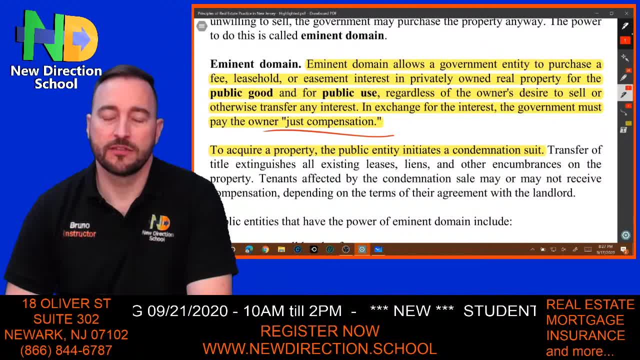 compensation. so the government needs your property for a reason, okay, it has to be for public good or public interest. um, not for their own private. obviously it's a government not for their private use, but something that will benefit the community, and sometimes we're thinking of, uh, schools, right. 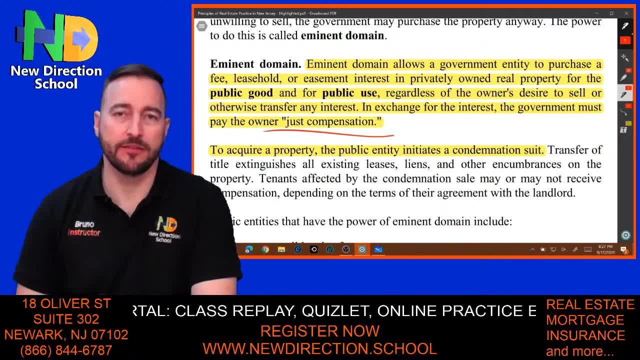 not always. i can acquire your property, let's say on the town. i can acquire your property to build that stadium. now why do we want the stadium again? revenue to the town right. redevelopment of the town. because if a stadium comes, more people visit for whatever reason and they might stay. so now it forces people. 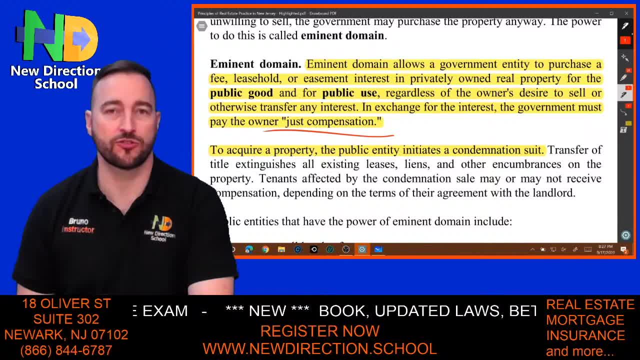 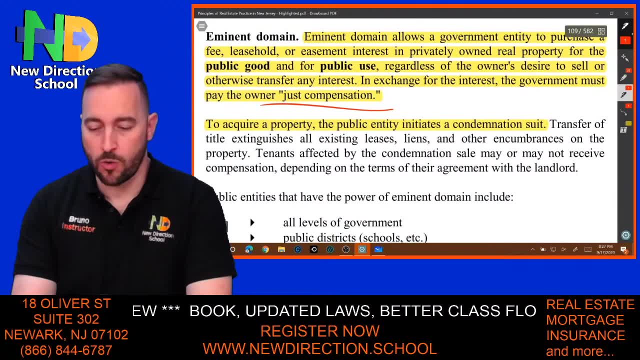 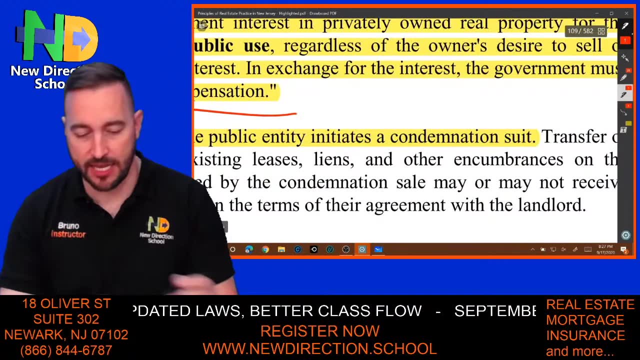 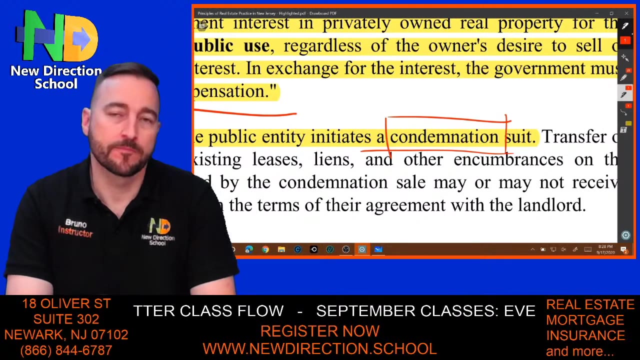 to upgrade, uh, the buildings or newer constructions. you guys got it. everything improves with certain type of things. now, to acquire the property. you need to get used to this term. to acquire the property, the government, the government, the government initiates a condemnation suit. condemnation suit or lawsuit, so they're going to sue you. right, it's not a lawsuit like uh, uh you. 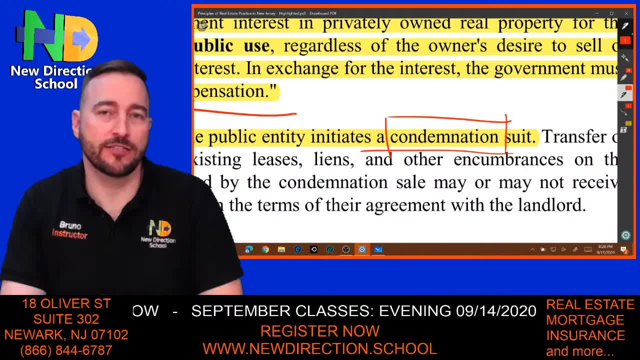 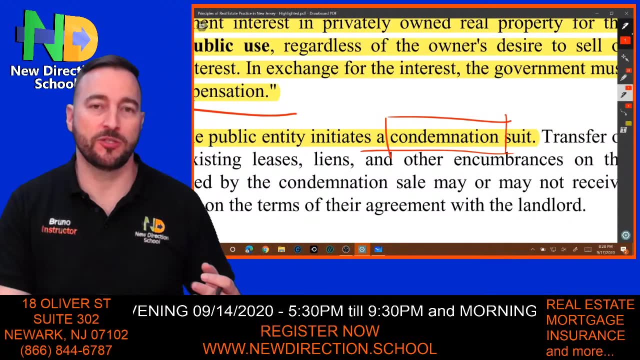 committed a crime. they're going to sue you for their rights to acquire your property for that public use. but why is it called condemnation? condemning something simply means putting an x on top of that property that says it cannot be occupied. it must be torn down. a lot of people think condemnation as hazardous. 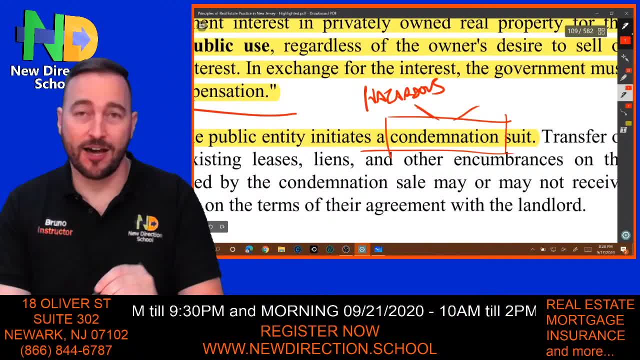 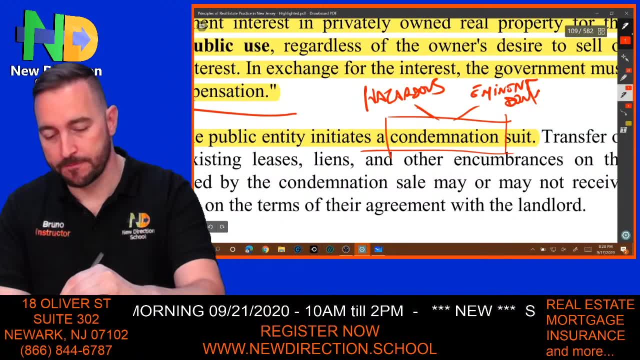 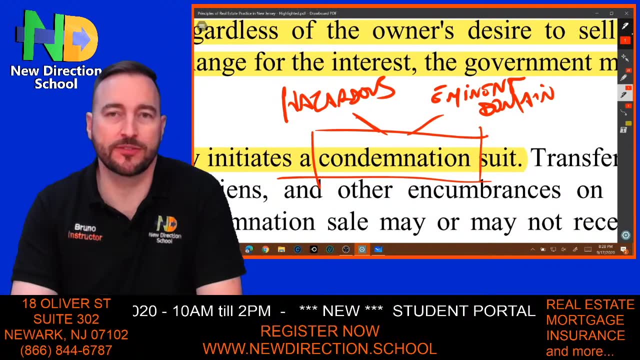 right. a lot of people need to know now that it could be based on eminent domain. so hazardous or eminent domain condemnation is the same. it must be brought down, either because it's in a hazardous condition or because the government needs it. that's where the word kind of 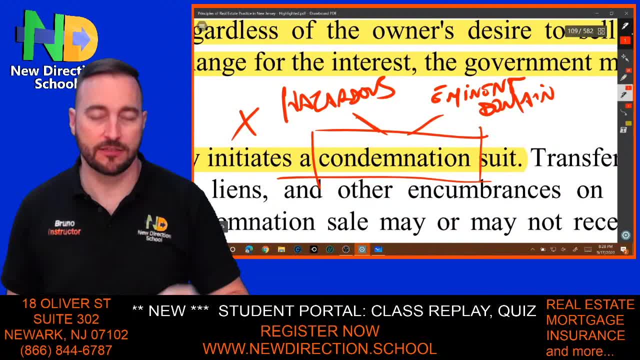 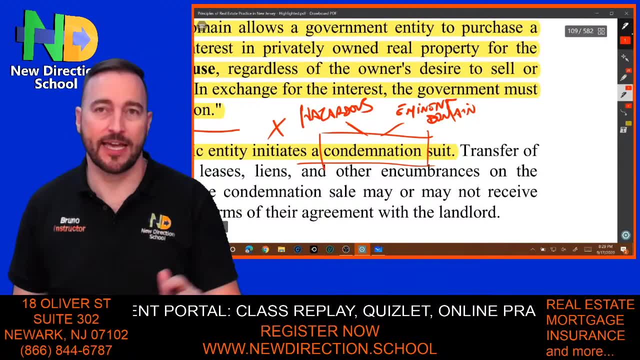 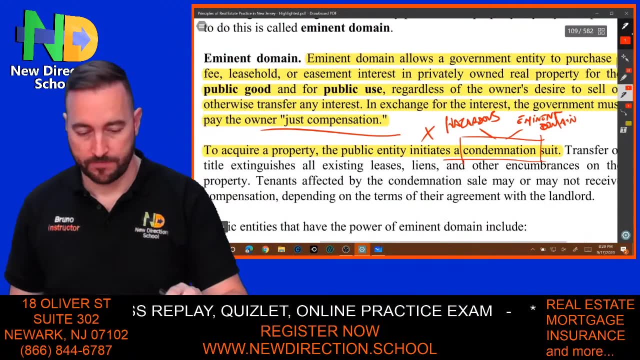 will be is simply an x on top of your property. bring it out, okay. just remember that condemnation suit in this case. it's not hazardous. in this case, government needs it. okay, because i know if you were to see condemnation in the question you'd be like: no, it can't be this. 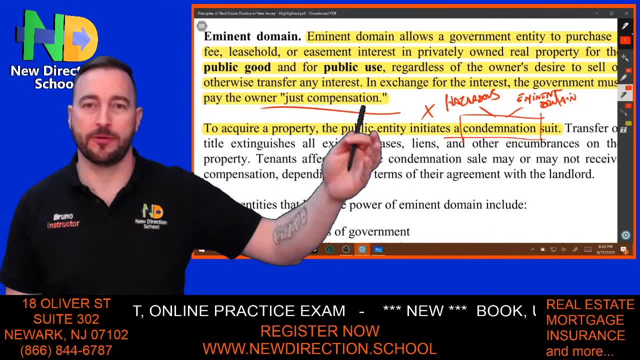 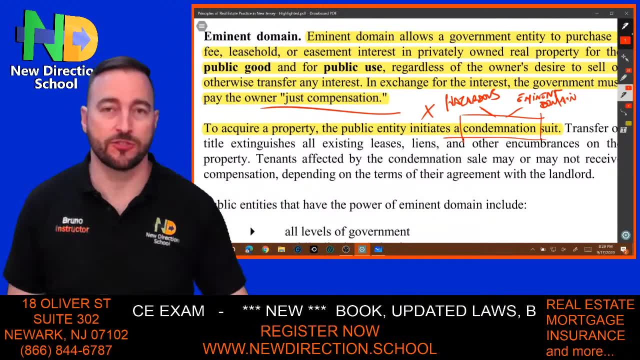 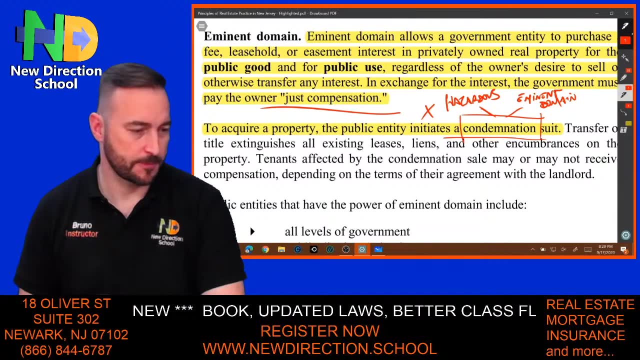 right, doesn't talk about the property being destroyed. why would the government want to take over a property that's destroyed? doesn't make sense, right? so you would completely ignore the answer that says condemnation suit as an option. hey, muslima, you got a question. some of you are way too comfortable. that is no good for you to study, just saying. 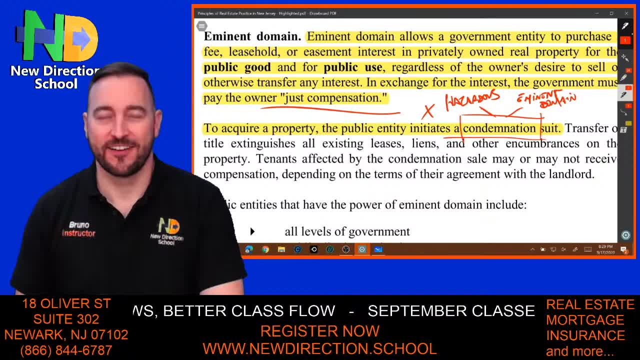 all right. i had this conversation earlier with somebody and i said that i fall asleep just at the cover of a page. but if i'm leaning against the pillow, if i'm leaning against the pillow, i'm gone. all right, muslima, do you always get a payout when the government takes the property? 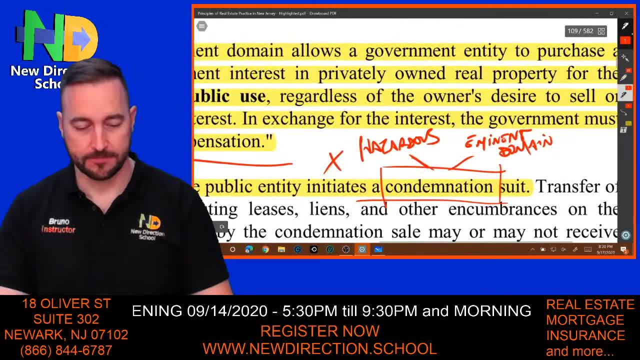 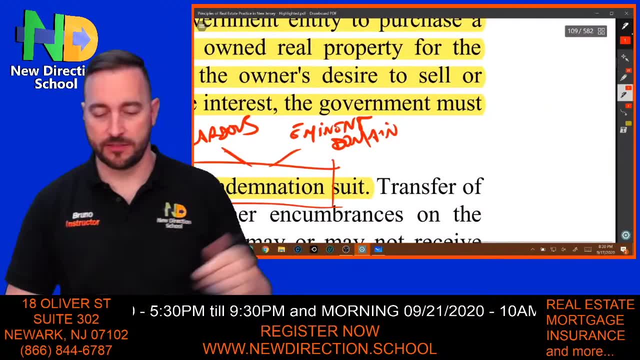 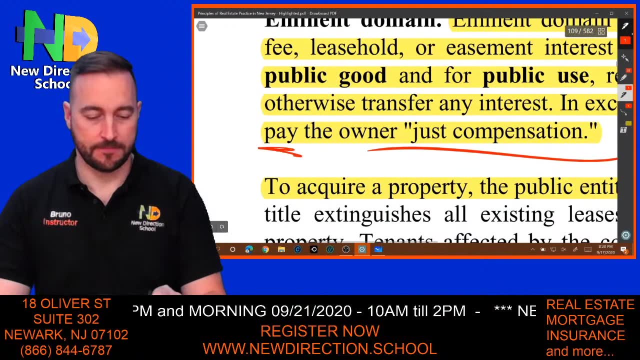 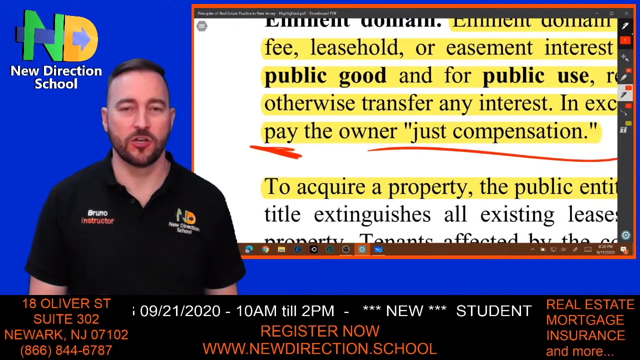 the answer is right here. in exchange for the interest, the government must give you a fair compensation. okay, so they have to give you just compensation, and the word just means fair. okay, even though most of the times is just a little bit, so you can don't complain. 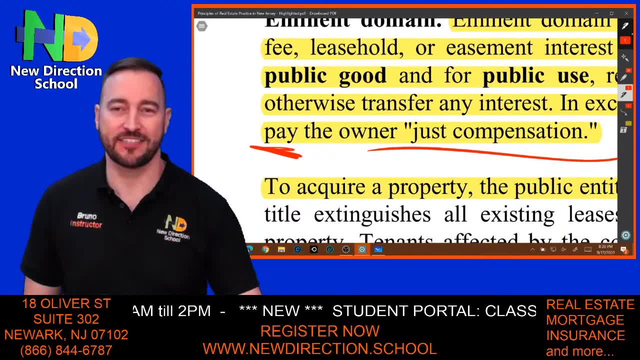 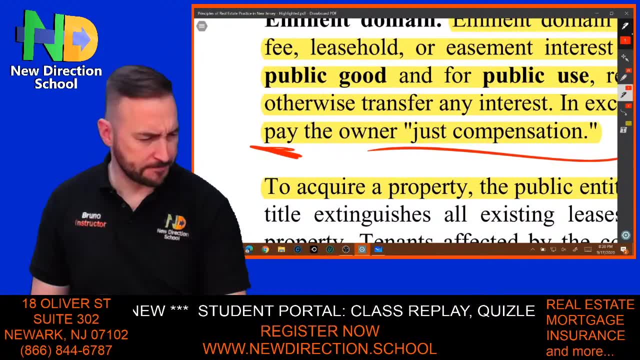 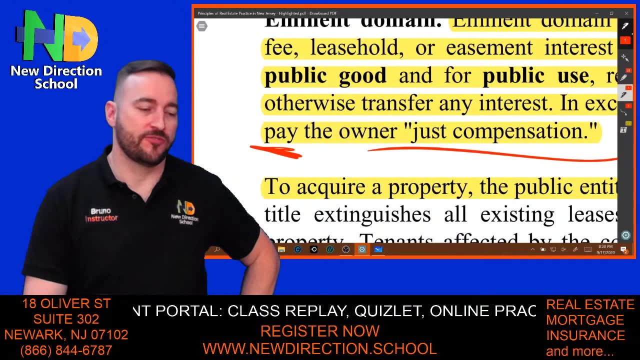 but it means fair compensation. they will assess your property and whatever value they attribute, that's what you're gonna get. it's your loss. everybody got to go. there's a building with 10 tenants. Everybody got to go. The owner of the building gets paid for the building, not for the. 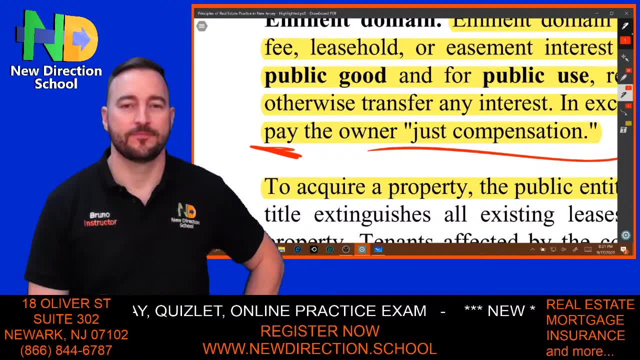 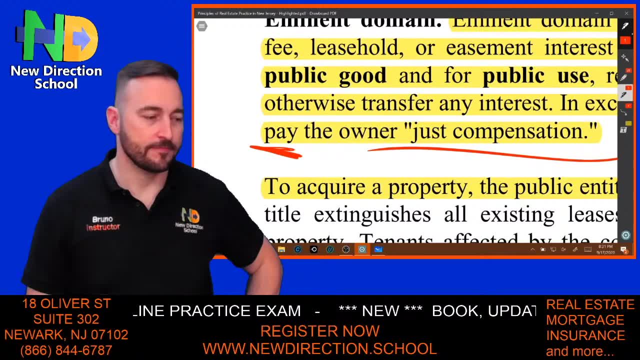 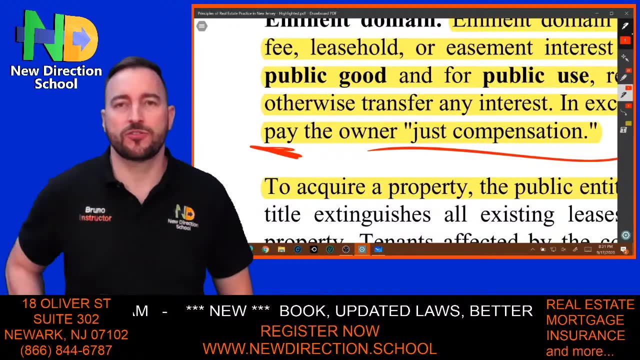 rent loss: Yep, They'll assess the value of the building, as is Yep Businesses. it's the same thing. Do they need to provide housing? No, because you have to think about this. Condemnation suits takes years. It's not something like I've been telling you guys. the whole planning part. 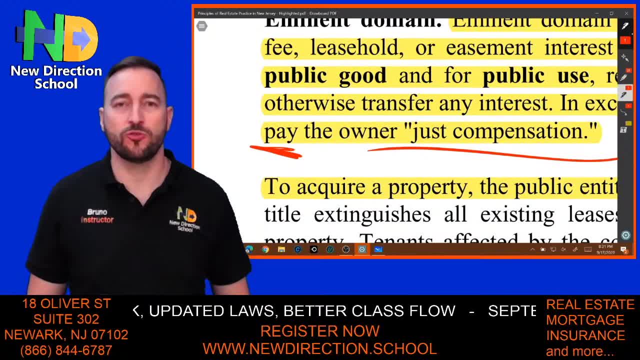 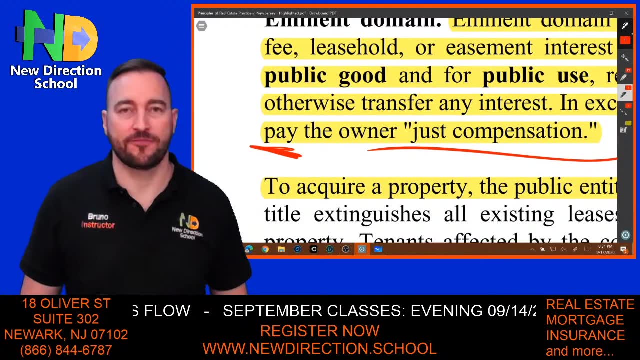 it's not an overnight thing, So they're going to send you a letter and say: hey, two years from now, I need this or I need that from you, So you have enough time to give notice to your tenants that they have to leave. And that's what happened to Harrison Yep. A friend of mine had just bought. 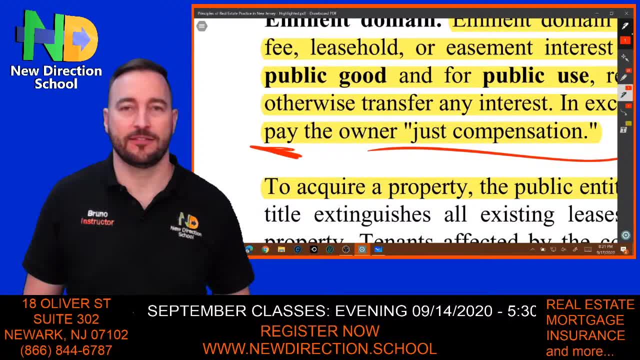 a business in Harrison. The seller knew and the realtor knew about this eminent domain. He bought the business- a bar at the time And I don't know if you guys know, but a business on average takes at least two years before it becomes profitable. 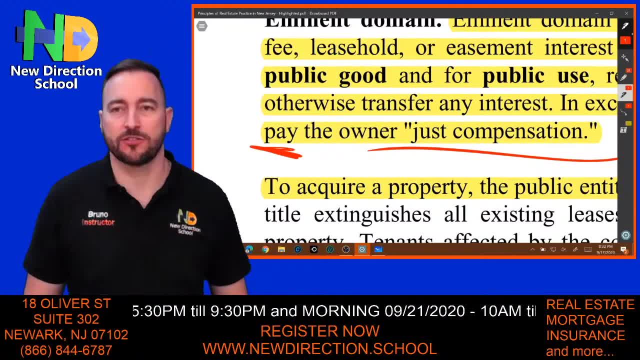 after purchase at least two years. Some could be faster. The majority of them take longer, But his took after two years. he was doing okay but still didn't recover his money. And then all of a sudden, here comes the town and puts a notice on the door that says: 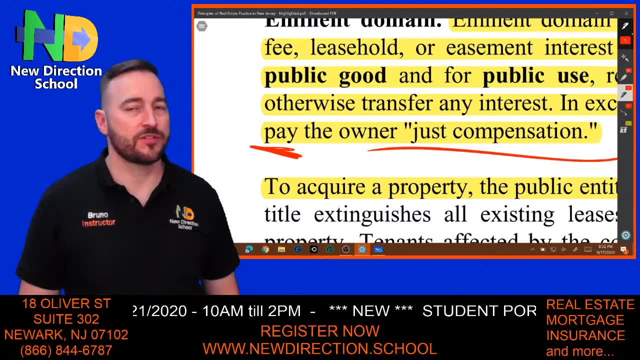 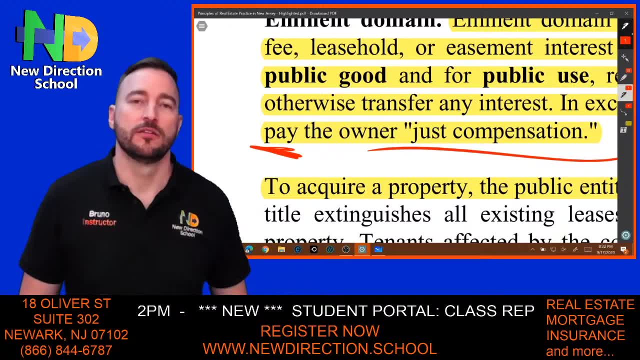 shut down. You got to go Right. This did not happen overnight. The previous owner had been given notice by the town, So the previous owner knew, the realtor knew and they still sold it to him. Right in Harrison A lot of businesses were kicked out. 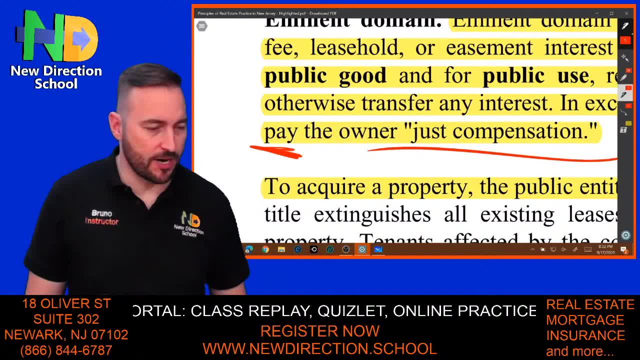 Verona says they did that to my friend. They paid him to give up their property to build a school on Walnut Street. You need storage, Yep, That's what it is. On South 11th, 11th here in Newark, they paid five properties to get out to build a school. 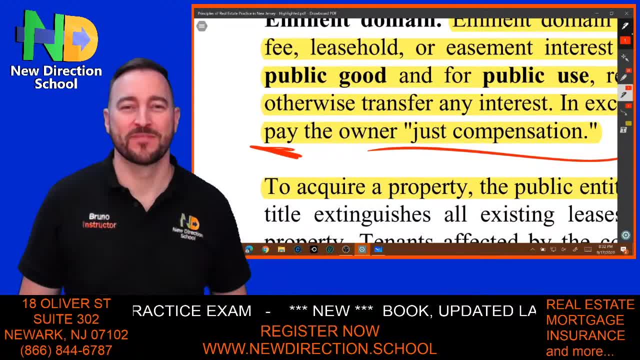 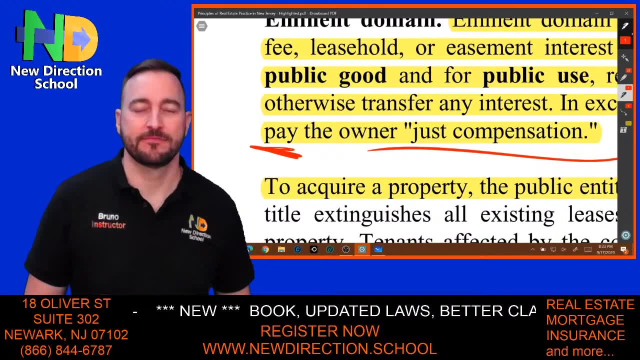 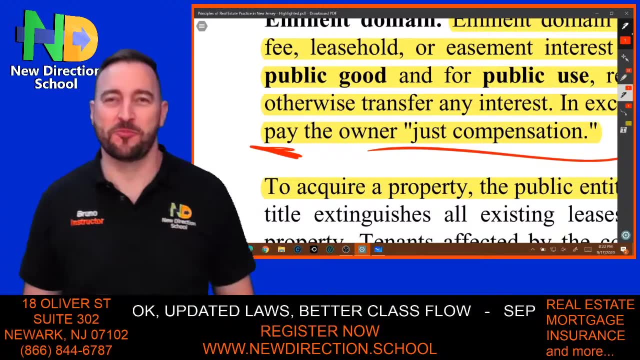 We're still waiting on that school. This was in 2007,, I think it was Something like that. 13 years later, the school is still not there. But yeah, But like I told you, they give you plenty of time to do something. 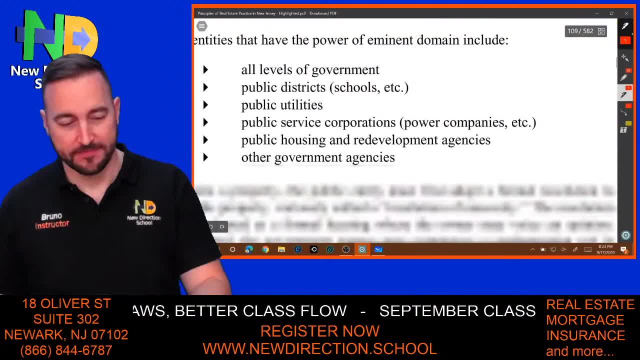 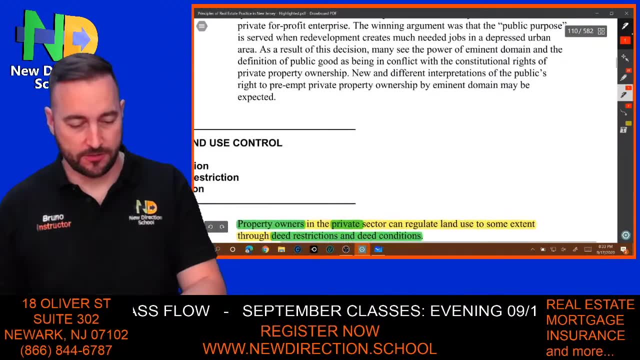 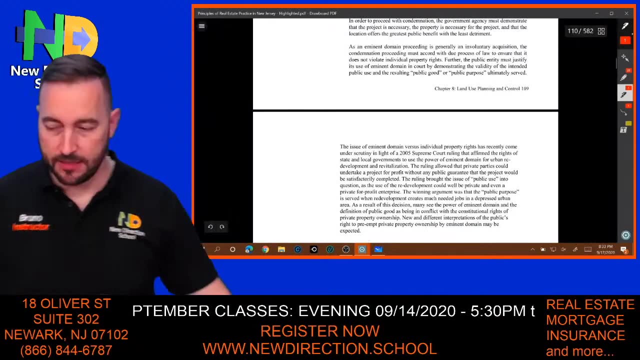 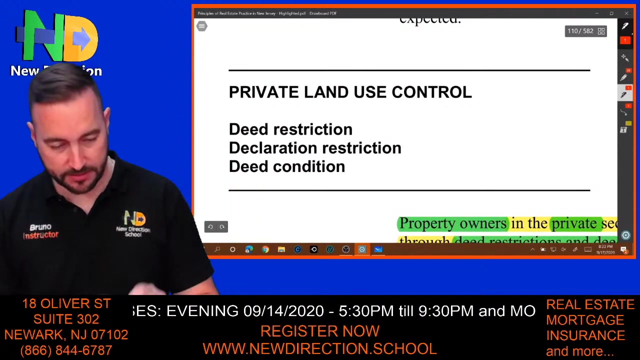 All right. Next, Covered all this, You can go all the way to Supreme Court. All right, Cool. So before we get to private, we're going to go to what Laura said before. All right, But before we get to this, let's go here. 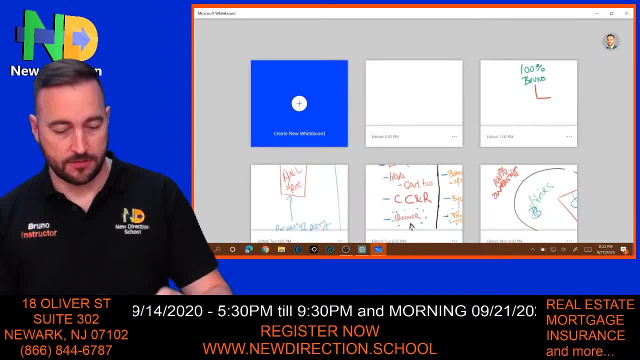 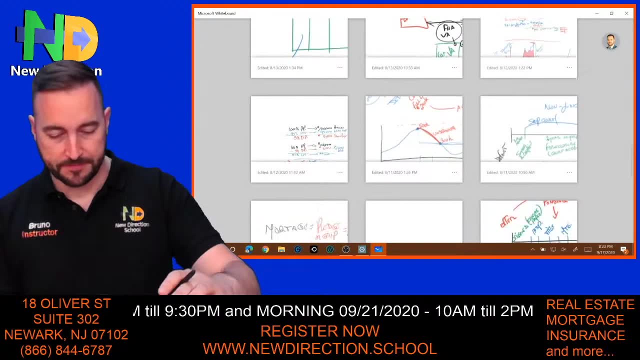 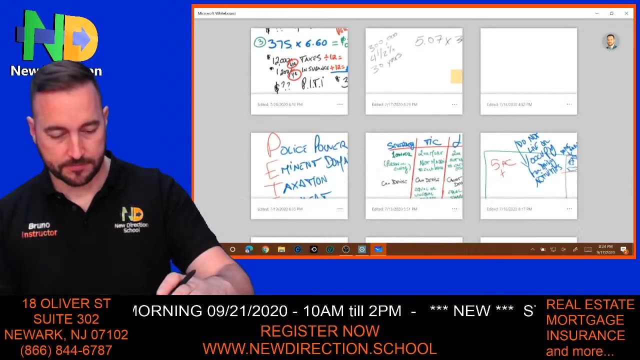 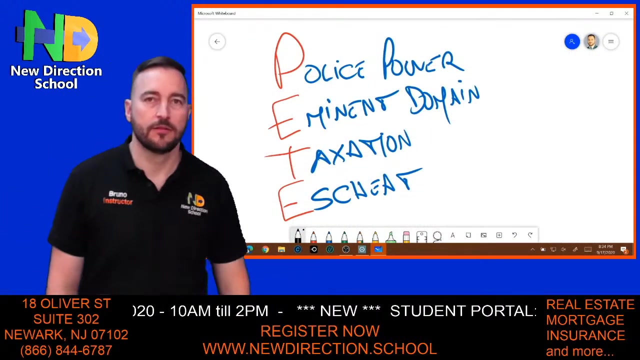 And we talked about. We talked about public land use controls. That's what we were talking about. Eminent domain and all that good stuff. All right, Police power, And here we go. These are the powers Pete. Okay, The government powers are Pete. What does that mean? 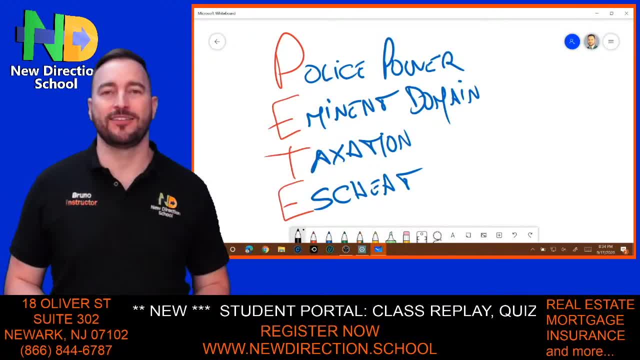 Police power, set of rules and regulations. Ambitious domain is the right that the government has to take over privately owned property Taxation. you guys know that you get taxed And this cheat: if you don't claim the property, the government takes the property. 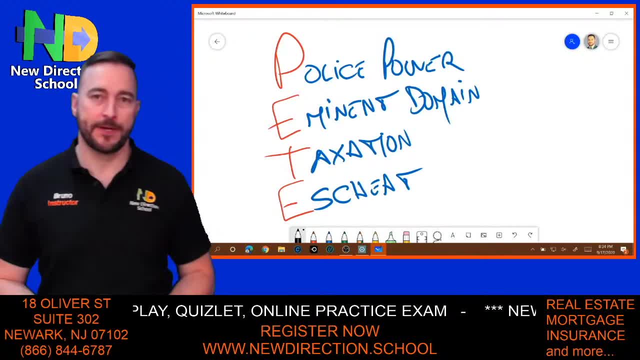 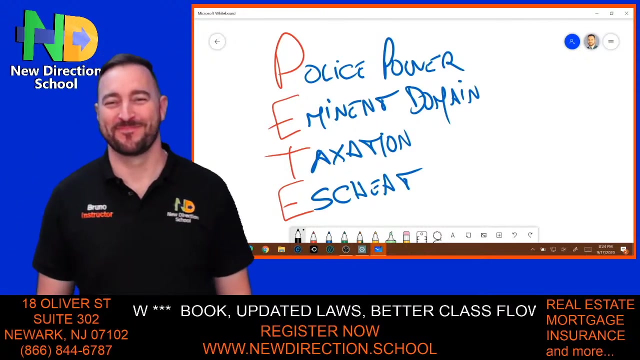 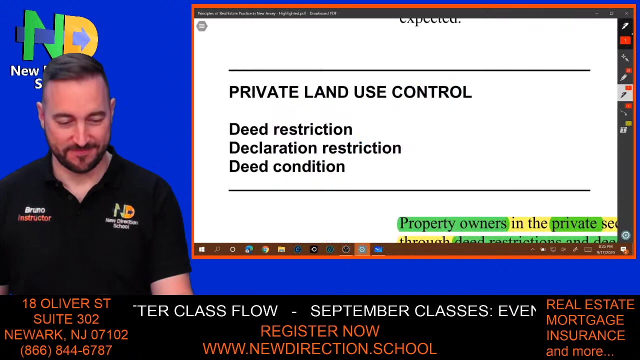 That's when you die without a will. And another 30, and now we're done. Okay, everybody wrote this down. We're good, Great. We're going to talk about private land use controls. You guys should know this by now. 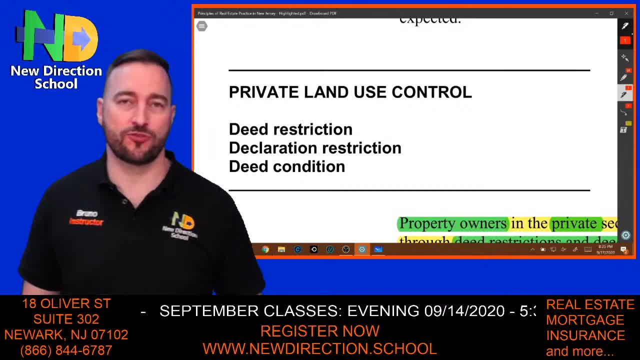 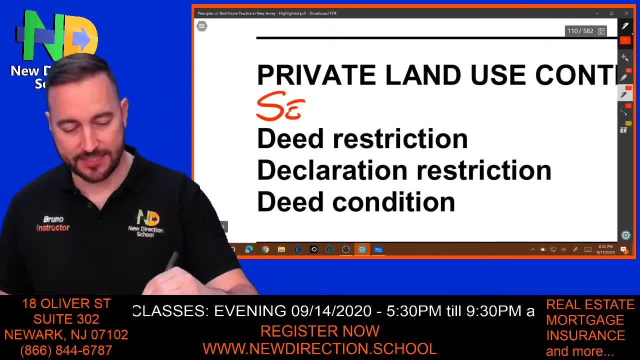 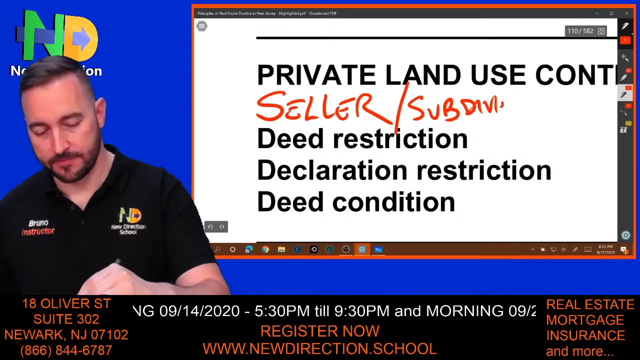 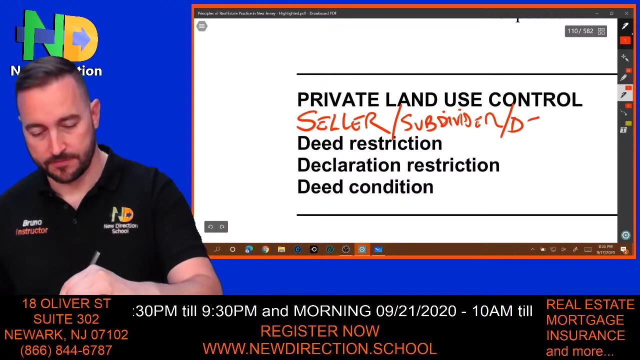 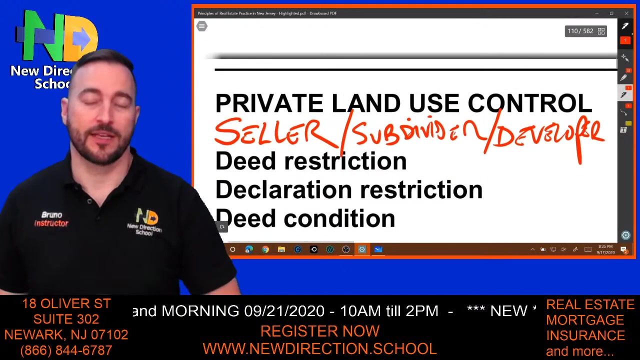 When I talk about private land use controls, it's not just about private land use controls, It's a deed restriction, Okay. So if it's private, it's seller or sub-divider or developer restrictions. In any event, it's the person that. 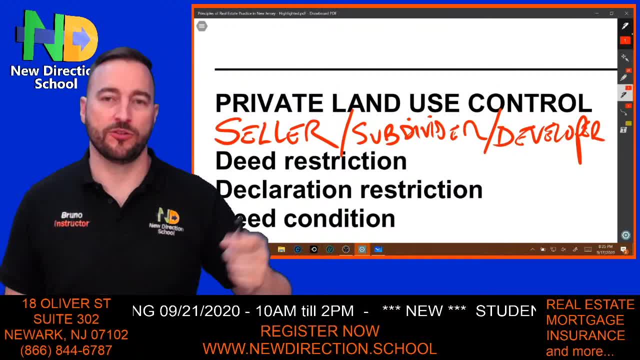 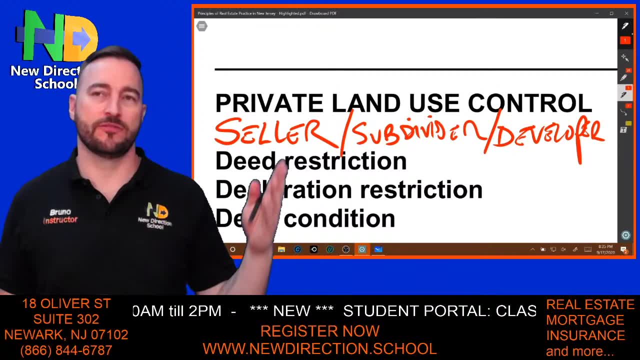 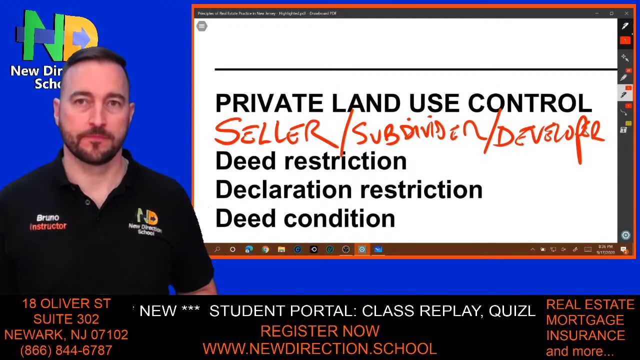 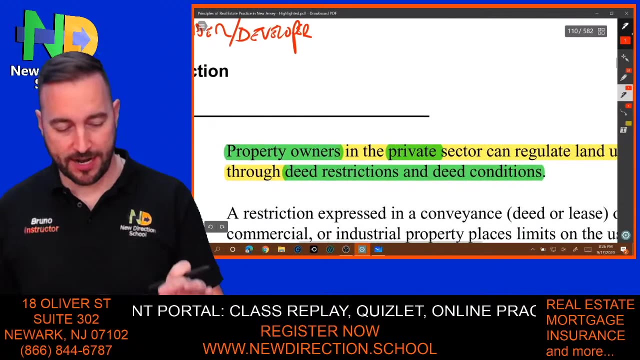 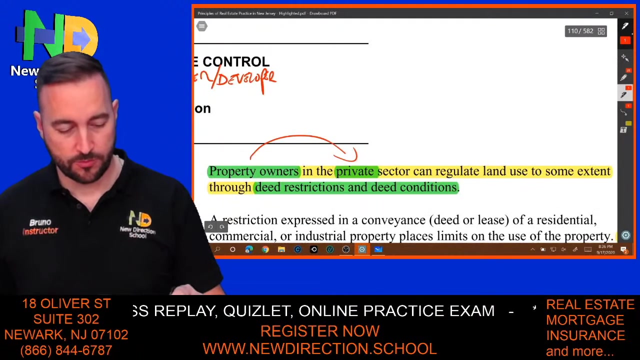 That currently controls the property that privately puts a restriction on you. Okay, So private land use control seller, sub-divider or developer. Okay So property owners in the private sector can regulate the land use to some extent. So property owners private right. 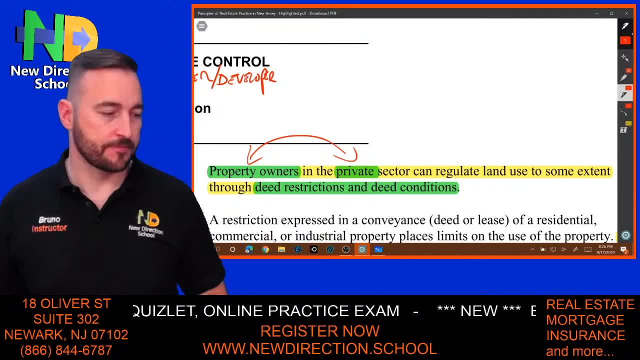 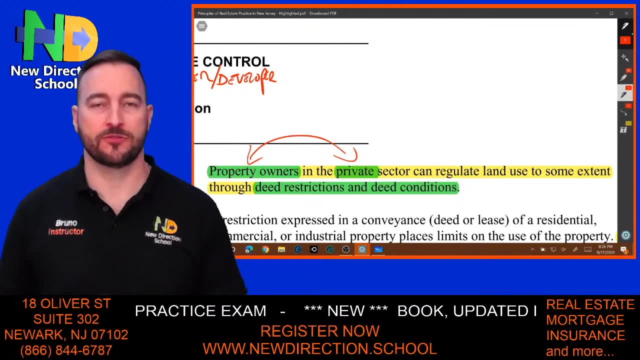 And they do so through deed restrictions, through deed restrictions and deed conditions. So again, guys, I sold the property to David to use it as a hospital. as long as he uses it as a hospital, It's his. The moment he screws up and does something else, like office building. 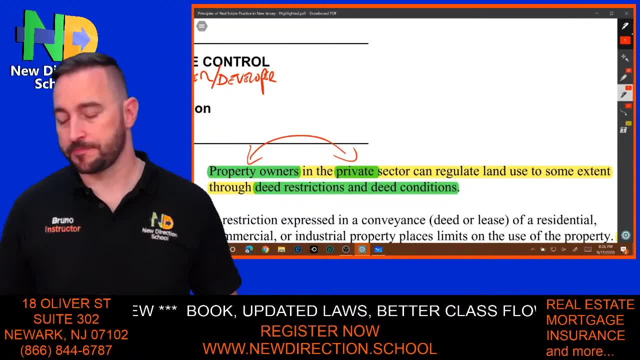 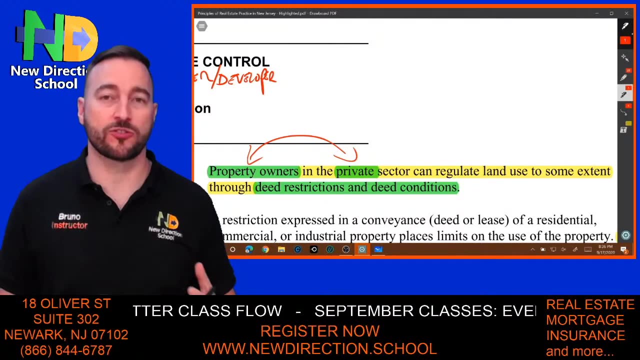 then it reverts back to me, right? If in a homeowners association scenario, the sub-divider and the developer or an order developer said the property has to have these characteristics, So there's something called master deed. If you guys remember this, we talked about master deed. 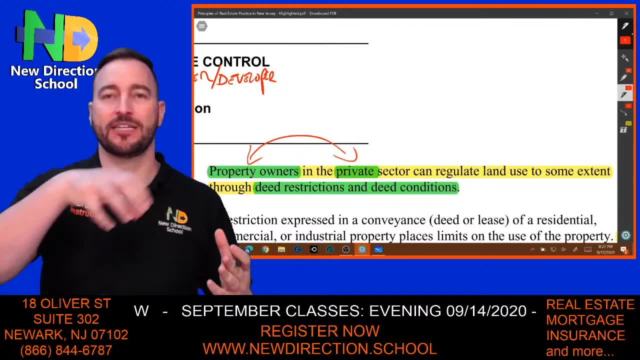 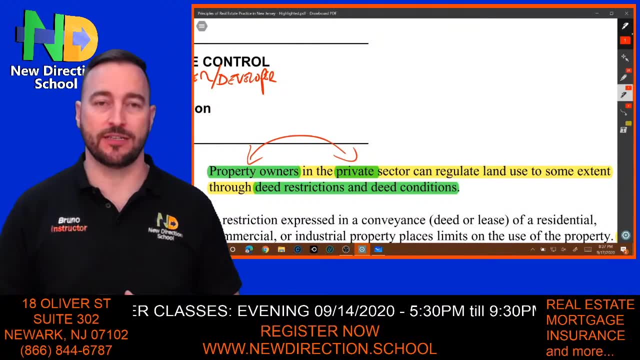 It's the one that regulates the whole land, And then every property that's on it must abide by whatever the master deed says. So if you change the structure that was intended for that subdivision, you could lose your property. Okay, So these are private. 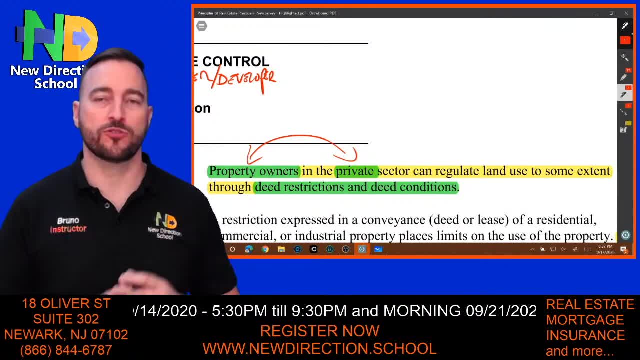 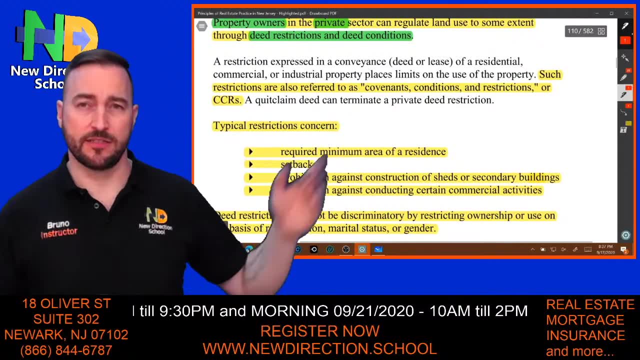 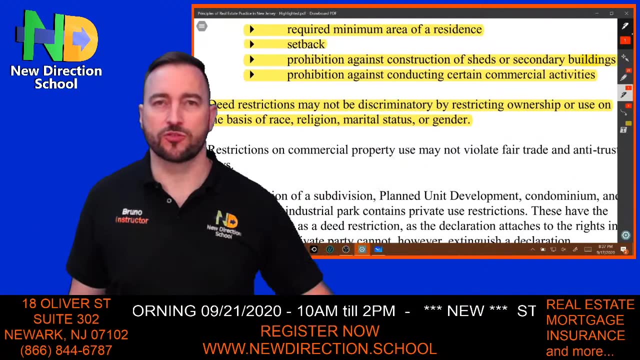 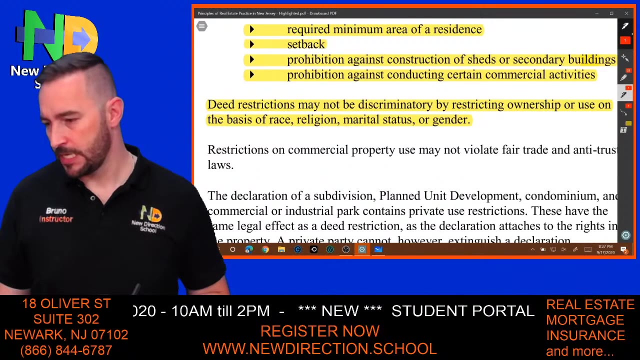 Private restrictions, Therefore, property owners or controlling parties. Okay, We just talked about this, The CC, and ours restrictions. Now these restrictions. we'll talk about discrimination, different chapter, These restrictions. Laura says my mic has static. Does my mic have static, guys? 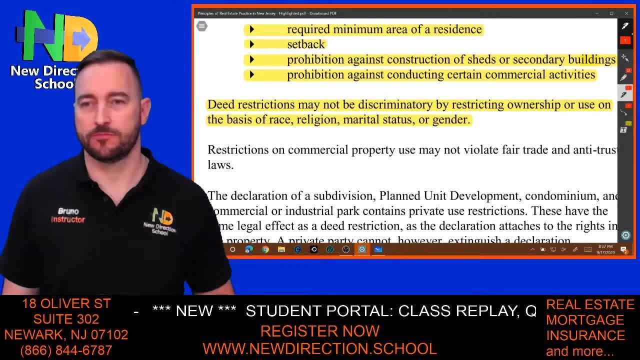 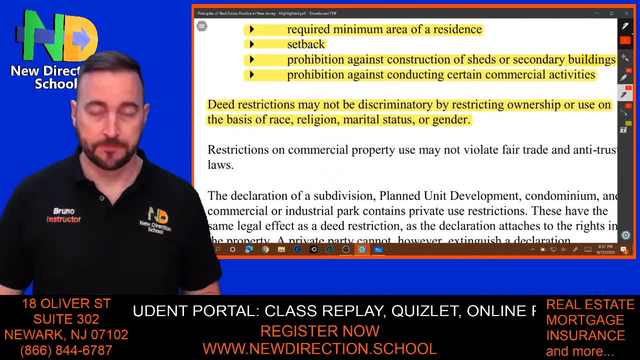 Is it staticky? No, Laura, if you can hear me, they are saying no, So it might be something with YouTube. Okay, So these restrictions may not indiscriminately, may not discriminatory, but we cannot say, hey, I'm going to sell the property to you. 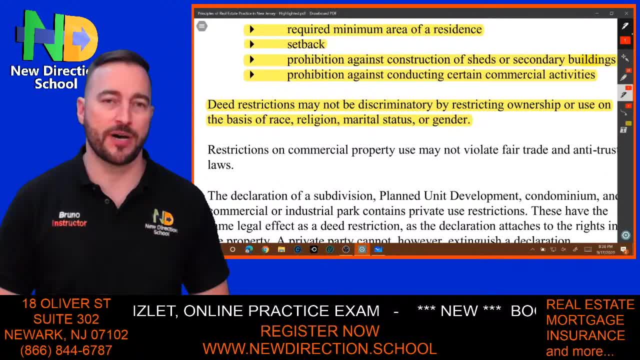 As long as no green people ever occupy or buy this property, And I put a restriction like that? No, because that's against public policy. We cannot discriminate based on color, based on race, based on gender, based on religion, based on national origin. 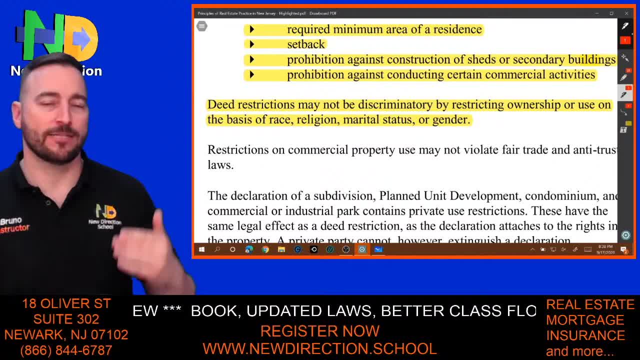 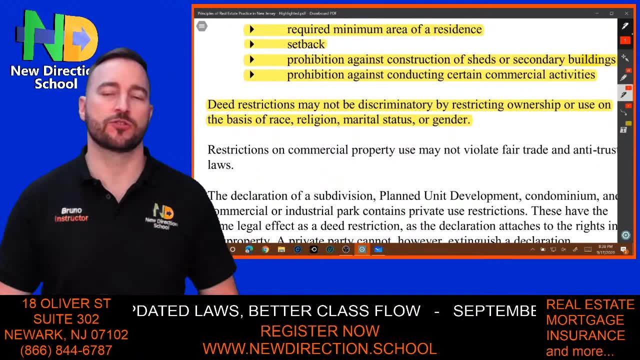 We're going to learn about all this stuff, So we can put a restriction. I can put this restriction there, But is it going to be valid? No, because it's discrimination. Okay, So in the past, a lot of people could do that. 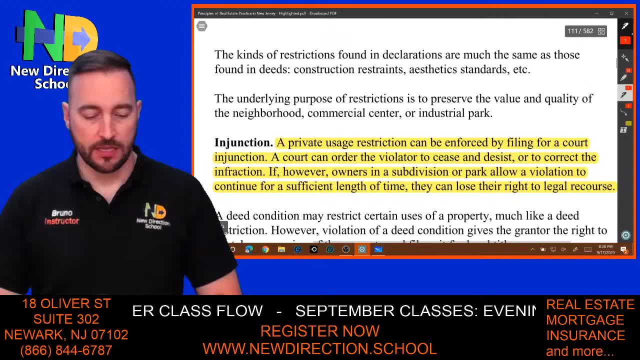 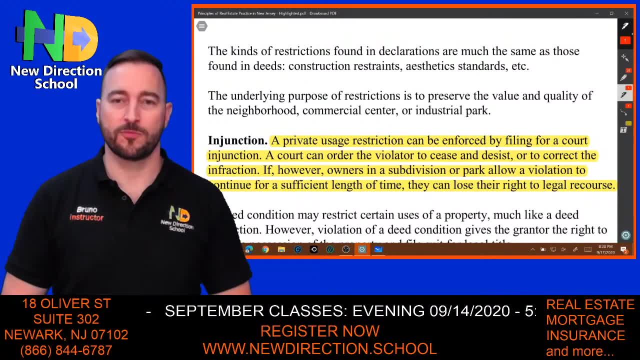 An injunction. And, guys, the reason why I'm skipping a lot of stuff is because already covered through my extensive speaking. So right now we're just going straight to the point with certain things. So, injunction An injunction is an order by a court. 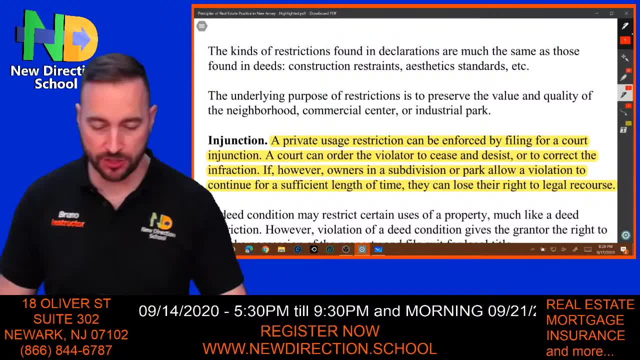 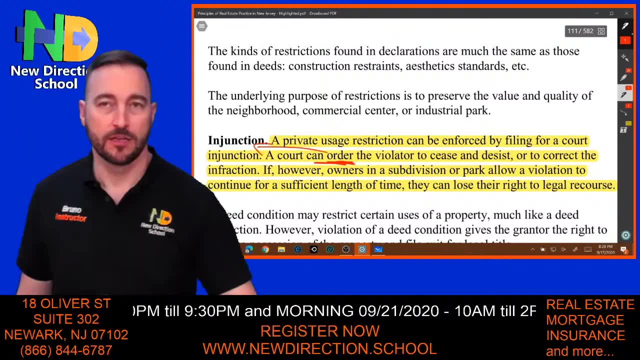 Is the court telling you to do or stop doing something. So injunction means order by the judge. So that's what an injunction is: It's an order by the judge to tell you to do or stop doing something. So they're forcing you. the judge or the court is forcing you to correct the issue. 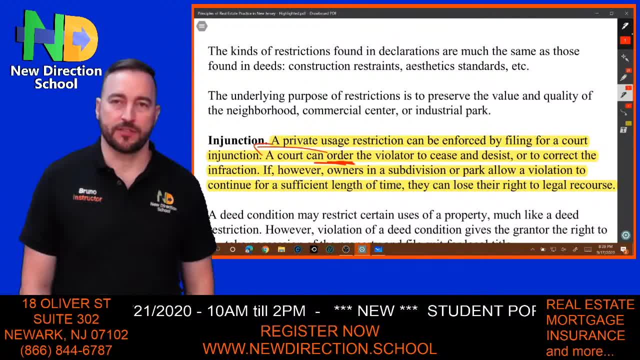 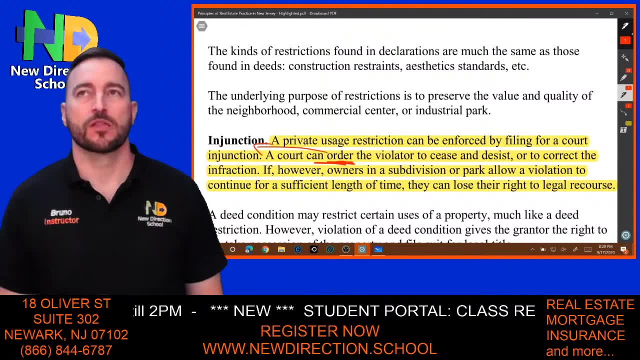 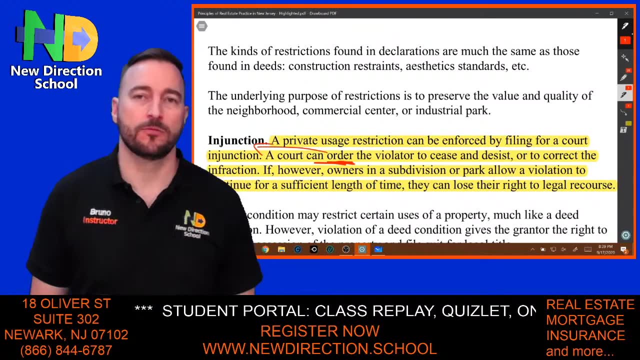 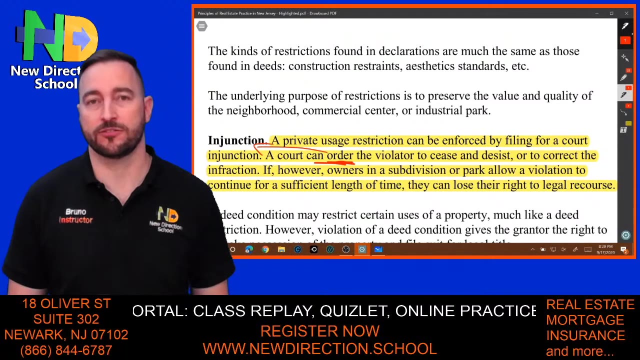 Okay, For instance, if you alter, if you alter the subdivision, let's say subdivision says the lots here have to be two acres And you divide that lot into two, then guess what? You're violating what the subdivision rules and regulations were according to the master deeds right. 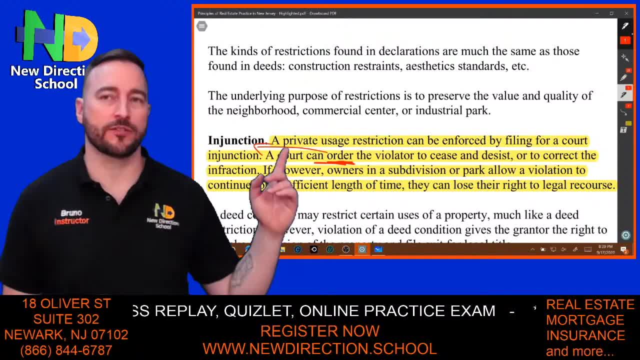 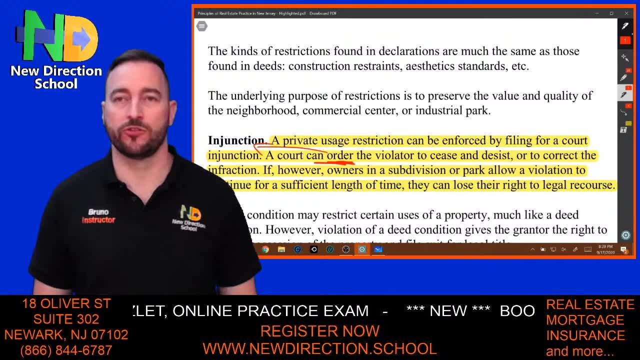 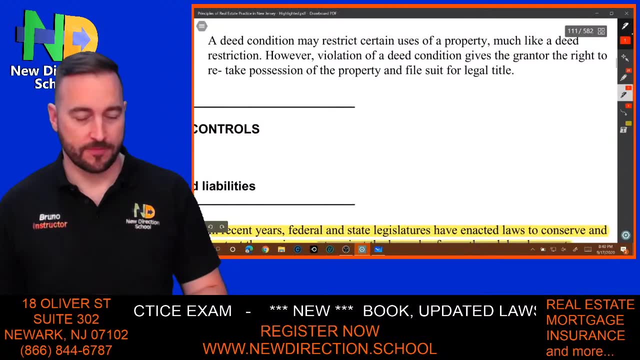 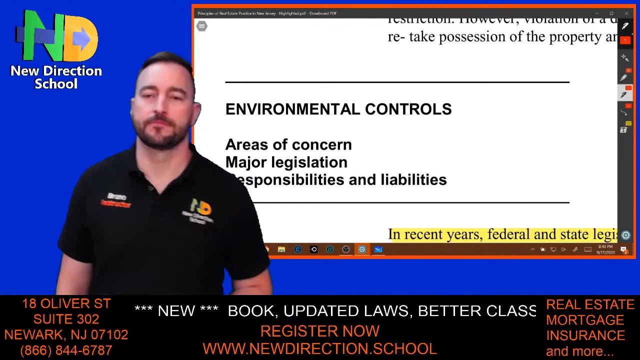 The neighbors can enforce it by taking you to court And then the court says: well, it was two acres, so you got to restore it to two acres. Simple, Very, very simple Environmental controls. So these regulations are based on stuff that affects what 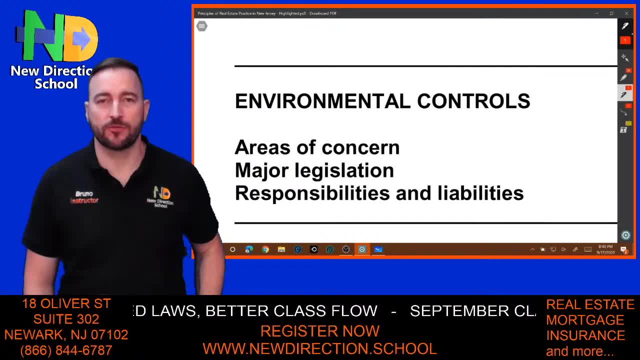 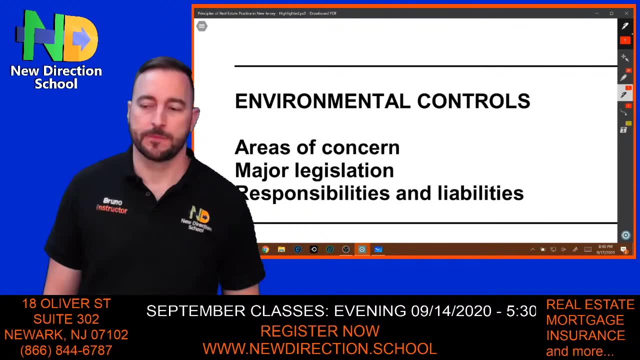 The environment. Let's go back to the story of the three little pigs. You think building whatever you want is a good thing. It's your property. you can do whatever you want- right. But if whatever you're building, If whatever you're building could endanger the society, right. 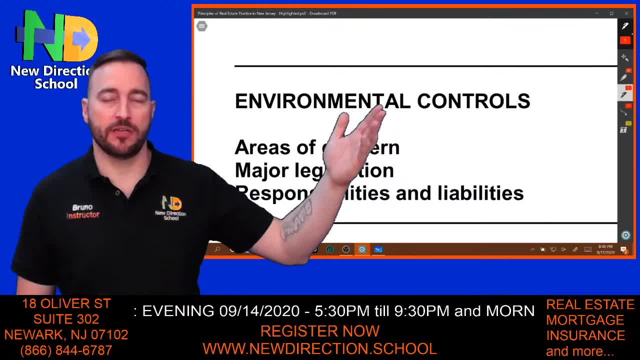 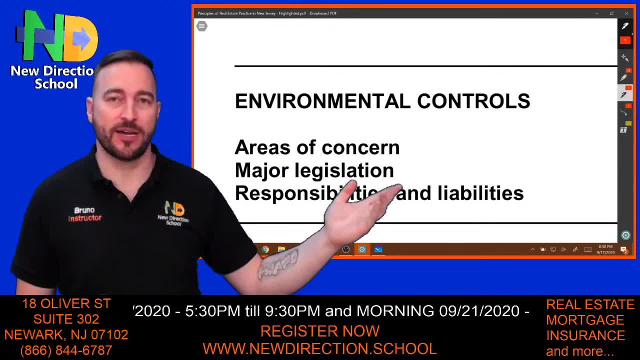 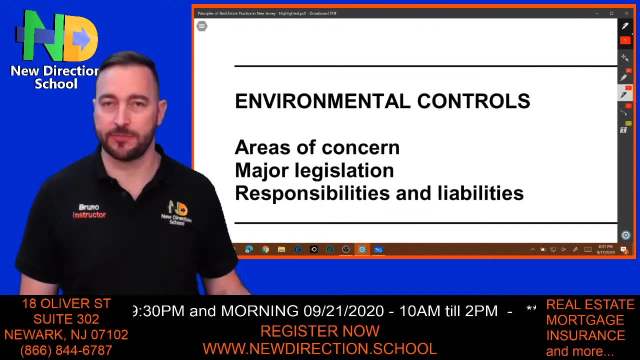 Then because of let's say, you're building a manufacturing by the water. By the water it means that you're manufacturing which most likely has chemicals, because every manufacturing, if there's machines involved, then guaranteed there's chemicals involved somehow, right. 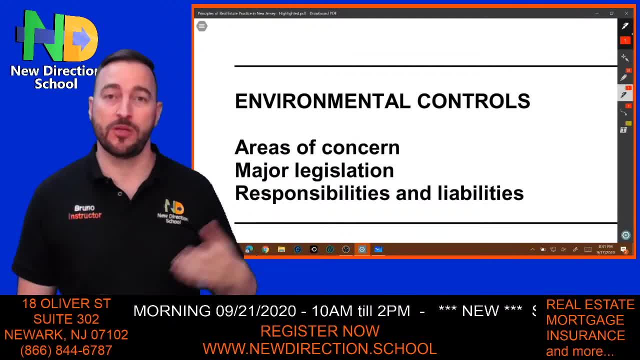 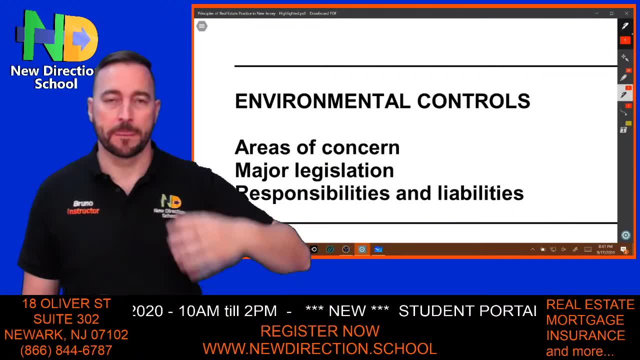 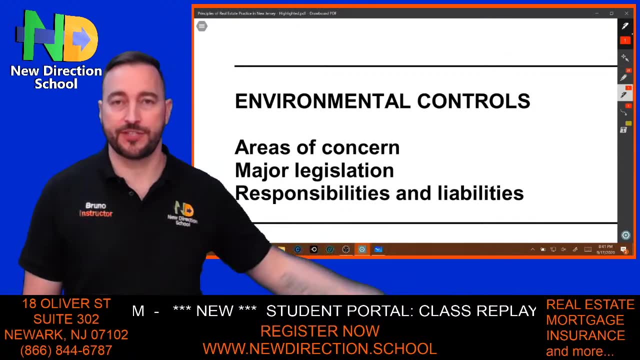 So if that pours into the water- which back in the day People were dumping those chemicals into the water- right If? if it goes into the water, then it could travel down the river or the lake and kill not only the marine environment or affect the marine environment, but also the individuals along said river. 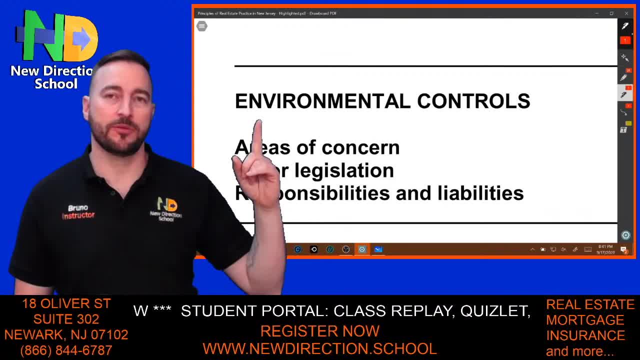 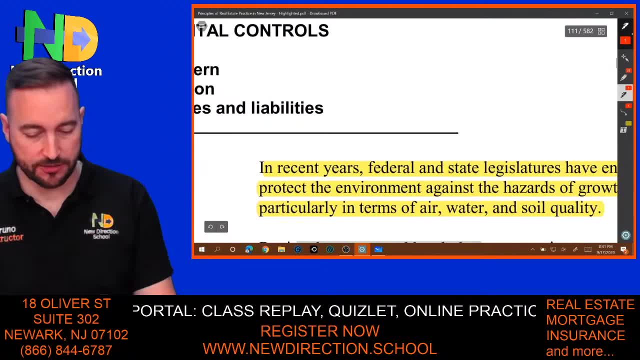 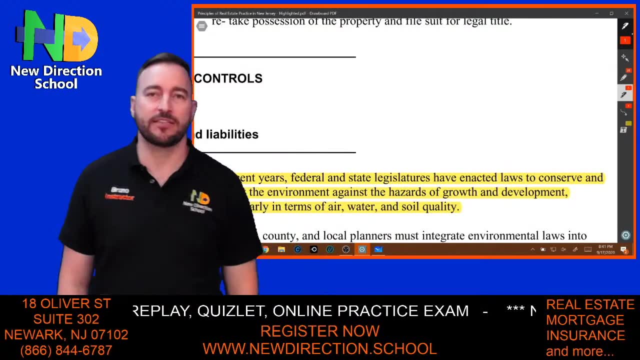 Okay. so because of things like that, they started implementing environmental rules and regulations as well. So in recent years, federal state legislators have enacted laws To conserve and protect the environment against hazards of growth and the development, particularly in terms of air, water and soil quality. 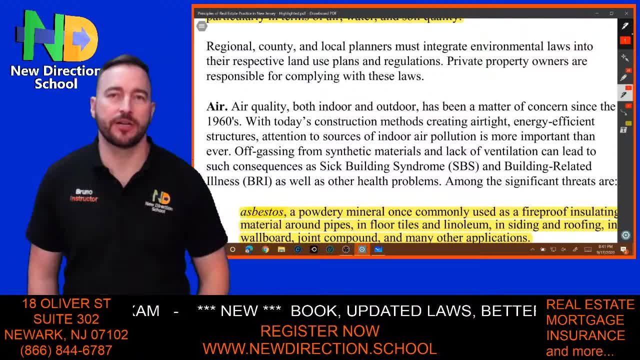 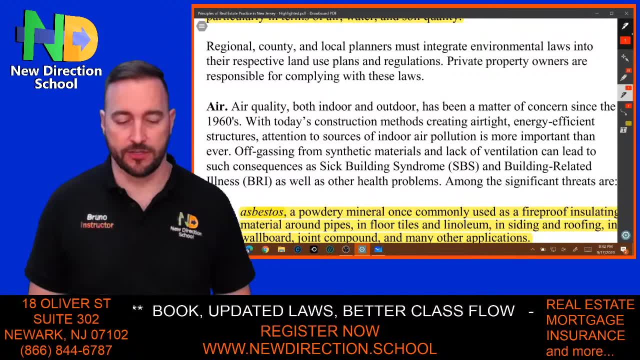 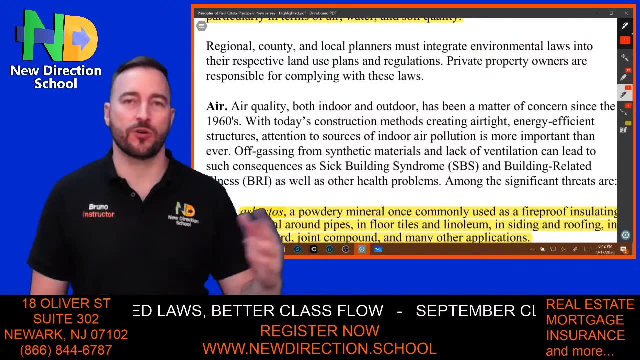 Okay, regional county local planners must integrate environmental laws into respective land use plans and regulations, and private property owners are responsible for complying with these laws. Now, one of the laws is based on air, Now the quality of the air. it could be indoors or outdoors, and we're going to address 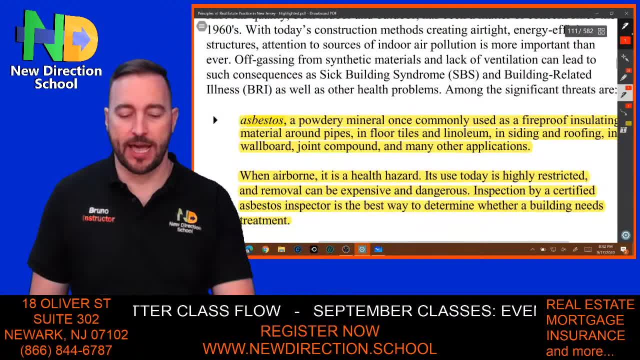 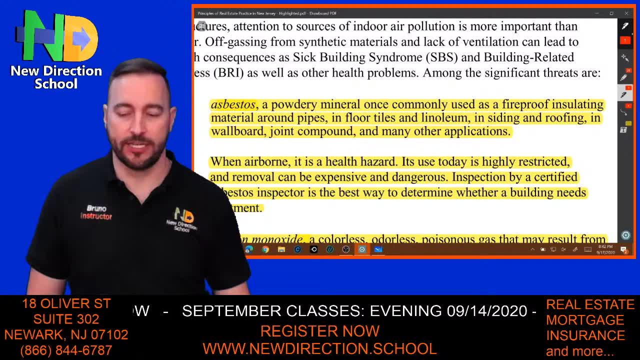 We're going to go straight forward to the indoors. The first one we have is called asbestos. The thing you need to know about asbestos is that it was a type of insulation. Okay, so when you see asbestos insulation, something to remember. 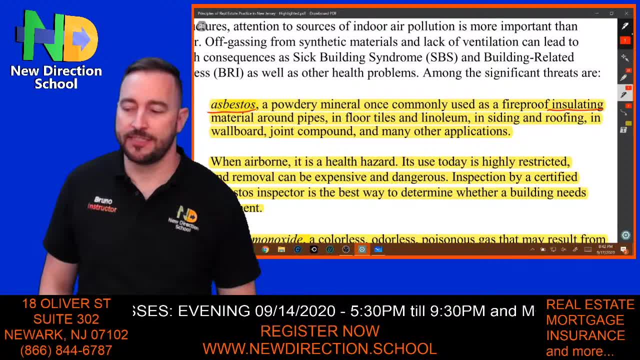 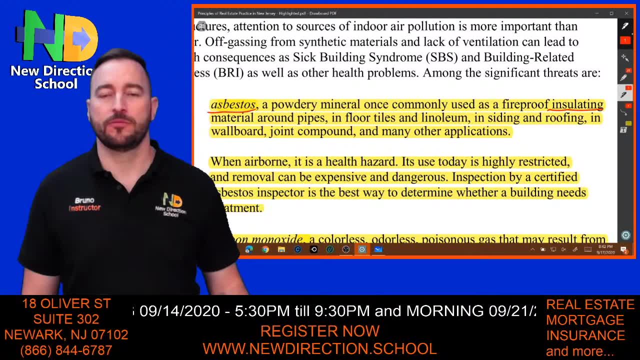 Okay, the problem with asbestos is that when you're when you're trying to renovate a property, you're going to have to renovate it, And when you're trying to renovate a property, as an example, if you touch the investors, if it's been there for a while, it could deteriorate and it could go into tiny filaments or particles and become airborne. 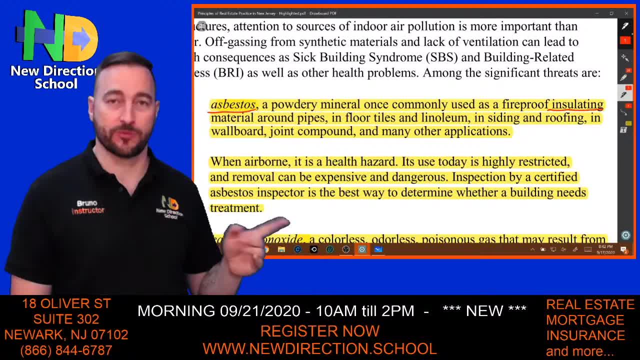 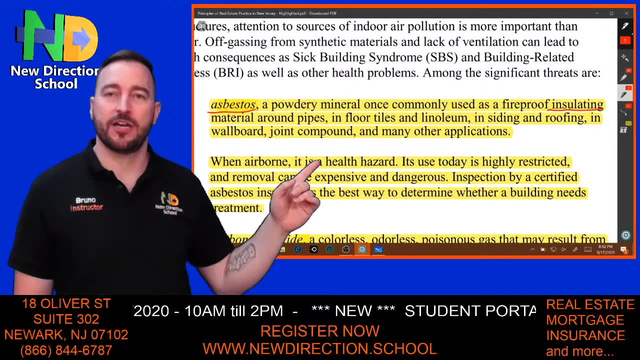 When it becomes airborne right- And I think by now everybody knows what airborne means, right After this whole pandemic airborne became the word. So when it becomes airborne it becomes a health hazard because we might not feel it, We inhale it and lodges into your lungs and can cause. 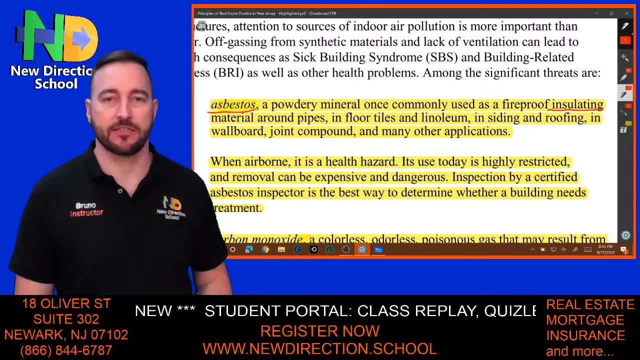 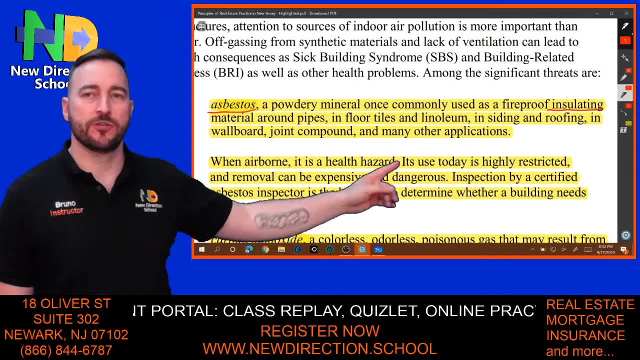 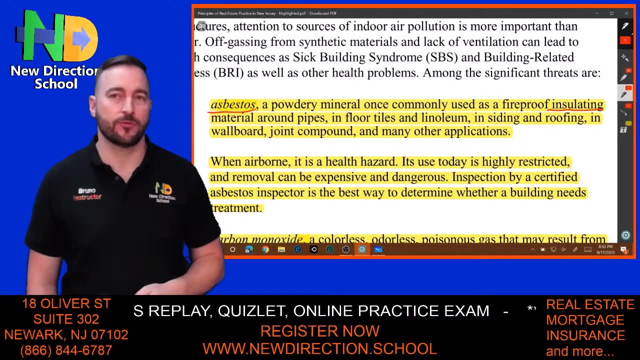 A bunch of other issues later, like lung cancer, as an example. Now it's used today is restricted as of 1978. It was banned so you cannot use it anymore. but removal can be expensive and dangerous because of what I just told you. you could go into your, you can breathe it, go into your lungs and become very dangerous. 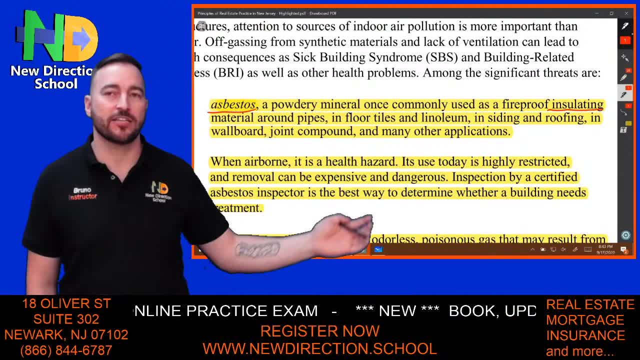 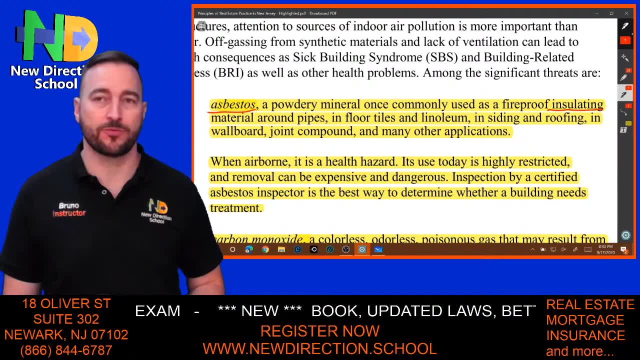 So asbestos to be removed has to be removed by a certified asbestos inspector. I'm sorry. inspection by a certified asbestos inspector is the best way to determine whether the building needs treatment, and treatment has to be by a state certified technicians as well. You cannot just remove it by yourself. or let me put it in a different way: 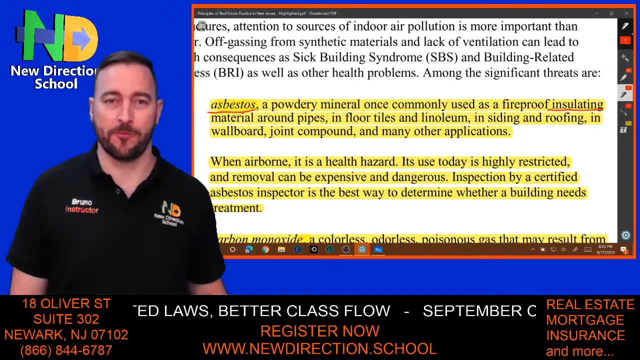 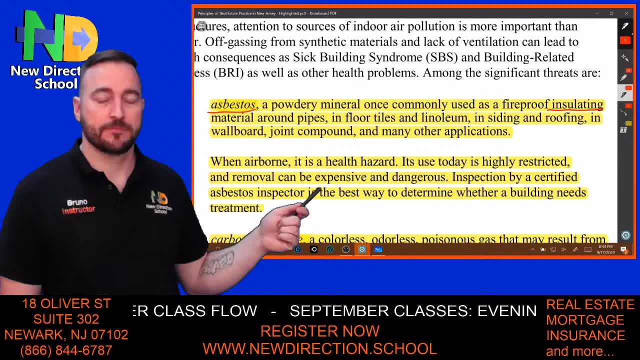 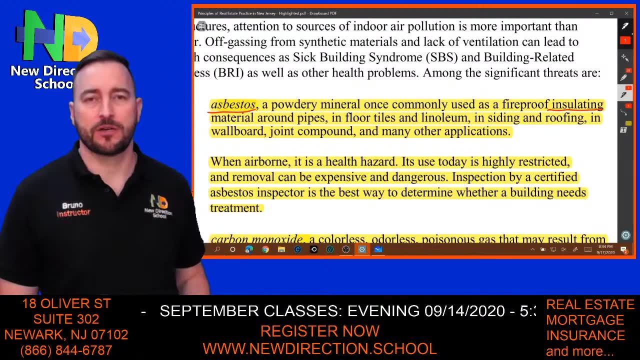 You shouldn't. The law says no, but people still do whatever they want, right? Especially those that don't know how dangerous this could be. All right, And it's very dangerous. OK, a friend of mine- And very Close A friend of mine- unfortunately passed away a couple of years ago- not too long ago- and he got it when he was 18.. 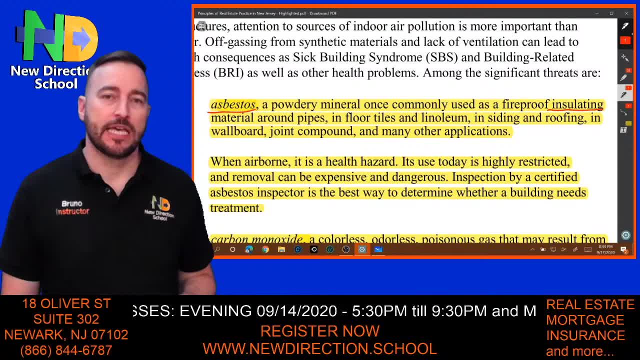 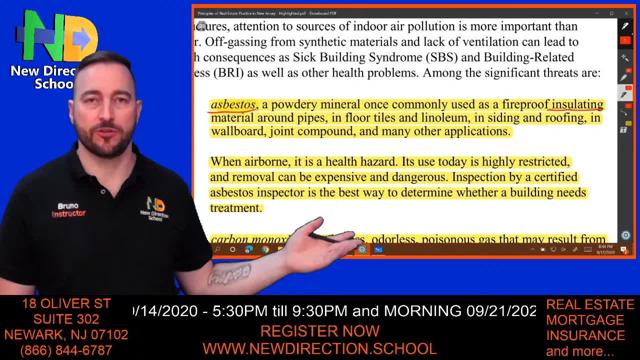 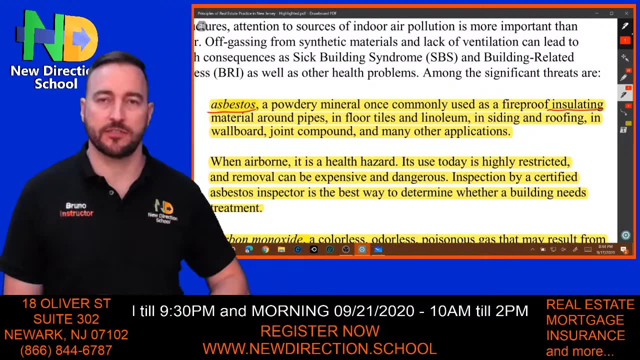 While working at a factory that dealt with this stuff and it lodged in his lungs. nobody ever caught it. he got a pneumonia a few years back and because of pneumonia and the treatment they were giving them, they did a bunch of x rays and then a bunch of other exams and they found that he had a mass in his lungs. 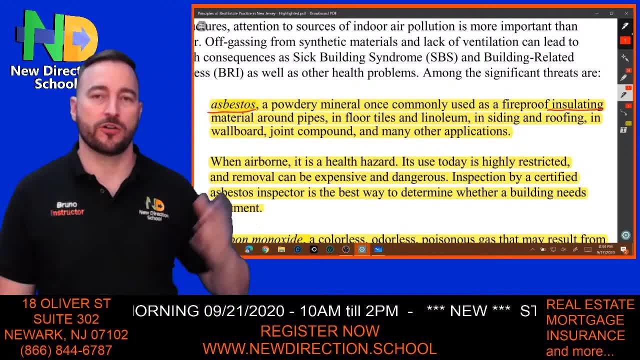 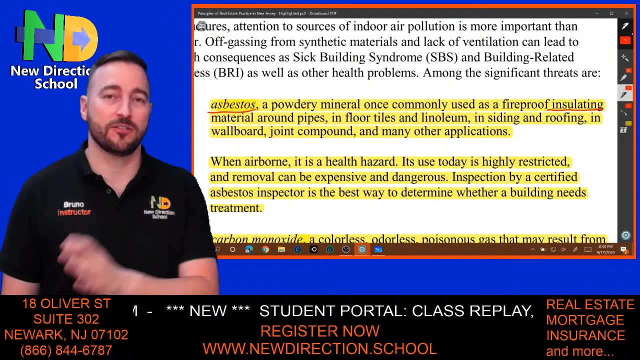 When they took a biopsy of it, they figured out that it was caused by a tiny film of asbestos that, lodged in his lungs, resulted in cancer. Unfortunately, he did not survive that at the age of seventy two or seventy three from it, But this was something that was in his lungs since he was 18.. 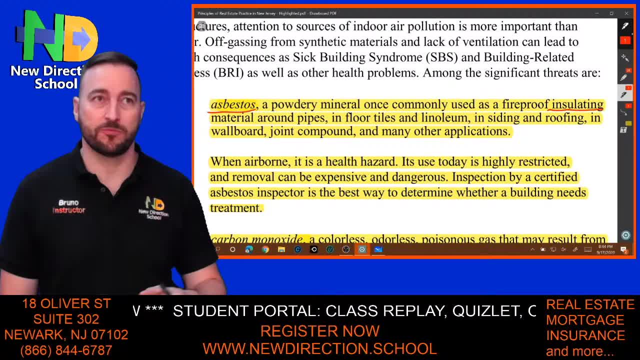 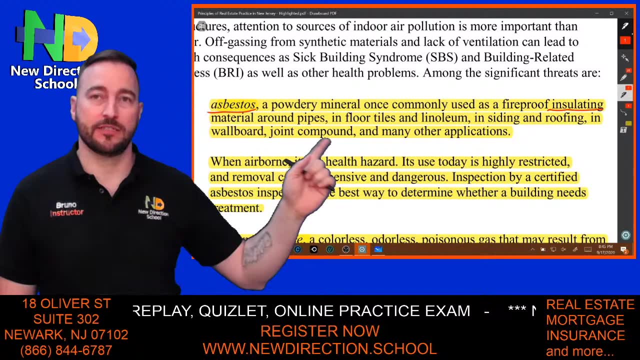 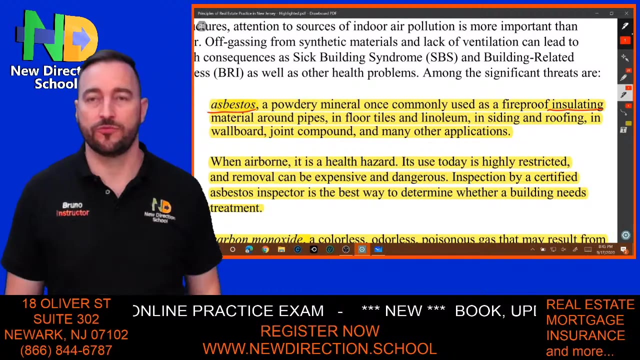 Now, good thing that he lived a great life, amazing person, probably one of the best persons I ever met in my life. a really nice guy, helped everybody. It was just just amazing person altogether And He lived a great life. but he died because of this lodging into his lungs and causing cancer. so it's very, very dangerous not attempt to remove. you'll never know when it's going to hit you. 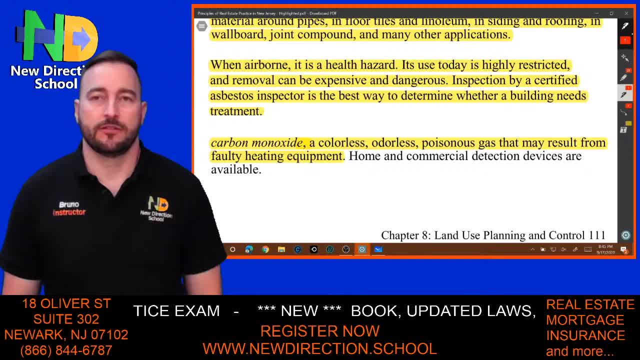 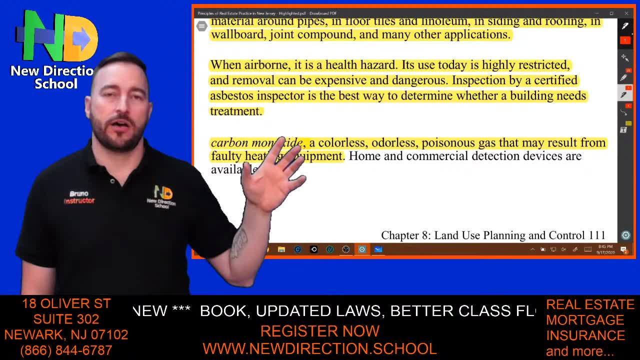 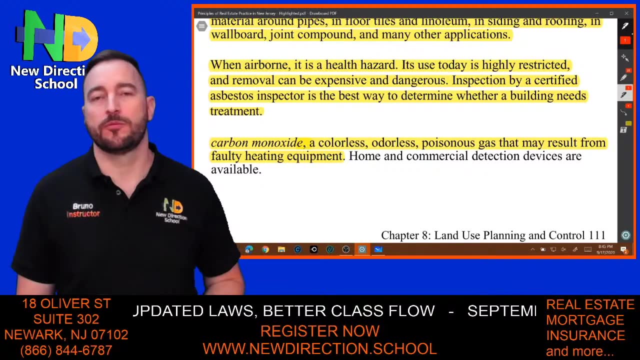 Carbon monoxide is another danger. right, It's colorless, odorless, poisonous gas that may result from faulty heating equipment- equipment. So if your appliances at home are not working properly, Or Even your stove, for instance, is not working properly, it could release carbon monoxide. 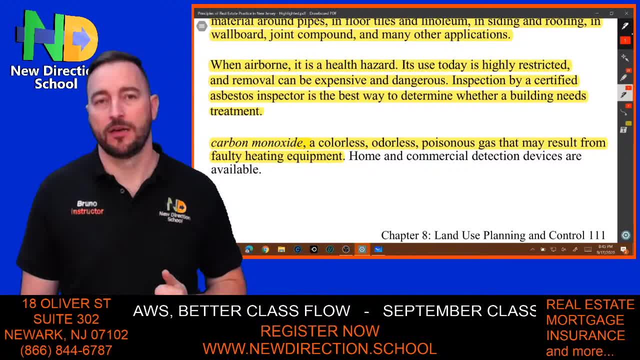 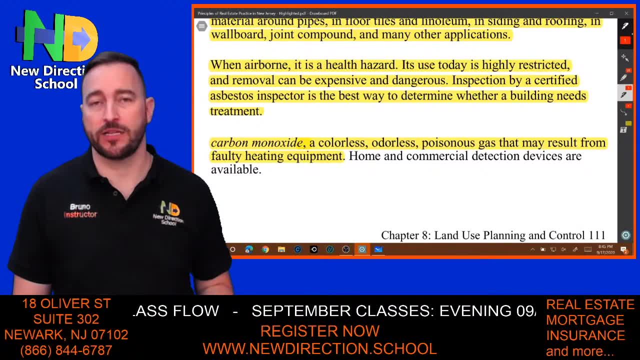 And this is called the silent killer, right Why? Because it's again colorless, odorless, but you don't see it, you don't smell it, And if you're sleeping, your brain does not react on time to this danger. 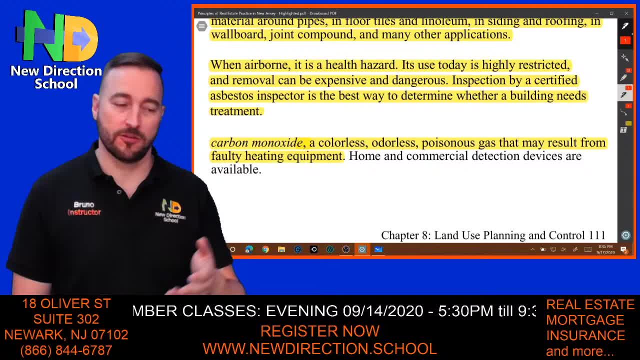 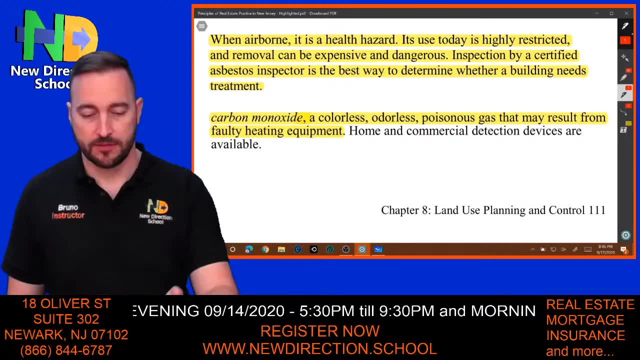 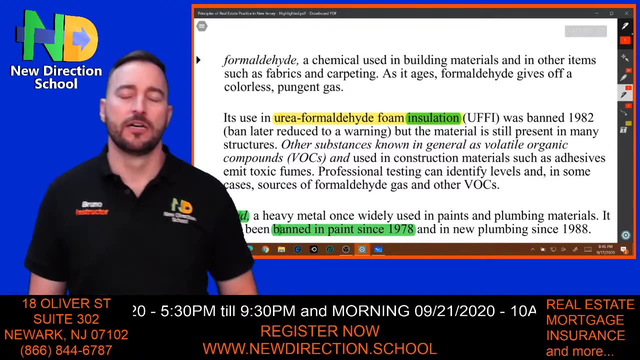 So you might just die again, Silent killer, You might die sleeping. That's why it's very dangerous And you have to have detection devices in your Property. So carbon monoxide detector. We have another one called formaldehyde, and this was also banned in 1970. 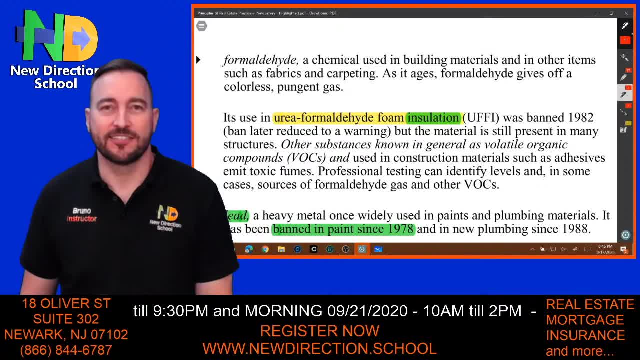 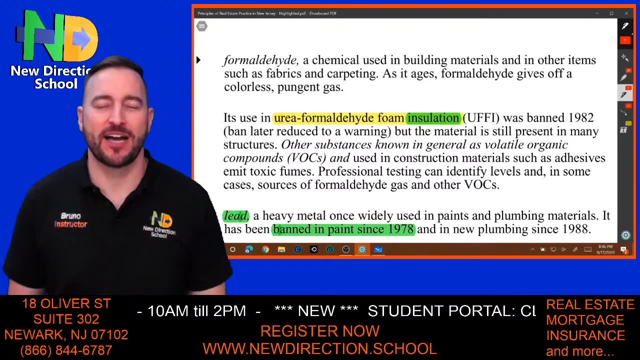 You're real formaldehyde or UFFI, right? Vanessa's smiling? Vanessa C is smiling because The we had this conversation today. you read it formaldehyde, and she had a really cool way of saying it, and I'm pretty sure all of you have a really cool way of saying this. but just go by UFFI. 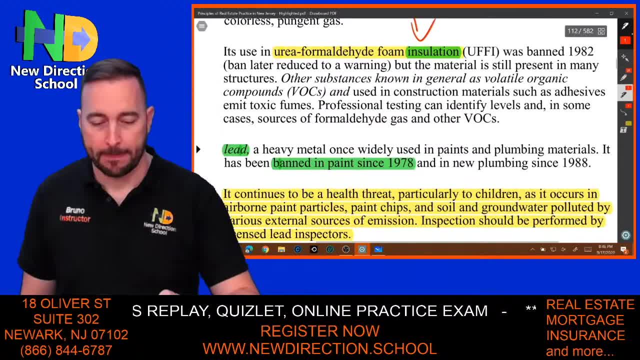 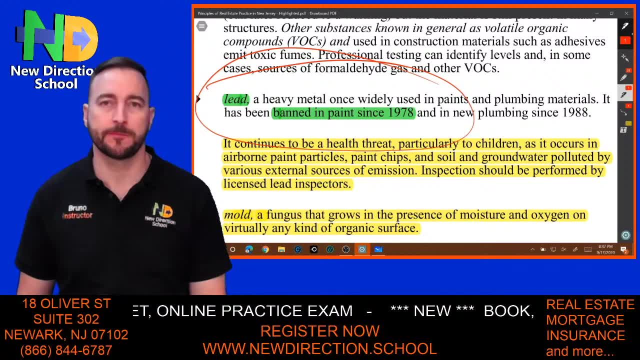 Most places don't use it anymore. This one is very serious and we're going to talk about it in a later portion of this book. Let So lead-based paint has been federally banned- federally banned since 1978.. This will be in your state: exam guaranteed or your money back. 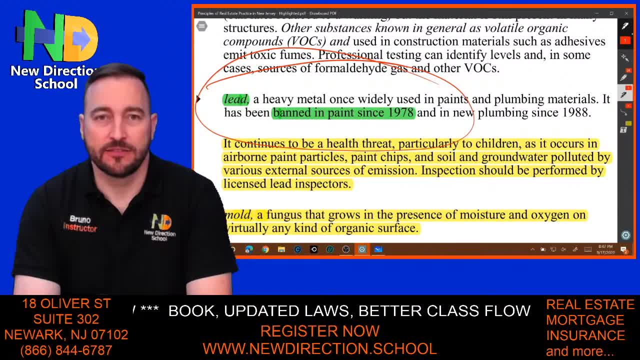 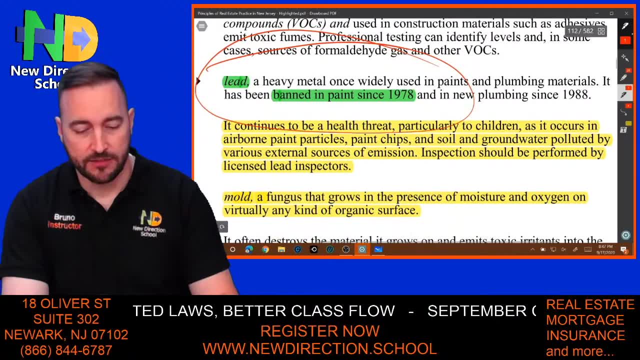 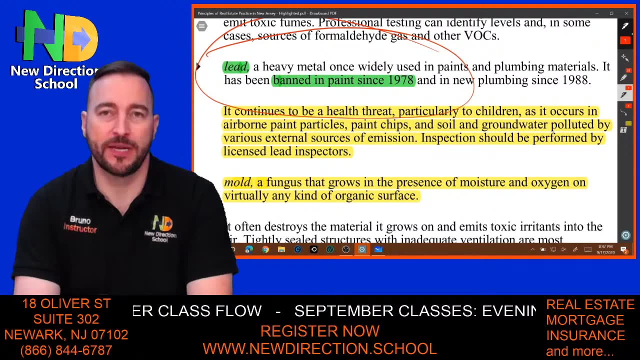 Okay, Lead-based. lead-based paint was banned in 1978. And it's very, very dangerous. It continues, as it says here, to be a health threat, particularly to children, as it occurs again in airborne part, paint particles, Paint chips. It's very sweet and the kids can grab it, put it in their mouth and there you go. It affects. it could affect their brains and affect their, their, their hearts. It could affect a bunch of stuff. So very, very careful that if the property was built before 1978, you have to inspect the property. 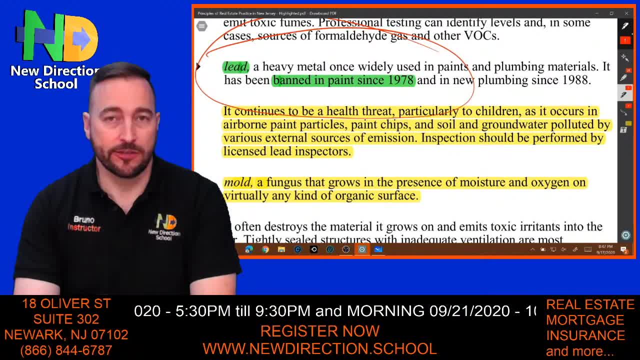 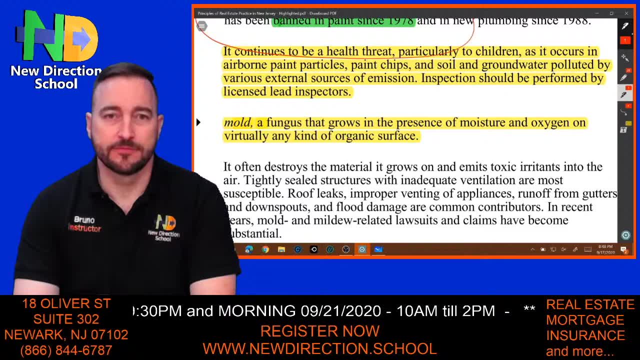 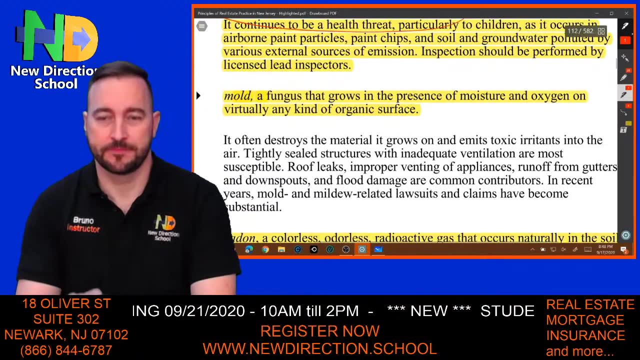 This is federal, OK, federal law. state law also has Mold. I think everybody knows what mold is. Right, Right, Is there anybody that doesn't know what mold is? Raise your hand if you don't know. All right, cool Moving forward. 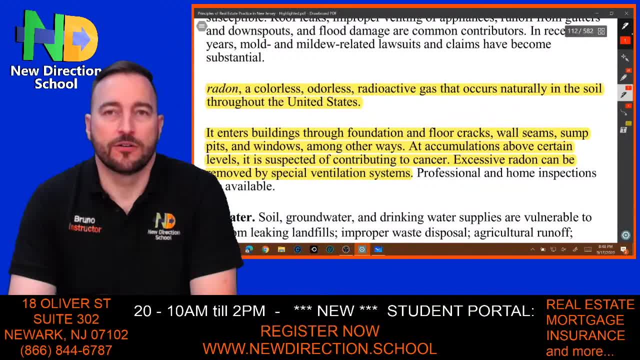 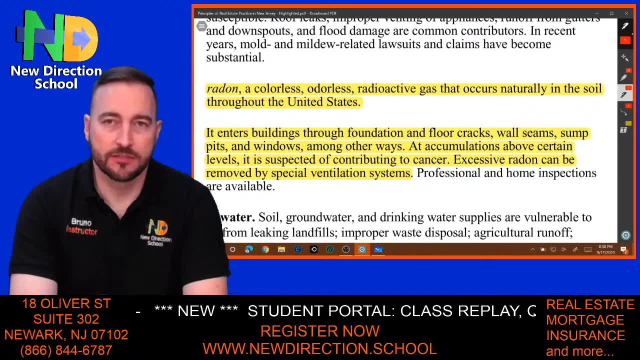 Radon. So radon is just like carbon monoxide. Radon is colorless, odorless and it's also tasteless, just like carbon monoxide. So you do not know it's there until it hits you Right. The problem with radon versus carbon monoxide: 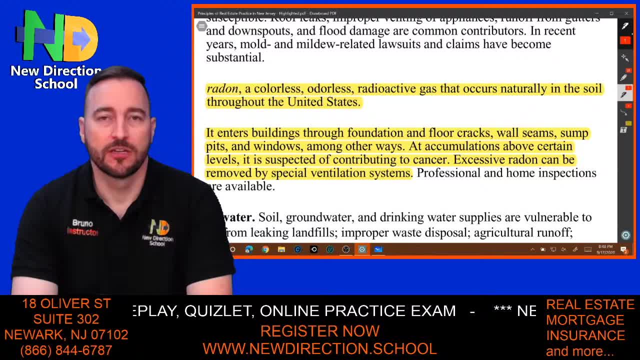 Radon is a natural radioactive gas that occurs from the ground up and in the northeast of the United States we are very, very rich or wealthy when it comes to radon. All right, I can show you a map later on about about radon in New Jersey. but there's heavy concentrations of radon in New Jersey. 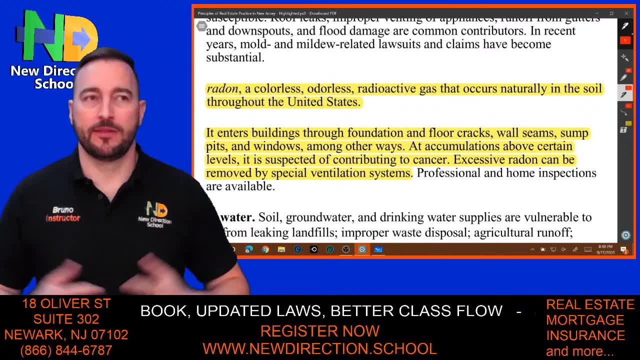 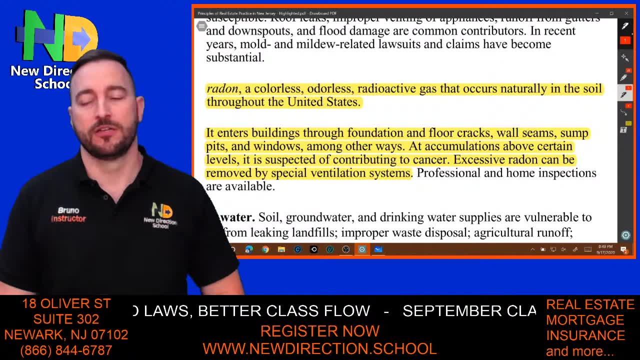 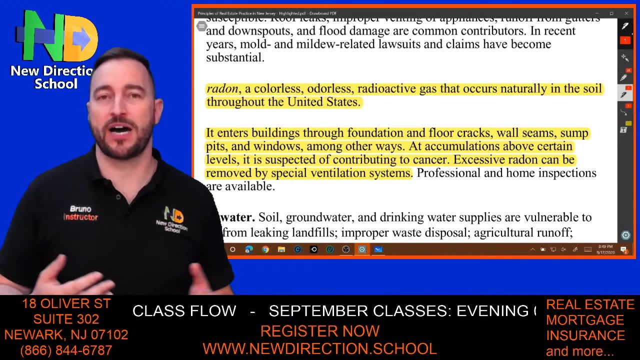 So for this reason, There's there's rules and regulations. every state has rules and regulations regarding the testing of radon and transferring property and all that stuff. So, because it's a natural gas, There's nothing that the that the seller is at fault and the buyer has to deal with. 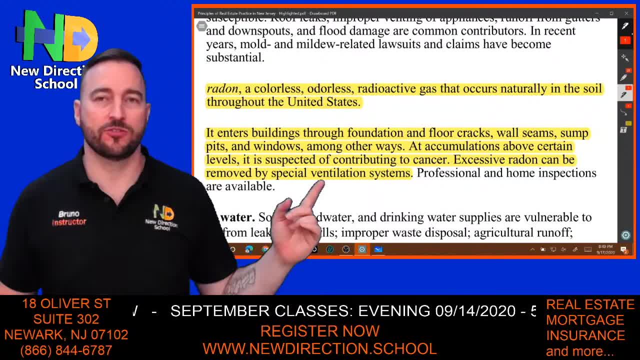 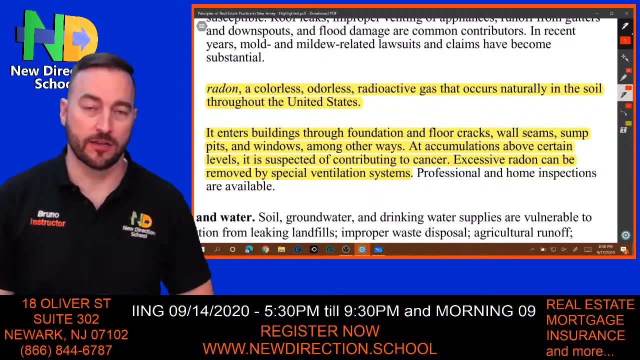 The cool thing about radon: it's very easy to to fix by having proper ventilation in the house. or if there's no way to have proper ventilation, You need to install a ventilation system. That's all it is. So you need to pump fresh air and move out or circulate the air they have inside the house. 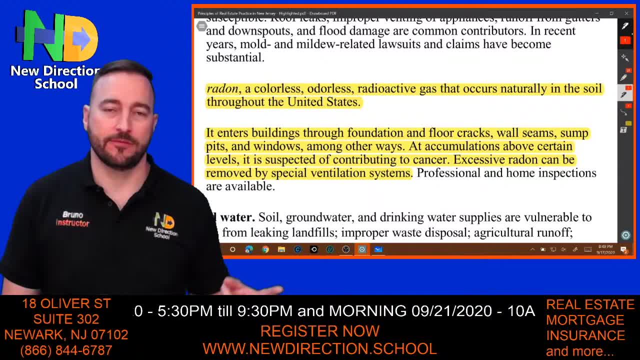 Radon, carbon monoxide and, obviously, fire hazards are the reason why you cannot live or sleep in a basement. There is a reason why most cities ban and states ban the renting of basements: Because, Because usually there's not enough ventilation in those areas. 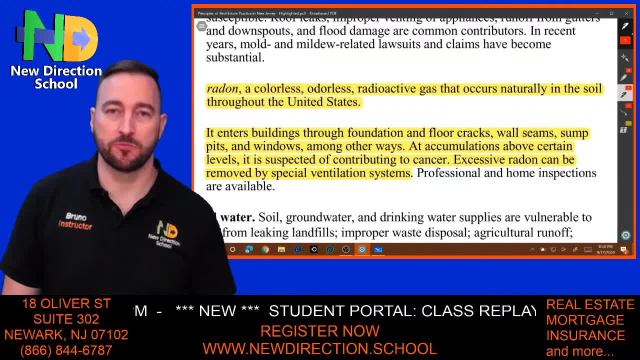 You guys understand. A lot of people think, well, but I got to make money to pay this mortgage. at what expense? Killing someone, Understand? turn it into something else. I was just telling somebody earlier. turn it into somebody else or into a storage place. rented a storage. 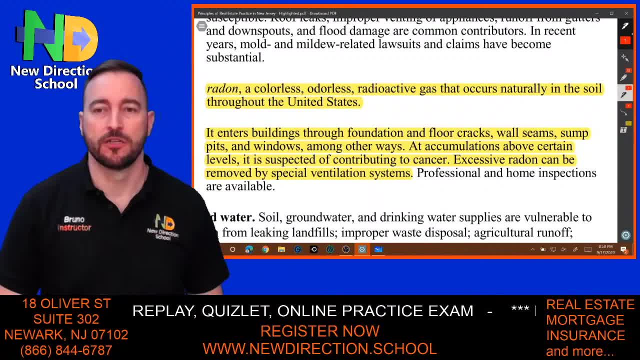 Basements attics. you can still make money with rented a storage. You probably don't make as much money, but at least you have peace of mind because nobody's sleeping there and dealing with this. OK, it's only when it's trapped in high. 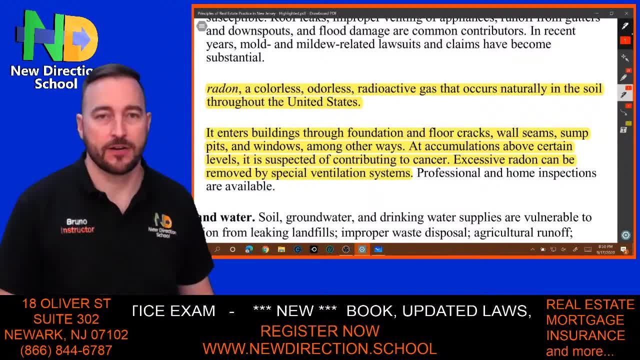 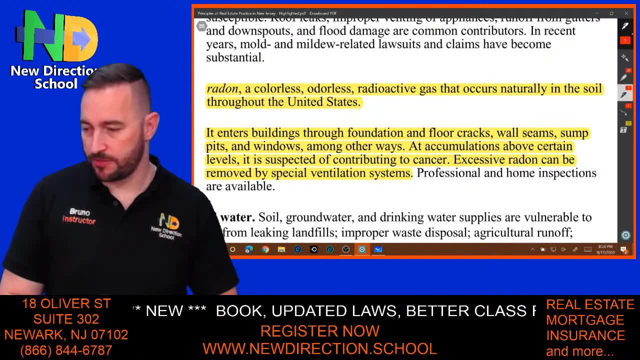 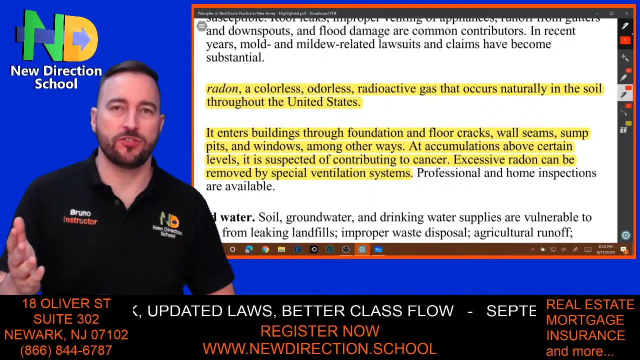 concentrations that it becomes dangerous. All right, That's good with it. So far Great. I was even has a question, so I'll wait for that. Laura said comes from the ground up At almost every transfer right nowadays they do the radon test anyway. 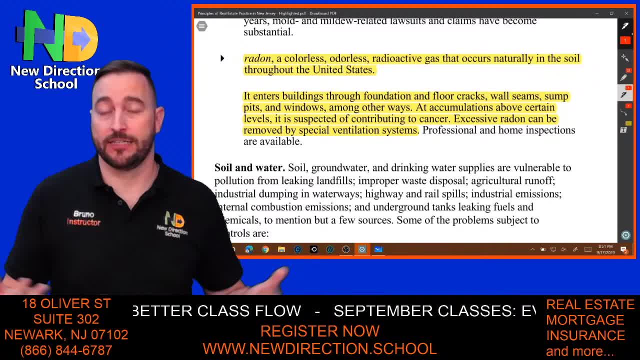 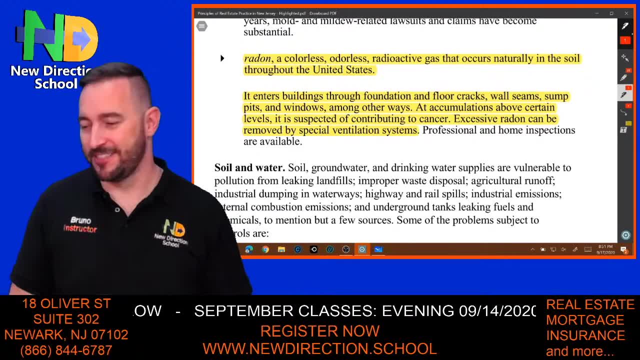 And this is something you cannot ban because, again, it's natural, like it just happens. OK, Muslimah says: what if there are windows in the basement? I knew these questions were coming. What if there are windows in the basement? 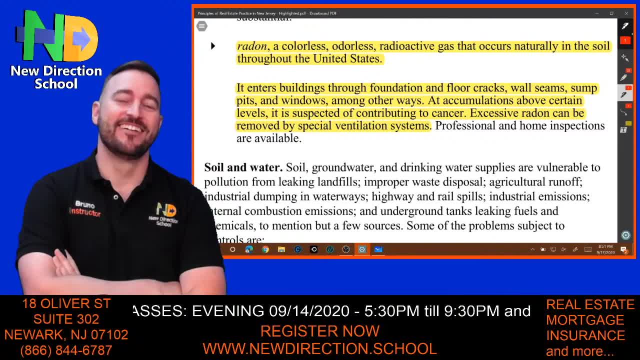 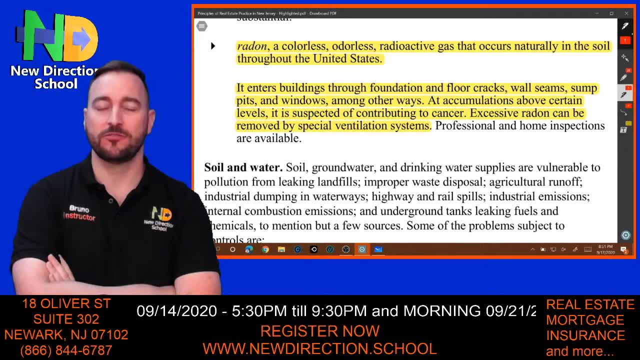 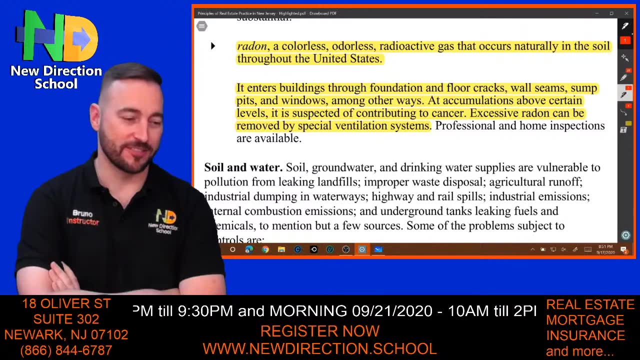 Can we stick people in there? OK, you're. if you have an above ground basement right, your town might allow that basement to be converted into a legal apartment or half apartment. let's call half right because small. I think I just answered. 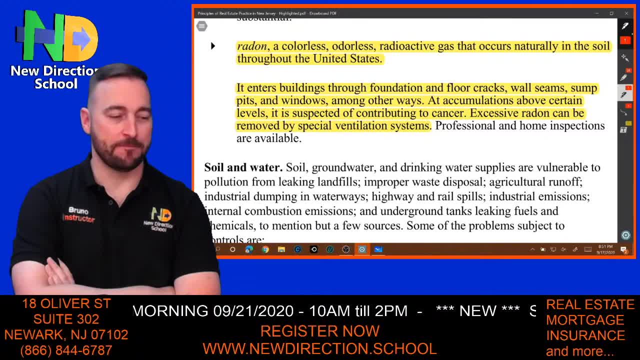 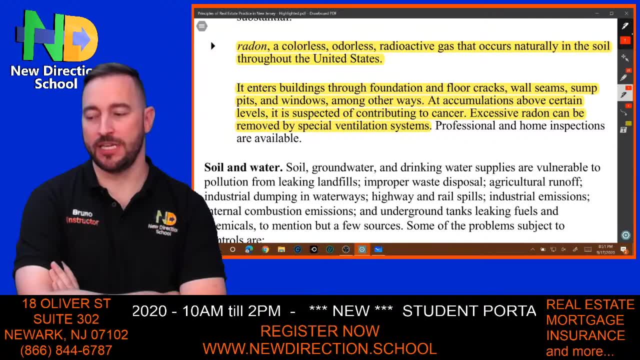 He's too funny. I think I just answer you. but if it's a below ground or mid-level right, It's very dangerous, even if you have high windows. even if you have high windows, there's not enough circulation, because having windows doesn't mean they're open. we're talking about circling air. 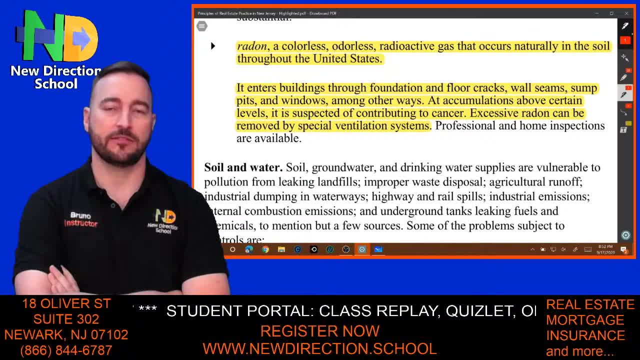 So the in and out of the units Right. If it's above ground, usually there's the. you open the door, you open the second door and there's a flow right. Just having windows is not enough. Once Radon tested, it's clear. can it come back? 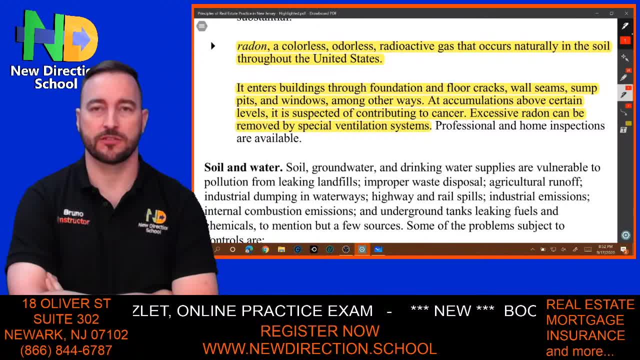 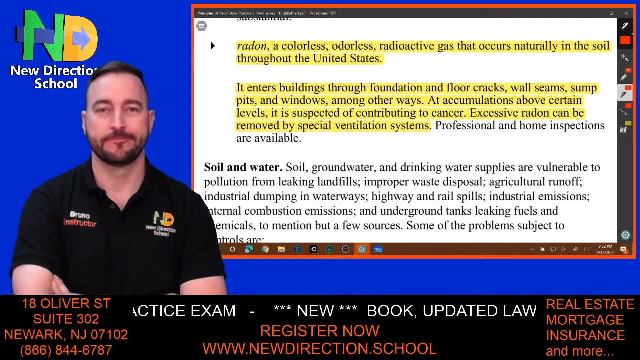 Like I said, it's a natural gas. In some areas there's high concentrations of it- very high, So can it come back? It's something that's never, ever, ever going to go away, So You have to deal with it. 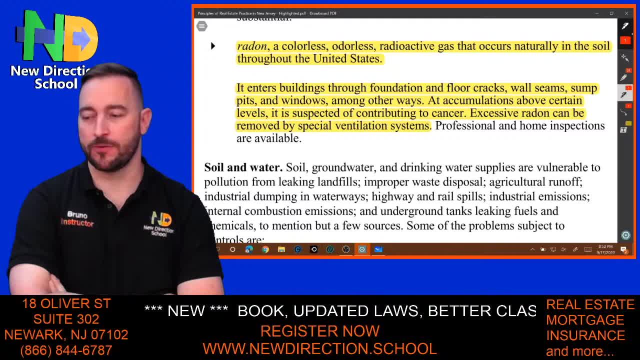 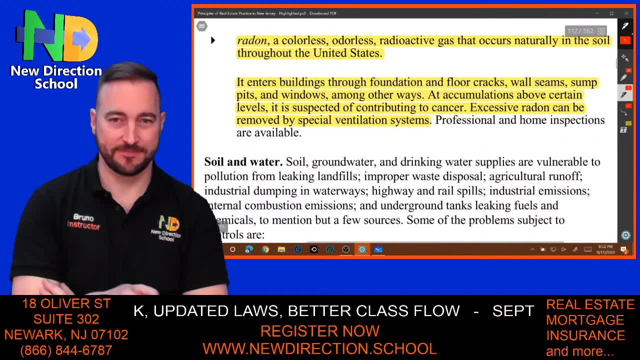 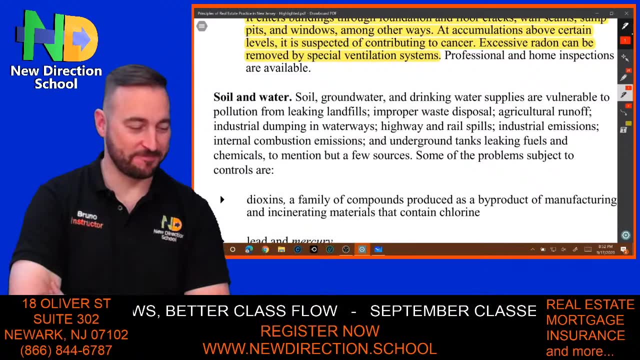 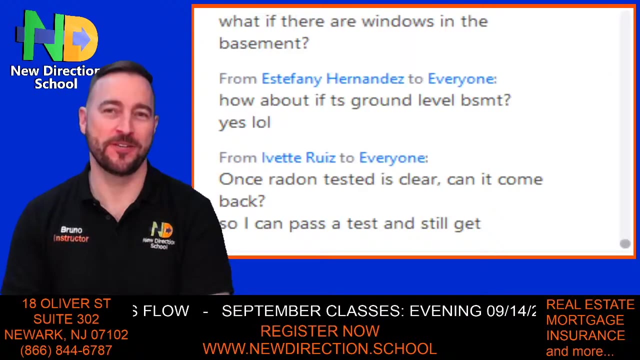 You got it. Radon doesn't go away. That's good, All right. Some facial expression Like: if that is just the way you asked, Okay, I'm laughing just because of the way you asked, So I can pass the test. 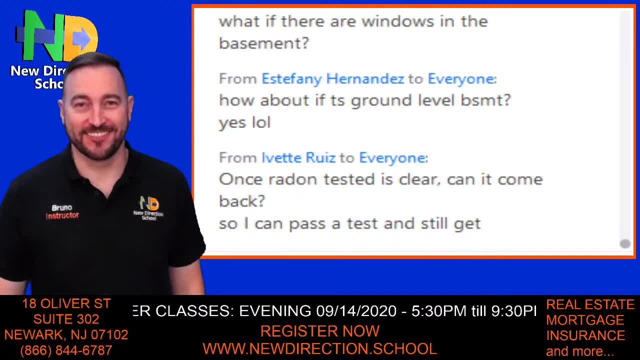 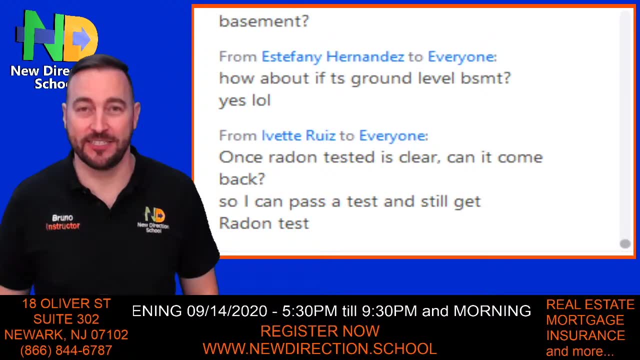 Do you still get it? Yes, It's funny because of everything. not funny, but funny because of everything that's happening now. But yeah, unfortunately, because it's a natural thing, that's always going to be there. you can test now. 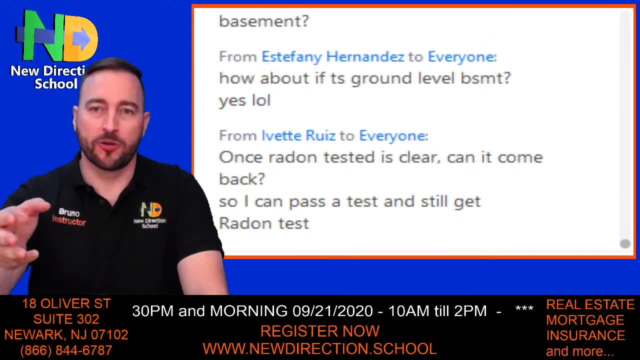 Let's, let's think about it this way: You're a person, but you're a person that keeps the windows open all the time, But then you sell the property to somebody else and that somebody else Always has the doors, windows, closed, always central air, because we got used. 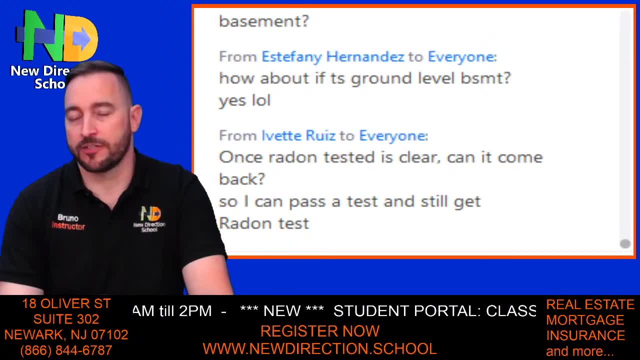 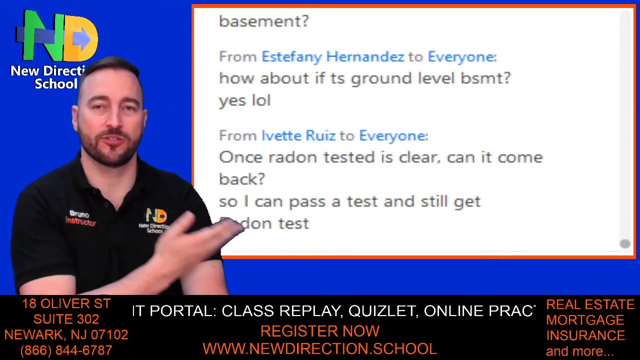 to that lifestyle, the central air lifestyle, right Always, or the air conditioning in general, So it's always closed, Always. the air is trapped, It doesn't circulate out in or out Right, So the next person, right The next person, could be accumulating radon for the lack of ventilation. 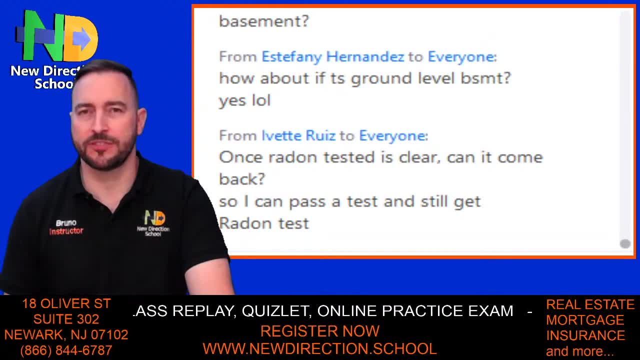 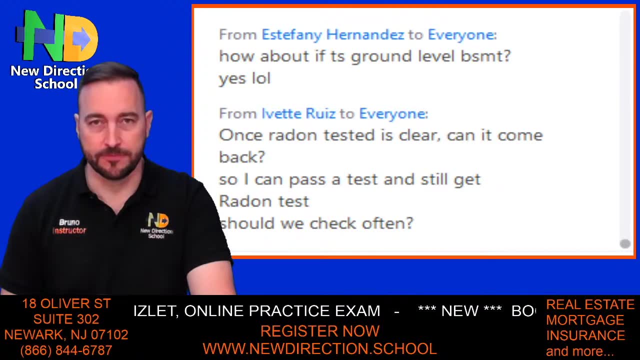 Right, And even though, Okay, so let me. probably some of you are like: oh, but you just said, You just said air conditioning. So if there's air conditioning, there's circulation, not enough circulation, Depending on how you have the air condition modes. 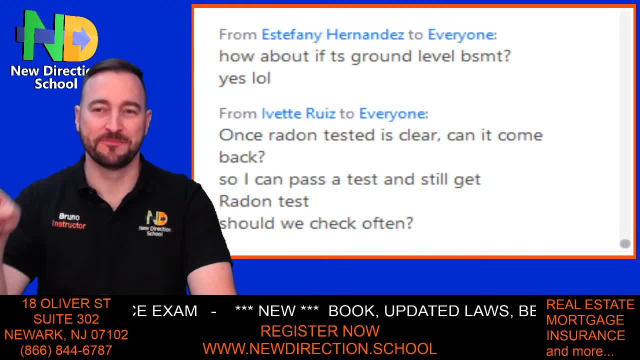 the air conditions are circulating. the air that's inside The air conditioning is not bringing air from the outside in, You guys understand, or taking air out, So you got to be very careful with that. Should we check often? I'll just put it. 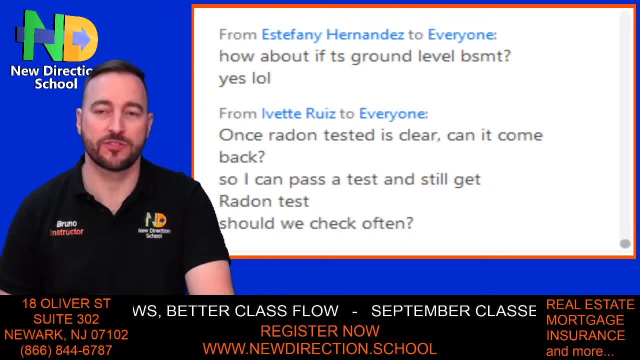 This way. if you intend to sleep in the basement, let's say you're a single homeowner, single family homeowner. If your rooms are in the basement, Yeah you should. If you spend considerable time in the basement, Yeah you should. 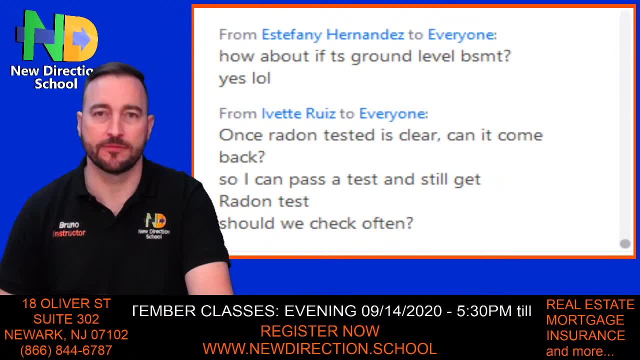 It's not that expensive. so once a year if you want like 80 or 90 bucks To do it yourself. if you bring an inspector it's probably more, but do it yourself. It's a little canister that you put there. 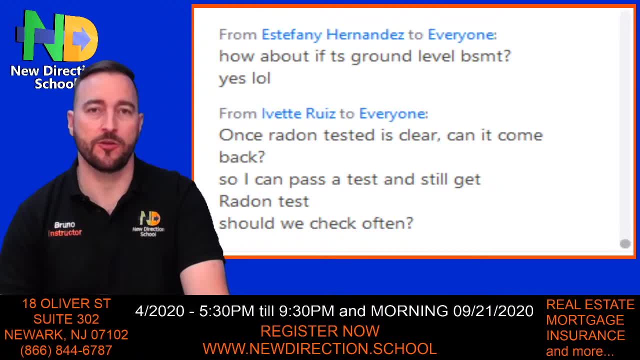 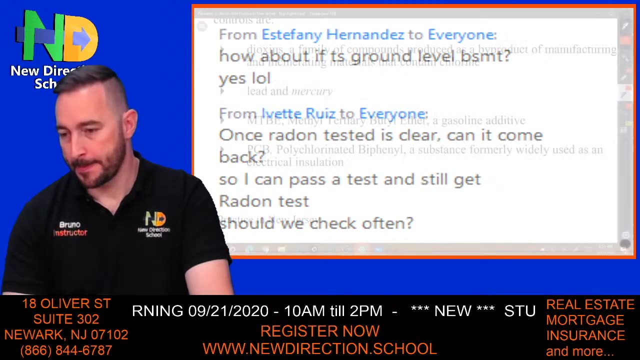 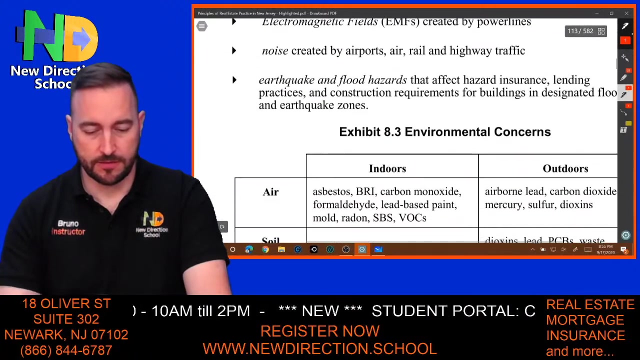 It stays there for 24 to Three hours, depending on the canister that you buy, and then you have to submit it to the lab and the lab tells you the results. Simple: OK, But yeah, do it Next, If this is OK. 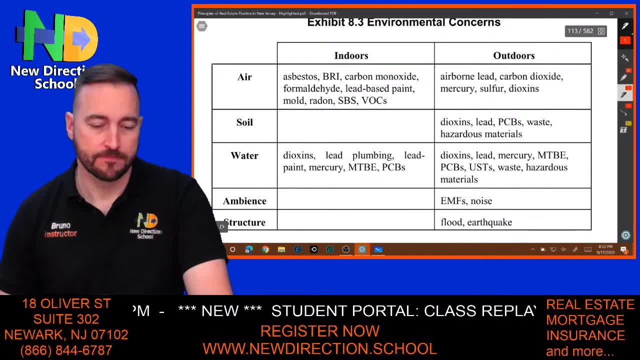 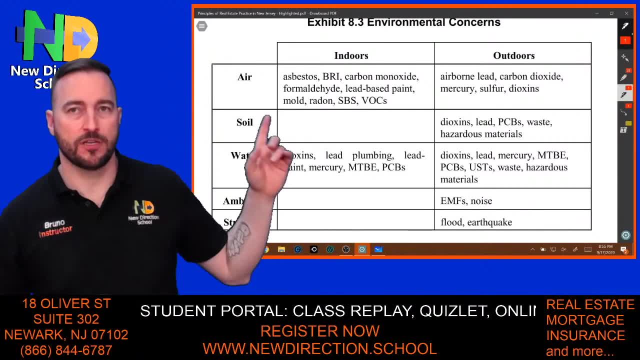 Environmental concerns. you guys should be aware of these Indoors For the air and water. These are some of the issues: The BRI, SBS, VOCs- and this MTV is there right here that tells you right here what they are. 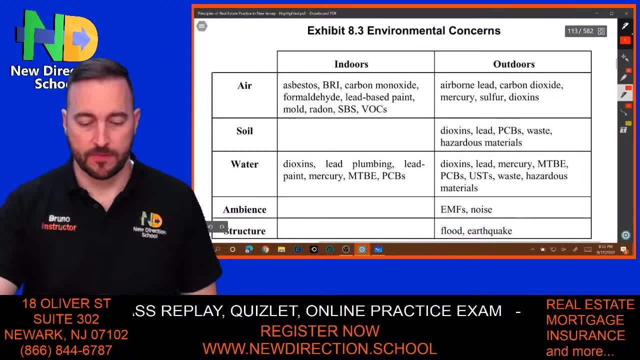 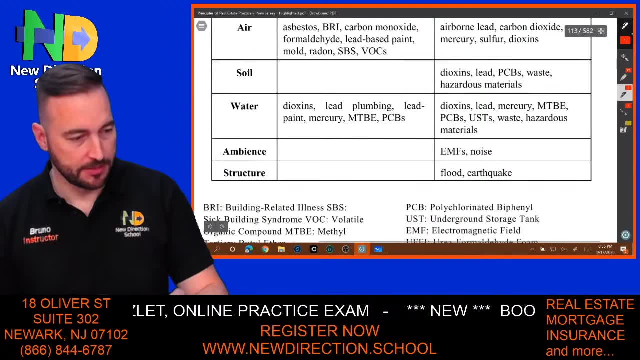 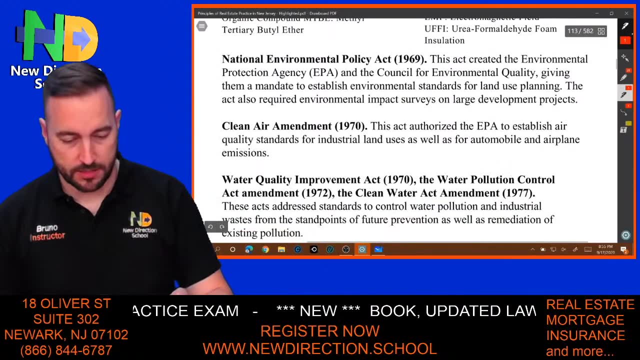 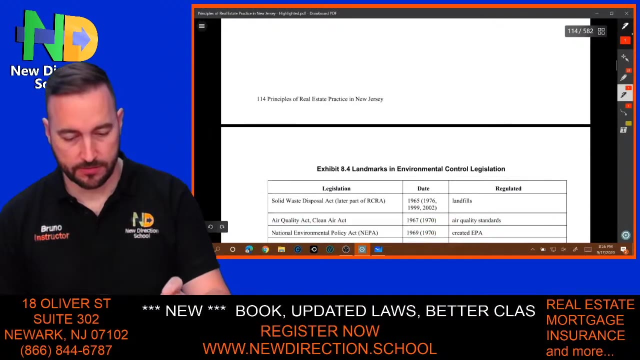 OK, It could affect you indoors or outdoors. These are some of the issues That could affect you. OK, oh, there you go, right underneath. gives you the what they are, And I'm going to move to Landmarks. OK, 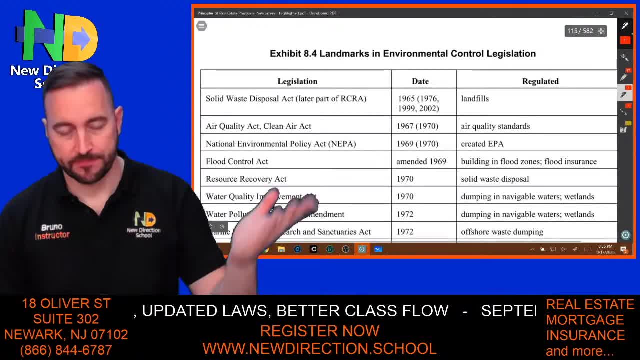 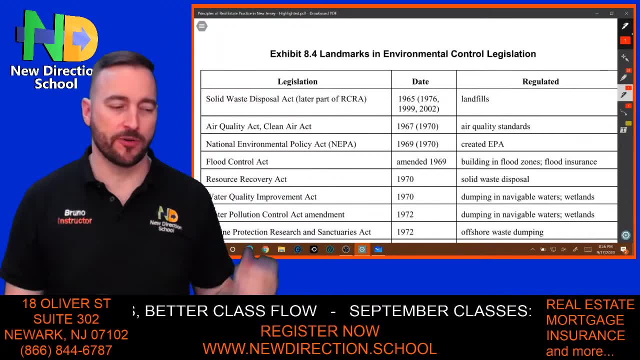 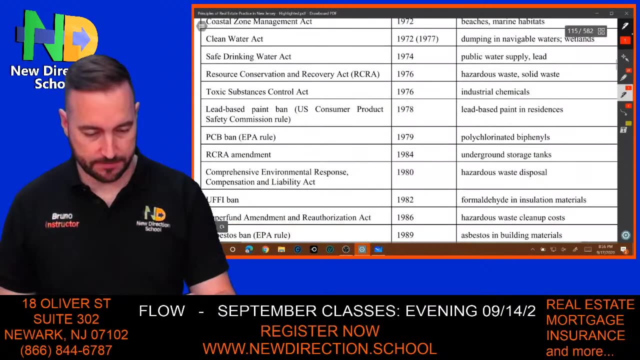 For state exam. It really does ask you who regulates what in terms of environmental? The only two. they, the only two things you might need to remember is CERCLA and EPA, and CERCLA is the comprehensive loss right here, And the other one is the. 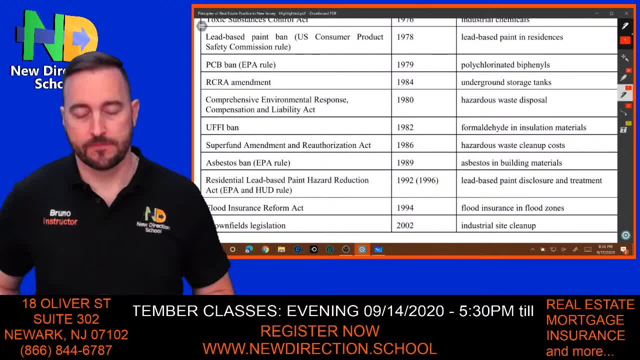 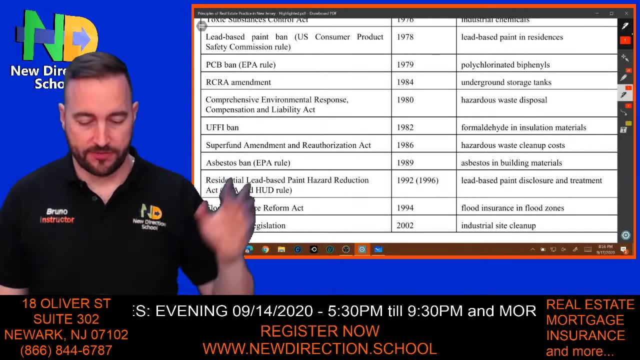 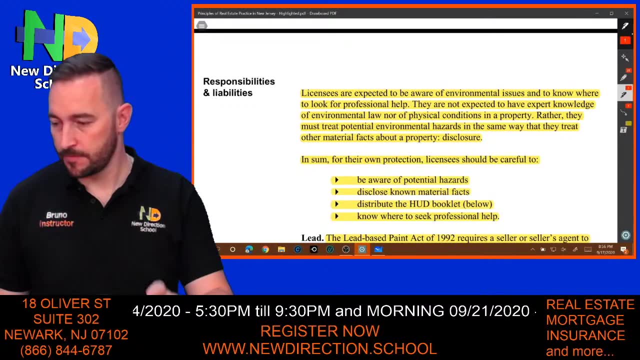 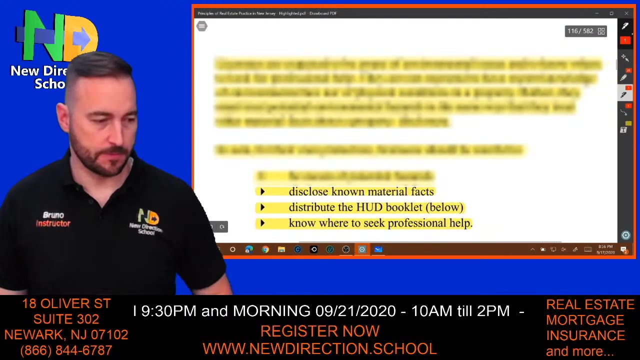 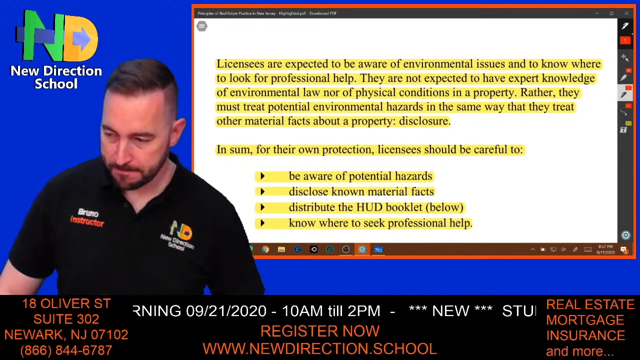 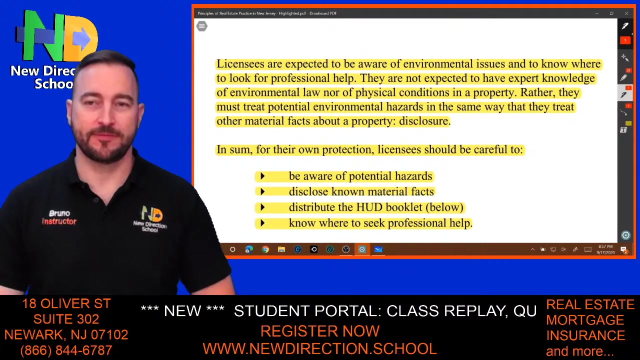 response compensation liability act. This is implemented by the, By the EPA. OK, so that's probably the only one you need to really remember out of these four. state exam. OK, We're now on page one sixteen. You want me to repeat that? 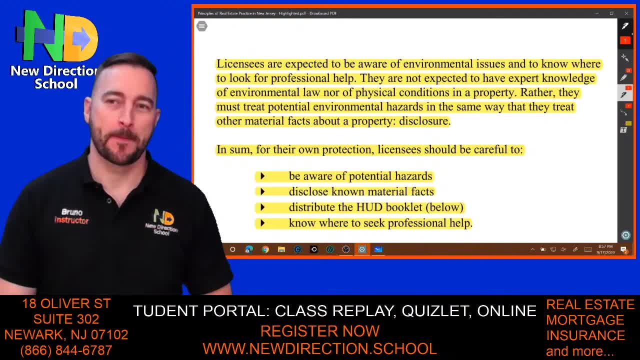 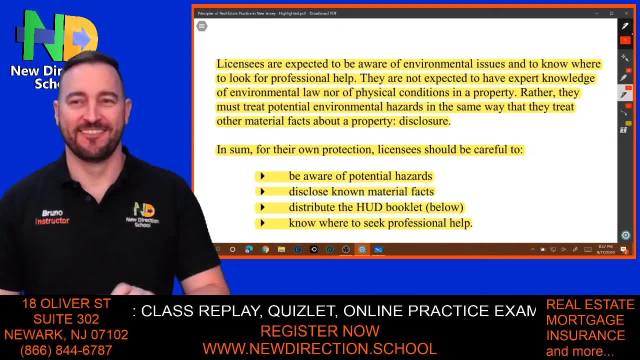 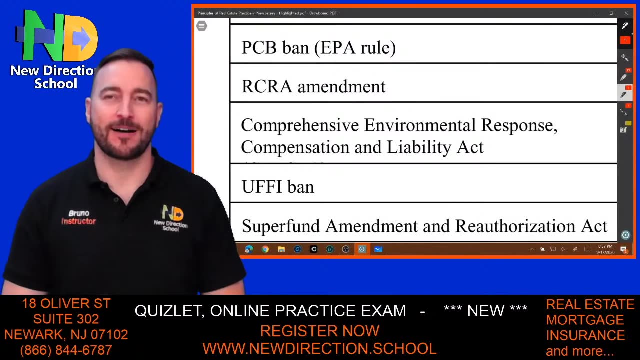 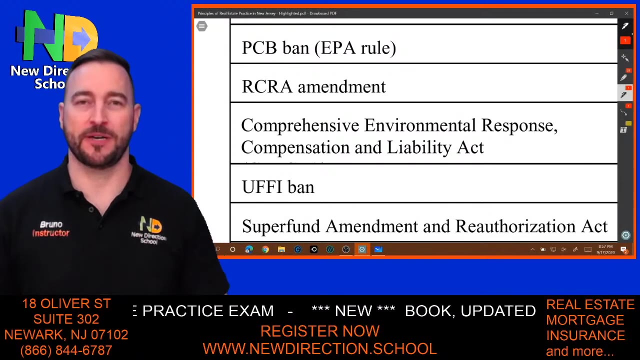 You know I'm going to do it right, Right That What I was saying is CERCLA- Comprehensive environmental response compensation and liability act, CERCLA. I'll talk about it better in the later on or in a different chapter. 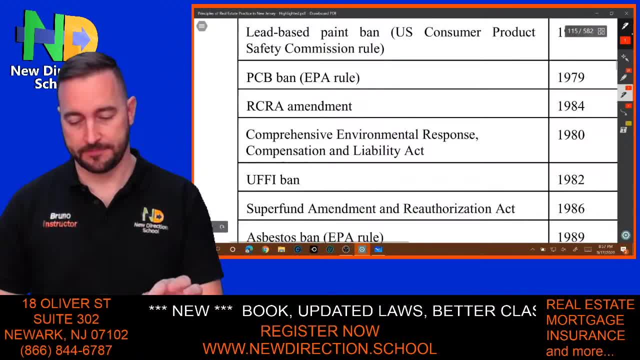 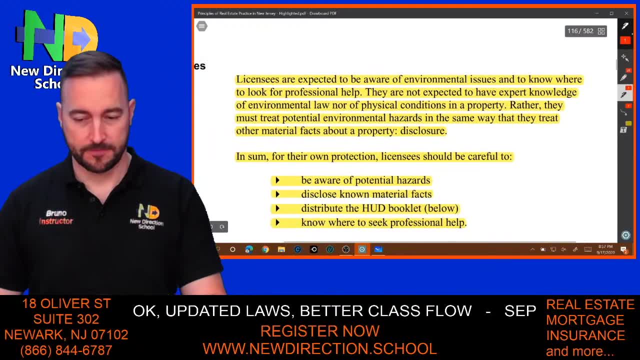 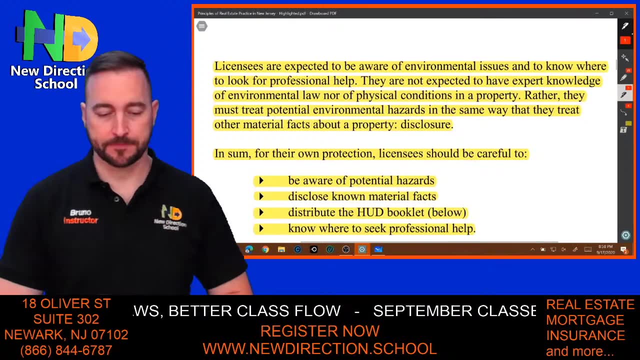 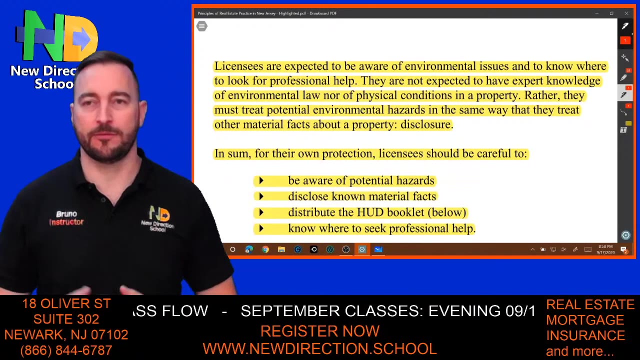 OK, but CERCLA- Comprehensive environmental response, compensation and liability act- OK. so responsibilities and liabilities Again. you're here, probably thinking: why do I need to know all this stuff about carbon monoxide, about radon, about lead based paint? why do I need to know all this stuff? 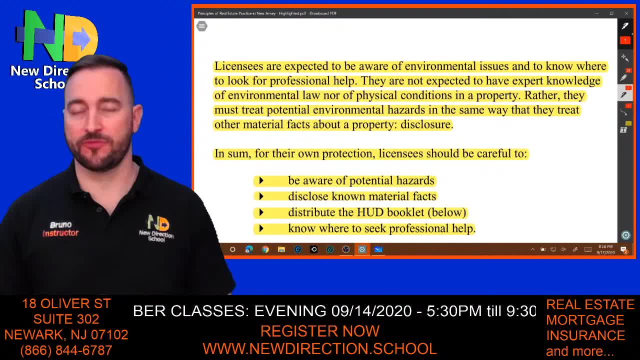 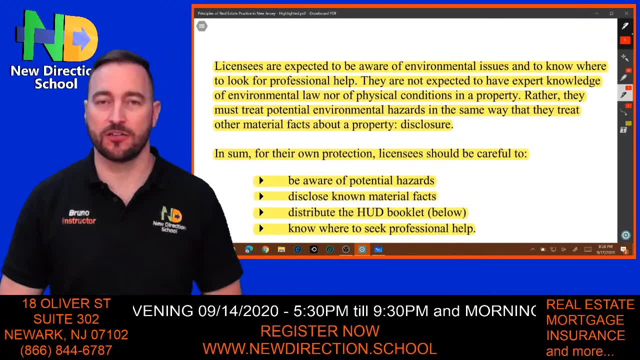 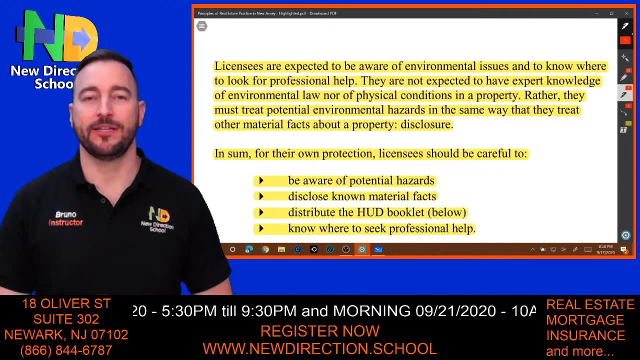 Because, one, you are the professional, correct, That's number one. Two being the professional and real estate consultants. people will rely on you to know these things and at least indicate them on the right path, where they need to go, at least. 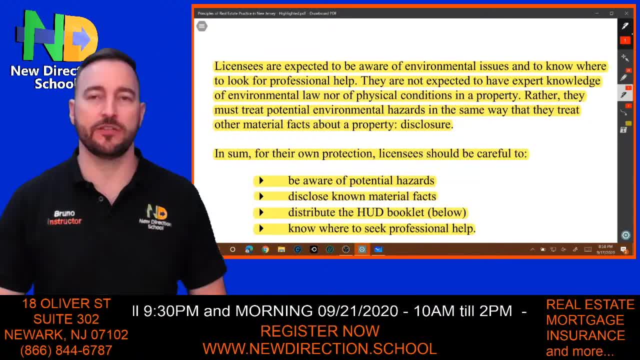 So you don't have to know all these details in detail, but you need to have fundamental knowledge, So everything that you're learning here- sometimes you might question why, But again, fundamental knowledge. OK, so, like Muslima just said, to advise clients. 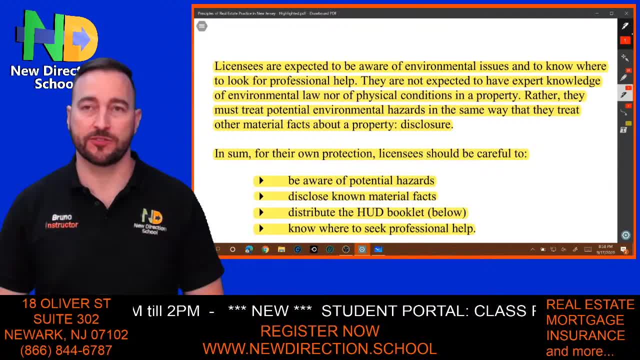 you're not expected, as it says here, to have knowledge of environmental law nor physical conditions of property or whatever, But you need to be able to advise of who can help you take care of these things. So, in sum, for their own protection. 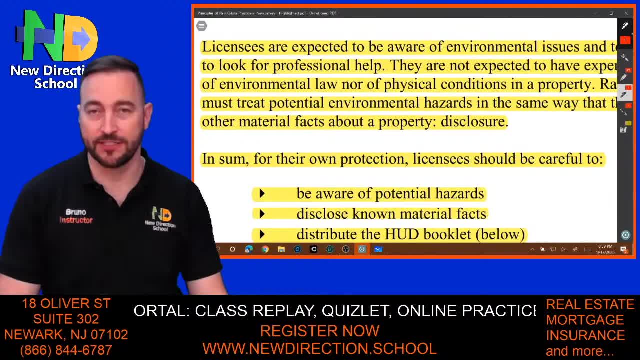 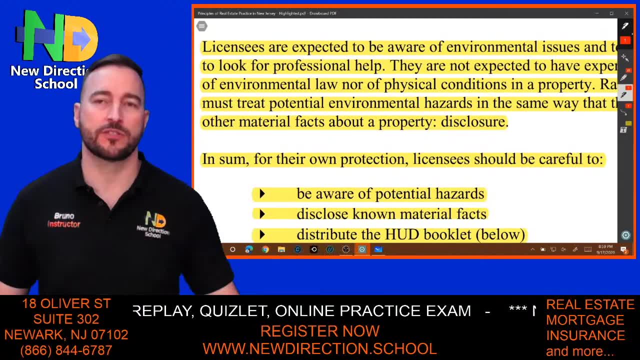 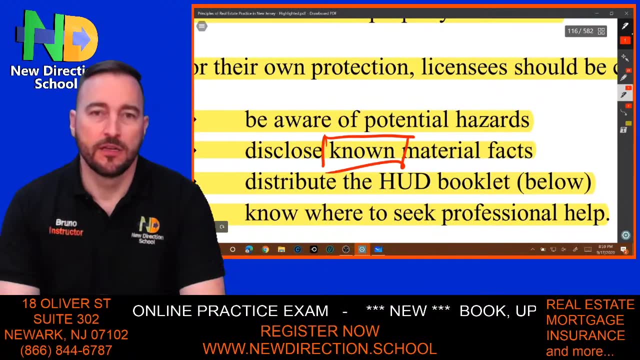 licensees, because you could be liable for not knowing these things as well. Licensees must be aware of potential hazards. We already addressed them. Disclose known material facts. This is key Known. If you don't know, then you don't have to. 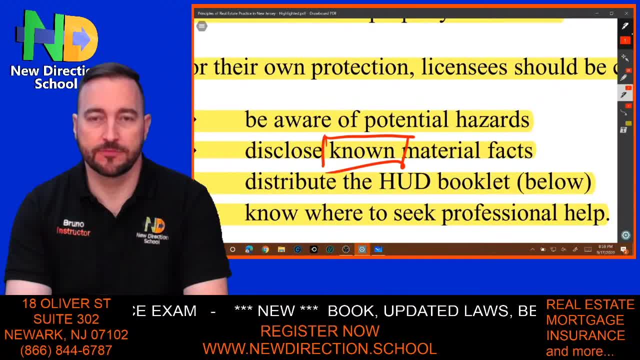 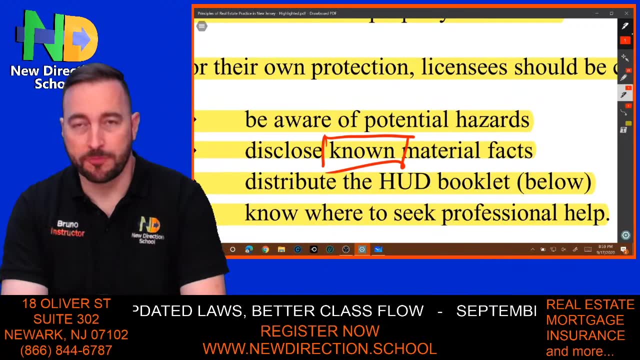 But if you know about it, then you must disclose. You got it. So material facts must be disclosed. OK, you must distribute the HUD booklet- we'll talk about it later- and know where to seek professional help. So if it's an underground storage tank. 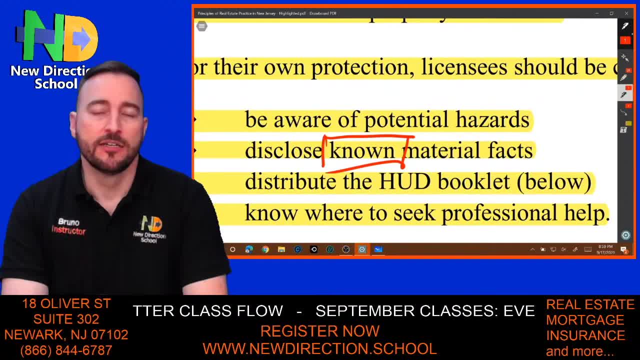 I just gave a contact to one of our realtors earlier today to do a tank sweep, soil inspection and removal And he said, OK, we're going to do a tank sweep, soil inspection and removal of the tank. So you need to know who to go to. 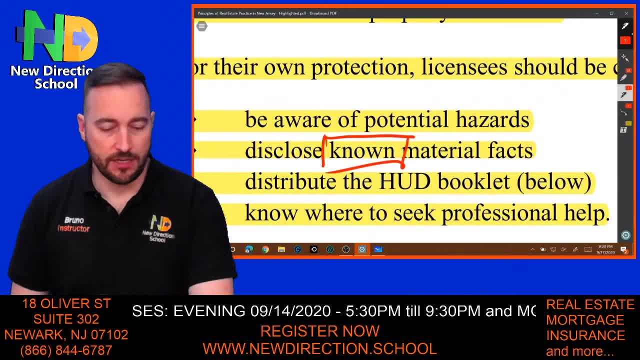 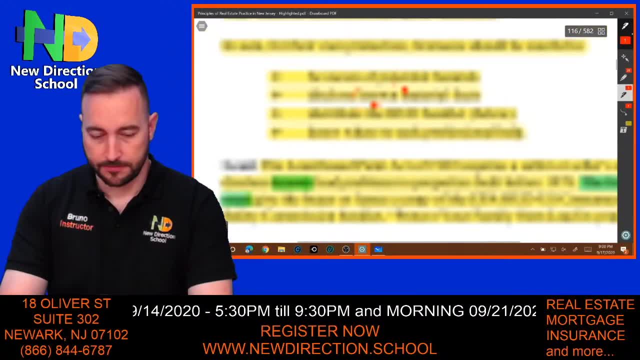 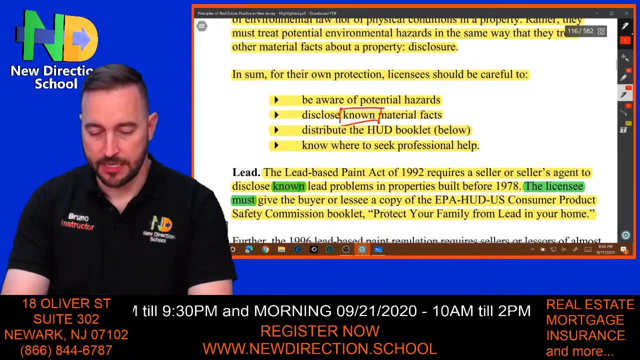 Right, Very, very important. We talked about asbestos. You need to know that you cannot do yourself, You need to have somebody certified to do the work, and so on. We did talk about lead, Lead-based paint. It was banned in 1978.. 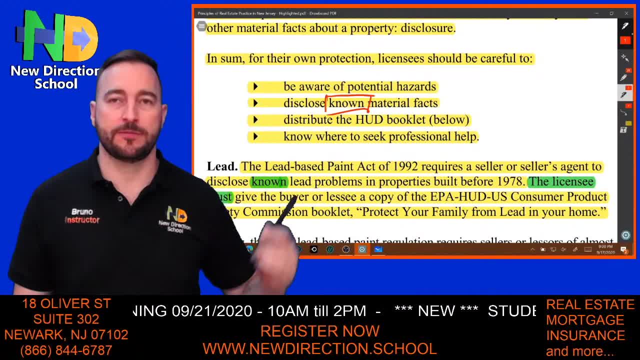 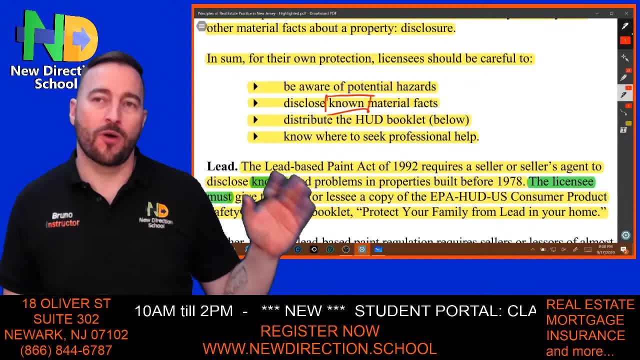 The Lead-Based Paint Hazardous Hazard Reduction Act, which is called Lead-Based Paint Act, of 1992, requires the seller- So it was banned in 1978, but requires the seller or the seller's agent to disclose Again. I have it in green, which is very important. 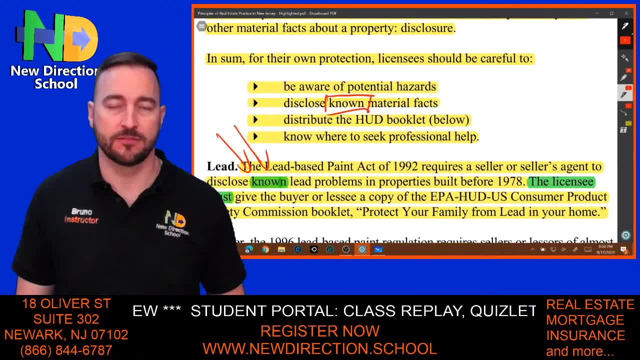 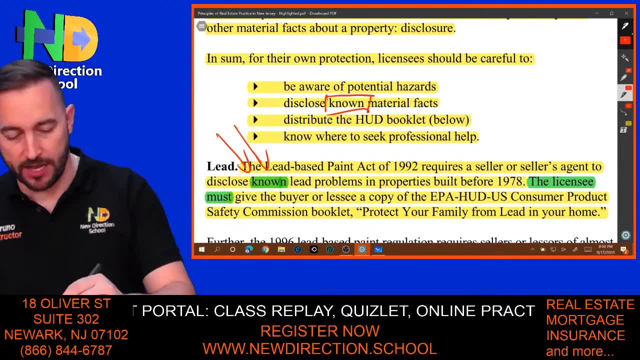 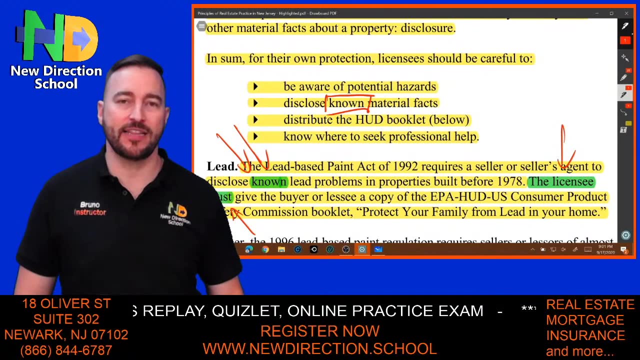 Known. If you don't know about it, you don't have to test, But if you know about it, you must disclose. OK, The licensee. So you guys, very important- must give the buyer- Or let's see So, even tenants must receive a copy of the HUD or EPA, HUD's Consumer. 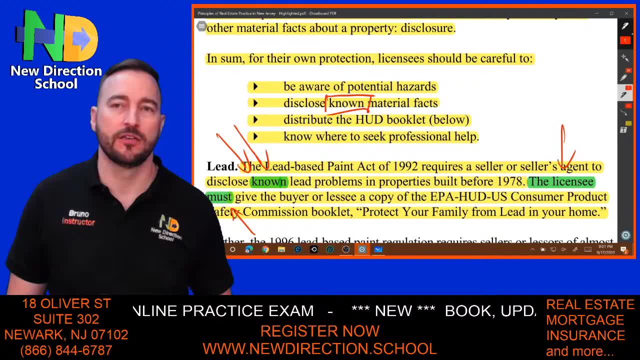 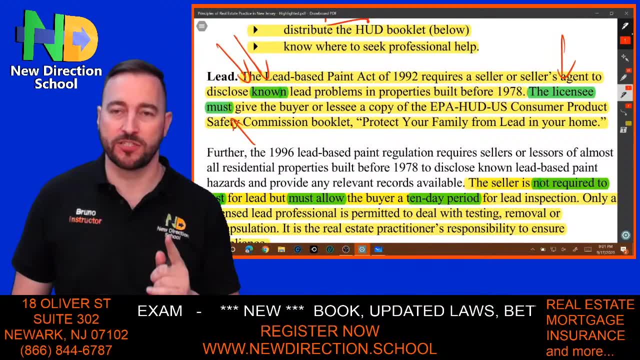 Product Safety Commission booklet. it's called protect your family from lead in your home. So this must be given to every tenant or buyer must be given. Take note of this because you have to have. this Must be given to every tenant or buyer of any. 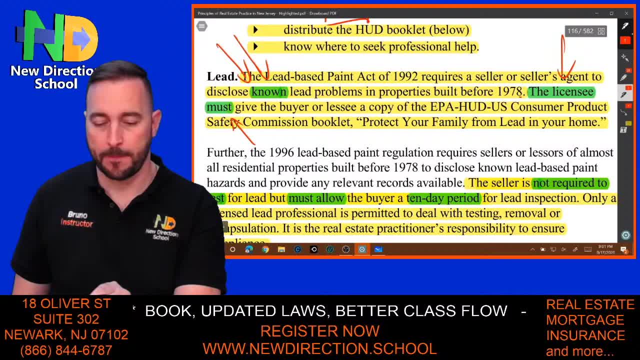 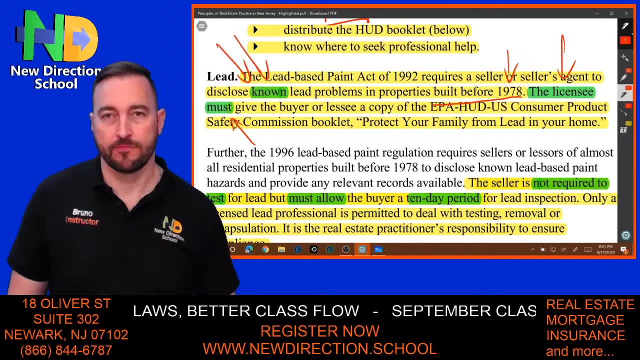 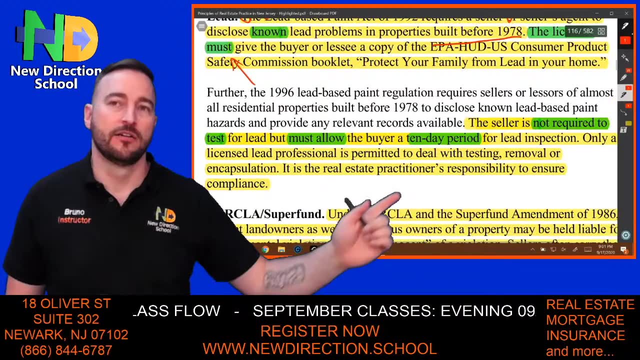 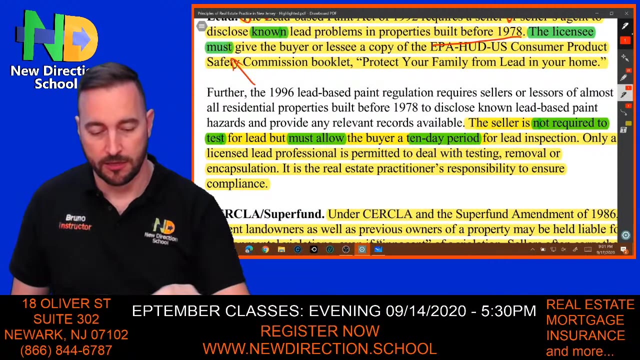 property that was built before 1978.. OK, Not only that, You have to provide a pamphlet, you have to provide a disclosure in the contract and the seller is not required to test. Look, I have it in green. It's not required to test, but must allow the buyer a 10 day periods. 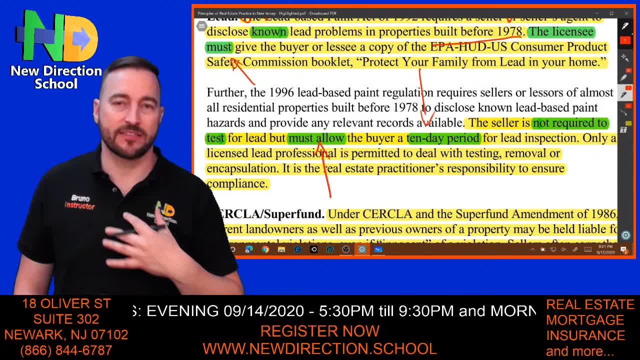 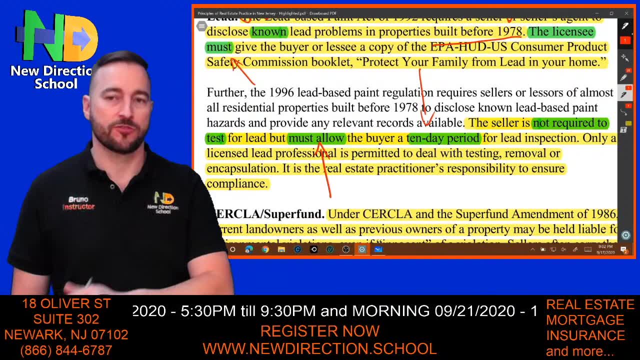 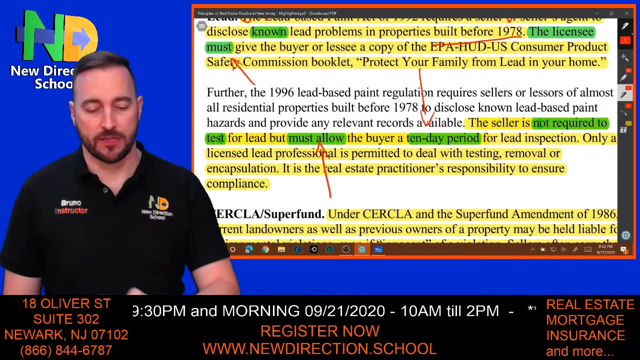 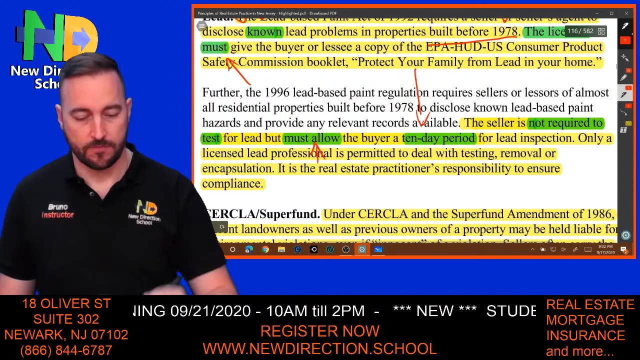 to conduct an inspection. So as a seller I'm not required to test Right, But I cannot force you into the contract without testing. I must allow you a 10 day calendar day period to inspect for lead. OK. And then it says right here, the very last sentence: 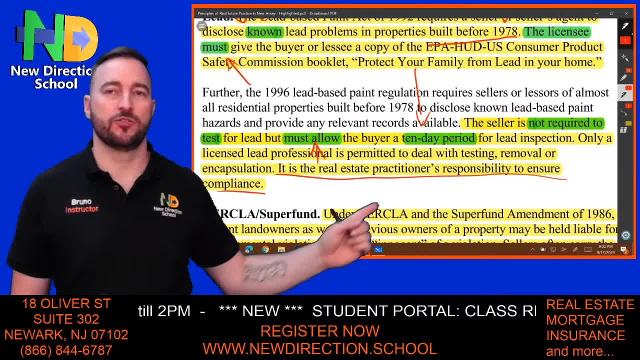 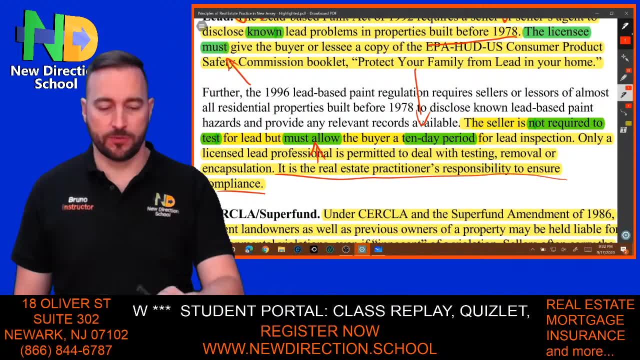 It is your responsibility, Realtors. it is your responsibility to make sure everybody complies with this. It's on you. So this one is probably the most serious one you guys need to remember, because it will be with you for the rest of your realtor life. Even if you live 100 years right as a realtor, they're still going to be properties that were built in 1978 by the time you reach your 100 years as a realtor. OK, So this will be always with you. 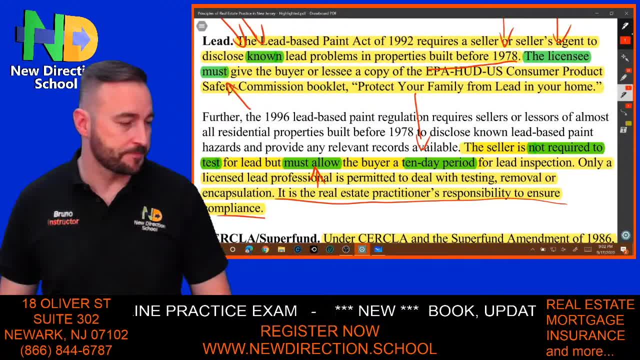 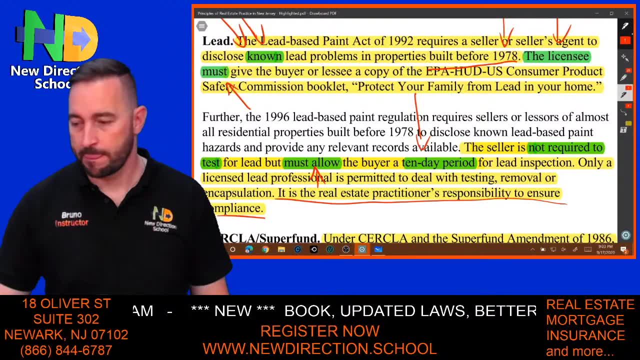 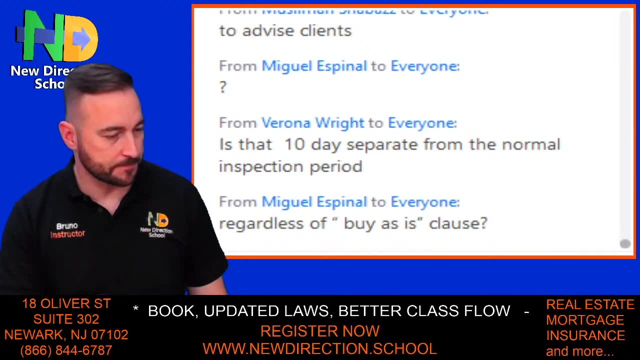 There's a lot of properties, older properties, built. Miguel has a question coming through. All right, let's address that. Laura, if you have any questions, or whoever's watching on YouTube. if you have questions, drop them as well. Is that 10 days separate from the normal inspection period? 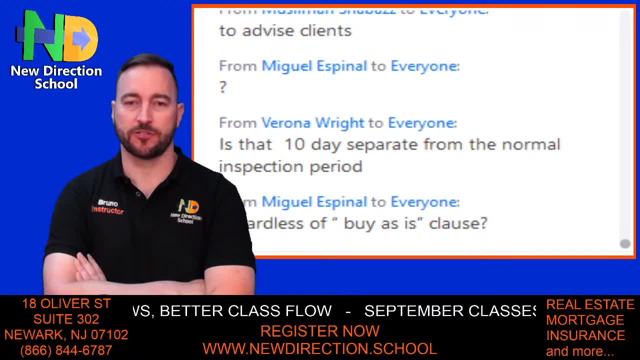 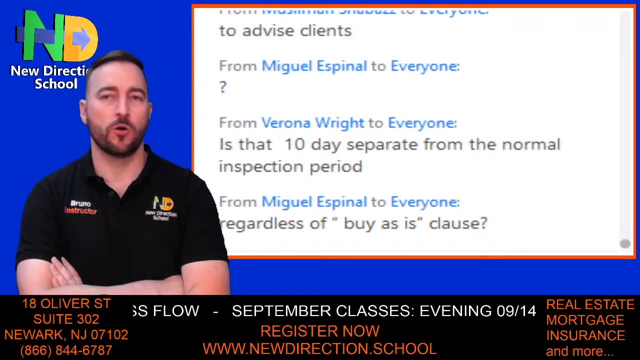 Well, First of all, there's no normal inspection period. It actually is a blank in the contract And we decide what the inspection period will be, So nobody is required to inspect. So when we give, let's say, 14 days inspection period or 10 days, 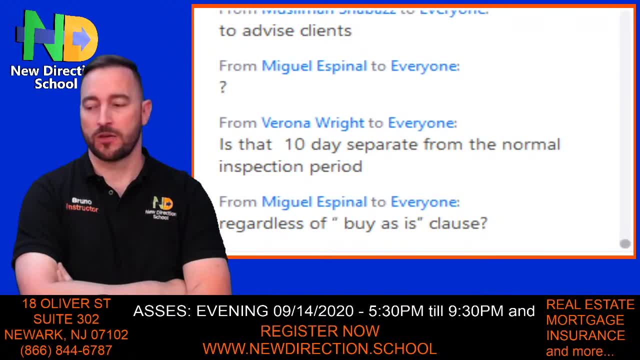 whatever you want, we get 14 days or two weeks when you give that time period for inspections. In this case it's already included the 10 days. The reason why we give the 10 days most of the times: most agents. 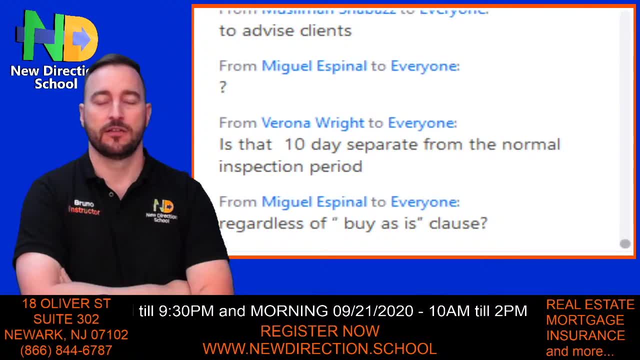 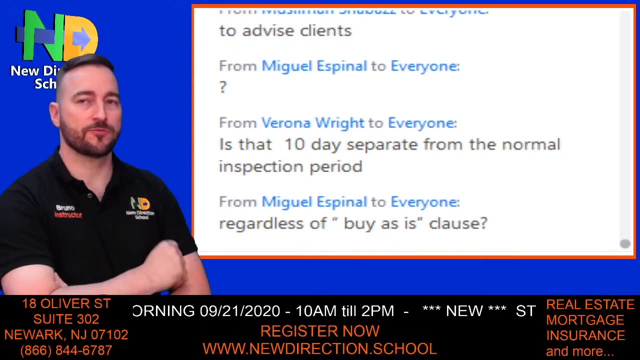 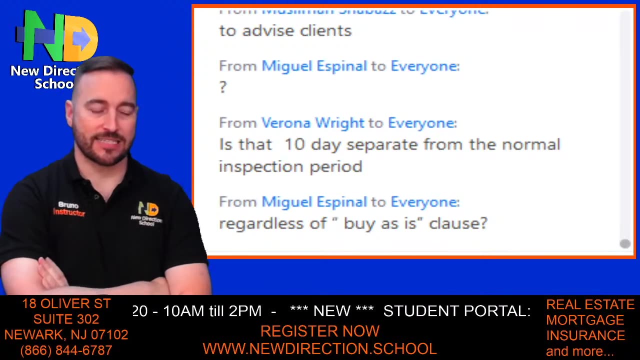 give the 10 days is partly because of of this issue. Yep Lab-based paints Miguel says: regardless of buy as is clause. now you're getting into a different ground. So, As I said yesterday- OK, I think it was- it was yesterday or two days ago. 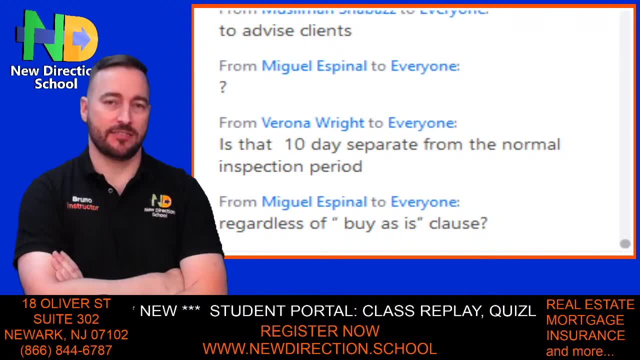 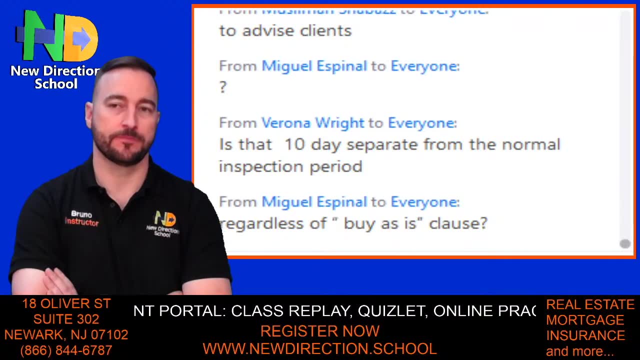 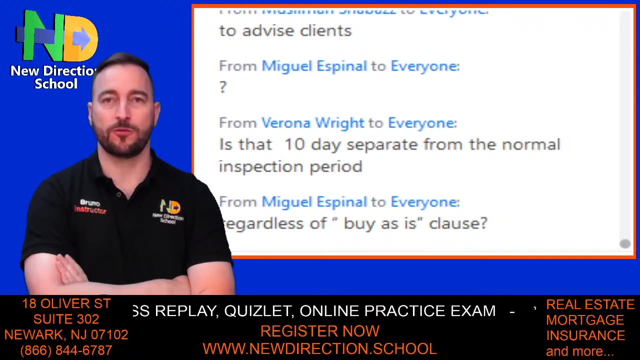 as I said to you guys, when you buy as is, you're buying the current condition of the property, as long as it's not structural. Lead-based paint is not structural- OK, not structural. But the buyer, the buyer- must still be aware of lead-based paint hazards and have the opportunity to to inspect. 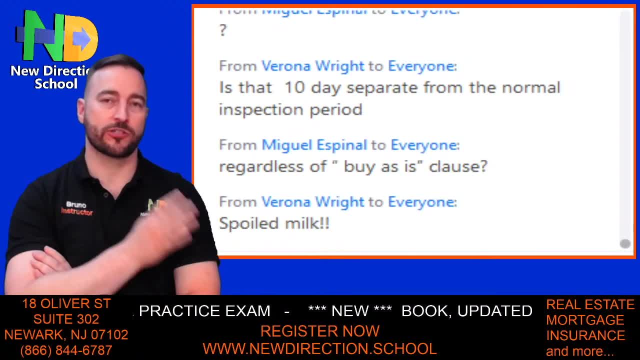 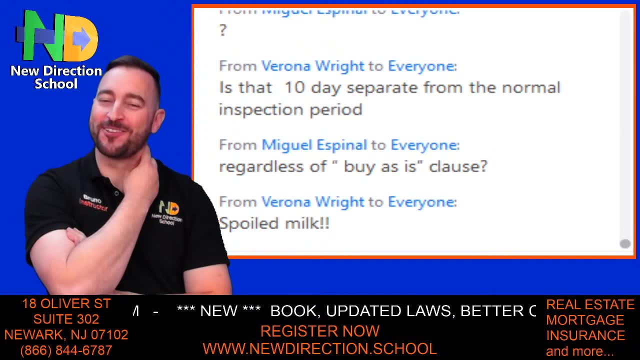 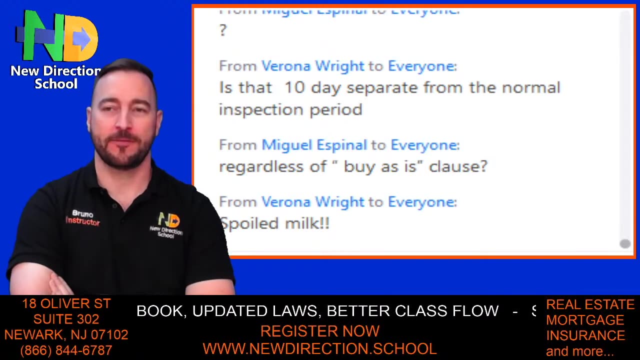 So, even though it's not structural, it's one of those clauses. No, That's right. So it's one of those clauses That still force you to to get it done. Yep, Got it. So, regardless of being as, as is for lead-based paints, 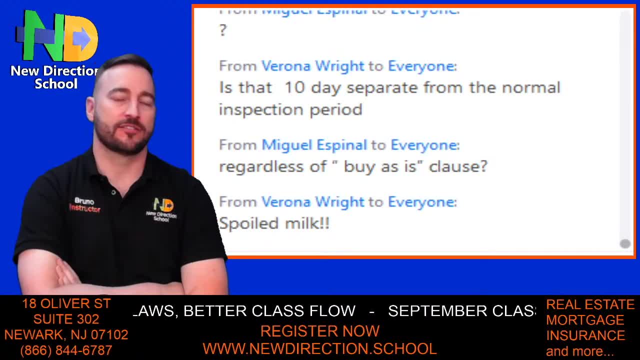 the only other condition would be structural. that's still. you're still liable for it. It's almost like the lemon law for the for the cars You could buy. a car six months later breaks down If it was something that was already existing and was not from normal wear and tear. Right. 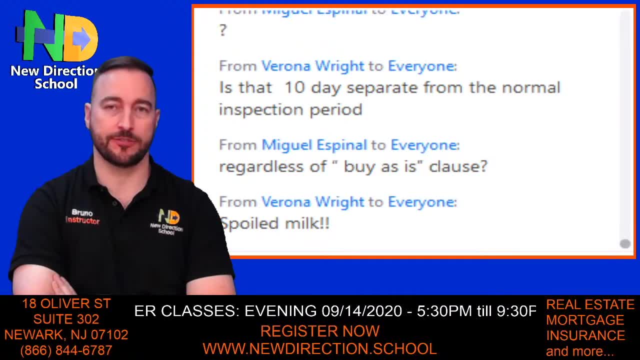 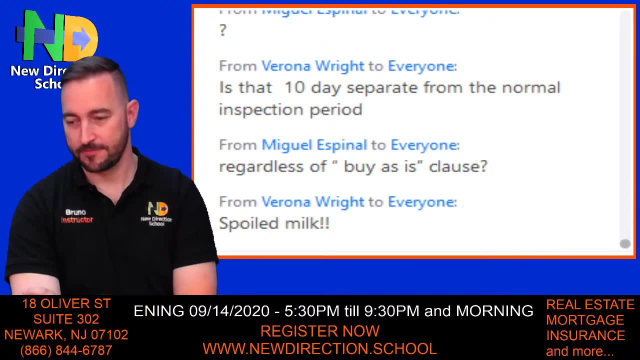 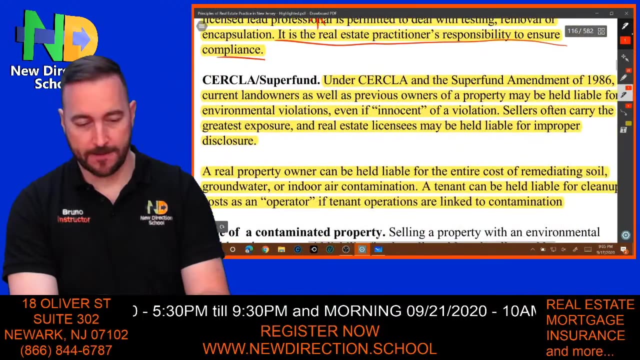 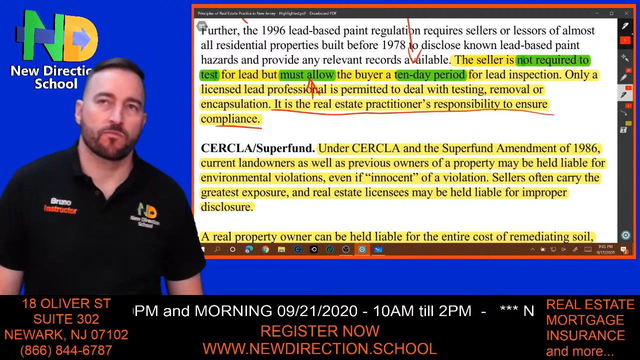 Right, You might have A way to get compensation That makes sense. So, no matter what, in this case you have to Circla. So I was talking about Circla guys. Circla was enacted or enacted in 1980, and then Sarah came along, which is: 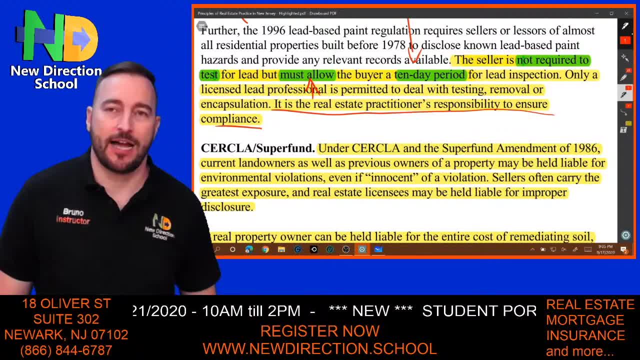 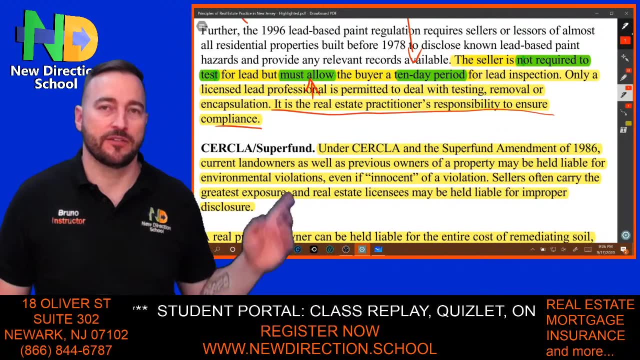 superfund amendment And then we had three enacting the act And it was 1986 or six years later And what I think happened, I tell everybody what I think happened is a lot of homeowners sued the EPA because of Circla. See, Circla was created to to take care of environmental issues. So if there's a there's a spill on your property that could affect the environment, CERCLA would activate what's called the super fund, and it's money set aside by the government. 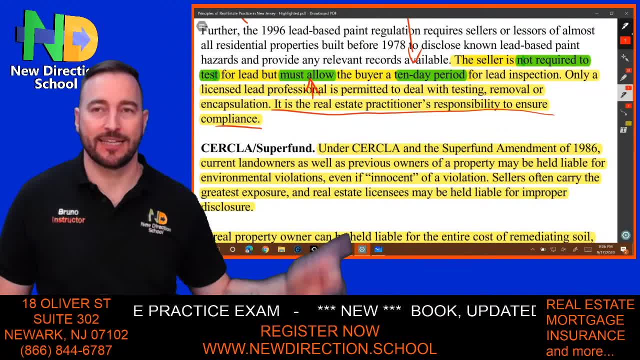 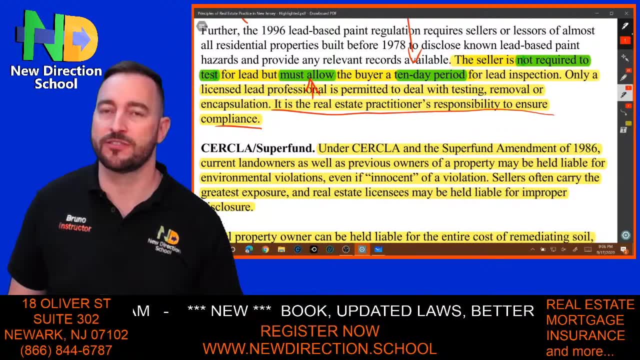 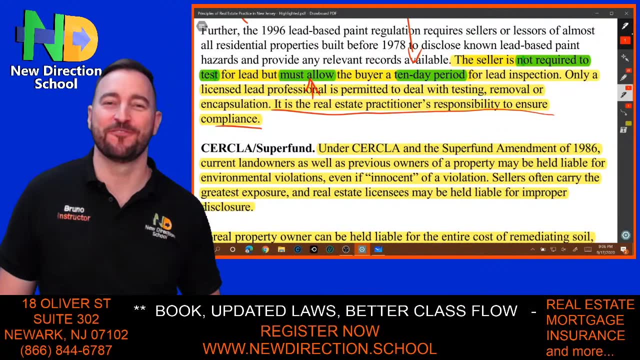 to clean these things. the problem is, as it says right here: current landowners as well as previous owners of a property may be held liable for environmental violations, even if innocent of a violation. bless you. so, even if it's not your fault, even if it's not your fault, you could be held. 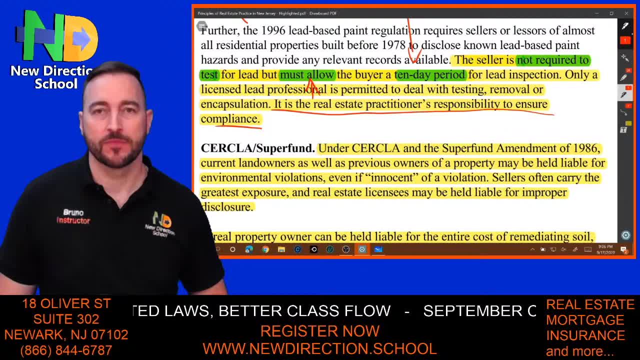 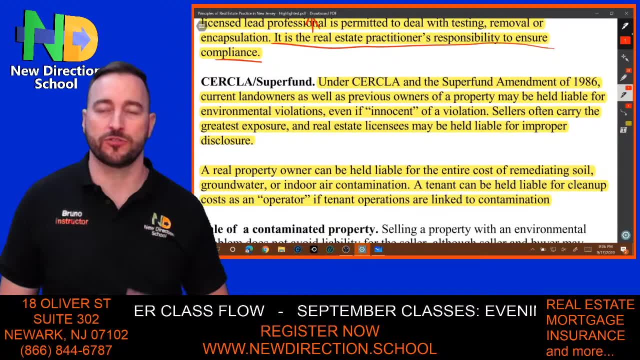 liable for the cleanup. okay, so sellers often carry the greatest exposure and real estate licensees may be held liable for improper disclosure. so if you know there's an issue, talk about it. so very simple: anything and everything that affects the proposed transaction must be disclosed. as simple as that. if you know something could affect the value of the property. 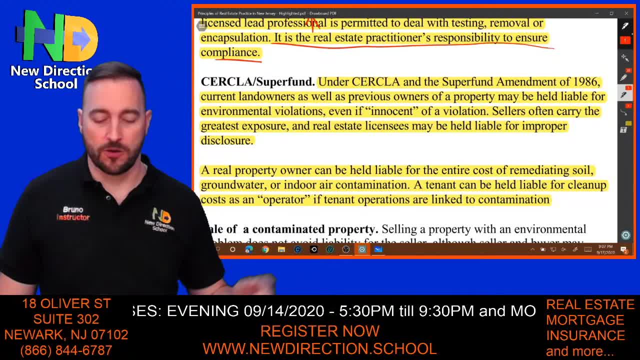 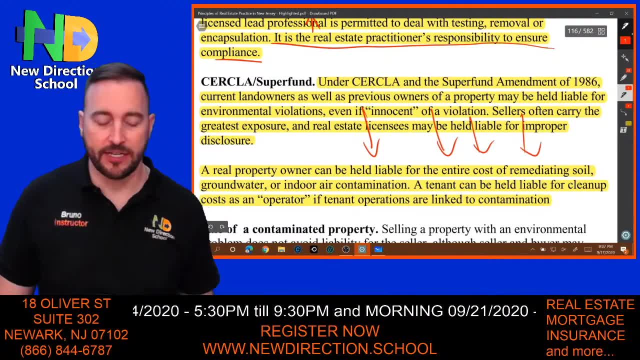 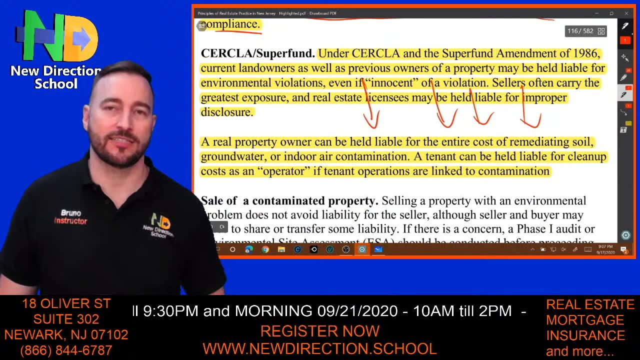 must be disclosed so a real property owner can be held liable for the entire cost of remediating soil, groundwater, indoor air contamination. a tenant could be held liable for the cost as an operator. this is mainly for for commercial right if tenant operations are linked to contamination. 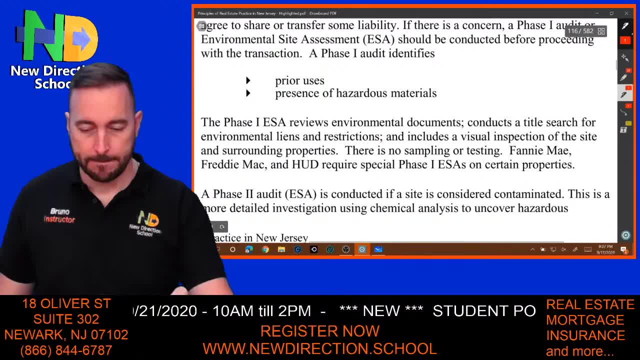 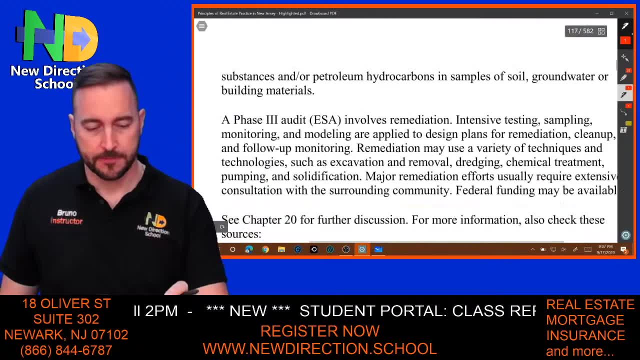 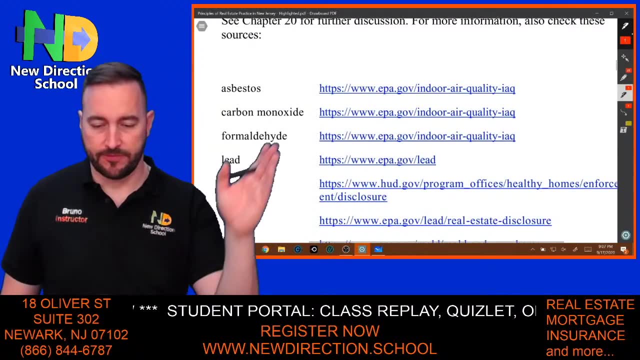 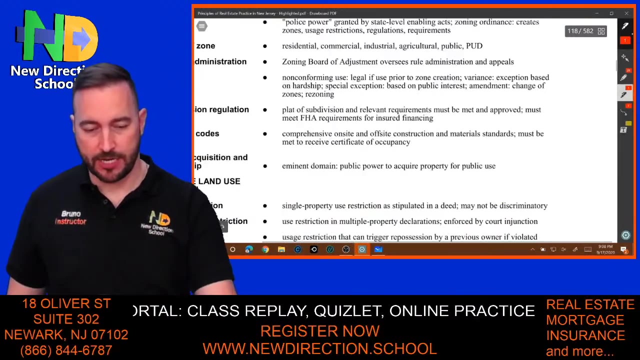 there's different type of testings: phase one, phase two, to figure out the condition of the property, right, and these are links you have in the book if you want to know more about it. oh, and that's it. we are done with this chapter. not bad nine ten. who wants to do one more chapter? 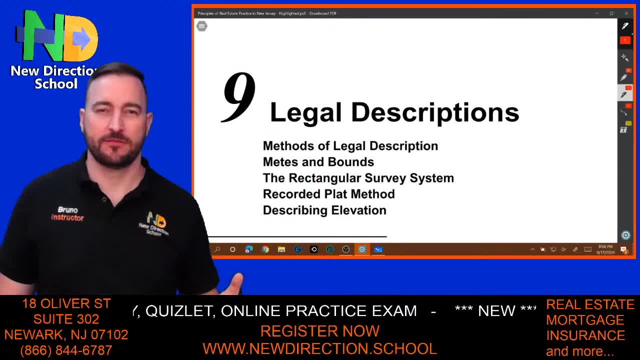 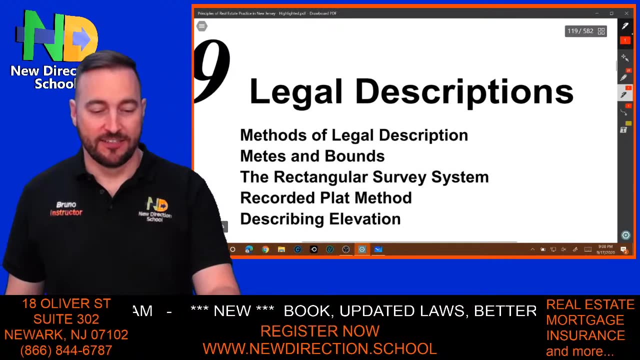 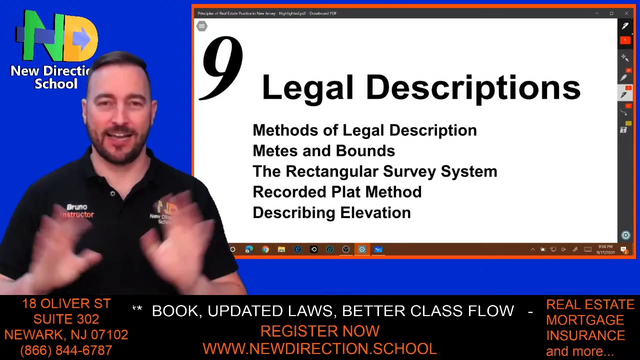 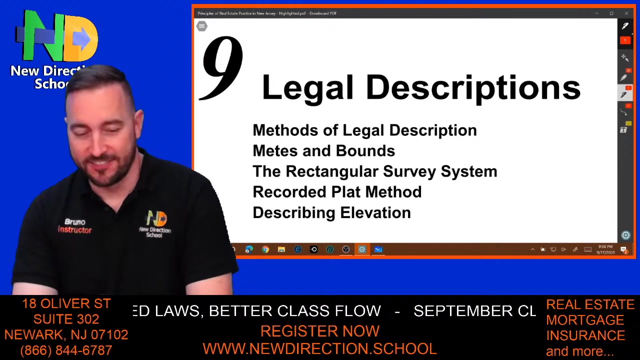 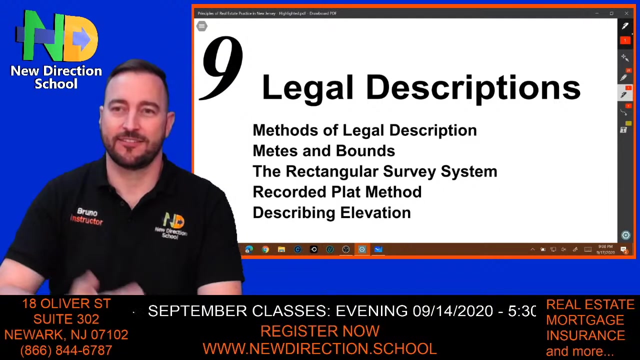 nobody come on until midnight. we still have enough time. no more chapters. no more chapters. no more chapters up. Don't be disappointed, please don't be disappointed. but tomorrow, uh, there's not going to be a class. Alright, thank you and goodbye, don't be disappointed. but why are you going like this? but you're going to be like, oh my god, why? 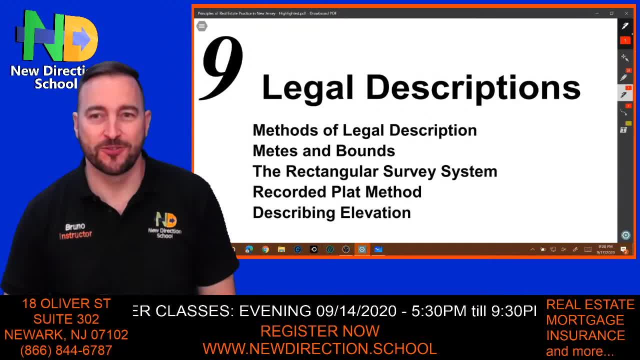 uh, so i'm going to give you guys a chance to- to celebrate, i mean to study, uh, the first eight chapters, uh, to ask me any questions, so send me. um, i have something that i have to do and unfortunately i might not be back on time, so i prefer to cancel versus um, yeah, well, it has to be. 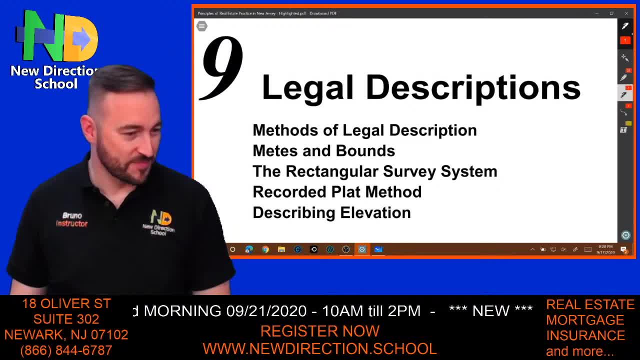 sorry, um. miguel says wasn't going to be able to get on tomorrow. robin says: good time to study. there you go. do we have to make up the hours? no, east of funny. no, okay, um, so don't worry about it. uh, let me. let me tell you real quick about the hours again. 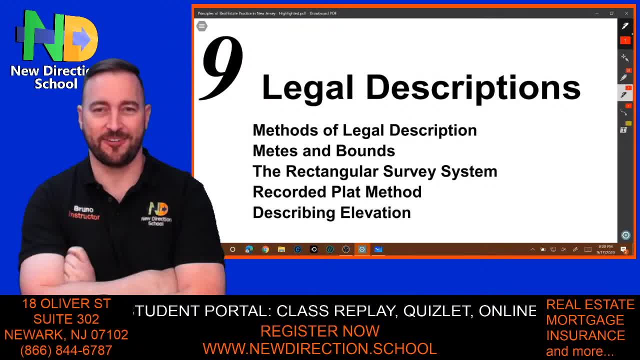 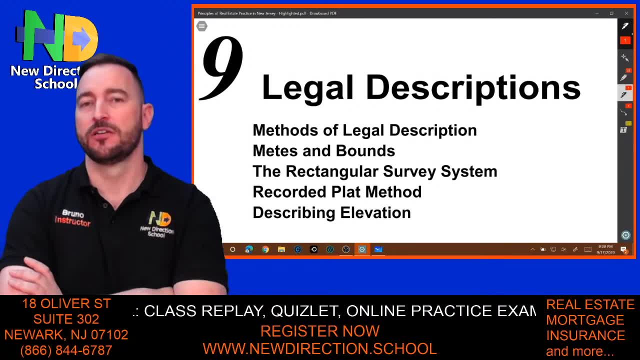 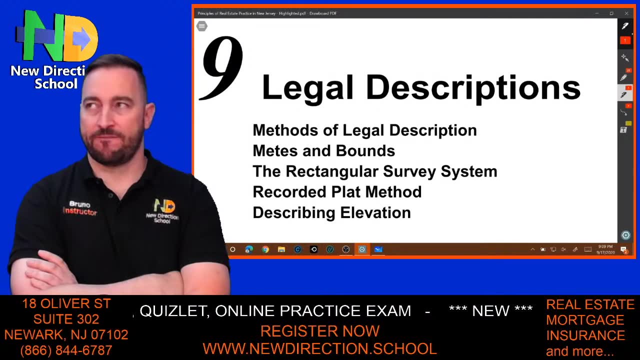 and vanessa is vanessa, the matters is sad, oh, i'm sure. uh, let me tell you about the hours again. the 75, 75 hours is what the real estate commission believes to be enough to cover everything i have in in the. in the four weeks that we established, i have put enough, um, enough time. 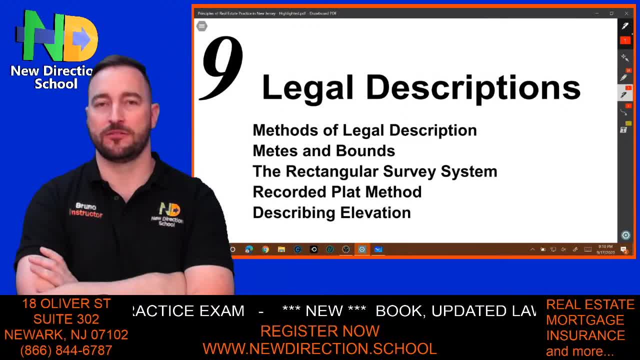 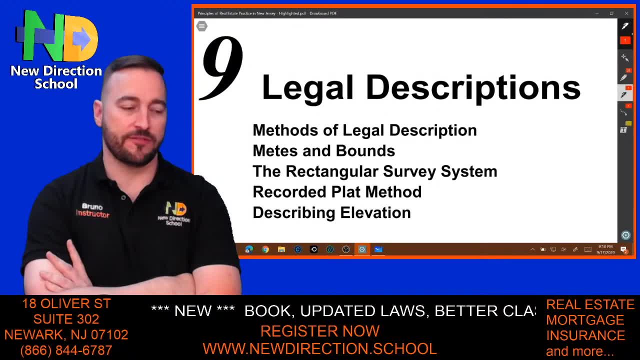 enough cushion for us to go over all the chapters and still do all these q and a's and stops, like i do, and ask a bunch of questions, move forward and so on. right, so there's enough. um, enough time there, so don't worry about it. the 75 hours are covered. 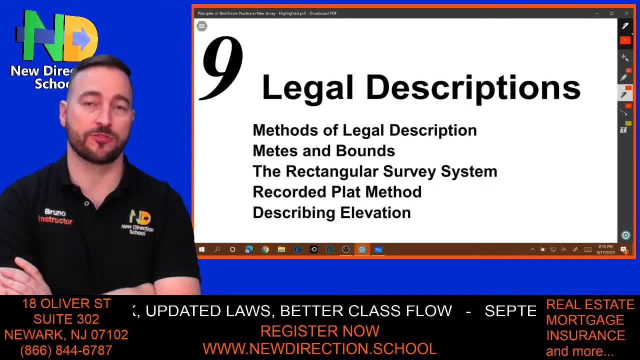 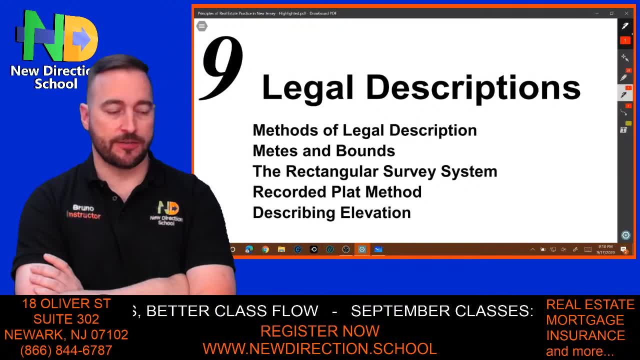 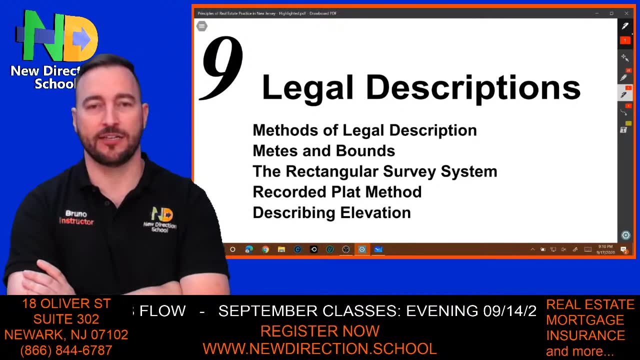 what i'm concerned about is you doing all the chapters. so if you miss chapters, you have to make them up. that's the only thing. okay, take advantage of um of this time off to to review everything. so don't go like, oh, it's friday night, i'm gonna go out. don't do that. it's only a couple weeks. 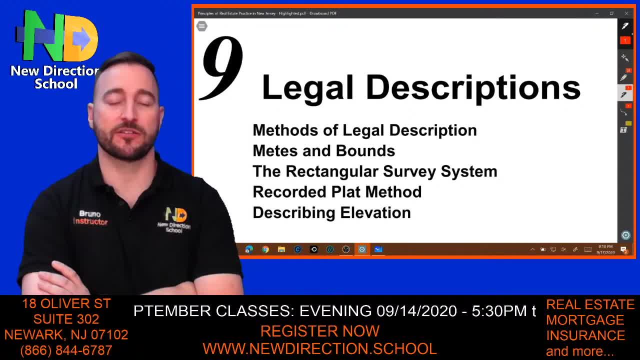 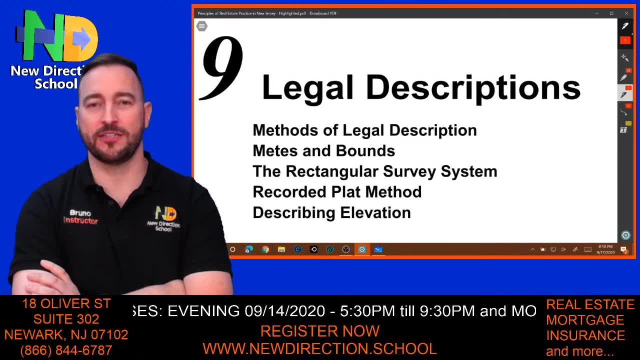 don't go out, don't go party. focus on this, because on the fifth week you're going to take the exam. on the sixth week you're licensed and that's it, we're done. then you can start making money and you can party as much as you want. that's up to you and your work ethic. after that, okay, but for